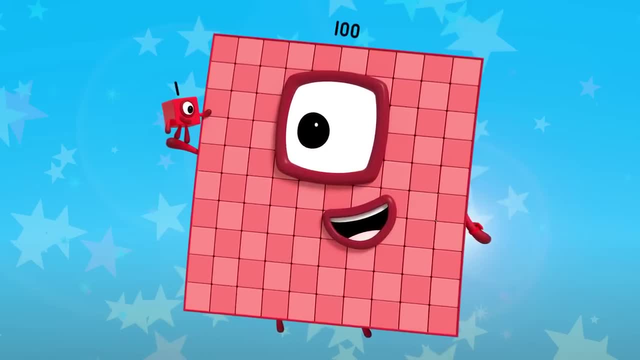 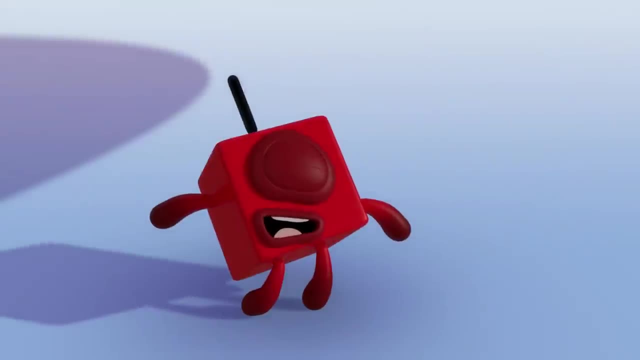 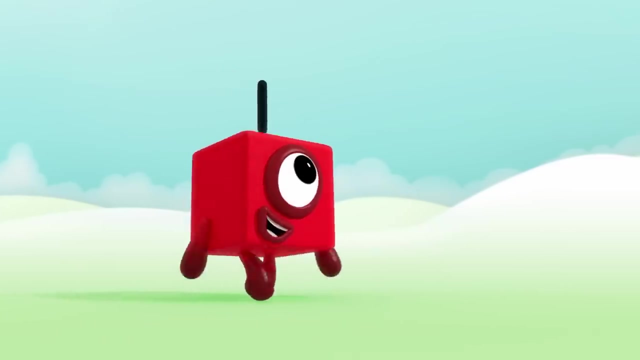 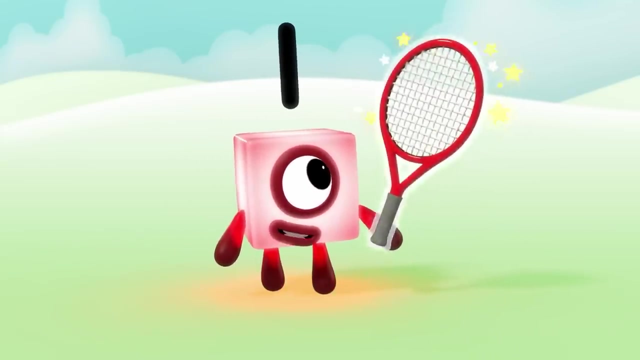 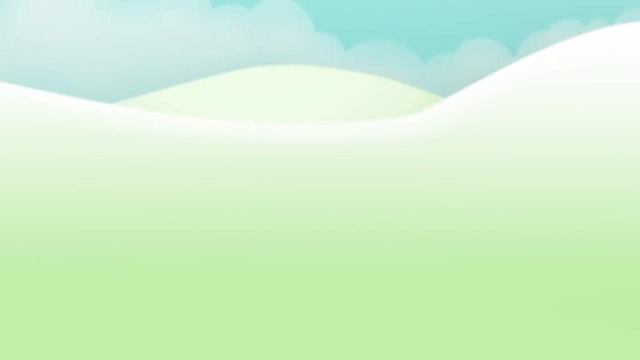 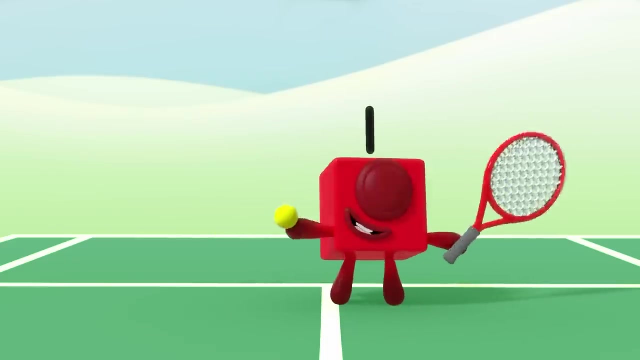 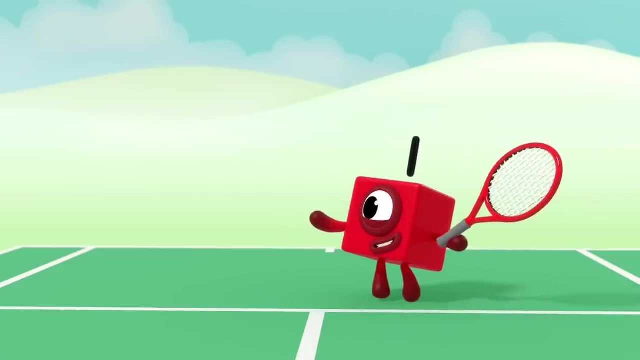 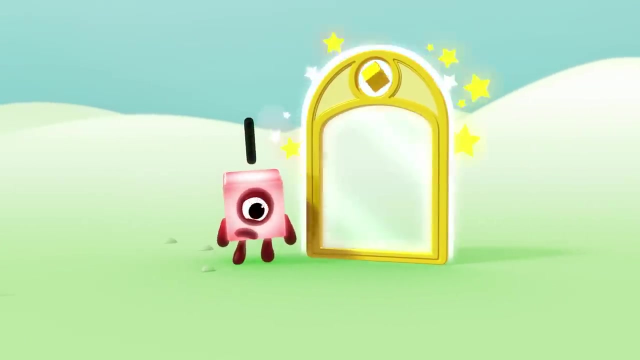 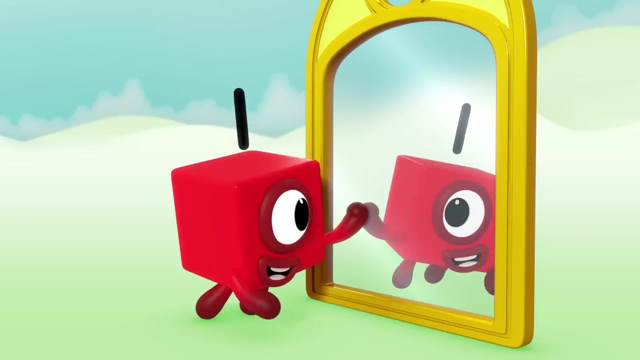 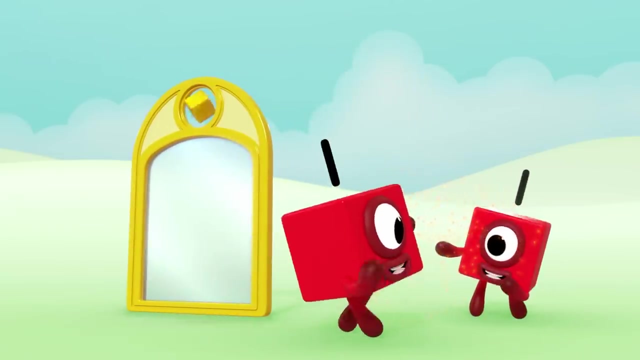 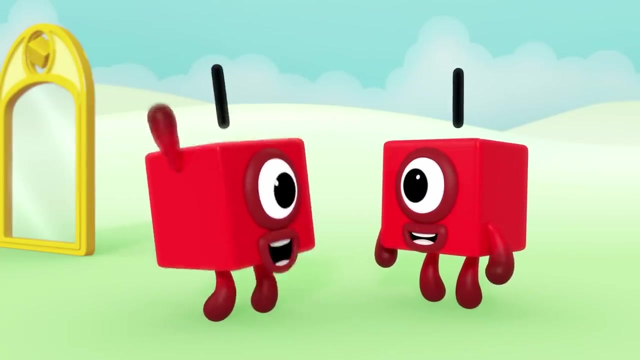 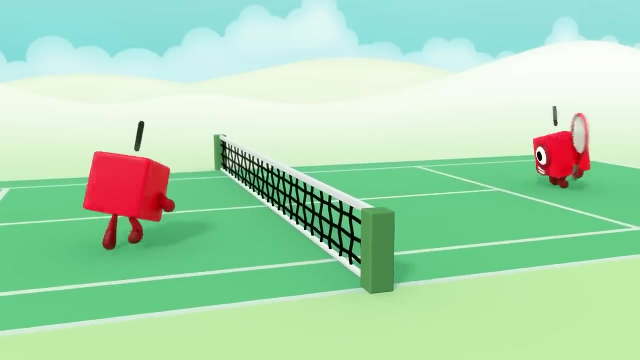 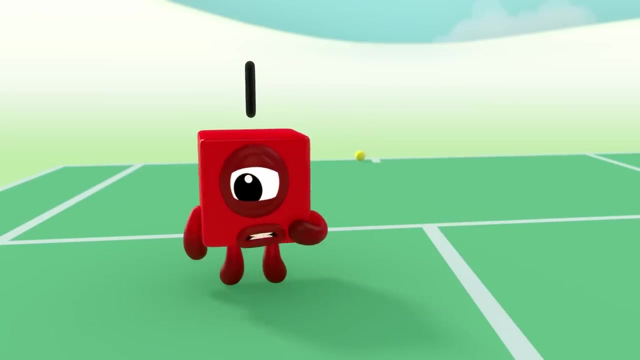 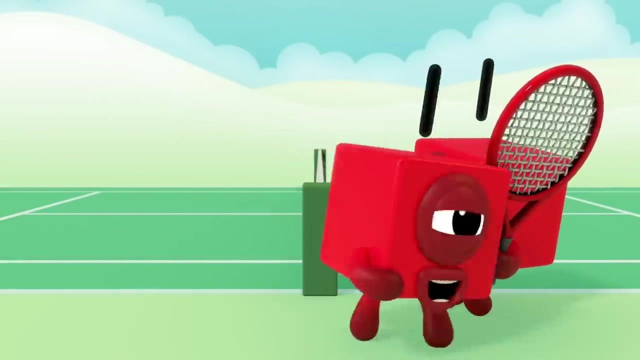 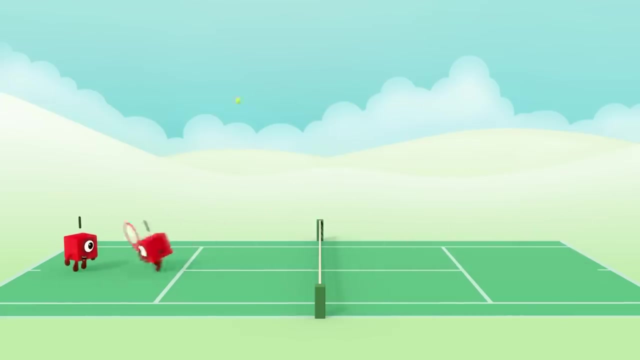 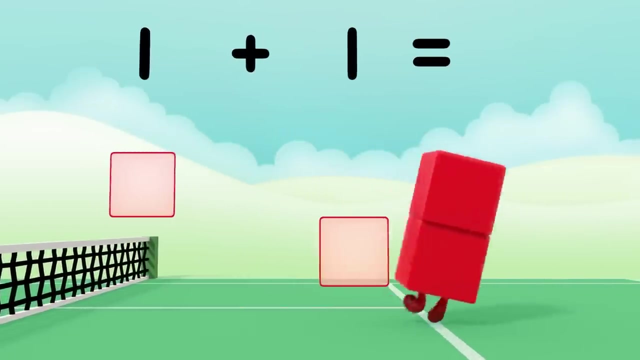 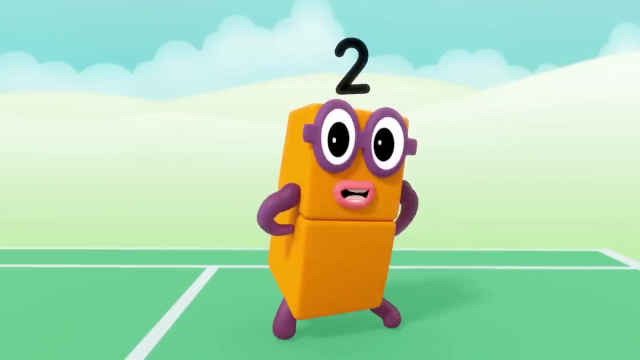 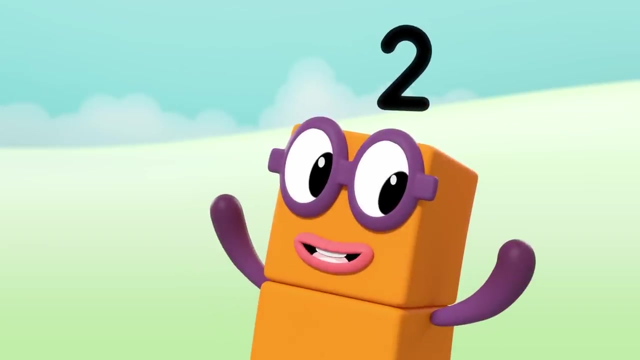 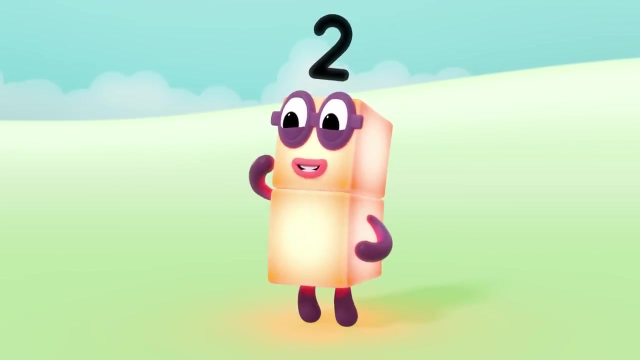 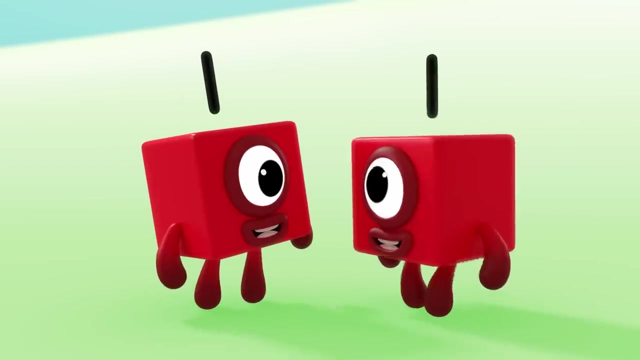 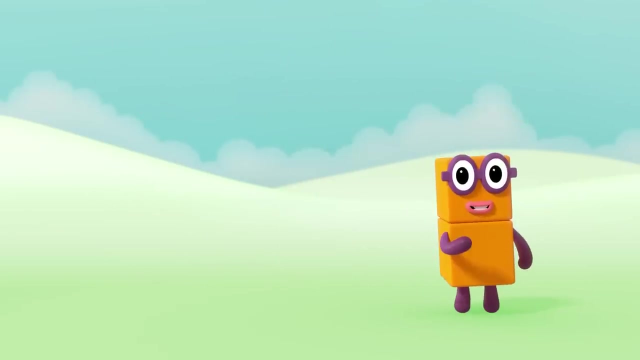 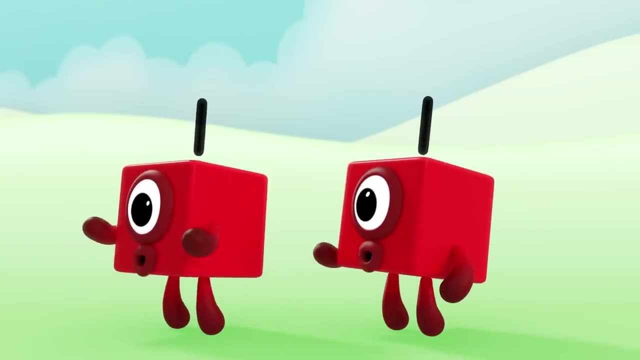 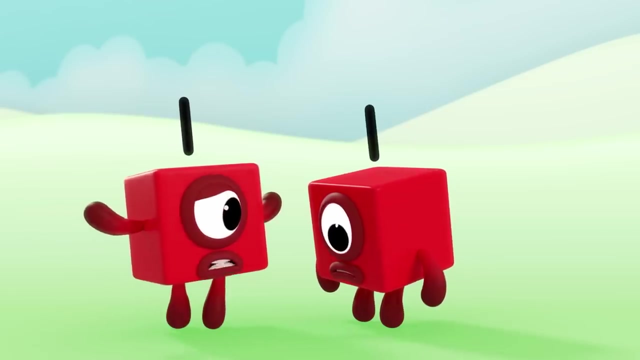 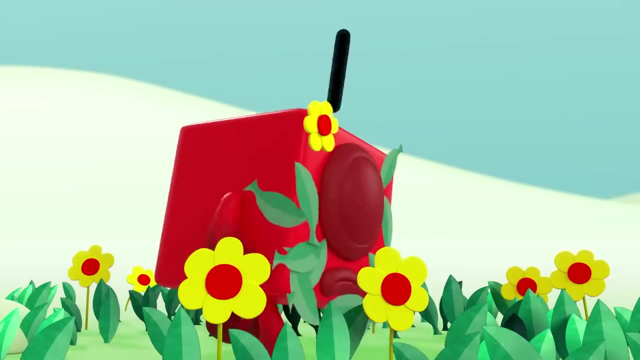 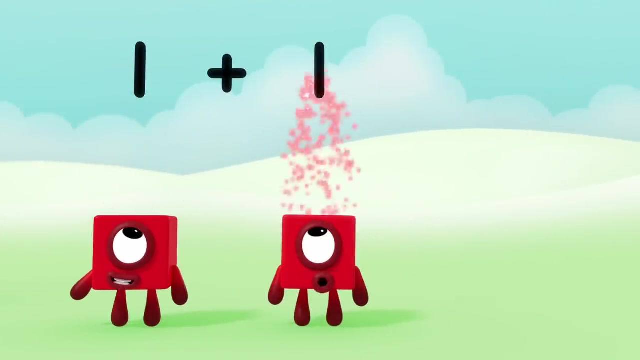 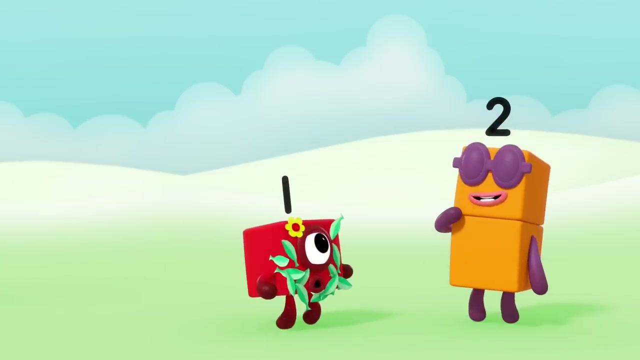 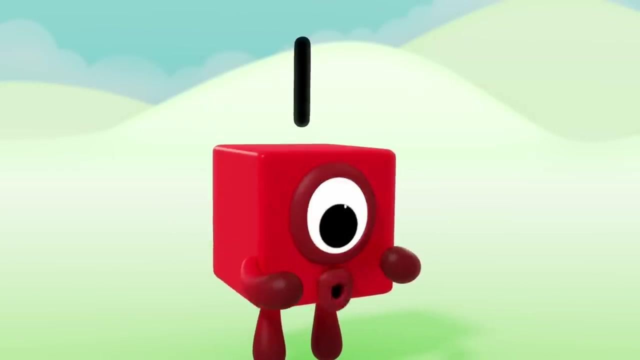 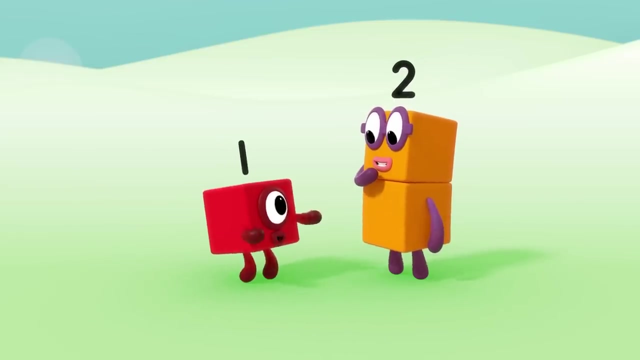 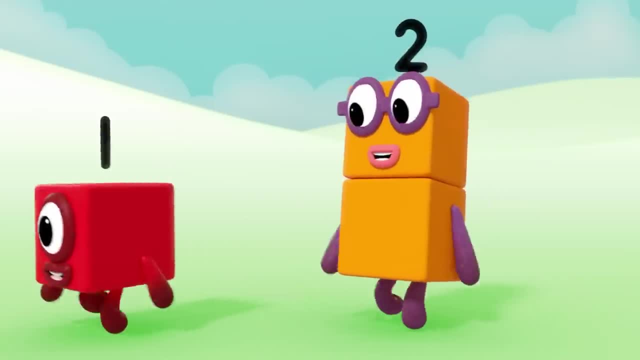 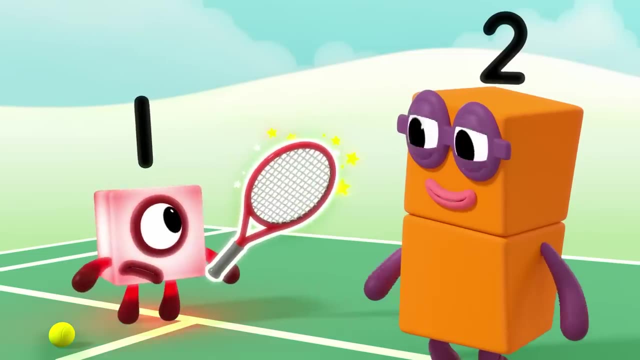 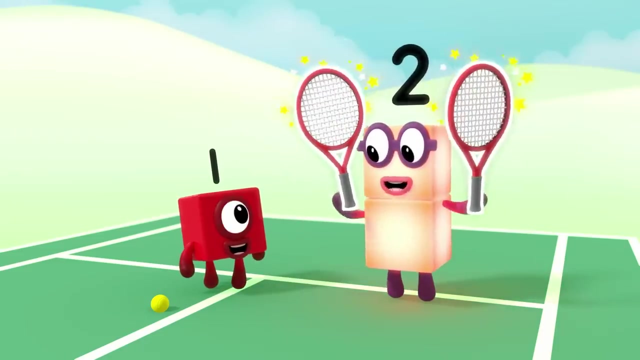 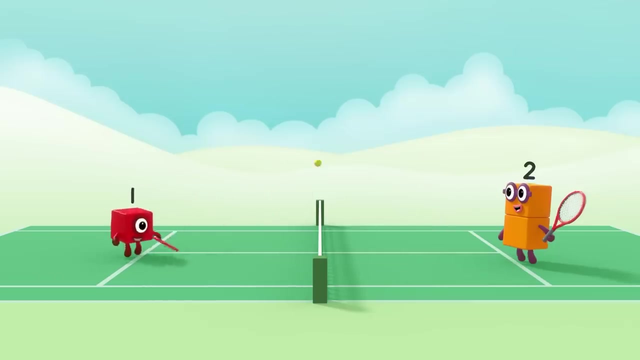 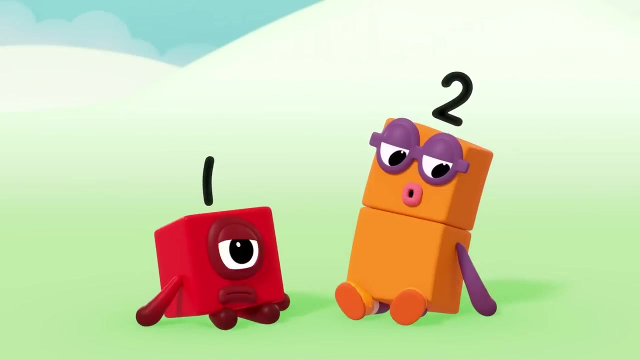 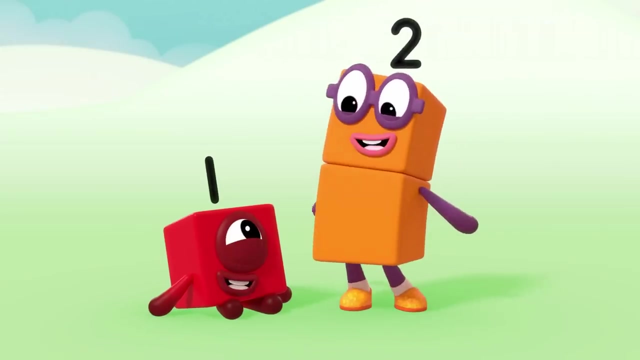 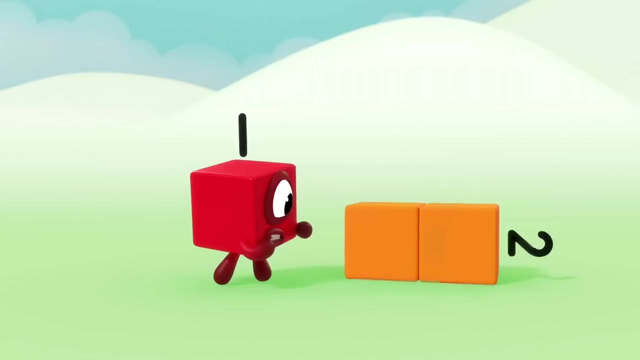 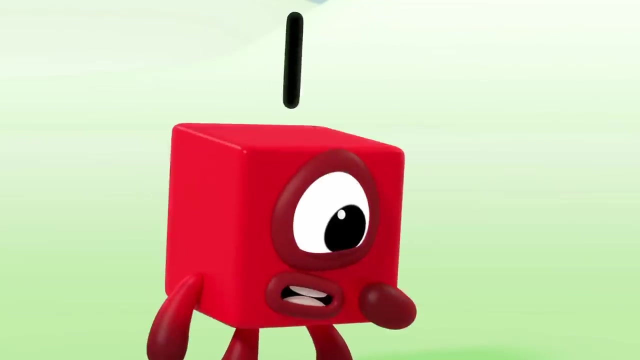 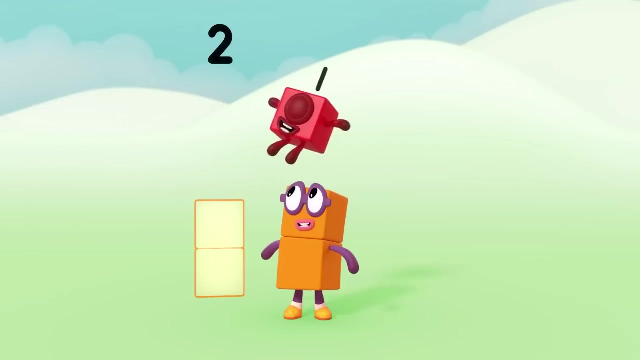 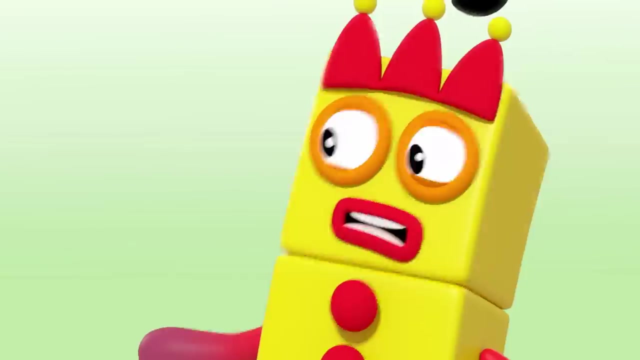 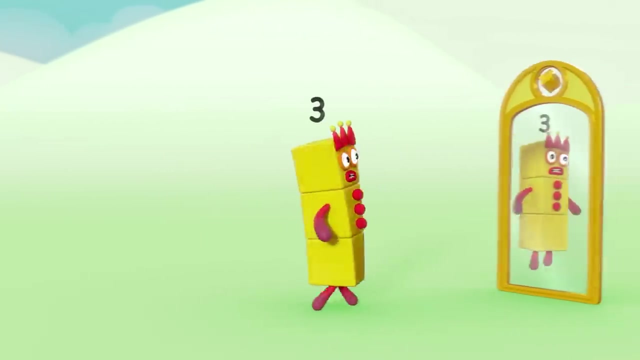 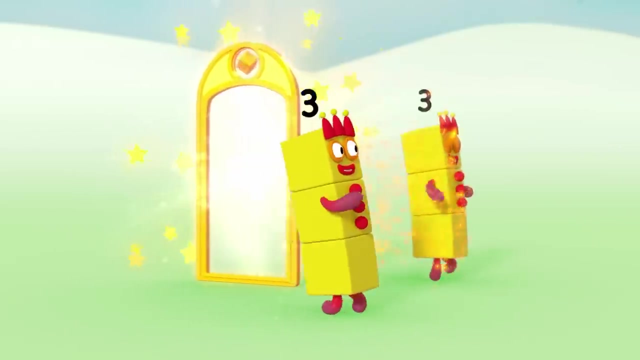 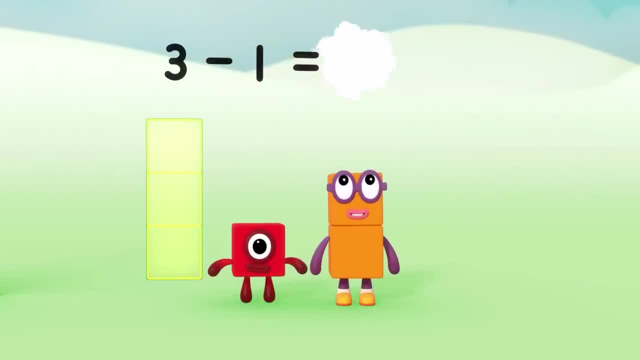 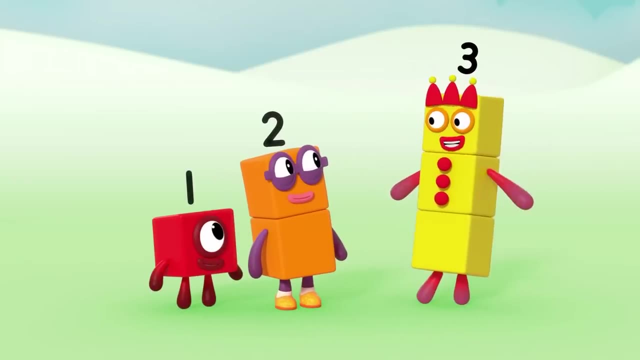 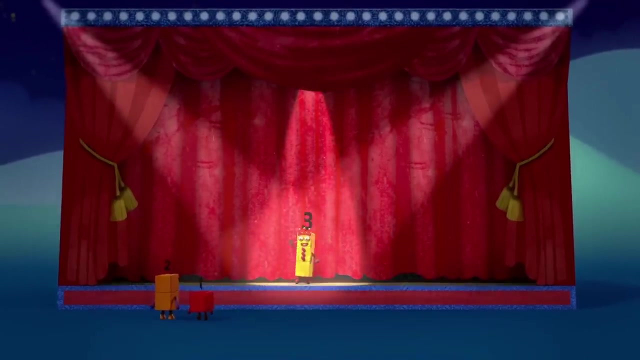 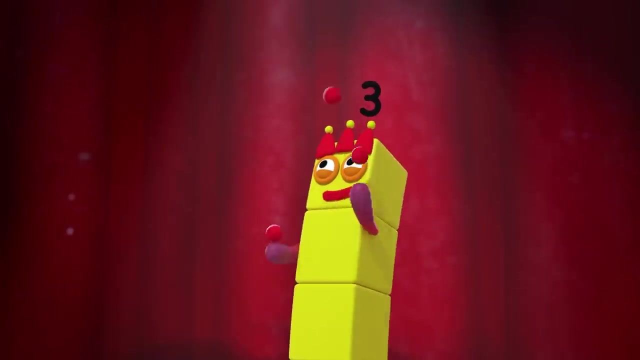 Three minus one equals two. My audience, That's better Ready. One, two, three. One, two, three. Everybody, look at me. I'm here to entertain you with this funky melody. I'll juggle three balls in the air and everyone will cheer. 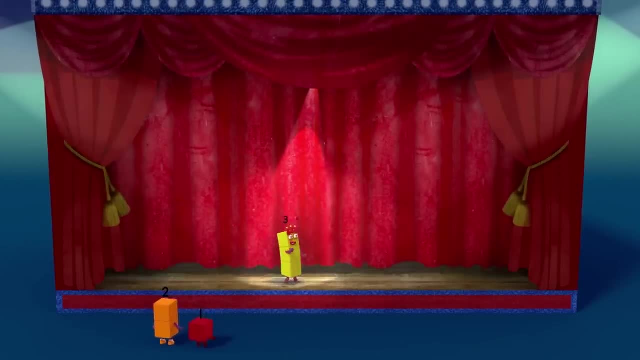 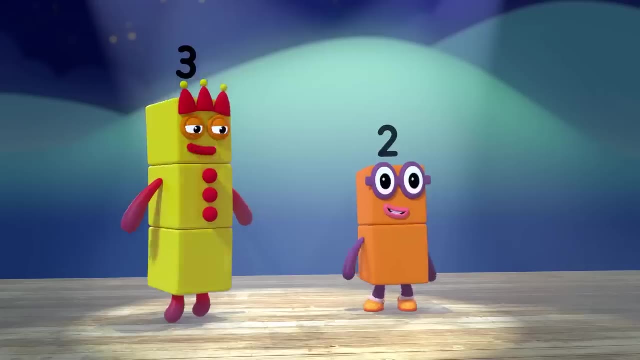 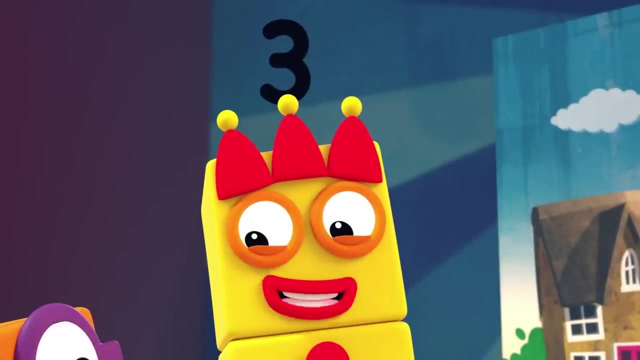 Yay, Everything's gonna be all right. Now number three is here. I'm in tic-tac-toe, I'm in ready, steady go. You're gonna have to count to three to get three in a row. You'll find me hiding everywhere. 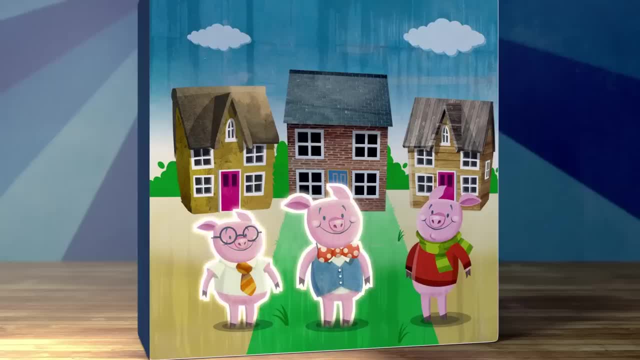 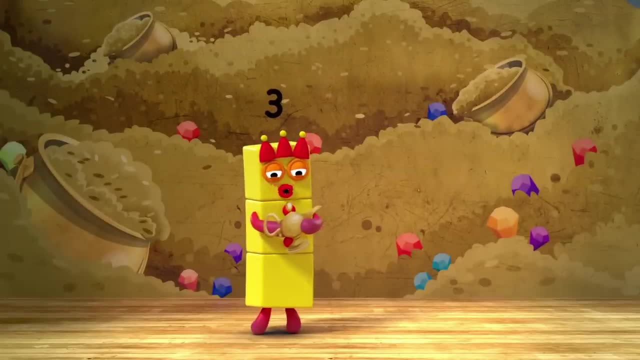 You'll look in a fairy tale or a picture book. One, two, three, Can't you see I'm in? three blind mice. Three wishes would be nice. You should try and try and try again. That's my advice. Goldilocks came across three bears. 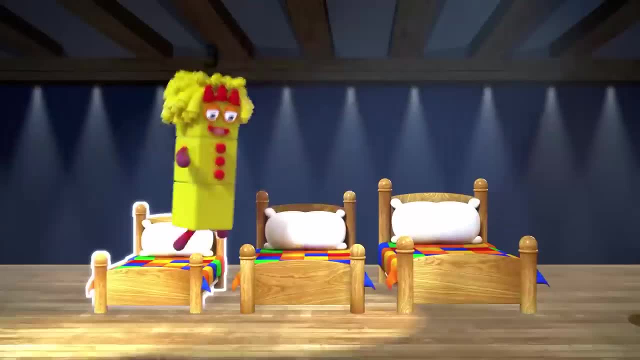 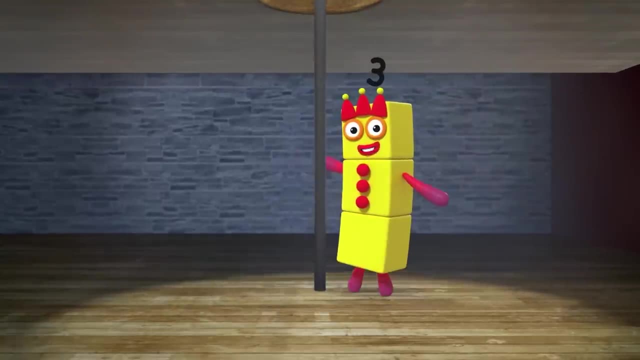 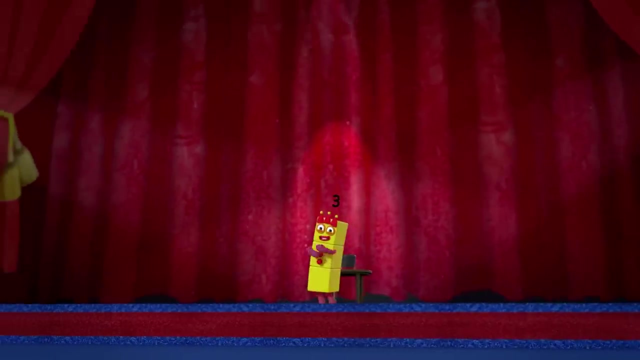 One, two, three, Three balls, three chairs, three beds upstairs. I'm here, I'm there, I'm everywhere. One, two, three, Everybody. look at me. I'm here to entertain you with this funky melody. 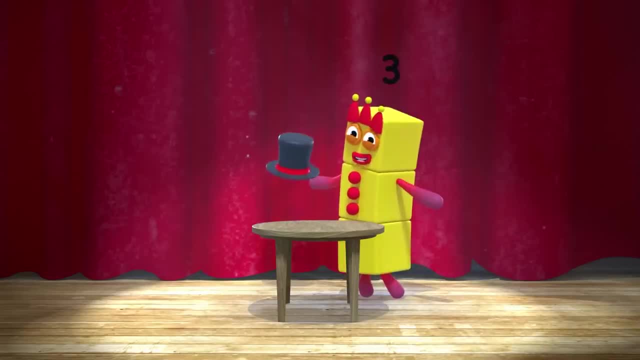 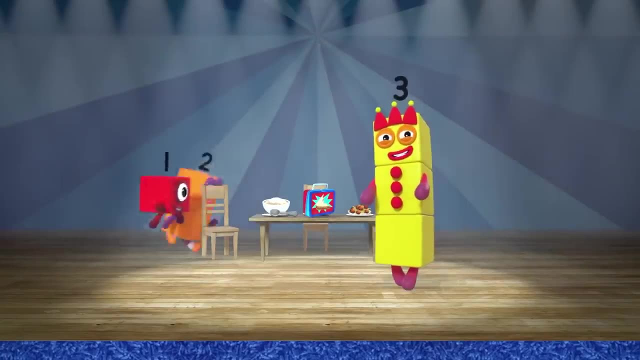 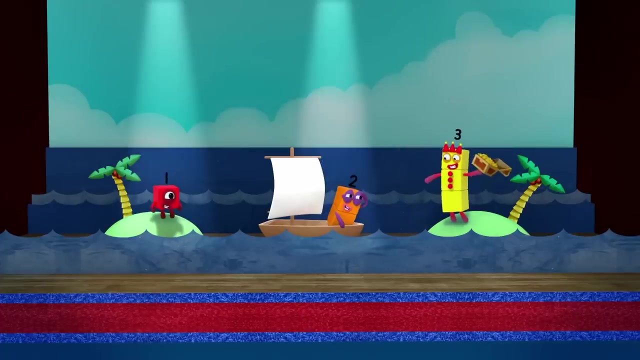 I'll pull three rabbits from a hat and make them disappear. Everything's gonna be all right. Now number three is here. Three meals a day, Three sections in a play: Beginning, middle and an end. That's the only way. Everybody better give three cheers. 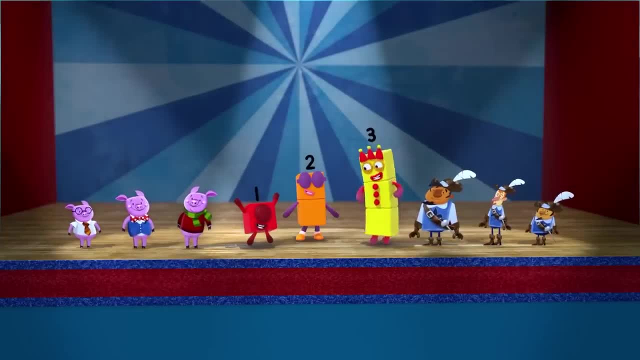 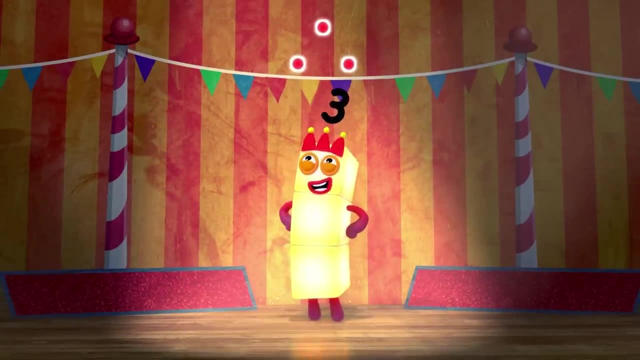 Three little pigs, Three musketeers. One, two, three, Can't you see? I can keep three balls up in the air: One, two, three. Sometimes they get stuck up there. One, two, three. The juggling balls can be your guides. 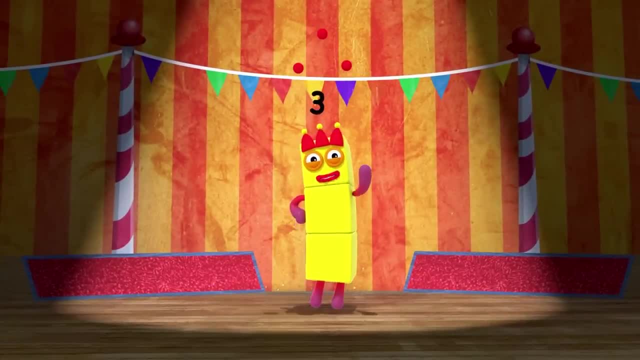 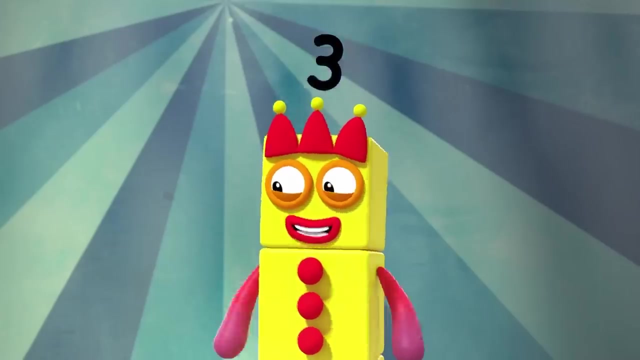 One, two, three. To make a shape that's got three sides: One, two, three. Do you know what it is? Bingo? It's a triangle: One, two, three. Everybody. look at me, I'm here to entertain you with this funky melody. 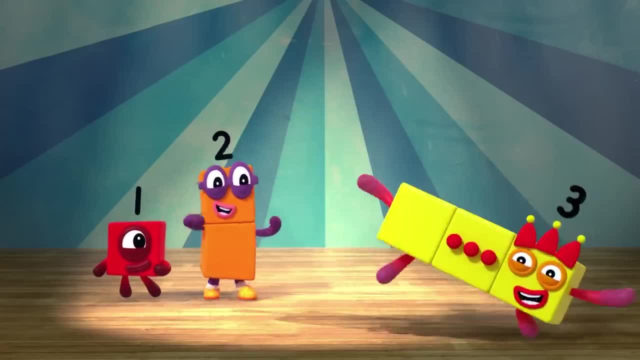 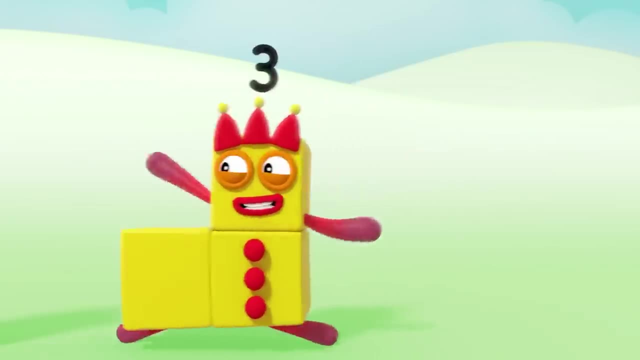 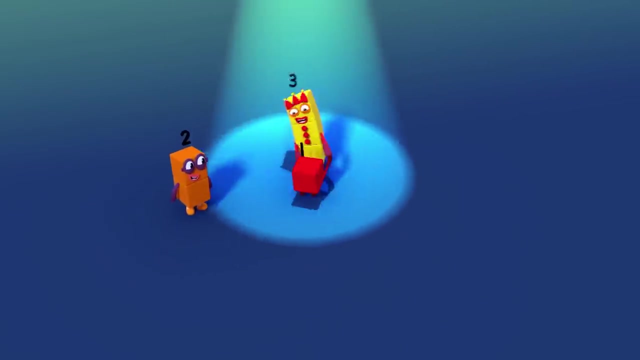 With jokes and jokes and throwing shapes. I take it off of gear. Oh no, I've broken three. Everything's gonna be all right. I'm three and I'm still here, Woo-hoo. And if you want to dance with me, 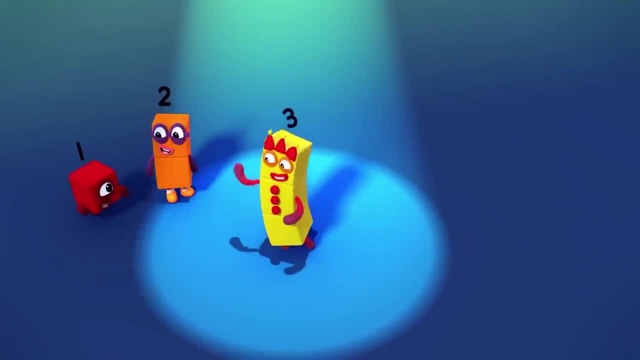 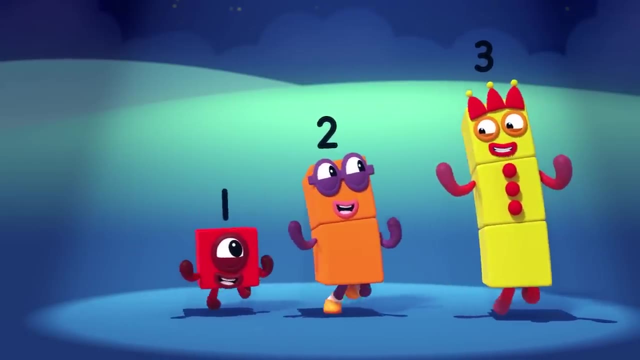 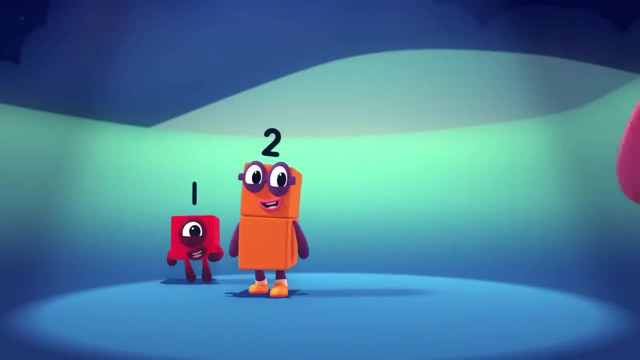 One, two, three, Everybody. look at me. I'm here to entertain you with this funky melody. I'll juggle three balls in the air and everyone will cheer: Yay, Everything's gonna be all right. Now number three is here. 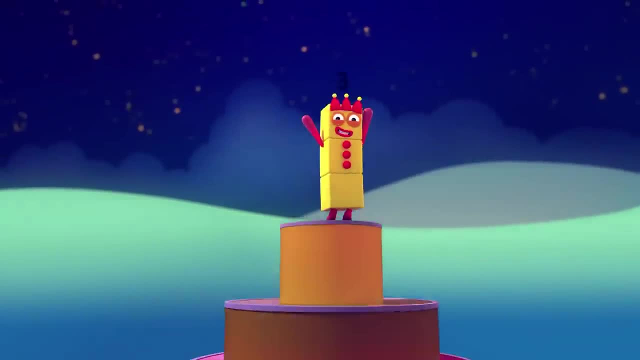 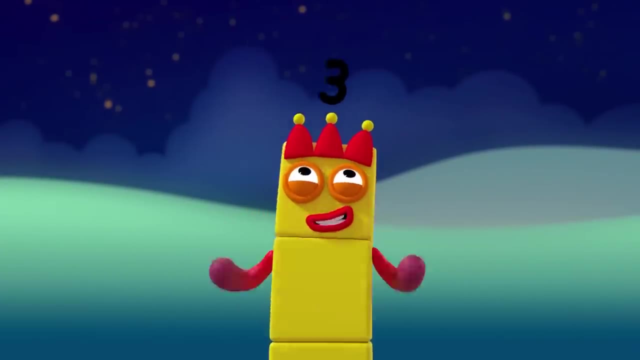 Everything's gonna be all right Now. number three is here. Well, now it's time to say goodbye, Bye, I'm You, Can You, You, You, You, You, You. Everything's gonna be all right now. 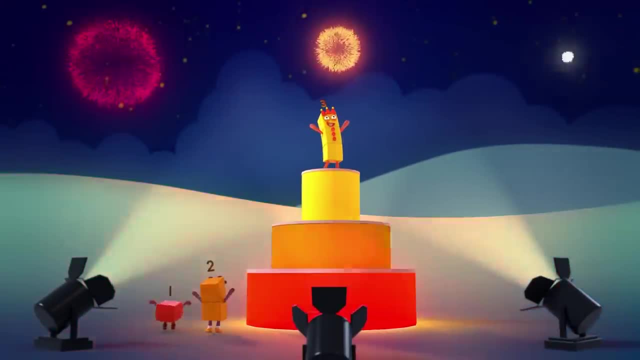 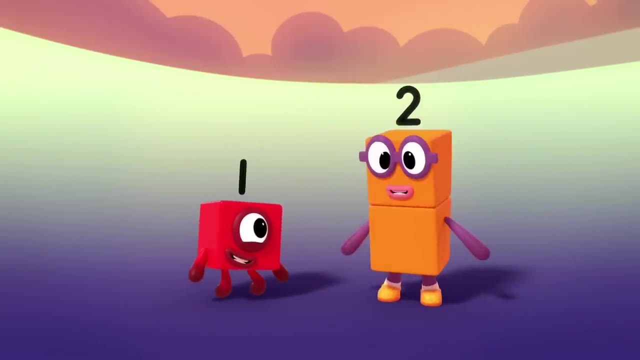 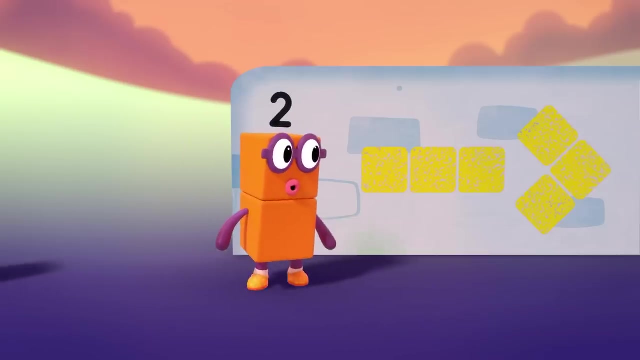 Number three is here. One two And again One two. Your turn One. I can't do it Right. What was that That way? Come on, Wait, Looks familiar. It's pointing to the sounds Quick. 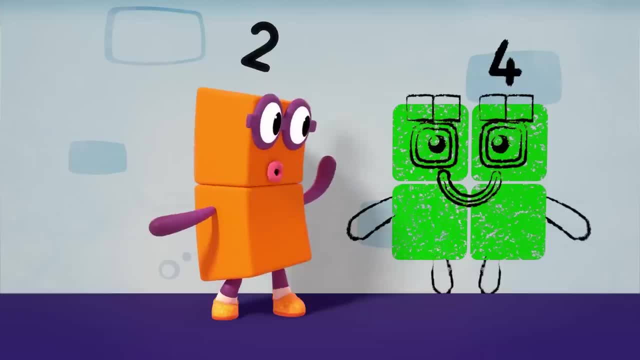 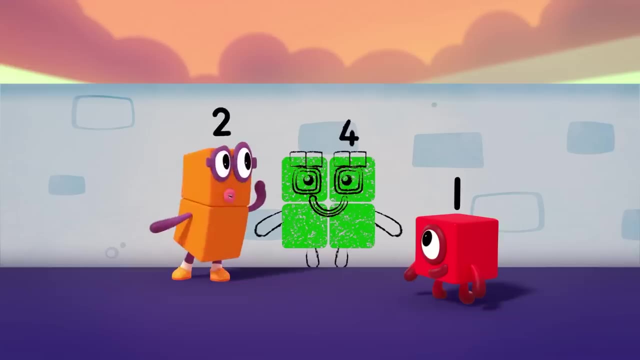 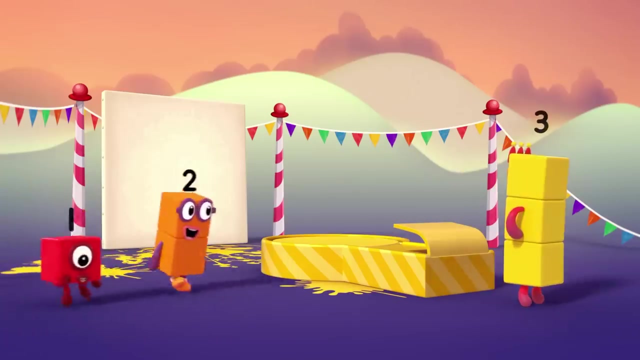 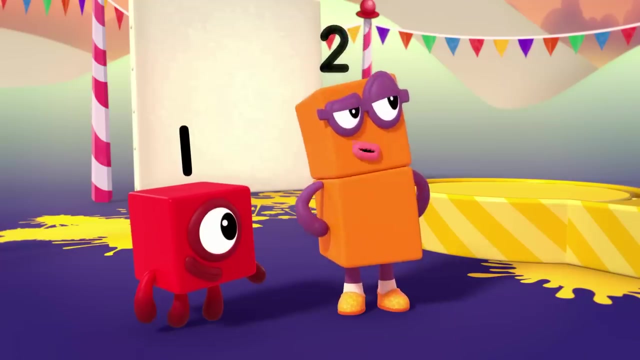 Hey, it's four, Four, Four. Are we playing musical statues? A painting, A painting of four. I knew that, But what's that? Welcome, welcome, welcome to my new stampoline park. Don't you mean trampoline? 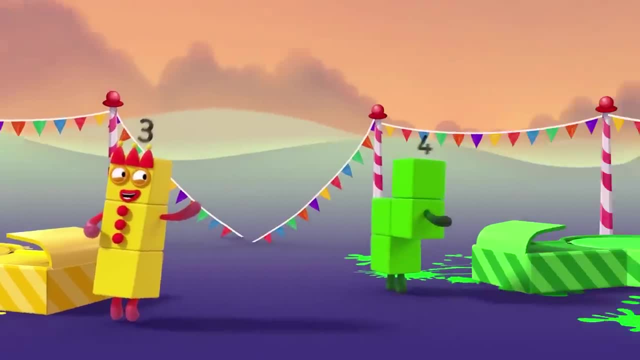 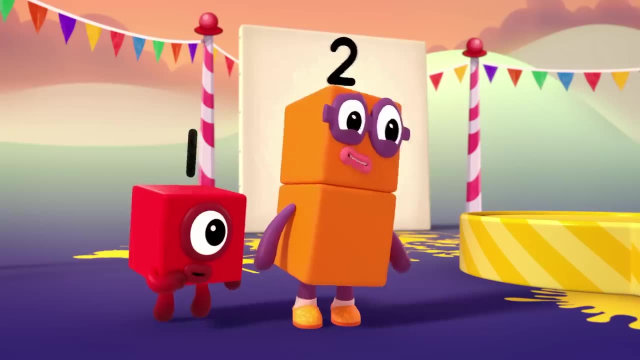 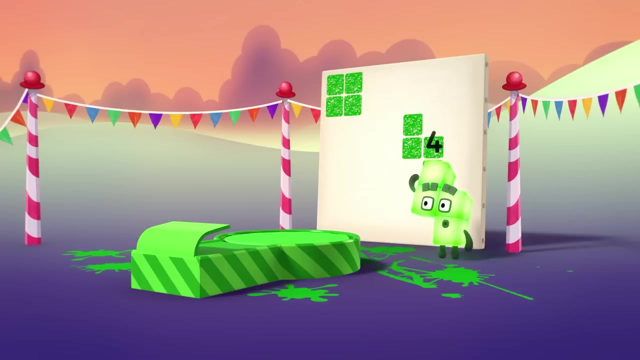 No, no, no, Look Whee, Ooh, that was fun. Four, Is that you? Of course. it is One, two, three, four, Four blocks, See Whee. Whatever way round I go, 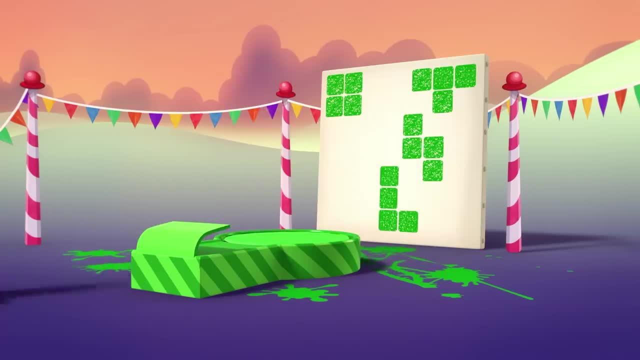 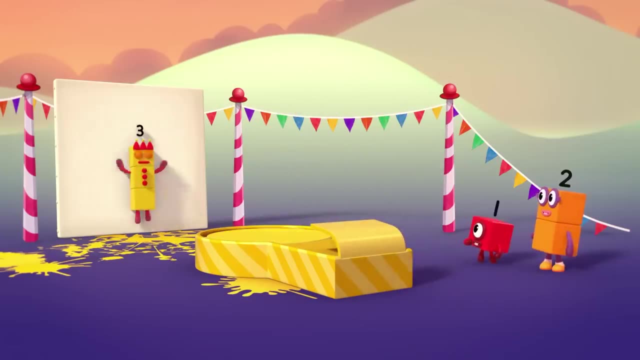 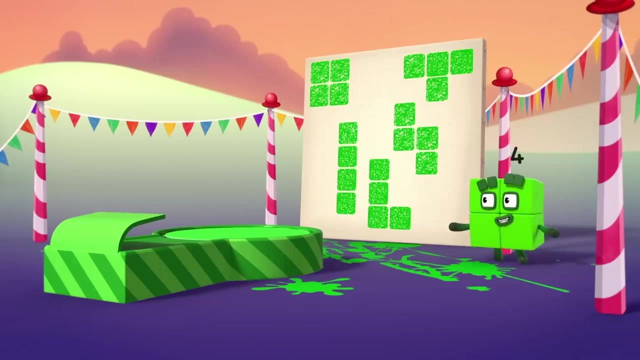 Whee, I'm still four Whee. Look at me, Whee, I'm still three. Whee, Whee, Whee, Whee, And you Whee, Ah, Clump Wow, Sarah, worried, come on. 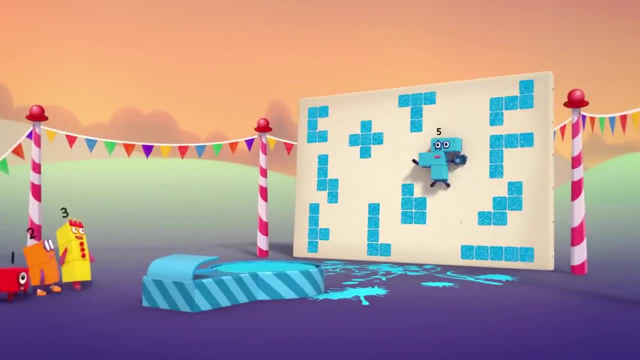 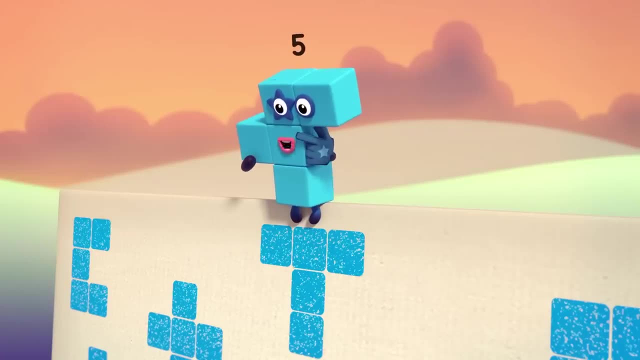 Whee, Let's go over and talk to the drawings. No, Oh, оп, I'm falling. Comment one, two, three, One, two, three, Woo Woo. Who is that? Woah, That's Eve. 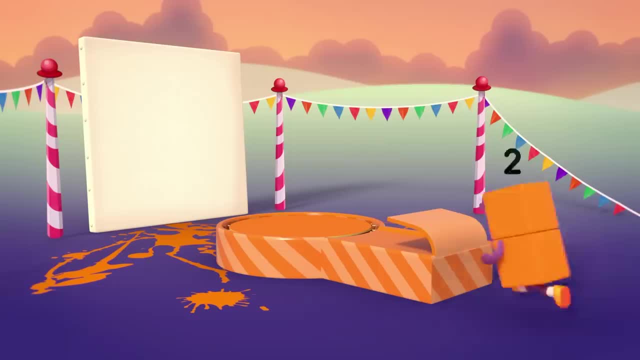 That's Kate Flurry. I'm already hungry. There's nothing more to do on this one, Not for these two hot dogs. What are you? Chat a little bit. Ah, I'm sick. Let's see if my cake has anything. 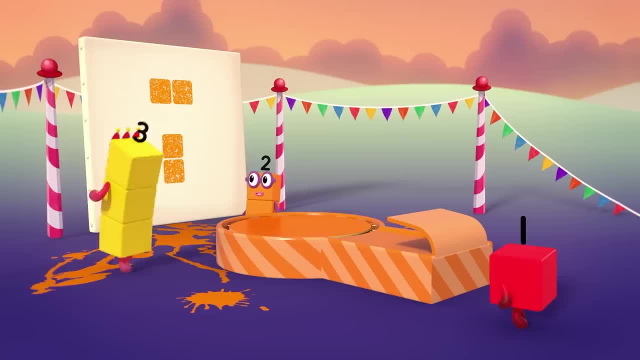 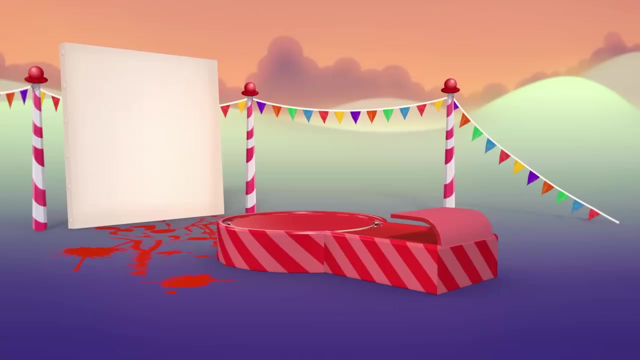 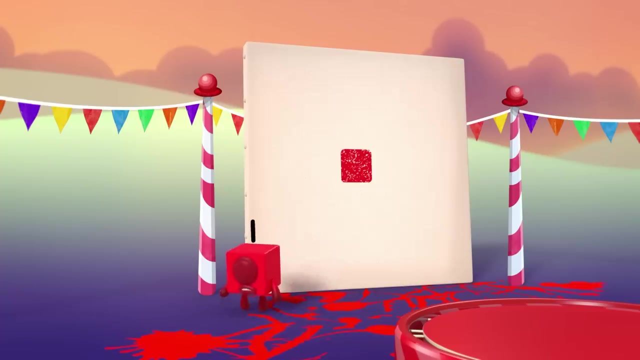 Umph, Hold on. Look Bad too. Of course, they're not really different shapes, are they? It's the same shape, one going up and one going across. Oh, it's still better than me, Look. That's all. 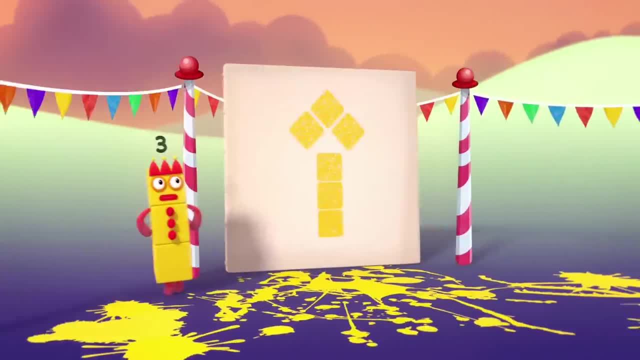 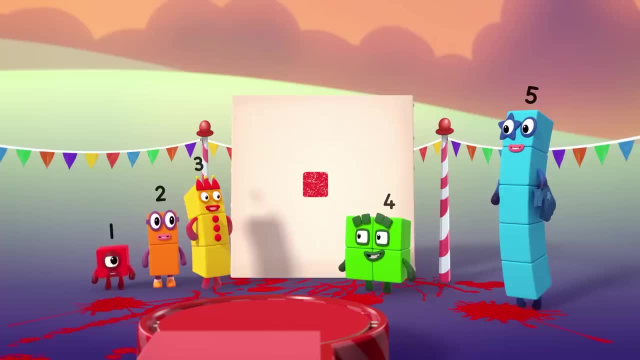 One shape, Not very exciting compared to all of you. Now, now, now You're forgetting something. One, two, three, Boo Hey. One plus one plus one plus one equals four. Every big shape is made up of lots of little ones. 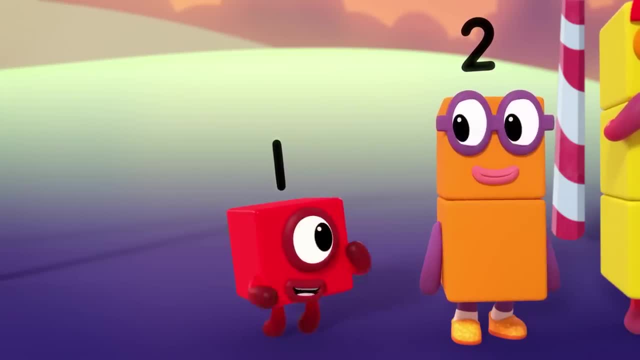 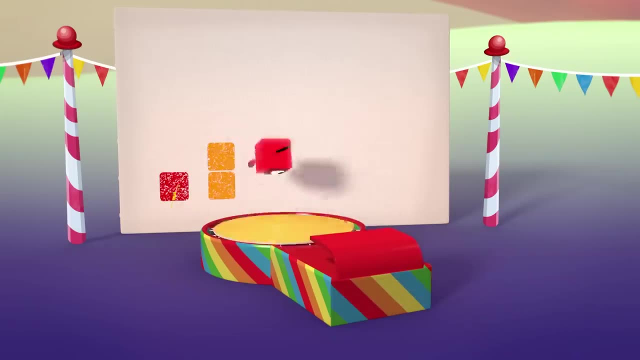 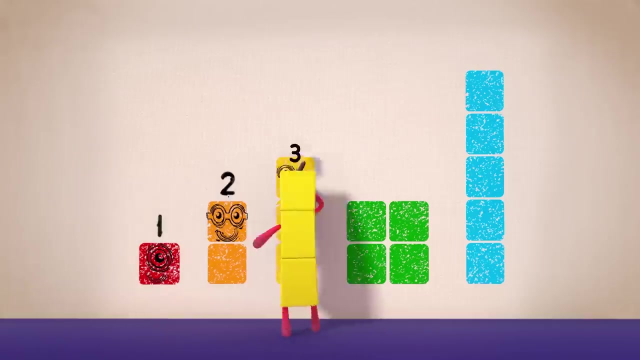 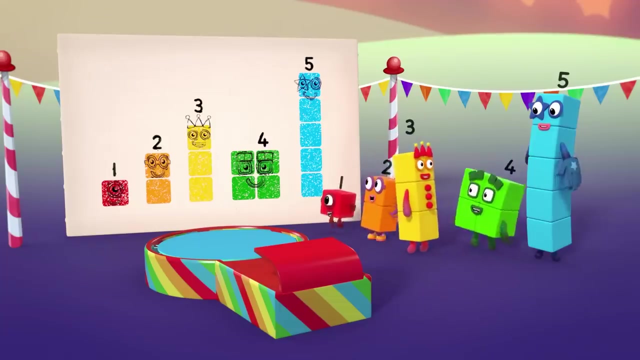 So lots of little ones can make every big shape. Look what I can do. Hooray, You made all of us All right. Well done, And just in time for the grand finale, What better way to celebrate opening my new park than with fireworks? 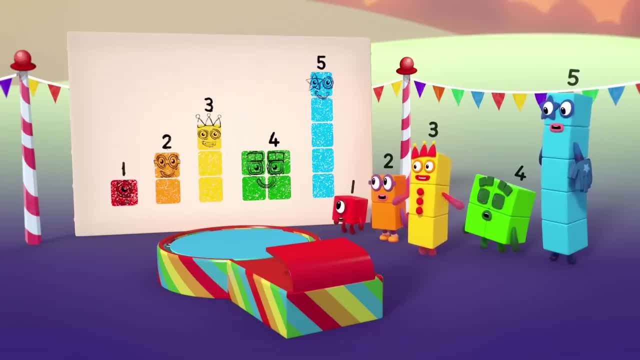 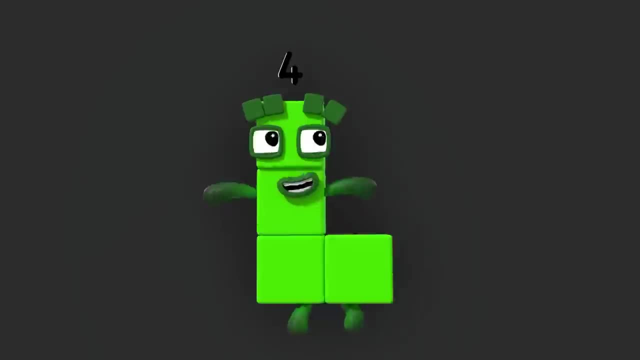 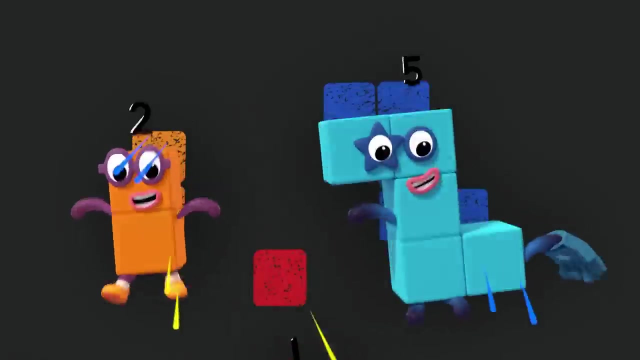 Ooh, May I present the Sky At Night? Woo Yay, Woo-hoo Yeah, Woo-hoo, Woo-hoo Yay. Yes, Woo-hoo Hooray, Woo-hoo, Woo-hoo. 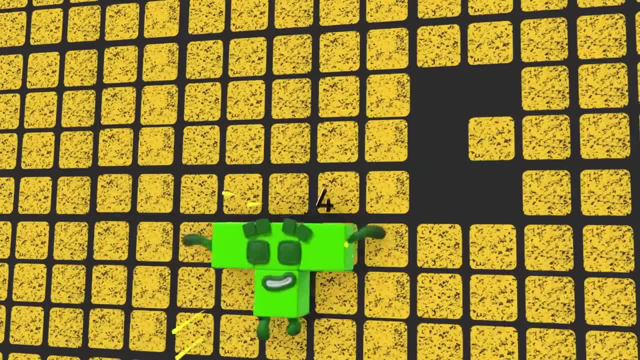 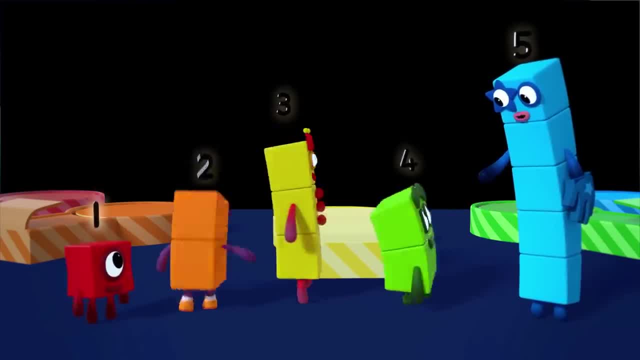 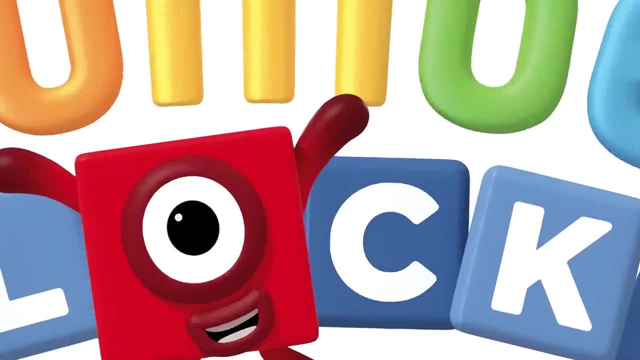 Yes, Hooray, Woo-hoo, Yeah, Woo-hoo, Woo-hoo. You see one, When we all work together, the sky's the limit, Woo-hoo, Woo-hoo. Let me tell you a story. 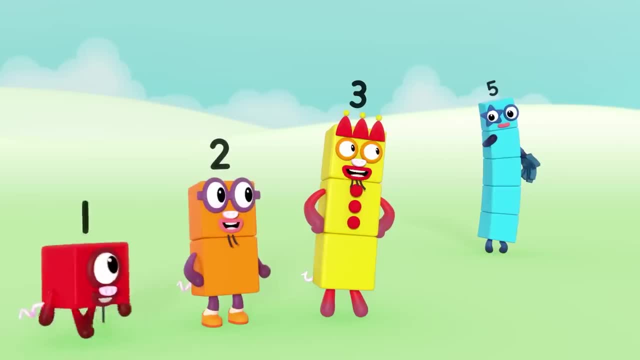 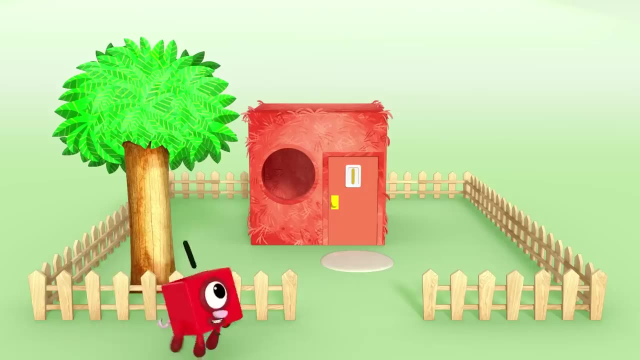 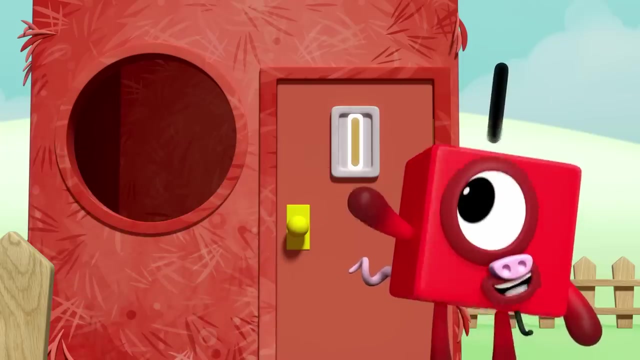 Once upon a time there were three little pigs. The first little pig had a house with one room. Look, It has one one window and one one tree in the garden, And there's a number one on the door, Woo-hoo. 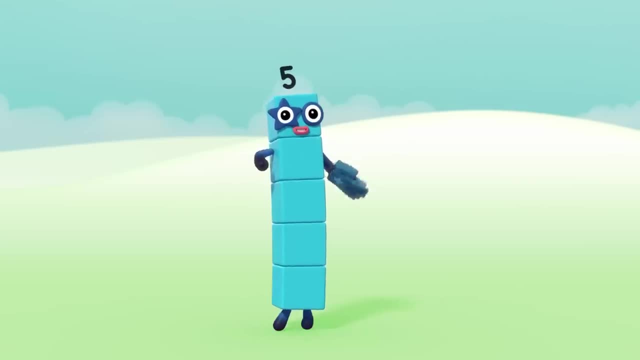 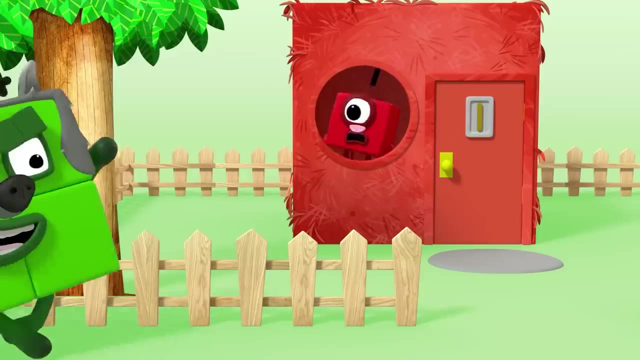 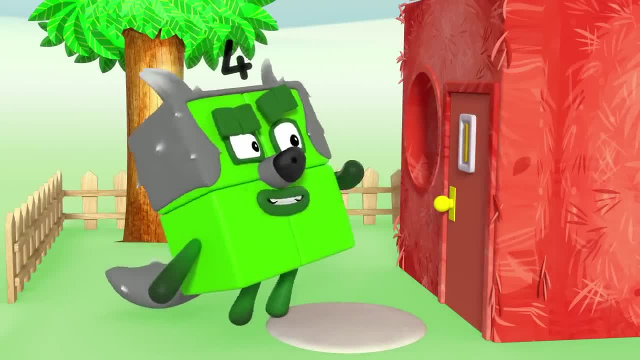 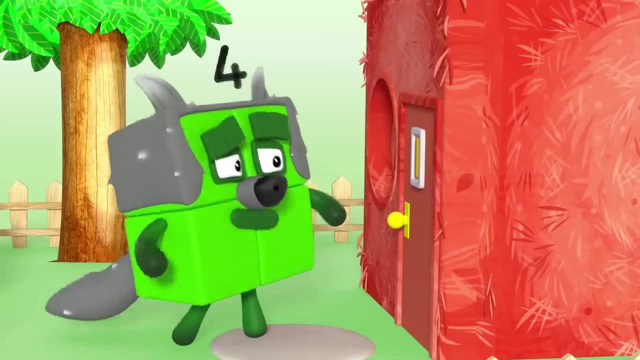 Little pig, Little pig, Let me in. Let me in Woo-hoo, Not by the hair on my chin. Then I'll hoof And I'll poof And I'll blow your house in Woo-hoo. Shame. 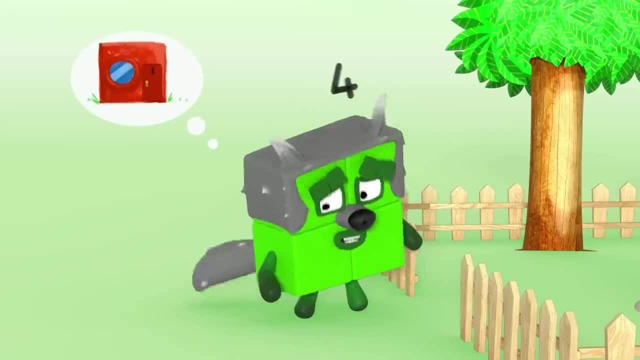 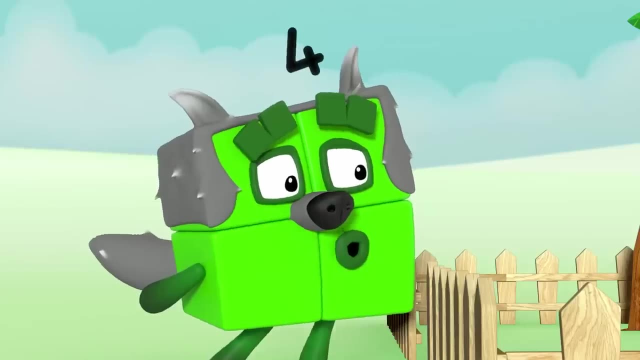 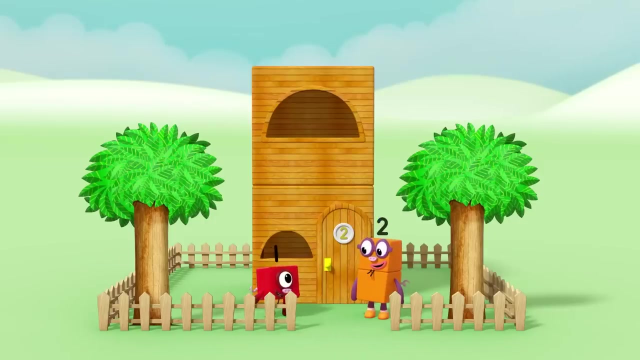 That's so square. Yeah, Woo-hoo, Oh, my Woo-hoo, Woo-hoo. Luckily, the second little pig had a house with two rooms, Room for two, me and you. It has one two, two windows And one two two trees in the garden. 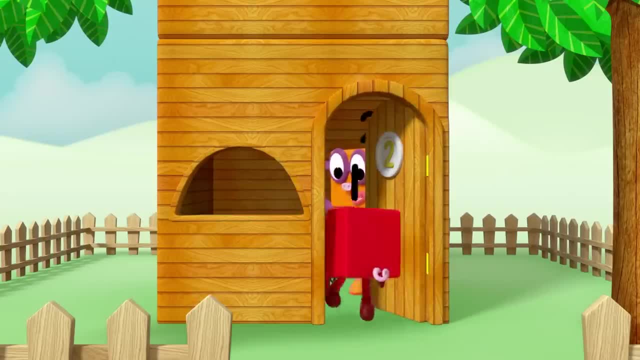 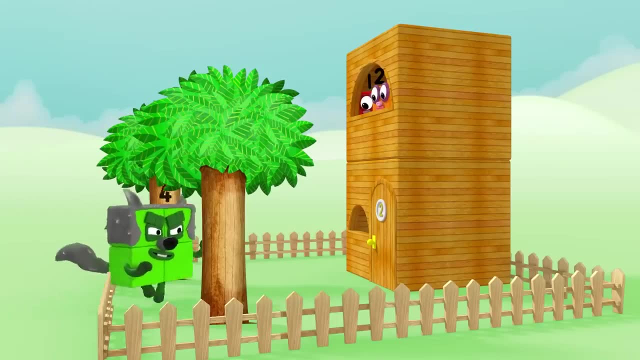 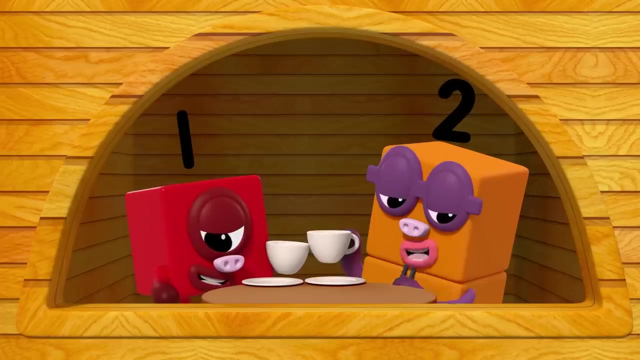 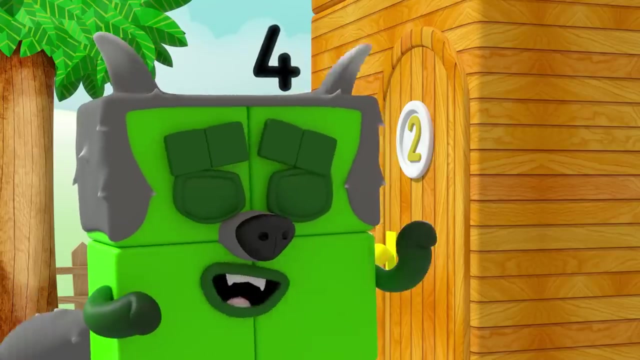 And there's a number two on the door: Tea for two and two for tea. Little pig, little pig, Let me in. let me in, Not by the two hairs on my chinny chin. Then I'll huff and I'll puff And I'll blow your house in. 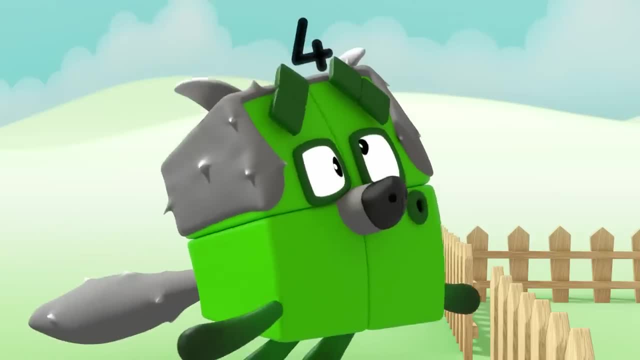 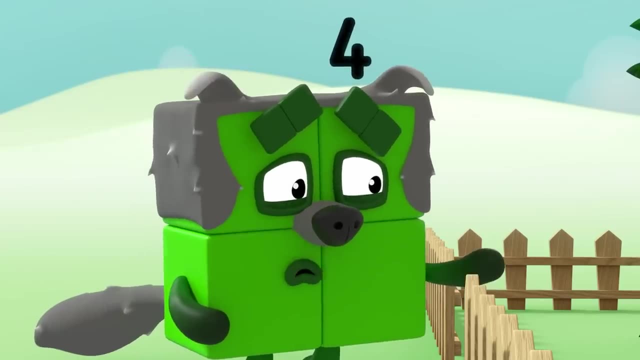 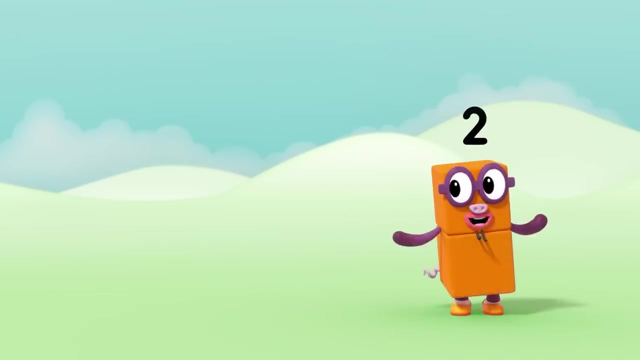 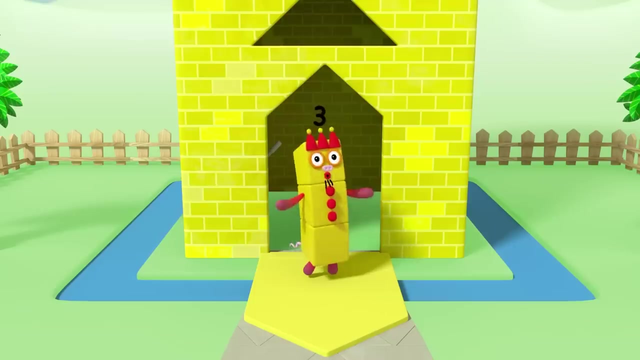 Oh, no, Oops, sorry, two. One plus one equals two. No worries, it's only pretend, But where will we live now? Luckily, the third little pig- Oh, that's me Busy, busy, busy- Had a house with three rooms. 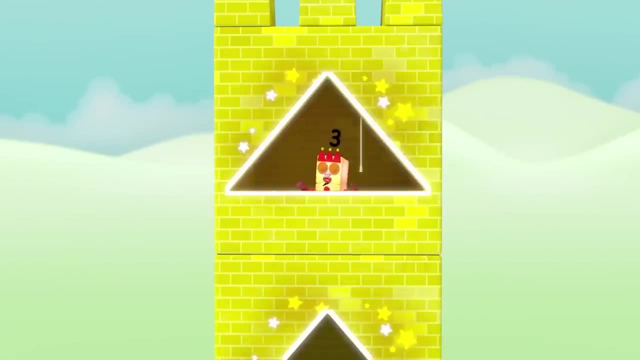 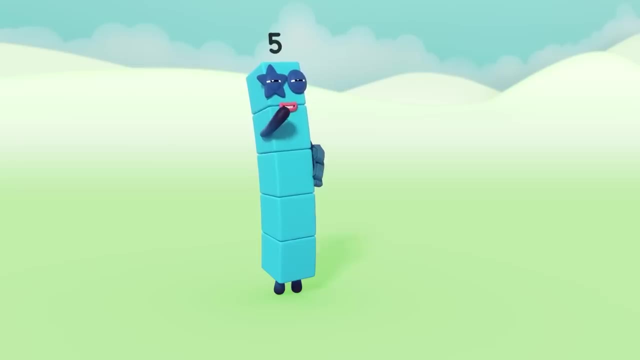 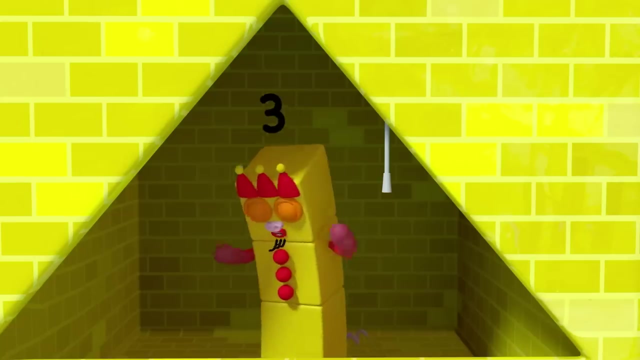 And one, two, three, three windows, And one, two, three, three turrets, And one, two, three, three flags. And yes, yes, thank you, three. Room for a couple more Sure, Two's company and three's a party. 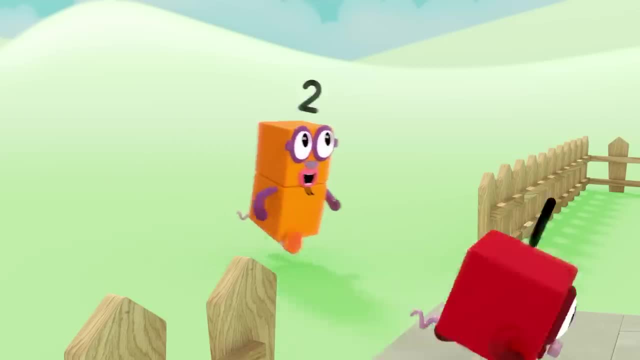 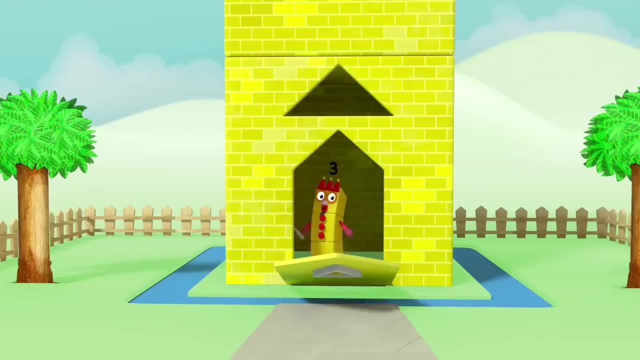 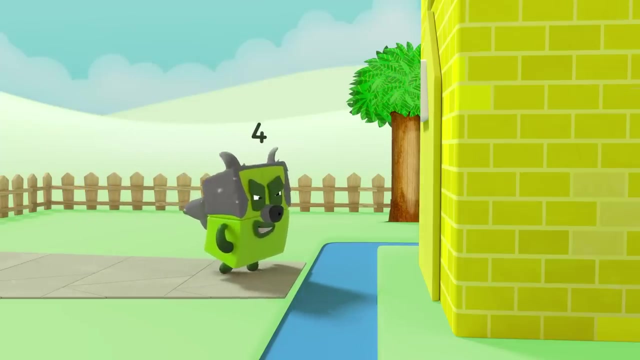 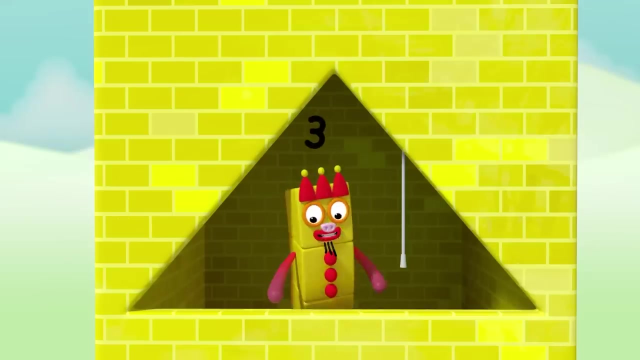 Keeping that big bad square out Is as easy as one, two, three Little pig, Little pig, Little pig, Let me in. let me in, Not by the three hairs on my chinny chin chin, Then I'll huff and I'll puff. 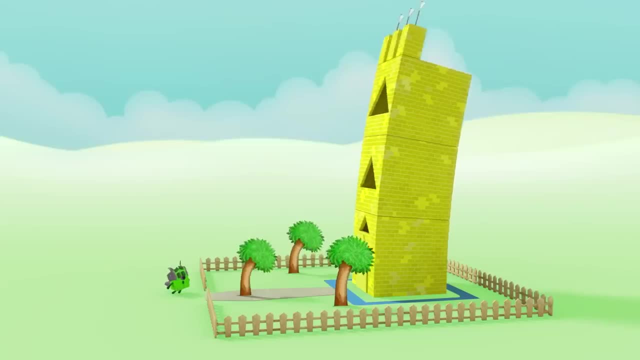 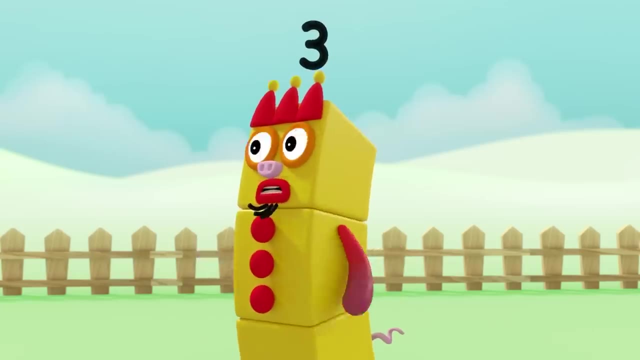 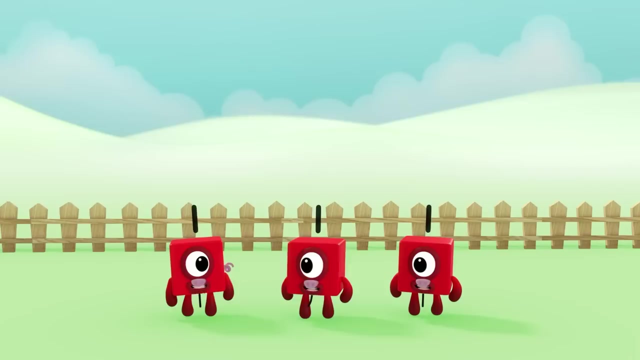 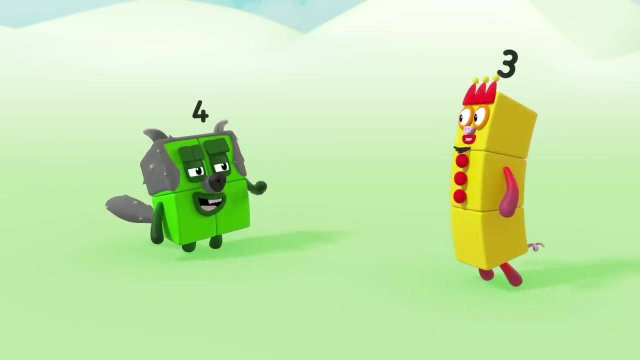 And I'll blow your house in. Oh What, But how? Just a little huff, Oh, Oh, Hey, Hey, Ah, This is not watching him. Well, that's the best I can do. One plus one Plus one. 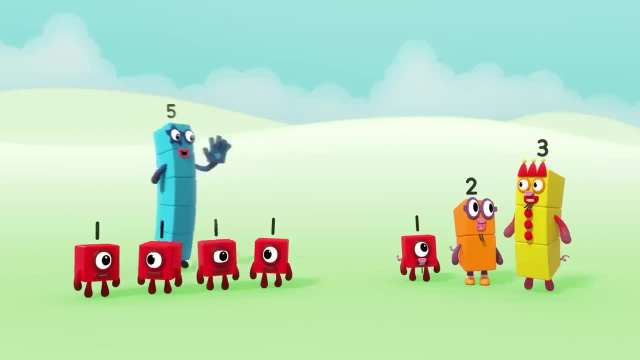 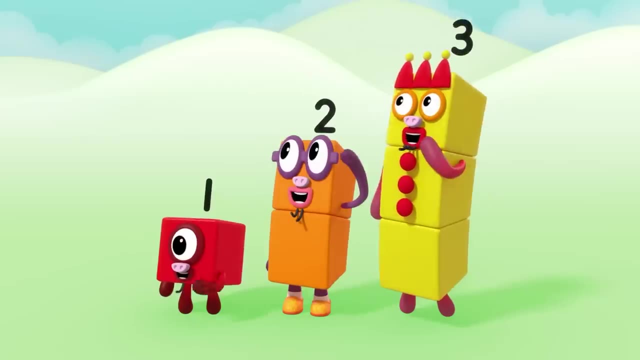 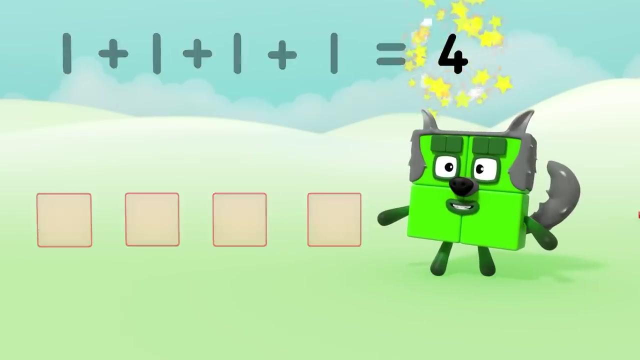 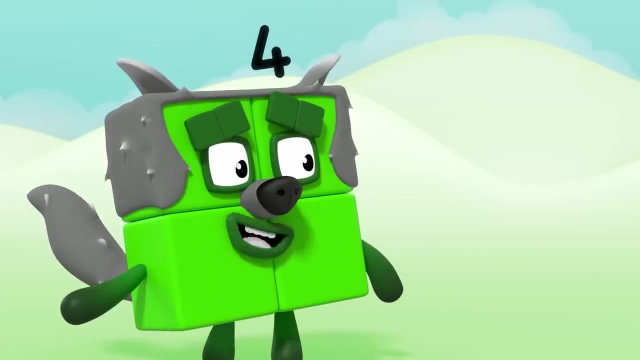 Plus one Equals Three. See how you like it. Stop. This isn't how the story goes. The third house doesn't get blown down. Where will the three little pigs live now? There's always my house. It's got four rooms. 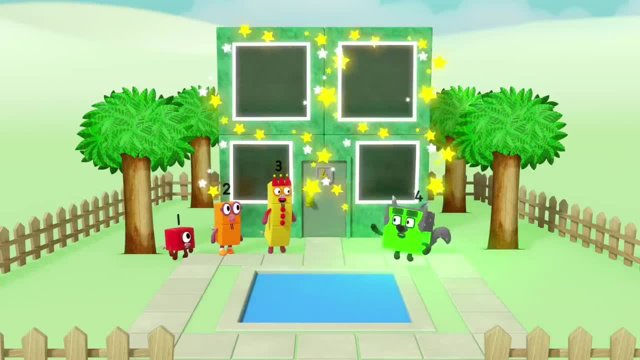 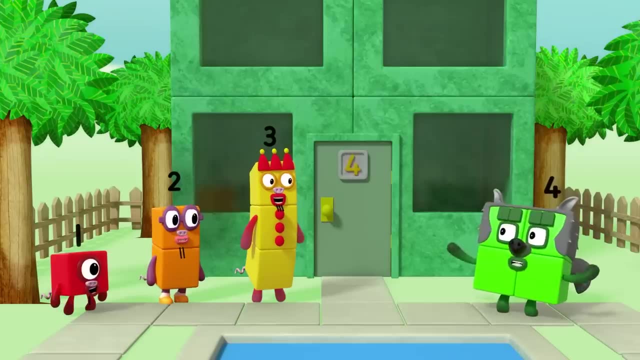 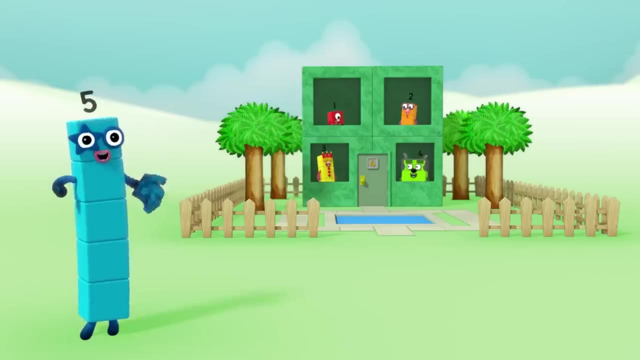 With one, two, three, four, Four windows, And one, two, three, four, Four trees And a number four on the door. One, two, three, four, That deserves a big hand. Once upon a time there were three little pigs and a big bad square. 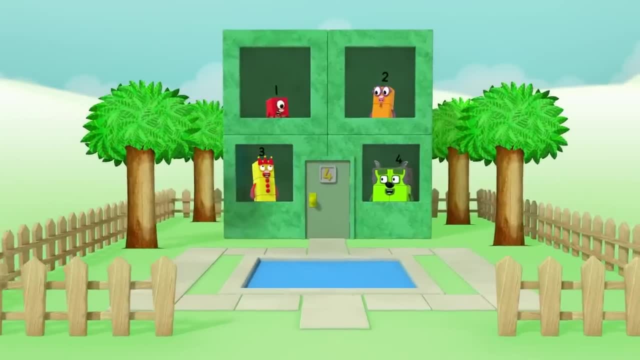 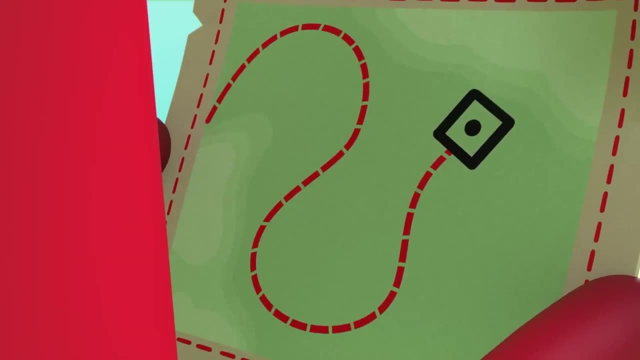 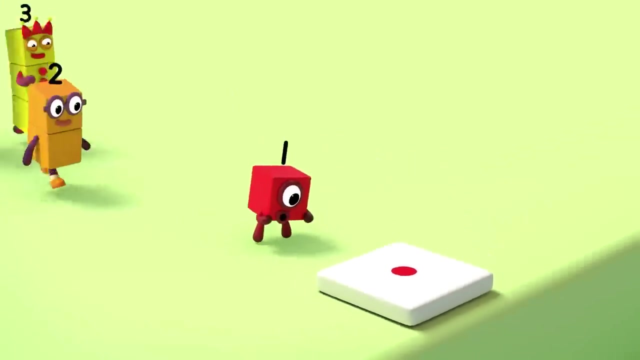 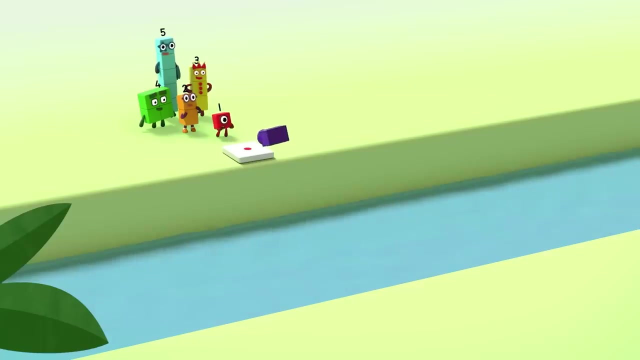 And they all lived happily ever after The end. Yay, If the map is right, the pattern palace should be right here. Oh, Welcome to the pattern palace where you can, Where you can play all day, But first you must cross the pattern paths. 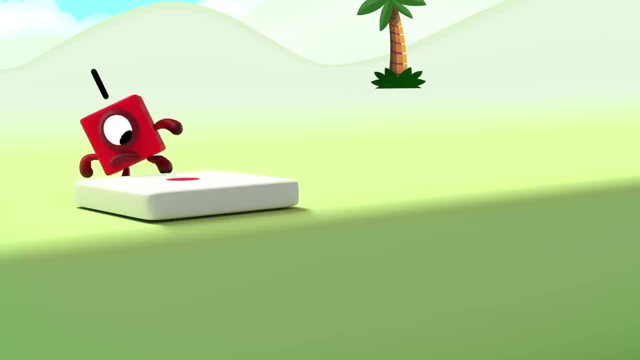 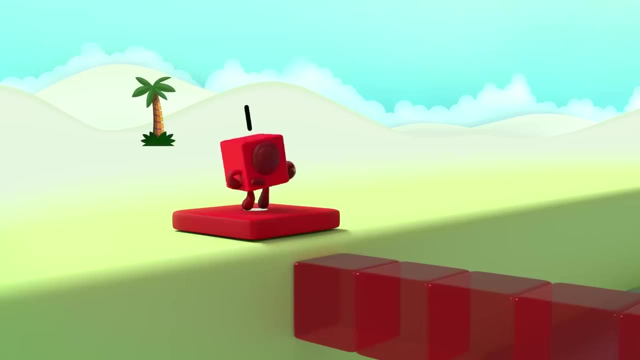 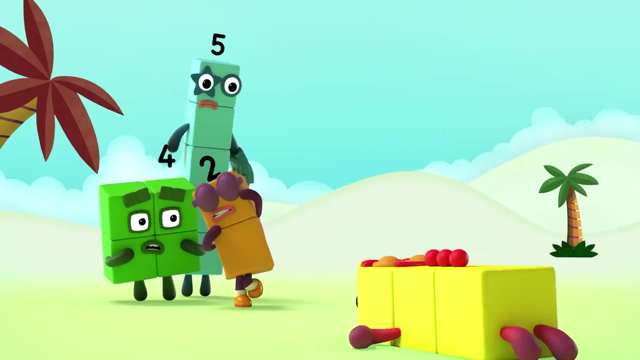 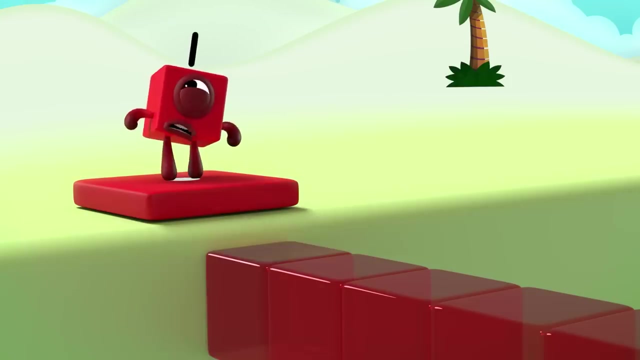 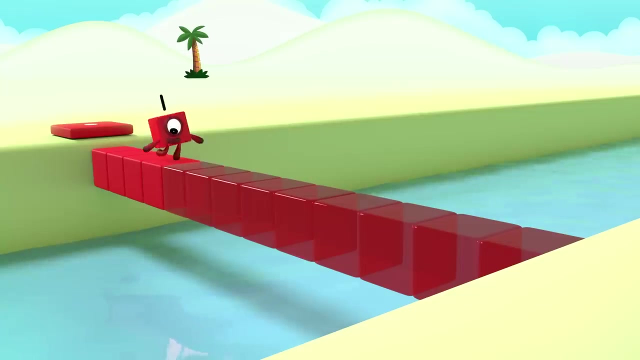 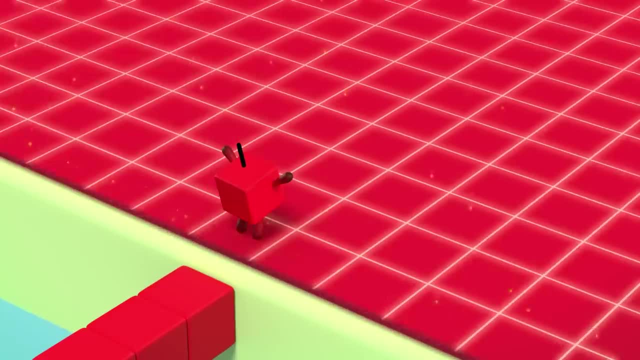 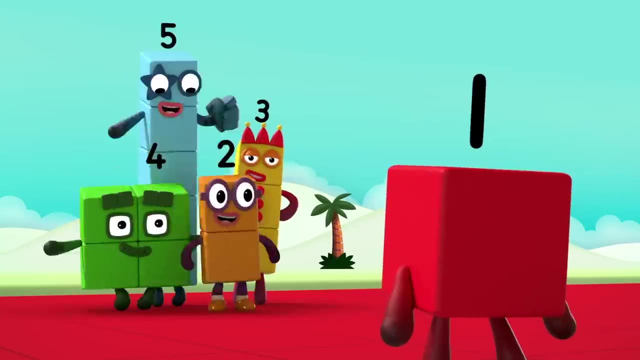 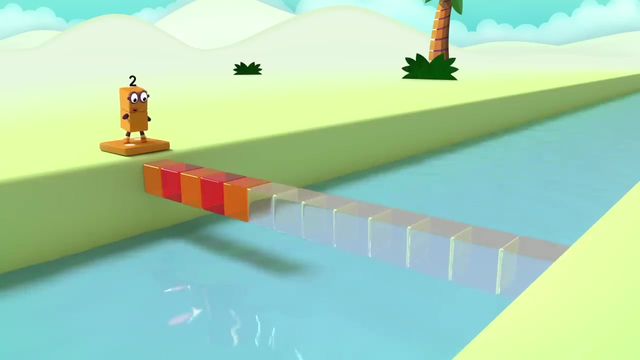 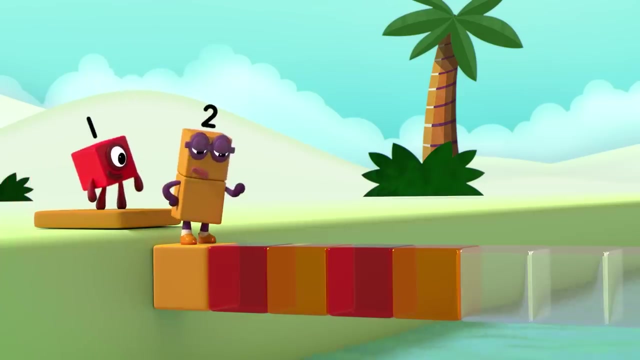 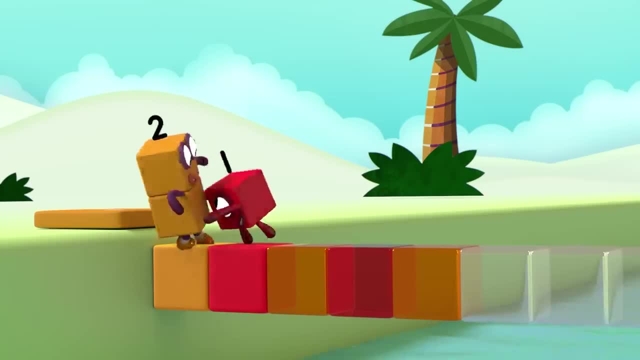 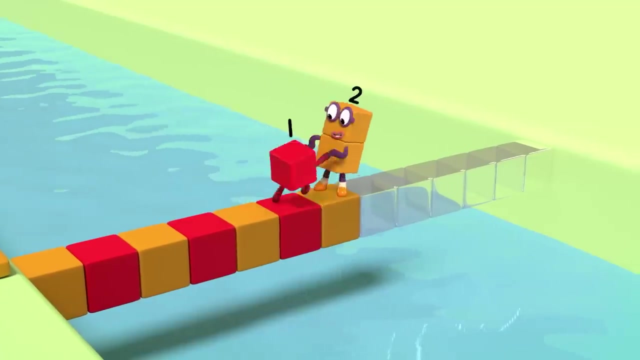 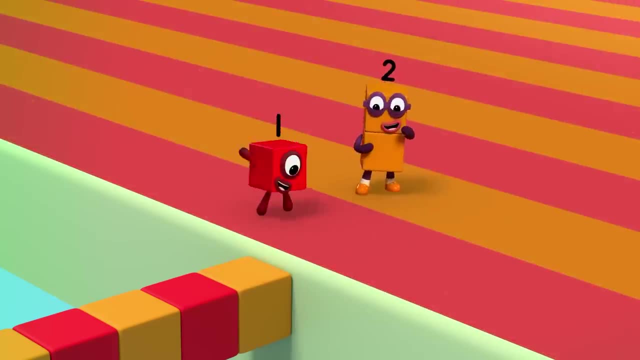 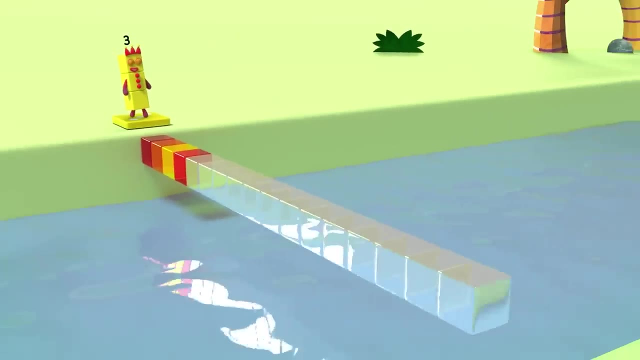 Woo-hoo, One One, One vault. Yeah, That's good. Good, Oh Okay, I got it At last. Me, me, me Yellow. No, it's not Red Orange, Oh yellow. 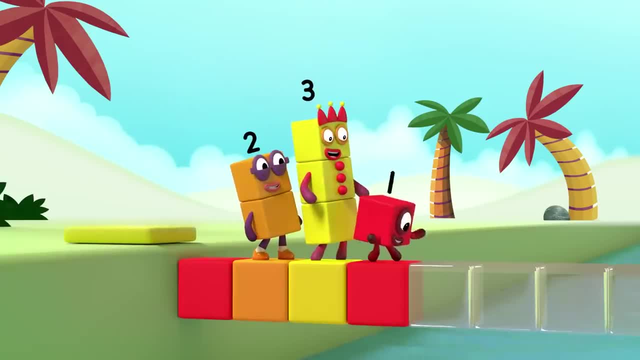 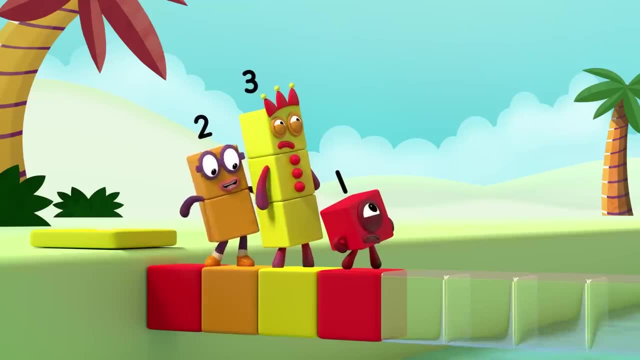 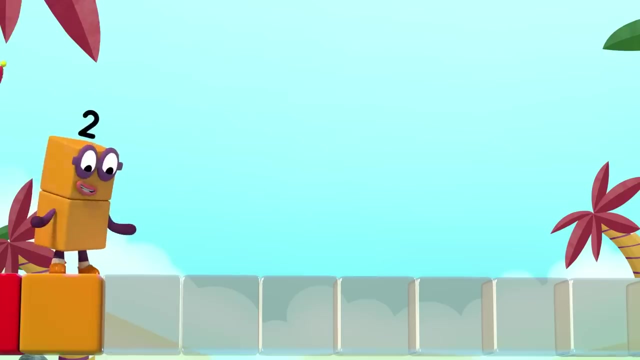 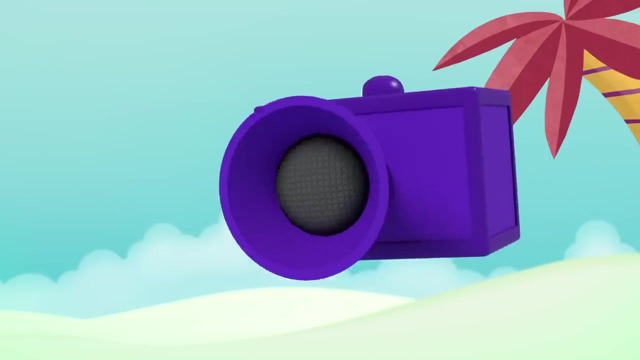 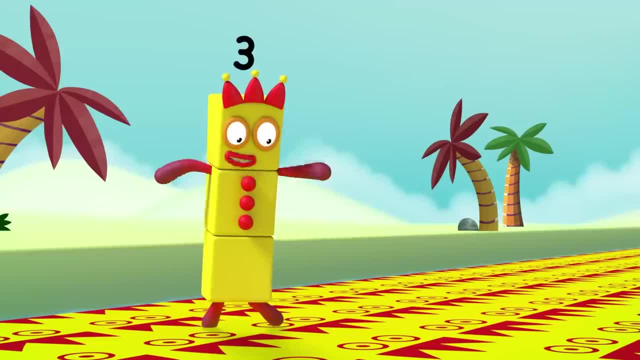 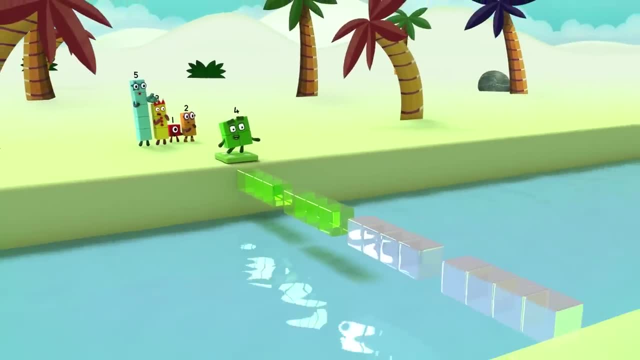 Pattern unlocked. Ooh, Now that's what I call a pattern. Oh, I know exactly what to do here. so if you Easy, easy, easy, Green, green, green, green, jump over the gap, Green green, green, green, jump over the gap. 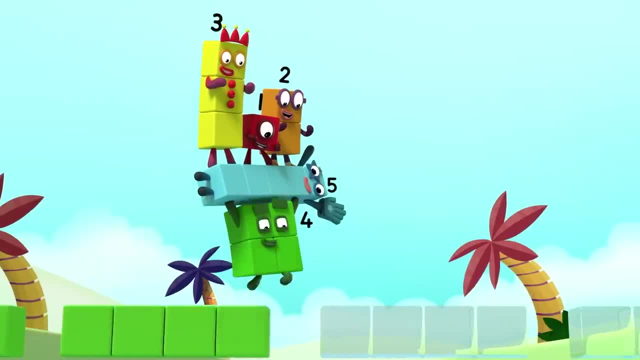 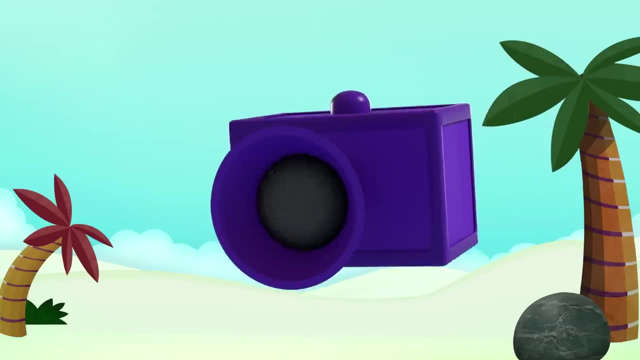 Ooh, Green, green, green, green. jump over the gap. Tell me the pattern. The pattern is It goes: four greens, Then a gap And repeat: Pattern unlocked: Oh, Squares, Squares, Squares. 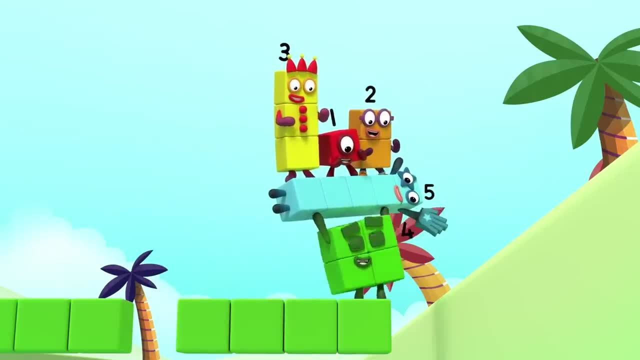 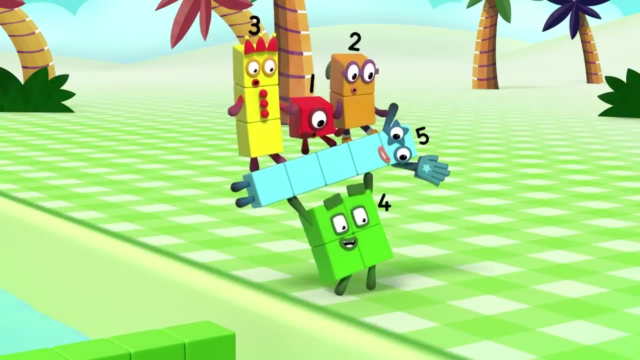 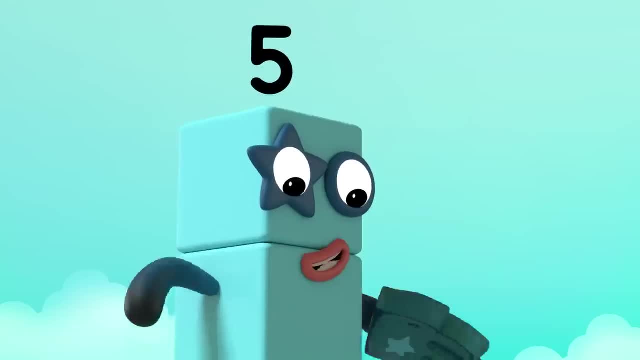 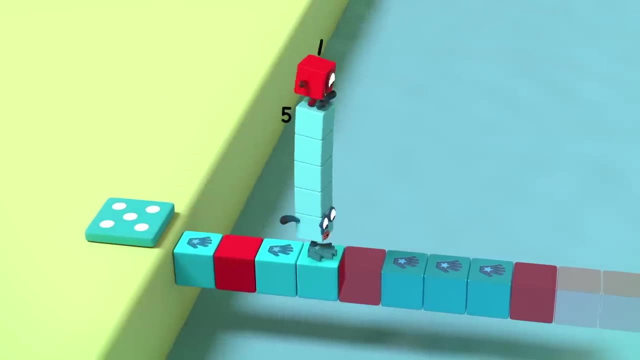 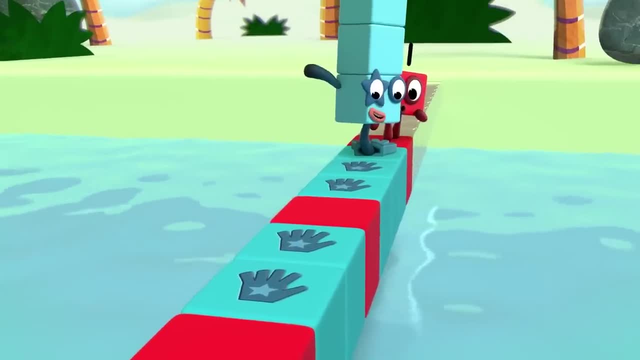 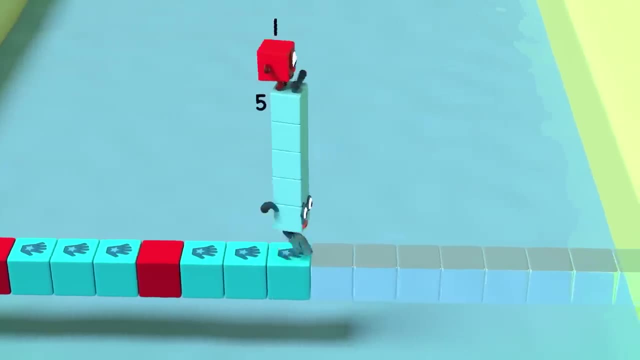 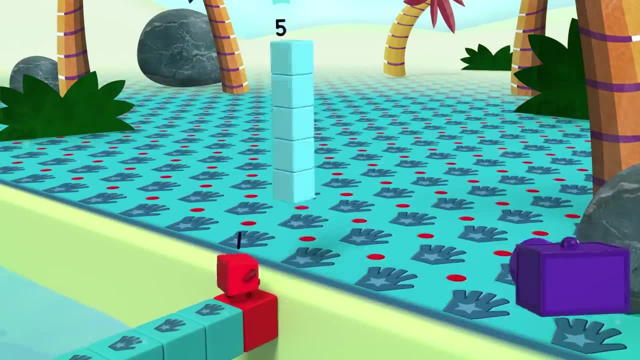 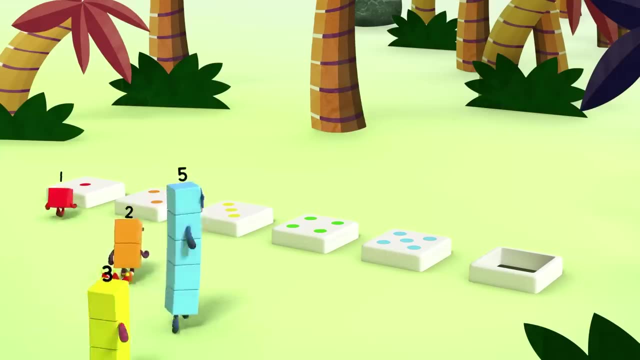 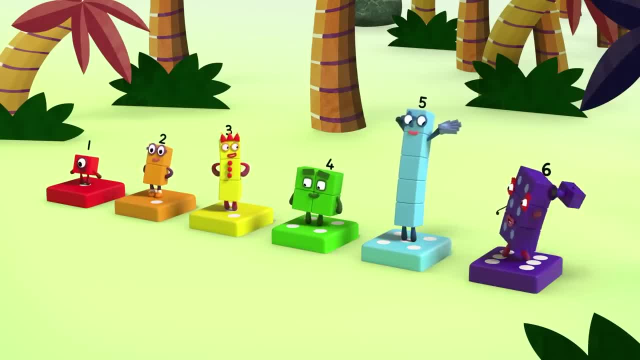 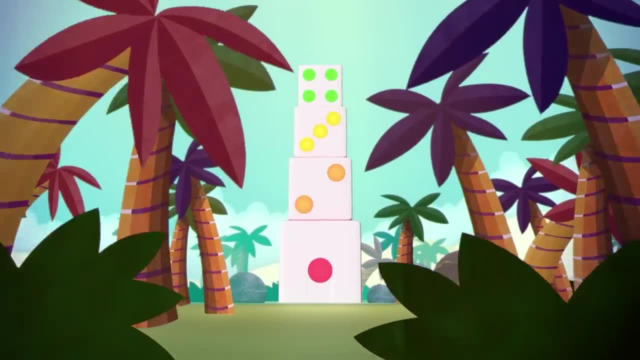 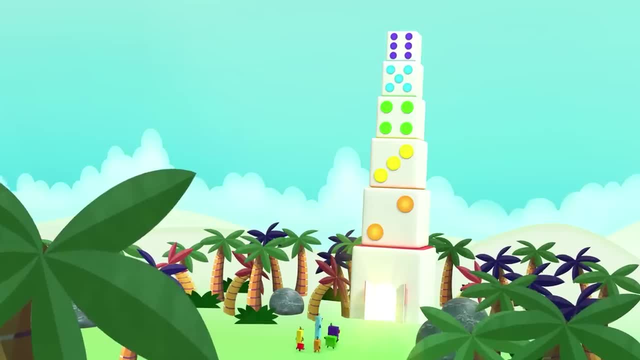 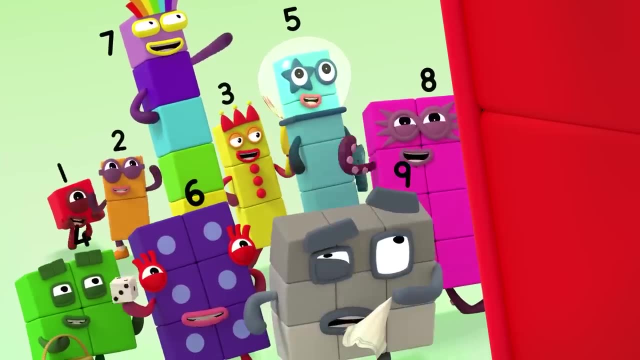 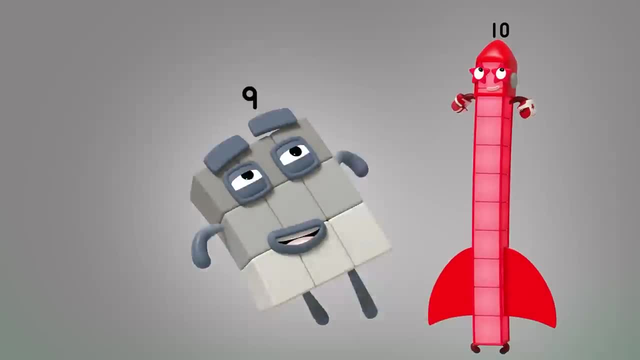 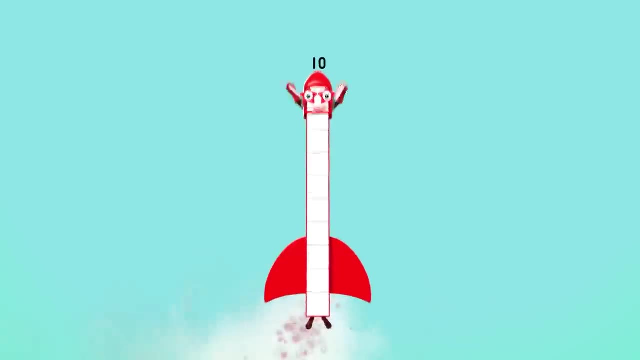 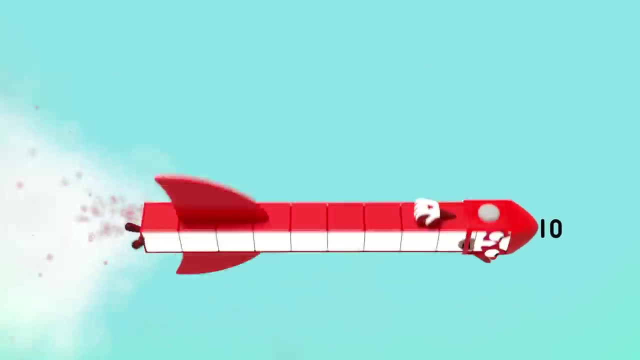 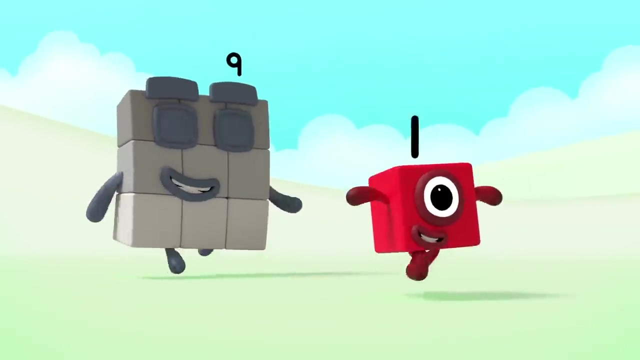 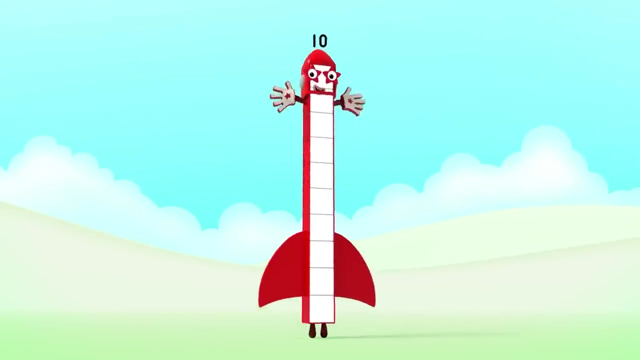 I'm ten, ten, ten and I'm flying through the sky. I'm ten, ten, ten. you can break me up any way you like. I can be nine plus one, going for a run, trying not to sneeze and having lots of fun. and then I'm ten, ten, ten again. I can be eight. 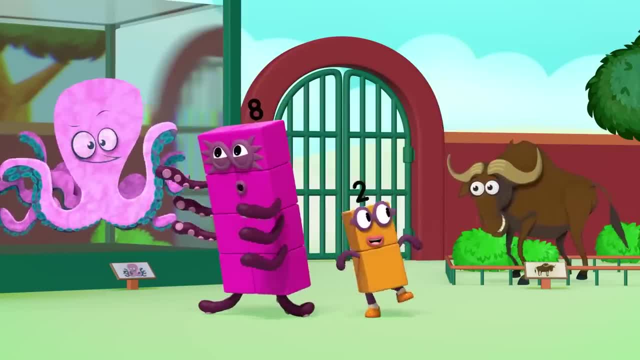 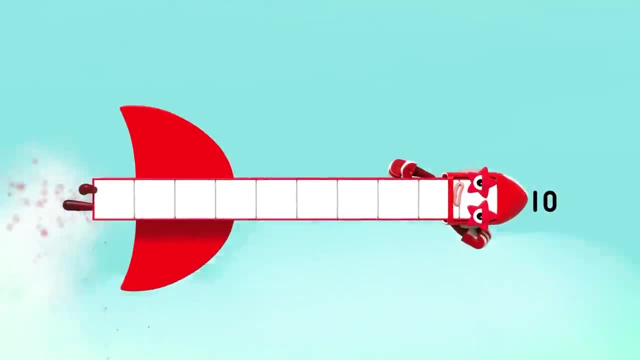 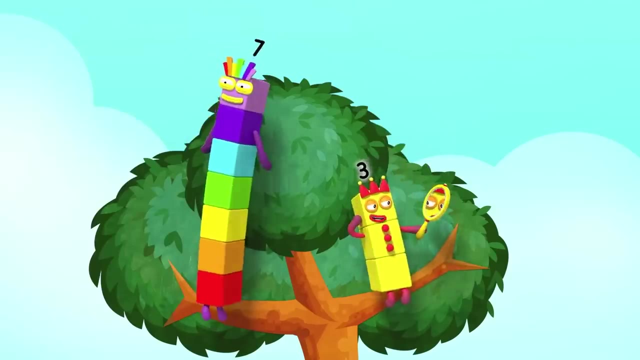 plus two, visiting the zoo, talking to the octopus and dancing with a canoe. and then I'm ten, ten, ten again, I can be seven plus three, sitting in a tree making rainbows and looking at me, and then 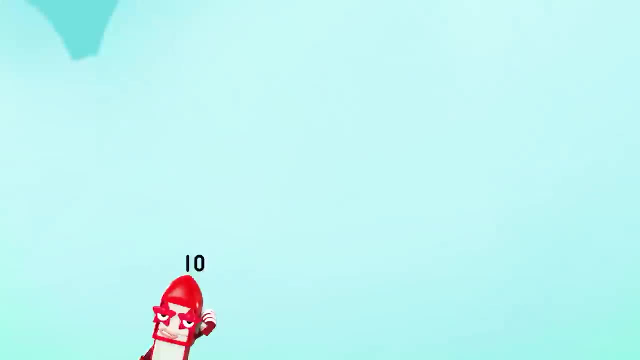 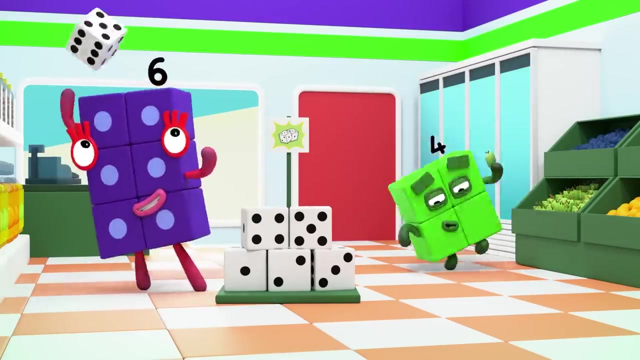 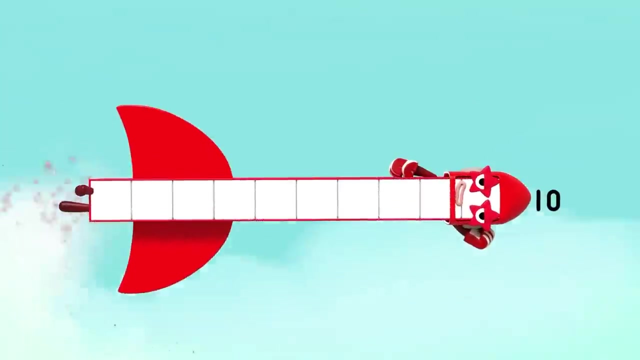 I'm ten, ten, ten and I'm flying through the sky. and I'm flying through the sky, and then I'm ten, ten, ten again I can be six plus four. shopping at the store, playing with the dice on a square tile floor, and then I'm ten, ten, ten again. I can be five. 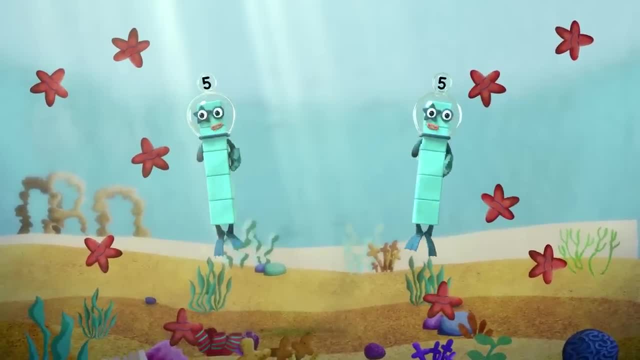 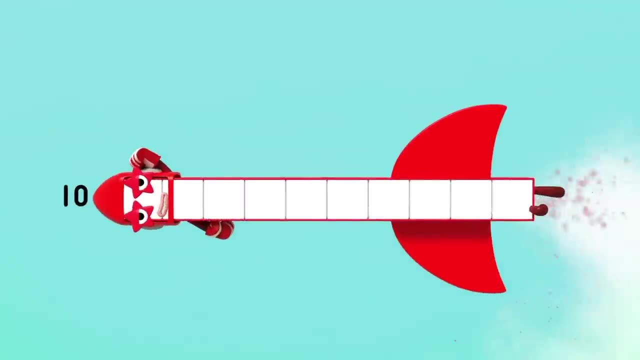 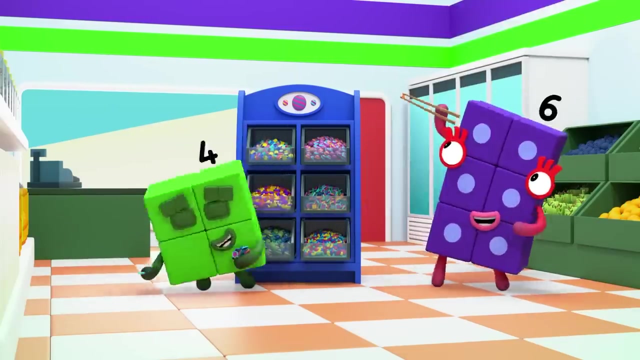 plus five on the school dive, swimming with the starfish and doing a jive. and then I'm ten, ten, ten again I can be four plus six, buying pick and mix, picking out the square ones and using chopsticks. 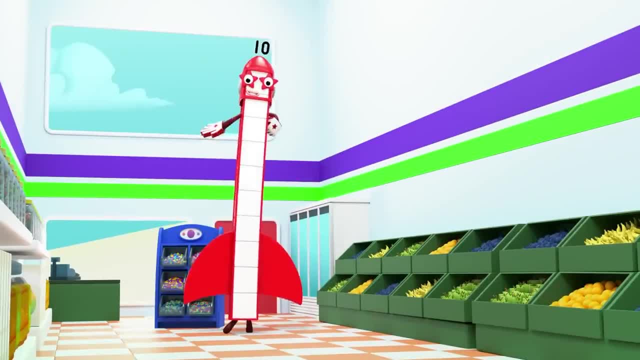 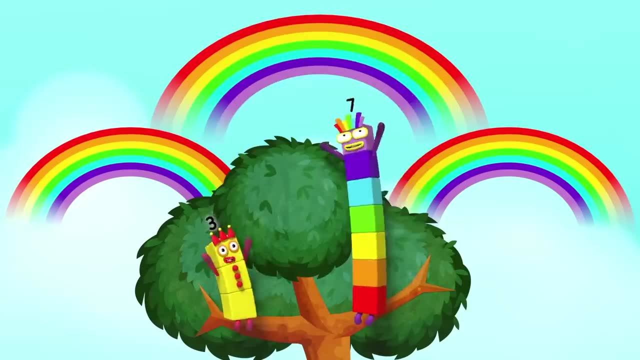 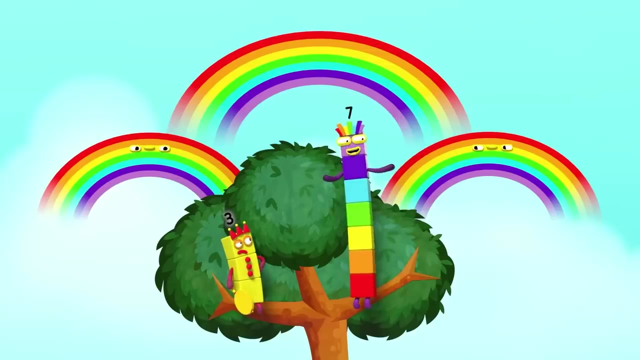 and then I'm ten, ten, ten again. I can be three plus seven, gazing up to heaven- no, looking at me, and a rainbow called Kevin. Kevin, and all my rainbows have names: Kevin, Rainbow, Dina, and that's Big Bob, hello. and then I'm ten, ten, ten again. I can be five. plus six, buying, pick and mix, picking out the square ones, and then I'm ten, ten, ten again. I can be six plus seven, buying, pick and mix, picking out the square ones, and then I'm ten, ten, ten again. I can be five plus seven, gazing up to heaven, no, looking at me, and then I'm ten, ten, ten again I can be six plus seven, gazing up to heaven, no, looking at me. and then I'm ten, ten, ten again I can be five plus seven, gazing up to heaven. no, looking at me, and then I'm ten, ten, ten again. I can be five plus seven, gazing up to heaven. no, looking at me, and then I'm ten, ten, ten again. I can be six plus seven. 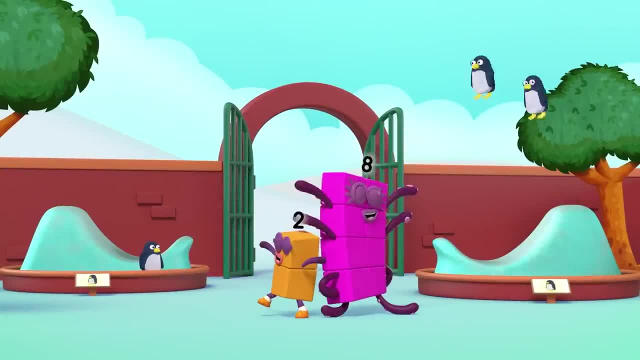 gazing up to heaven- no, looking at me, and then I'm ten, ten, ten again. I can be six plus seven- gazing up to heaven- no, looking at me, and then I'm ten, ten, ten again gazing. 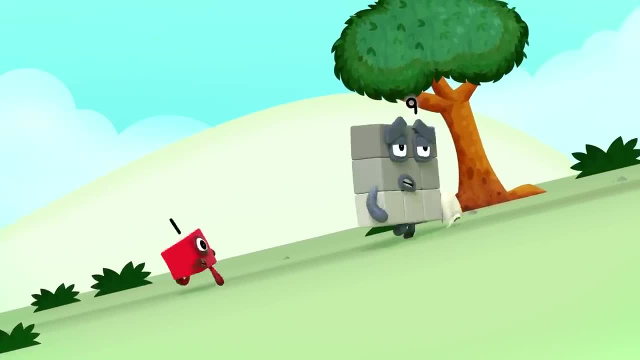 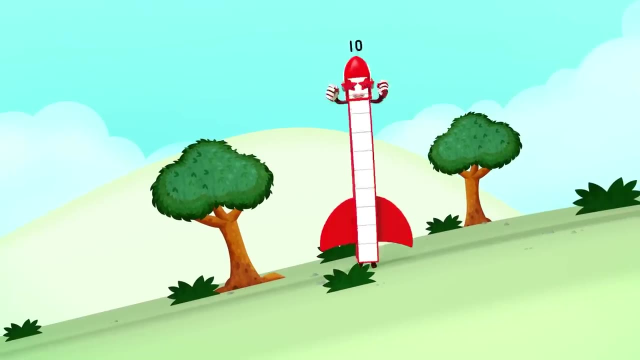 up to heaven, no, looking at me. and then I'm ten, ten, ten again. I can be six plus seven. gazing up to heaven, no, looking at me, hee-ah. eight plus seven: get ten, ten, ten, getting ten, ten, ten again. if I'm ten, ten. 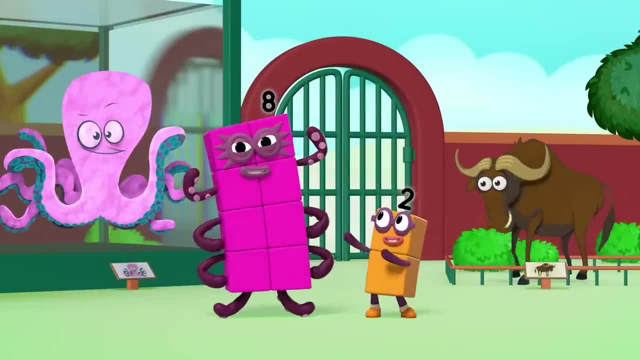 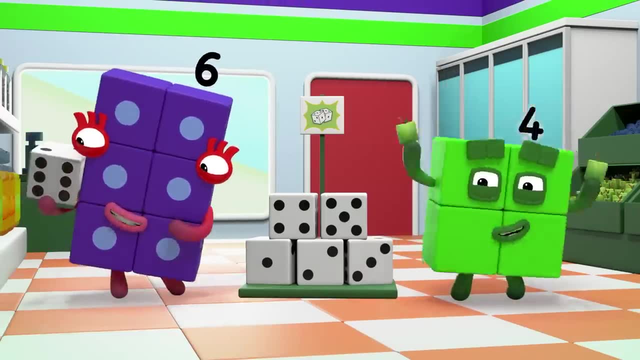 Ten Nino out Suzuka in Ten ten Johno Nino out Dah- 7 plus 3,. sitting in a tree: 6 plus 4, shopping at the store: 5 plus 5,. on a scuba dive: 4 plus 6, buying bigger mix. 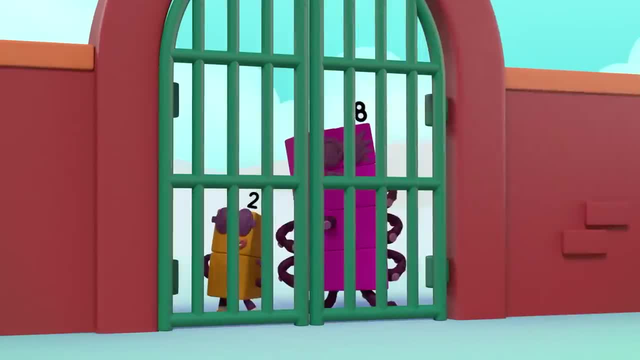 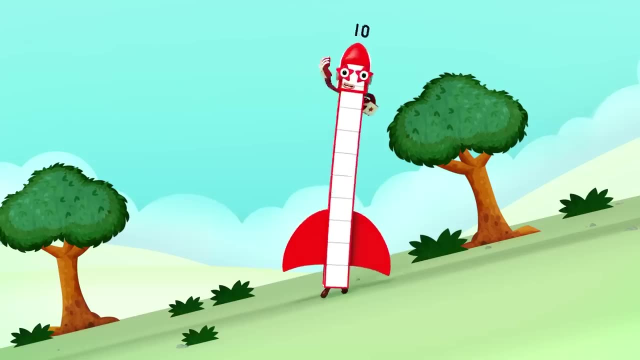 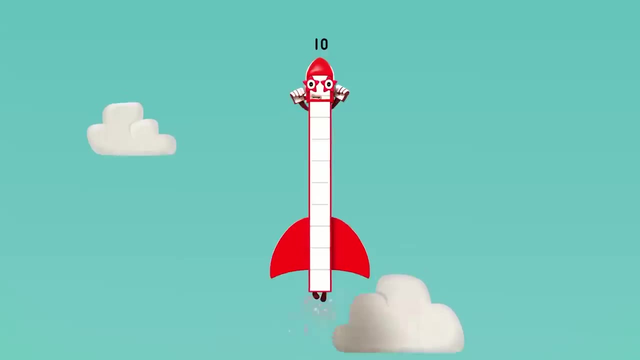 3 plus 7, gazing up to heaven: 2 plus 8, opening a gate, 1 plus 9, starting on a climb. and then I'm 10, 10, 10 again, again 9 plus 1, 10, again 8 plus 2, 10 again. 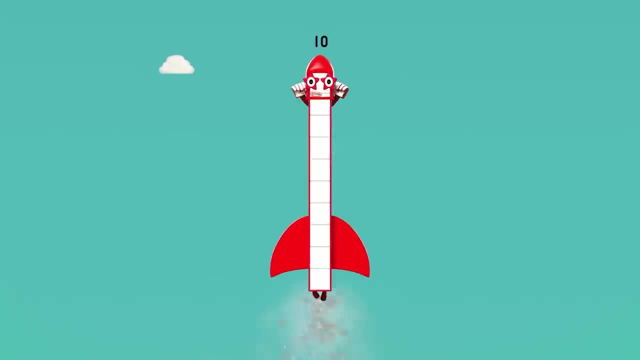 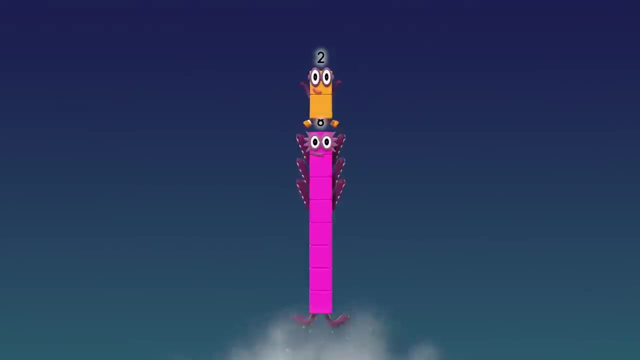 7 plus 3, 10, again 6 plus 4, 10, again 5 plus 5, 10, again 4 plus 6, 10, again 3 plus 7, 10, again 2 plus 8, 10 again. 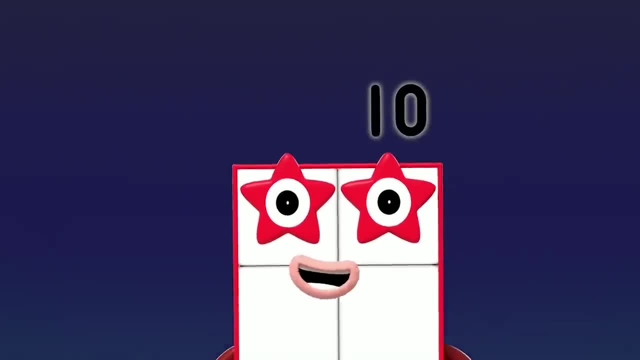 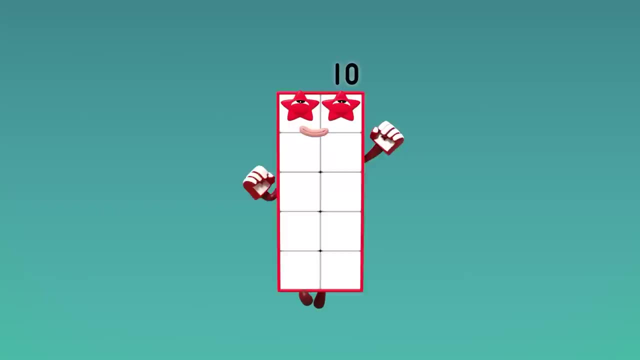 1 plus 9,, 10, again 10,, when 10, again 9 plus 1, 10, again 8 plus 2, 10, again 7 plus 3,, 10, again 6 plus 4, 10 again. 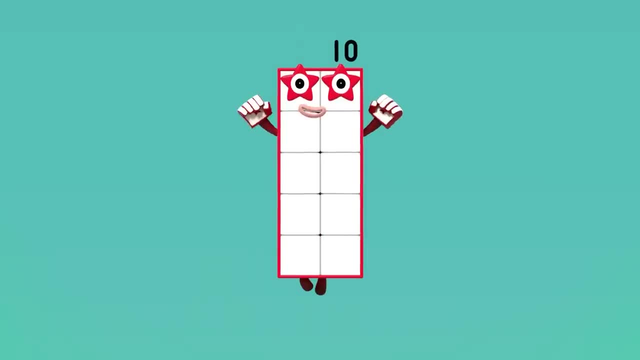 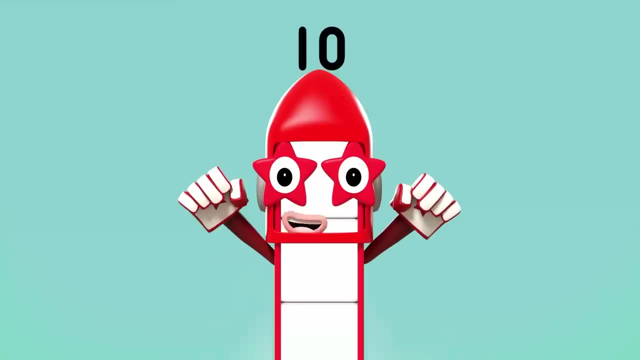 5 plus 5, 10, again 4 plus 6, 10, again 3 plus 7, 10, again 2 plus 8, 10, again 1 plus 9, 10, again 10, 10, 10, again again. 9 plus 1 or 1 plus 9, 10, 8 plus 2 or 2 plus 8, 10, 7 plus 3 or 3 plus 7, 10, 6 plus 4 or 4 plus 6, 10. 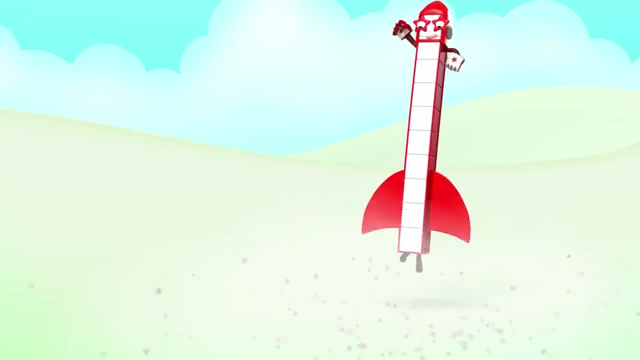 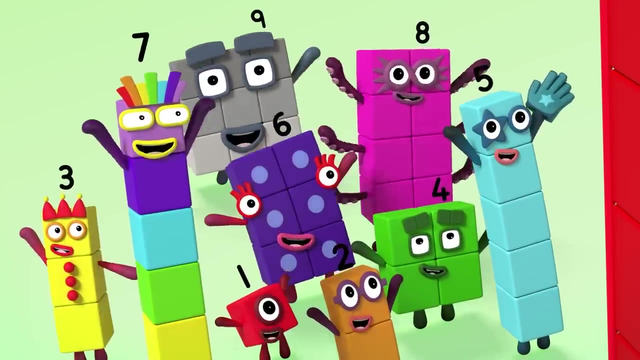 5 plus 5 or 5 plus 5, 10, 10, 10, 10 again, 10, 10, 10 again, 10, 10, 10 again. And what do you want to do today? Ten? 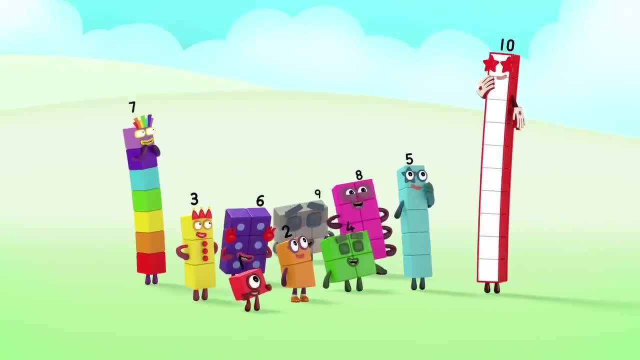 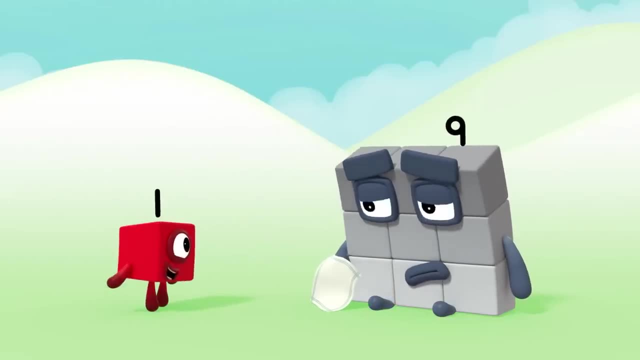 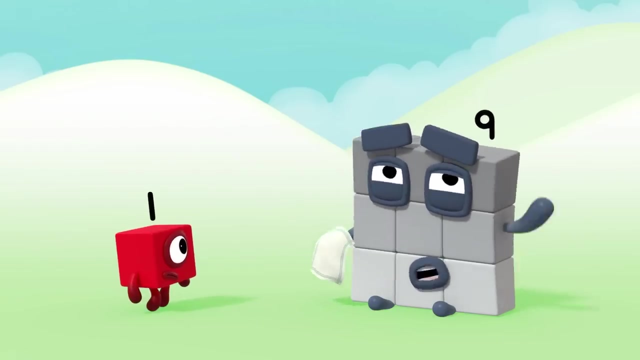 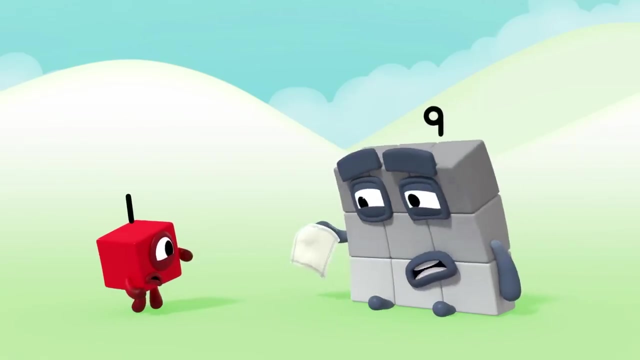 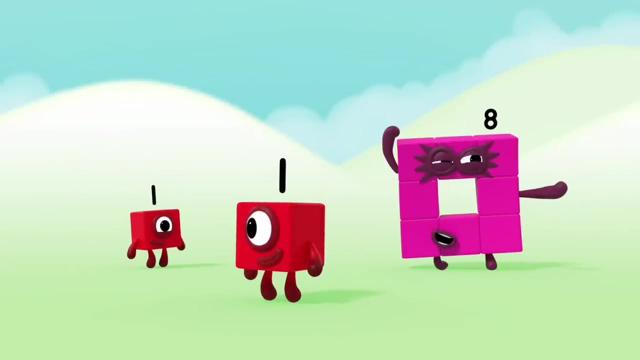 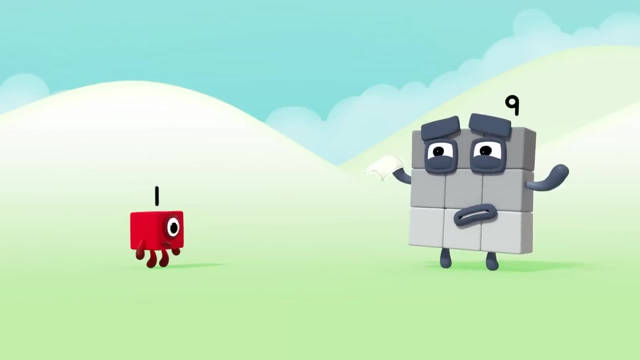 I need a nap, Hello Nine. What's the matter? One smaller? I always get one smaller. Huh, Every time I sneeze I get one smaller. Achoo, Oh See, Why can't I ever get one bigger? Maybe you can stand tall. 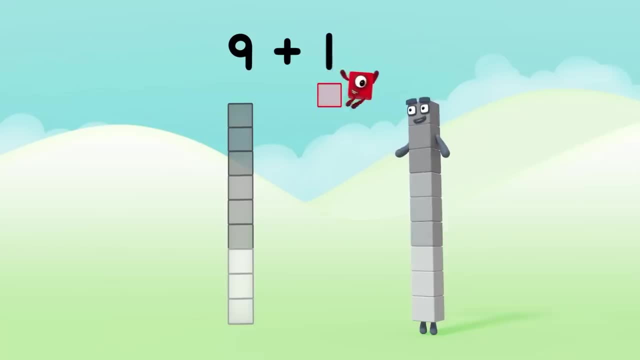 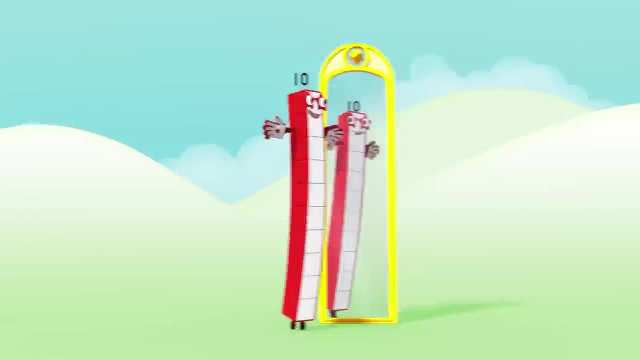 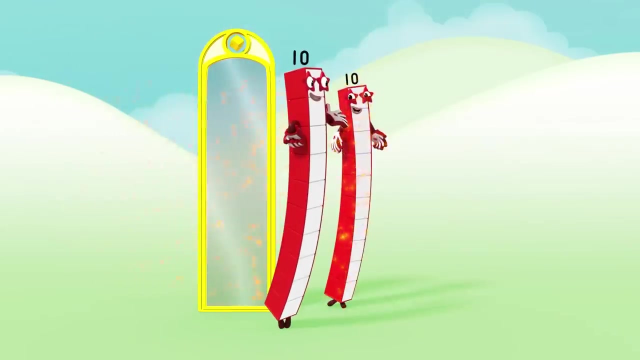 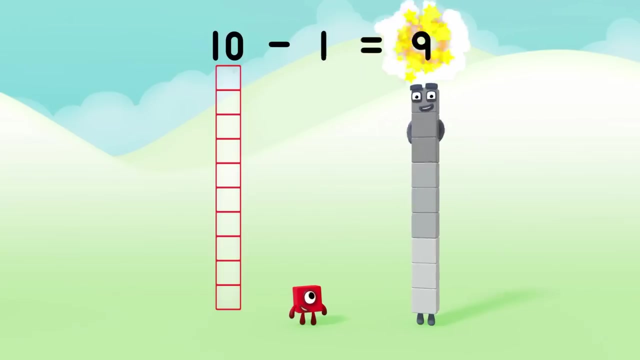 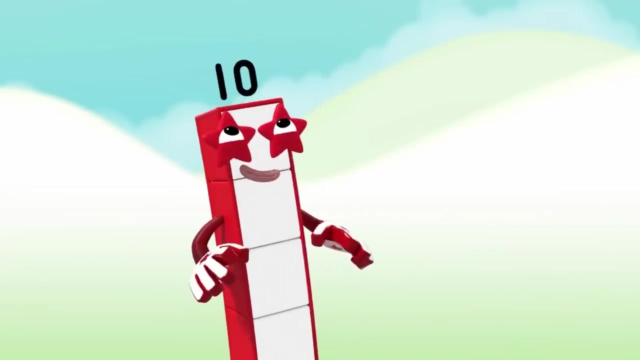 9 plus 1 equals 10. I am 10. Say it again: I am 10. Watch this: 10 minus 1 equals 9. Oh, You're amazing. One bigger. You're one bigger. Why do you have a 1 on top? If you're wondering why there's a 1 on top, 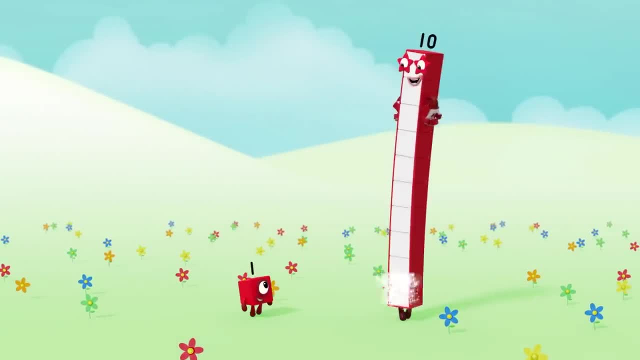 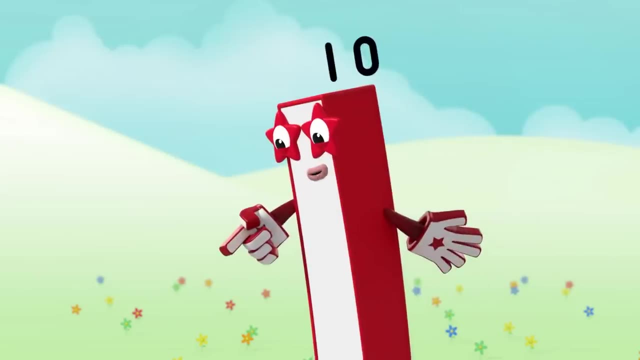 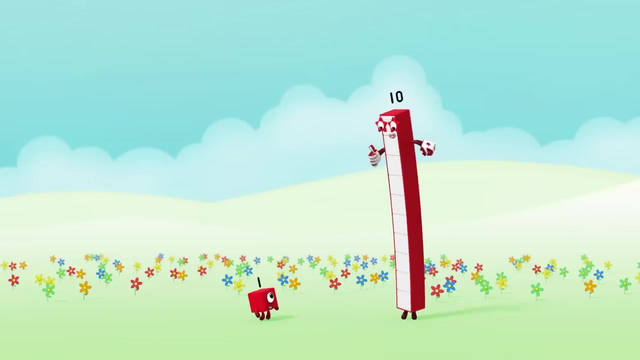 You'll know the answer when You realise I'm one big block. I'm one big, perfect 10. I'm a 10 block, I'm a 10 block. You might think we're different. Think again. We're more alike than you suppose. You're 1-1. 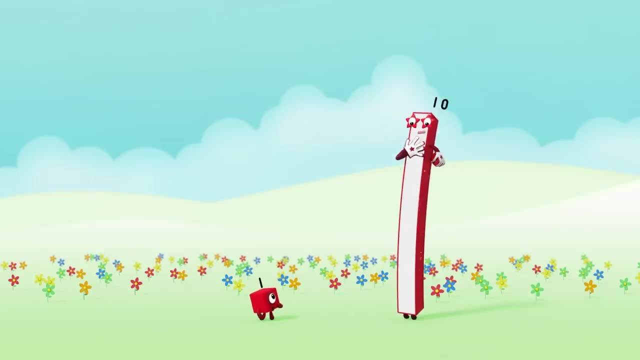 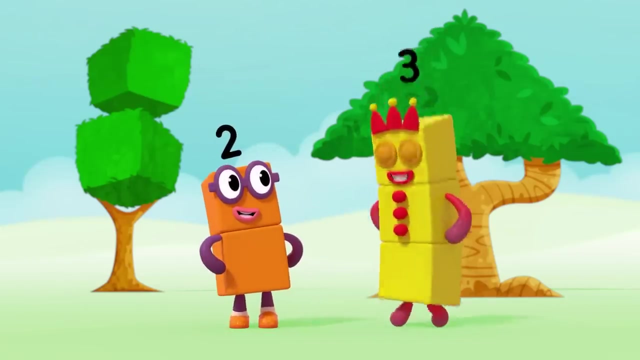 And I'm 10 ones, which means I'm 1-10, 1-2-3-4-5-6-7-8-9-10. 2 is made of 2 blocks. I'll always be your friend. 3 will entertain you. 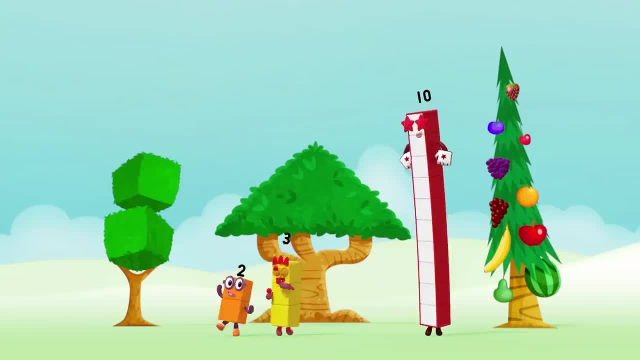 On that you can depend. I'm 2 ones And I'm 3 ones And I'm 10 ones, which means I'm 1-10, 1-2-3-4-5-6-7-8-9-10. 4 is made of 4 blocks. 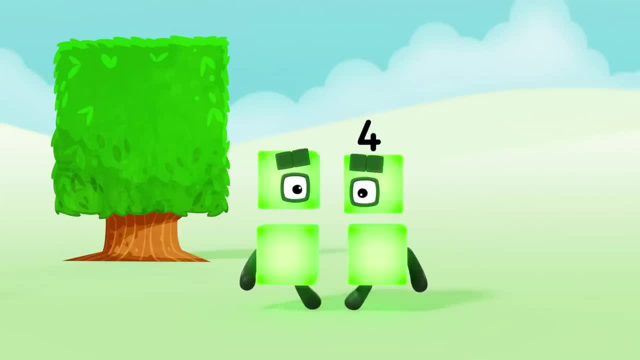 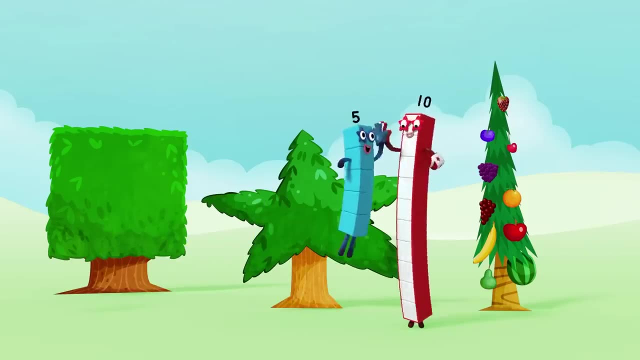 I love to be. a square 5 is made of 5 blocks. High five There. I'm there. I'm 4 ones And I'm 5 ones And I'm 10 ones, which means I'm 1-10, 1-2-3-4-5-6-7-8-9-10. 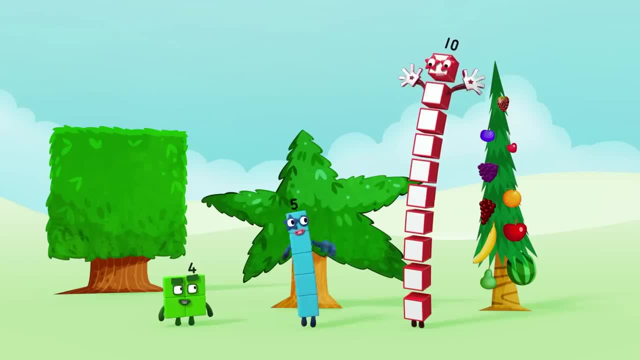 Oh, why have you got that? I'm 1-10, 1-2-3-4-5-6-7-8-9-10, 1-2-3-4-5-6-7-8-9-10. 1-2-3-4-5-6-7-8-9-10, 1-2-3-4-5-6-7-8-9-10, 1-2-3-4-5-6-7-8-9-10. 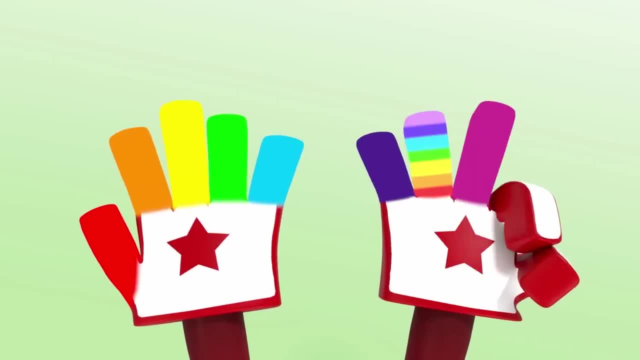 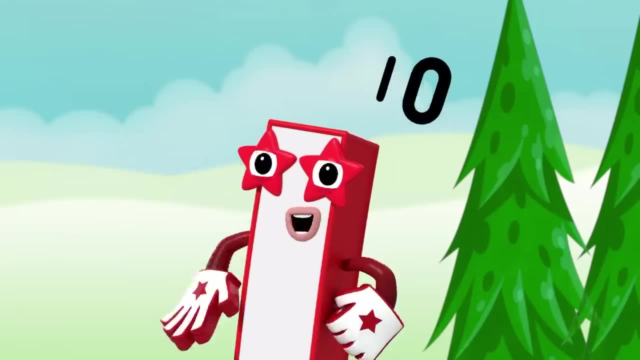 Why have you got that round thing next to your 1?? It's a zero. I need my zero hovering in space. It's there to keep my 1 in place And if you're wondering what it's for, It shows you I'm not one, I'm 1-10 and nothing more. 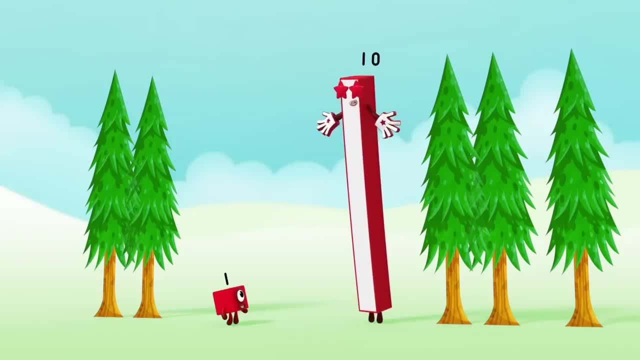 6 is made of 6 blocks. I love to be a square: 5 blocks. I love to be a square: 1-2-3-4-5-6-7-8-9-10. 1-2-3-4-5-6-7-8-9-10. 1-2-3-4-5-6-7-8-9-10, 1-2-3-4-5-6-7-8-9-10, 1-2-3-4-5-6-7-8-9-10. 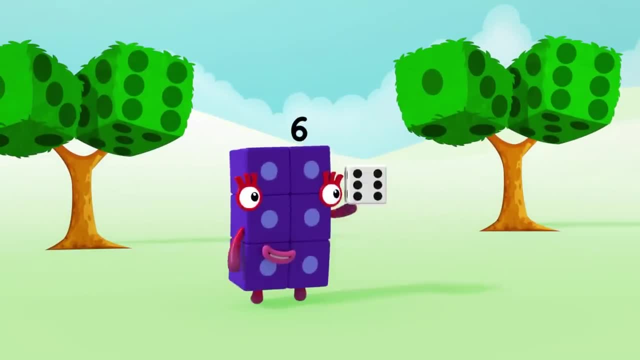 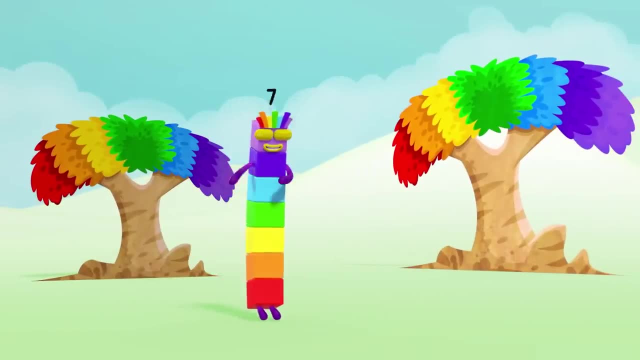 Six is made of six blocks. I like to roll the dice: Seven's made of seven. In a rainbow That looks nice. I'm six once And seven ones, And I'm ten once, Which means I'm 1-10, 1-2-3-4-5-6-7-8-9-10. 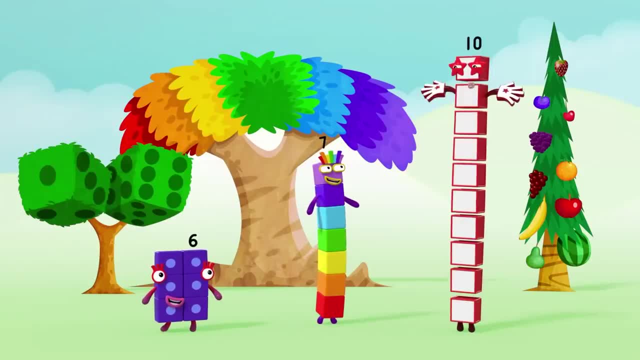 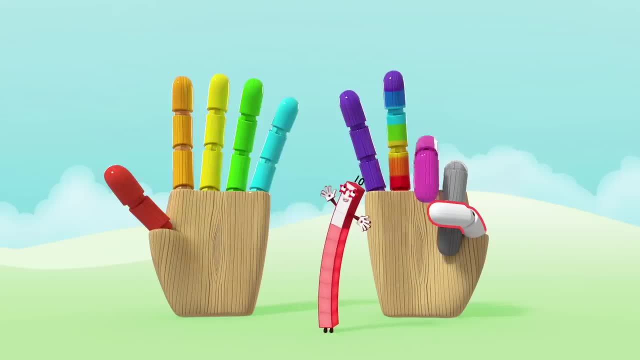 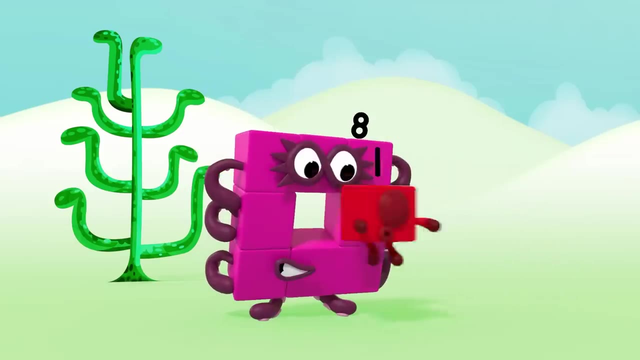 8 is made of Octoblocks And blocks And snow Tatas And JJ. And While I'm down, It's my turn. Let me find a spot Where I can rock. Come on, let's organizing you up, If you add one more. Nine is made of nine blocks. 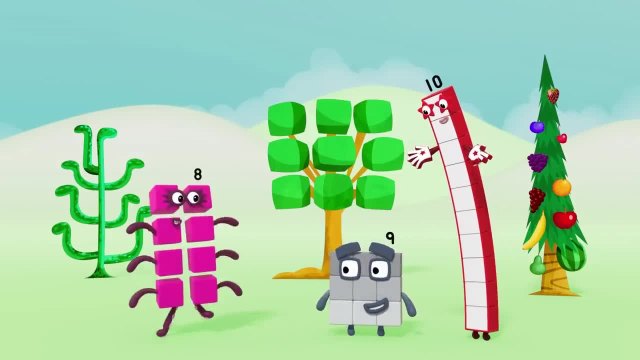 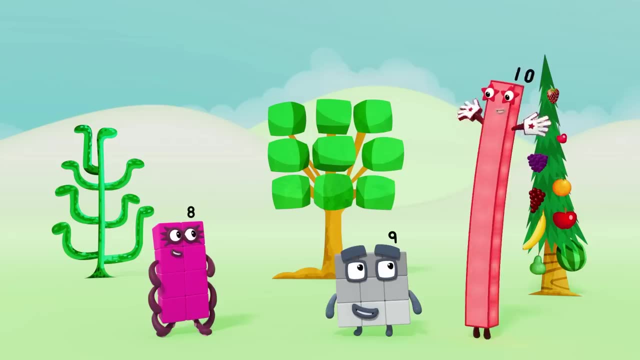 I'm a bigger square than four, I'm eight ones And I'm nine ones And I'm ten ones, which means I'm one, ten, One, two, three, four, five, six, seven, eight, nine ten. 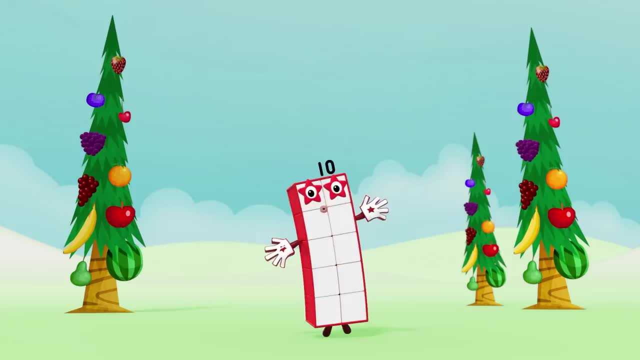 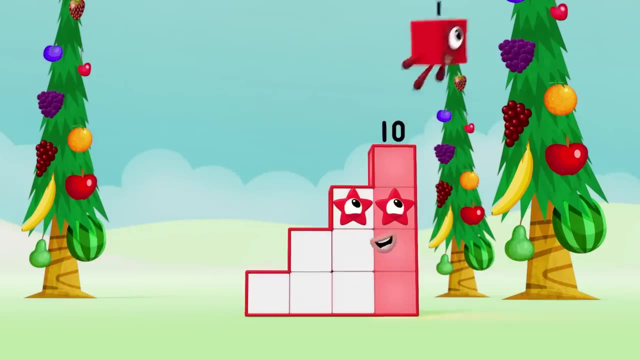 I can be two lots of five, or five lots of two, In other words, five pairs. I can be one and two and three and four. when you need to go upstairs, I'm a ten block. I'm a ten block. You might think we're different. 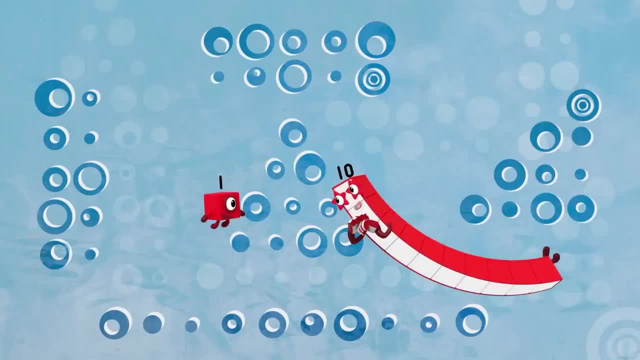 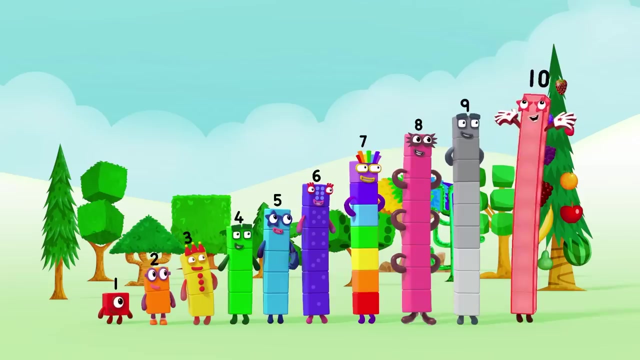 Think again. We're all just made of counting blocks. You're one one And you're ten ones, Which means I'm one, ten, One, two, three, four, five, six, seven, eight, nine, ten. I'm a ten. 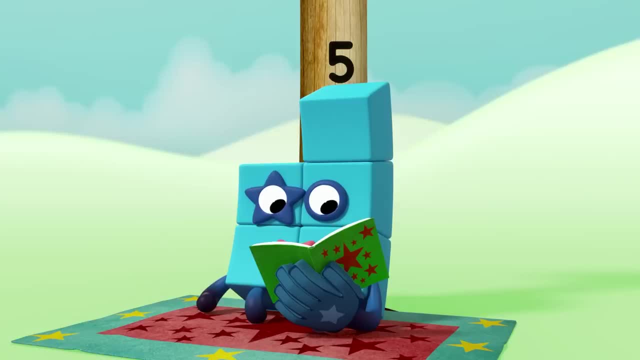 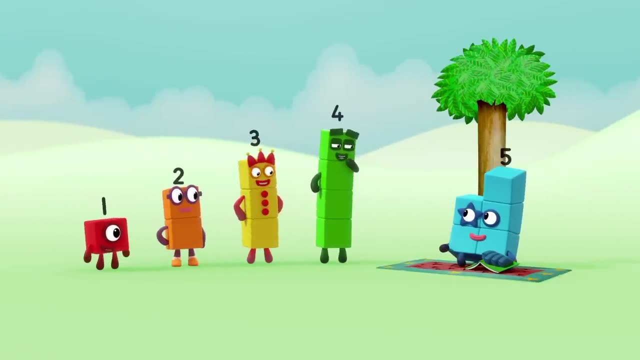 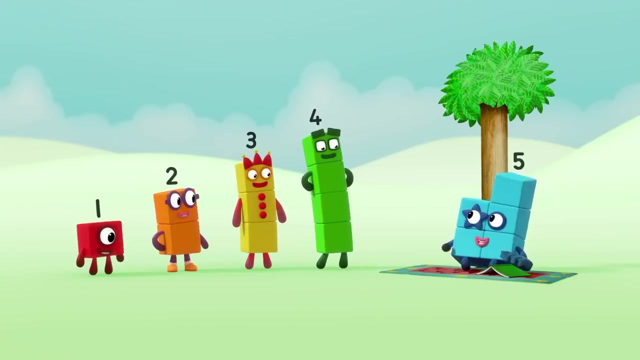 What do I do? I win. I win One, Two, Three, Four, Two, Three, Go Two Three. One Two, Seven, Six Eight Nine. The other one is a ten block. You're a ten block. 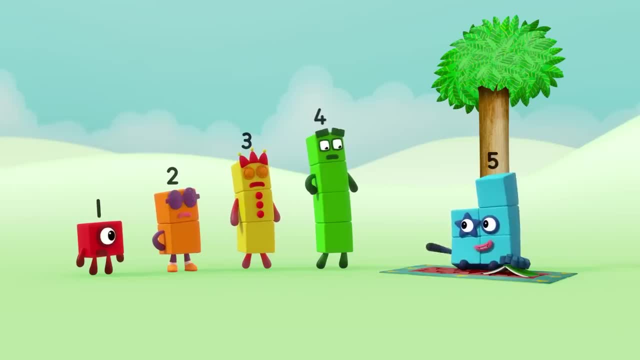 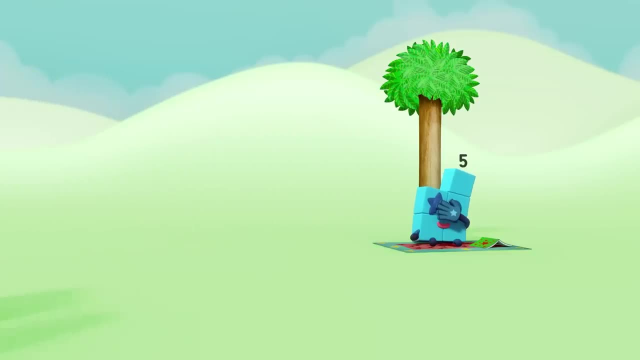 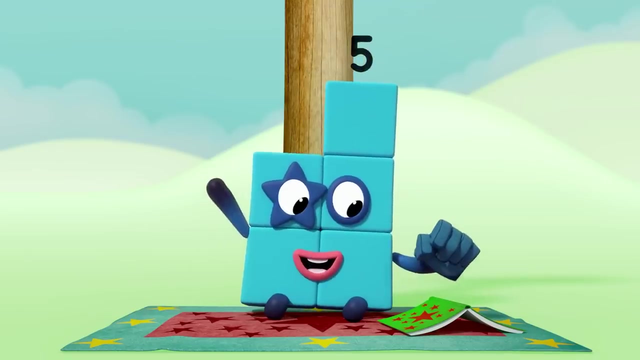 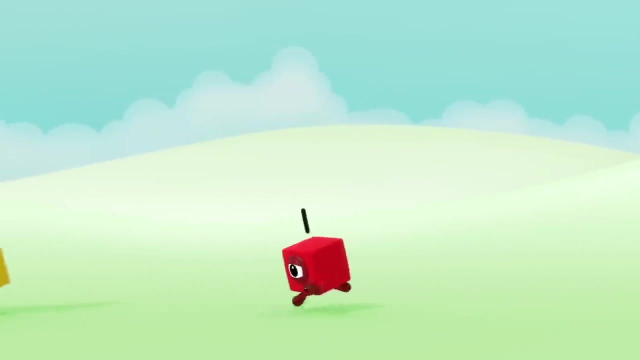 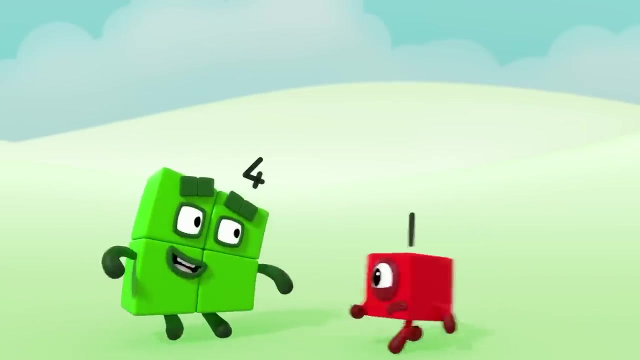 Eта looks like a lame Christianity contract Basic and honestly, Eta One, two, three, four, five, Ready or not, here I Get on with my book. Hey, Hide behind me, Where can I hide? I know, Behind you. 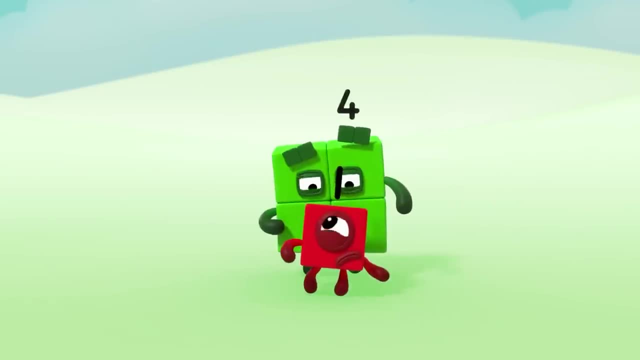 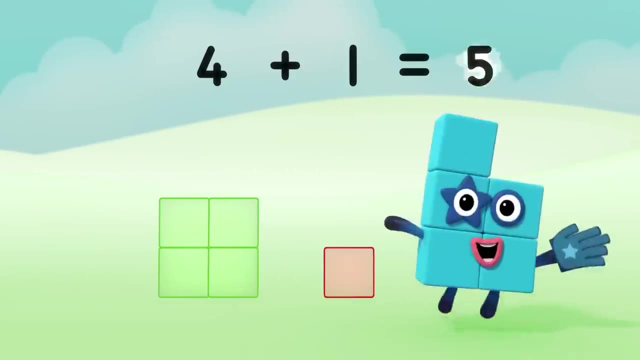 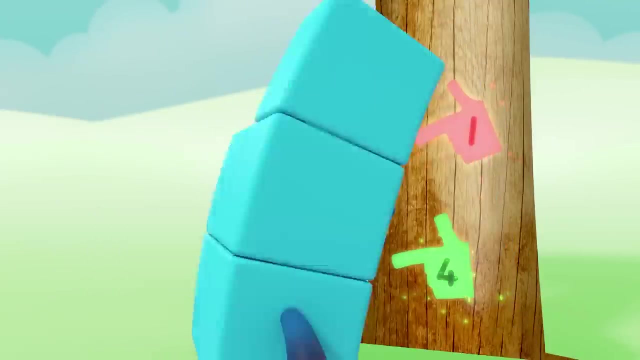 Four, Oops Huh. Four Plus one Equals Five. Ready or not, here I come. Find you four, find you one. Five minus one Equals four. Look Five, said she'd point us out to you. 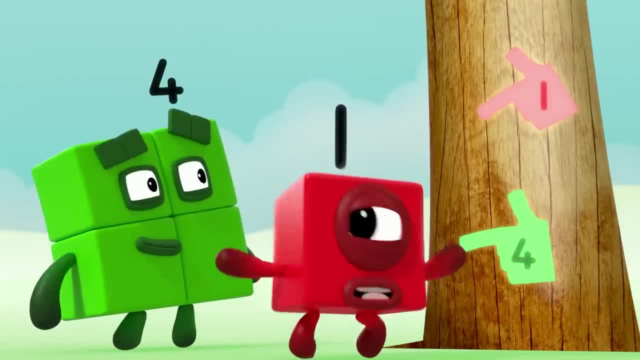 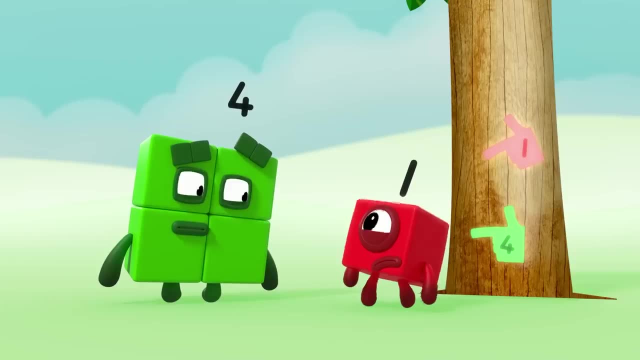 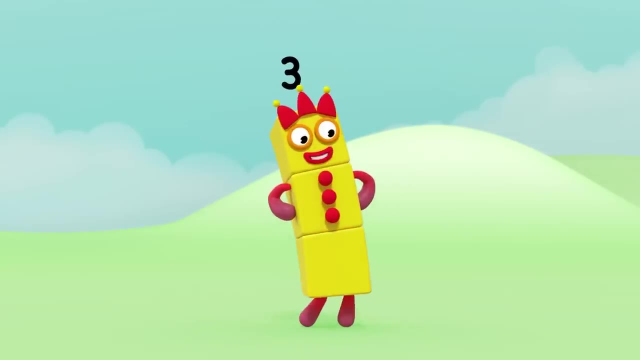 Oh, Oh, Oh Oh. Five was right here. How I am. Three Master of Disguise, Shhh Shhh. Two Pussies, Three Equals Five. Ready or not? here I be. 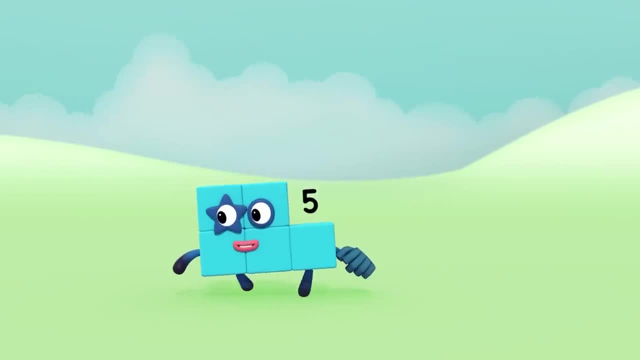 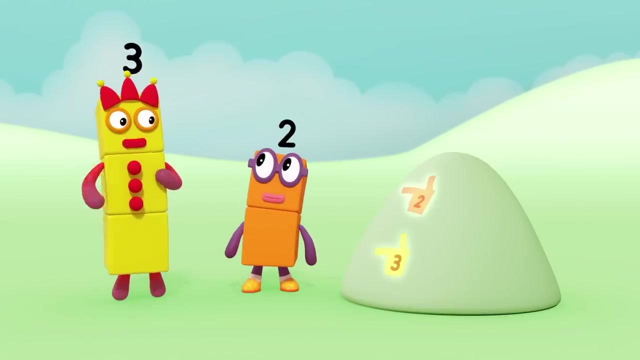 Find you two, find you three. Five minus Three Equals two. Huh, A pair of pointing prints. Five found us. Bu Bu, How There, Five, You're here. How did you Told you I was good? 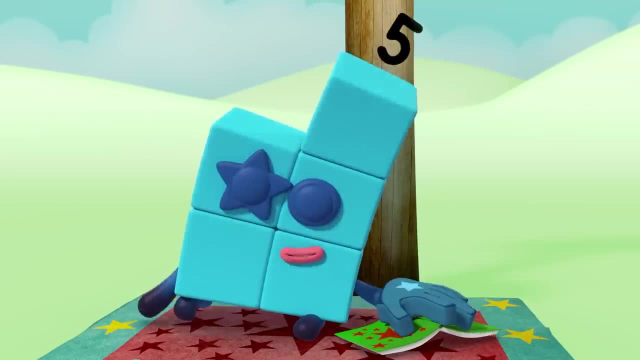 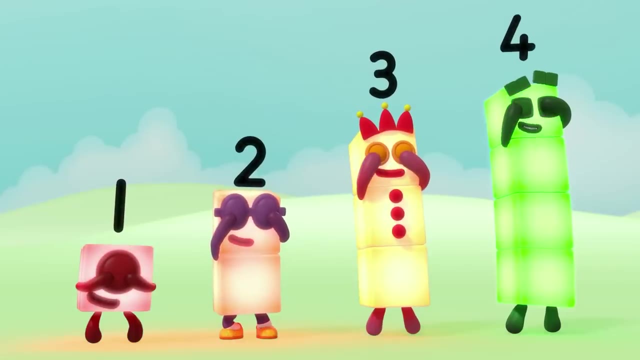 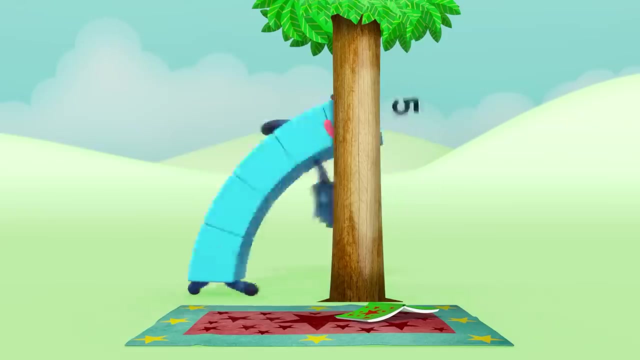 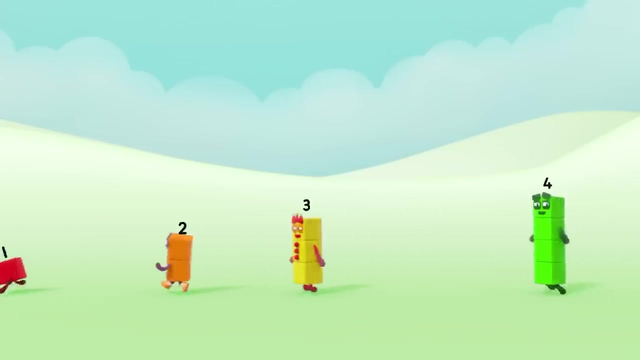 Now my turn to hide All the way down. One, two, three, four, Ready or not? five, here we come. Ooh Rock, Hup, Hup, Hup, Ooh, Whoa One. 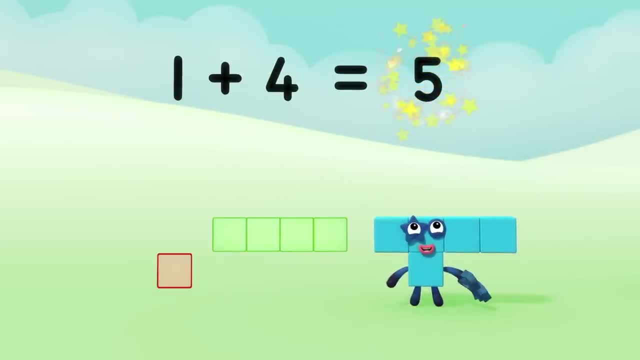 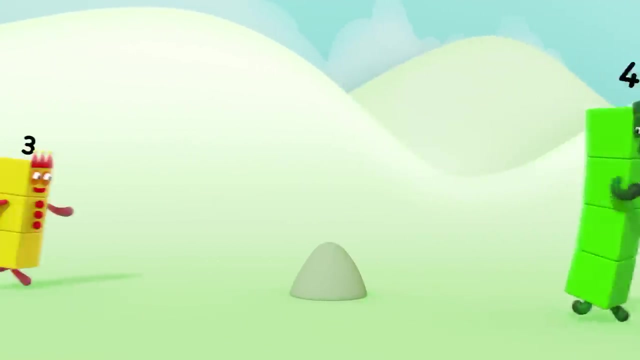 plus four equals five. Found you Amazing? Can you find me again? Five minus four equals one. Come on, Rock Hup Ooh, Look Ooh. Three plus two. 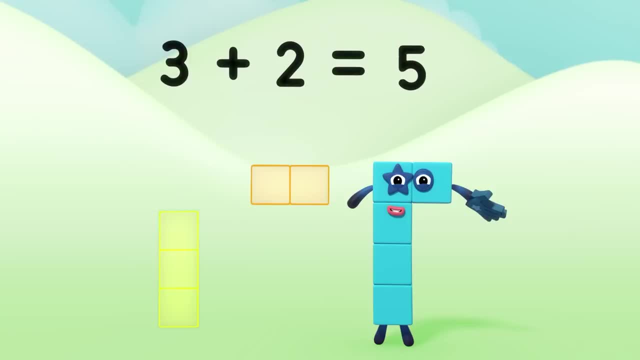 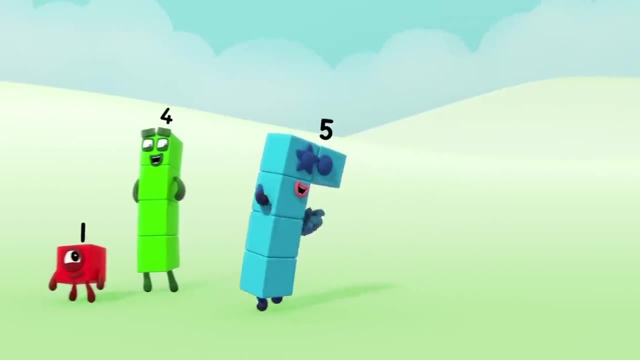 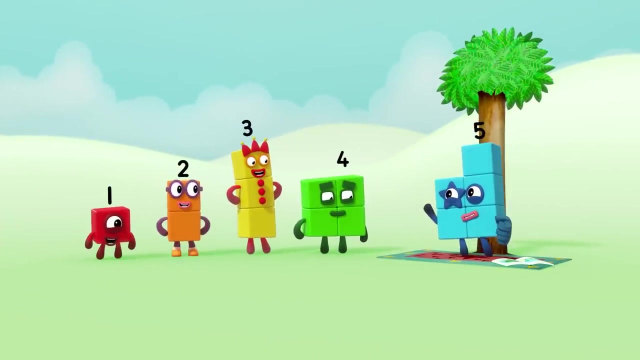 equals five. Found you. Fine, Fantastic, Can you find me again? Five minus two equals three. Found you. Hup, Hup You stars, Hup. You all found me, Yay. 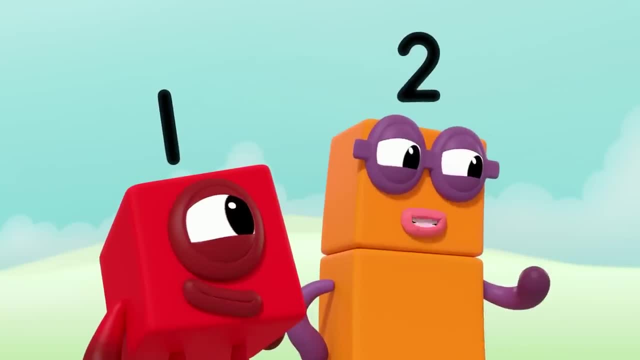 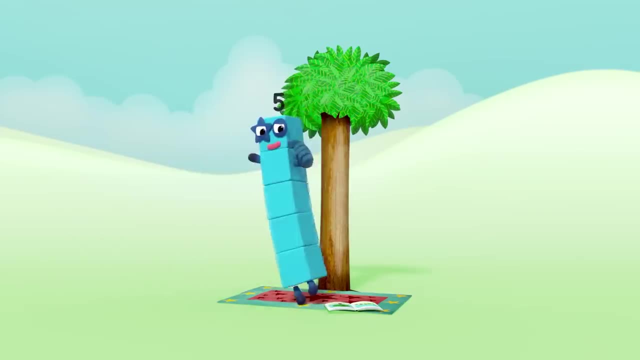 Yay, Yay, Yay. Can you teach us to be as good at hide-and-seek as you? Sure, I can Try this. Hup, Hup, Hup, Ah, Hup, Hup, Hup. 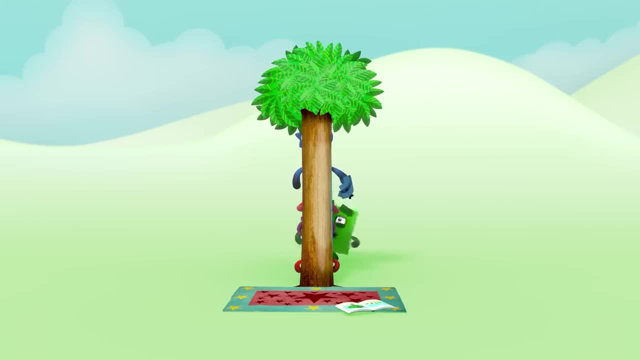 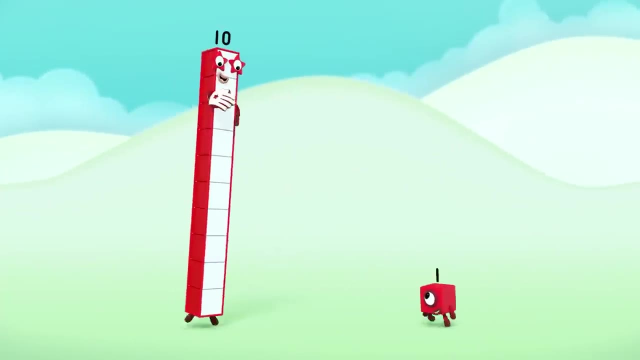 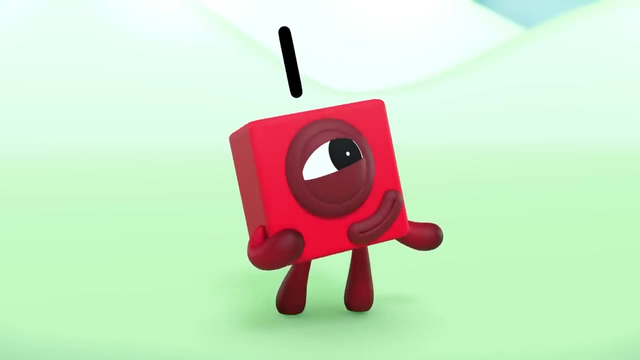 Hup Hup, Four, Hup Hup, Hup, Hup, Hup Hup. Hello Ten, Hello One. What shall we play today? Oh, Ooh, um, Hmm, Hmm. 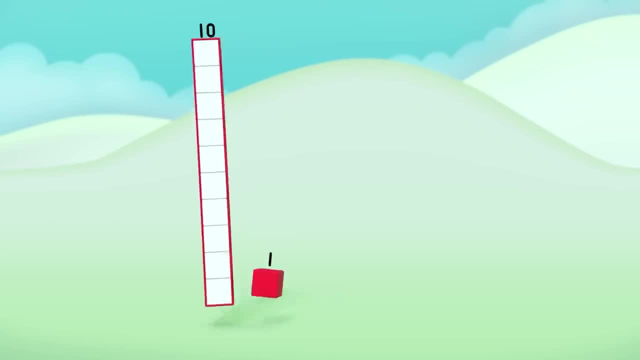 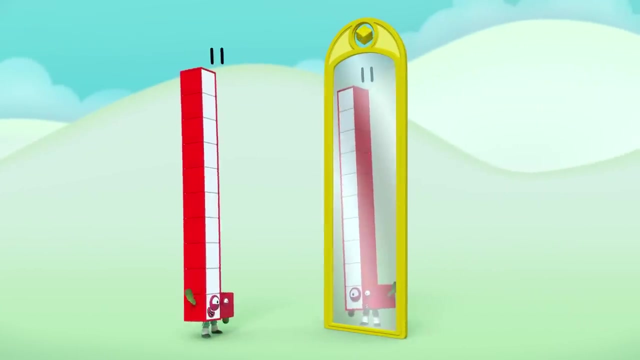 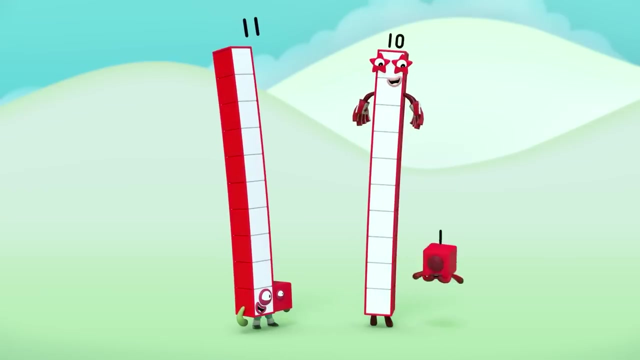 Ah, What was that? Who was that? A new number. block Ten plus one equals eleven. Hello, I'm eleven, So am I, And I'm ten and one. Oh, Whee Hup. 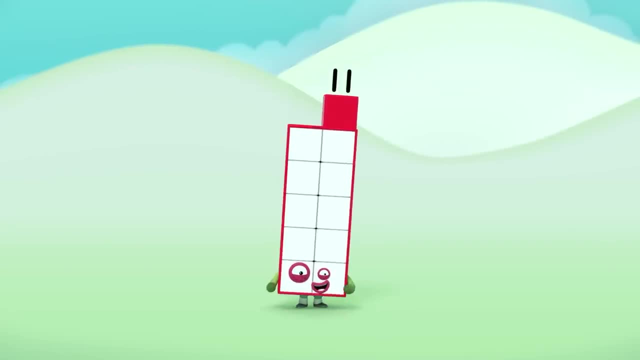 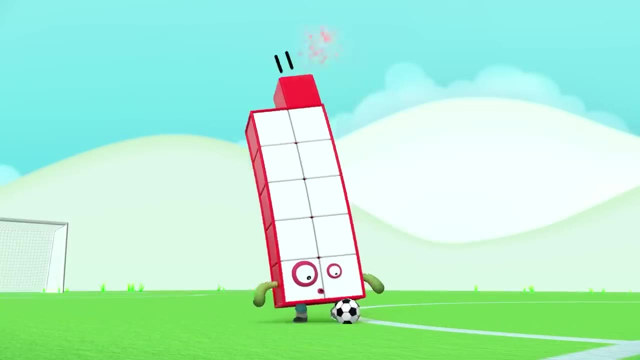 Hup, Hup Hup, That's better. Ooh Hup Hup Whoa. One, two, three, four, five, six, seven, eight, nine and ten Hup. One more is eleven. 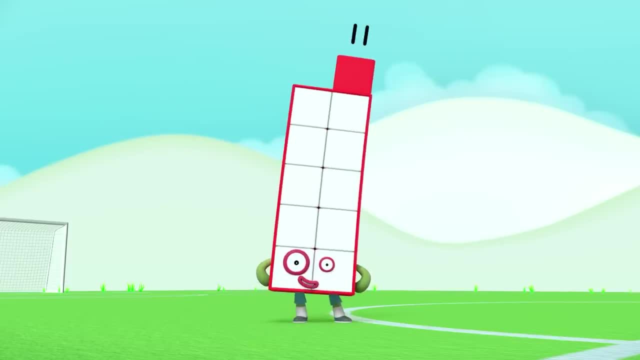 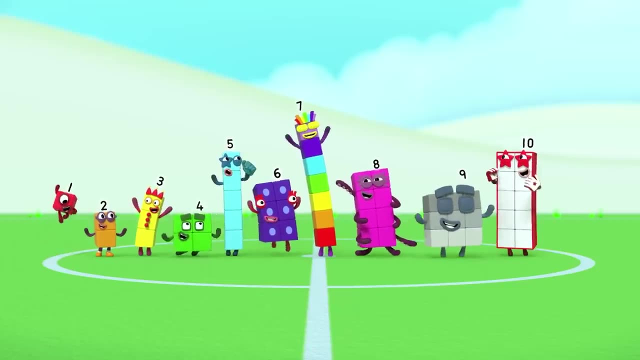 I am eleven And I love football. Hee-hee-hah, Wow, Let's play football, Hooray Hooray. One, two, three, four, five, six, seven, eight, nine and ten. 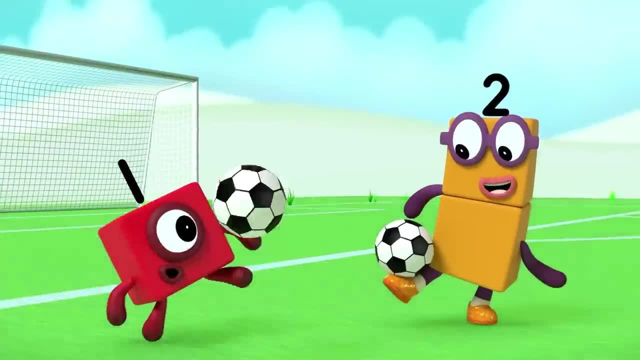 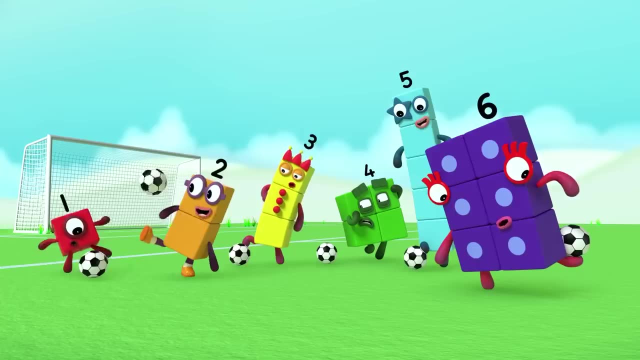 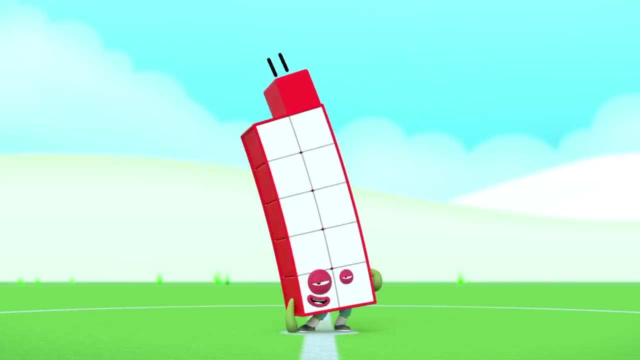 One more is eleven. We're on our way to victory. We're on a roll. We're ten on the pitch and one in goal. We will never be denied. We'll take it in our pride With ten and one. ten and one, eleven on our side. 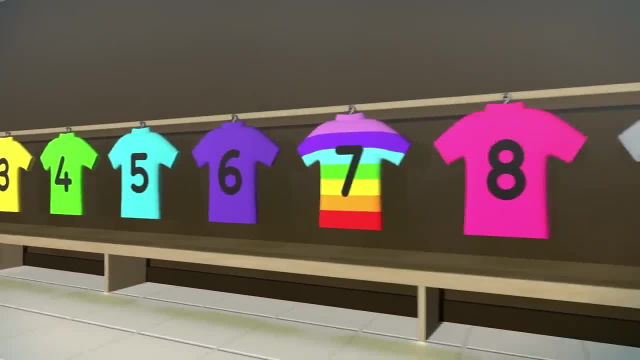 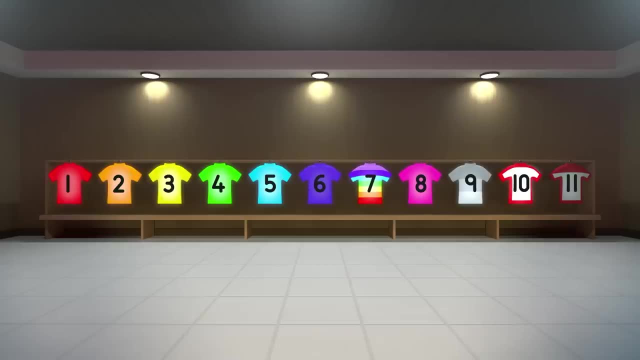 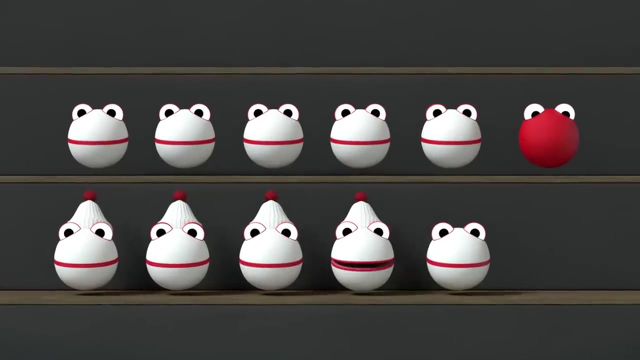 Football shirts. football shirts: one for every number block. Football shirts: one, two, three, four, five, six, seven, eight, nine and ten, And one more is eleven, Hooray. Bubble hats. bubble hats, one for every number block. 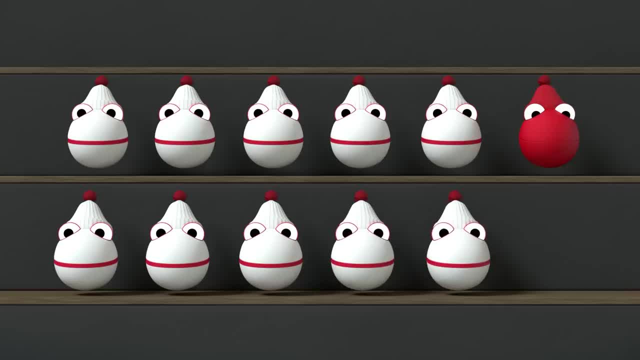 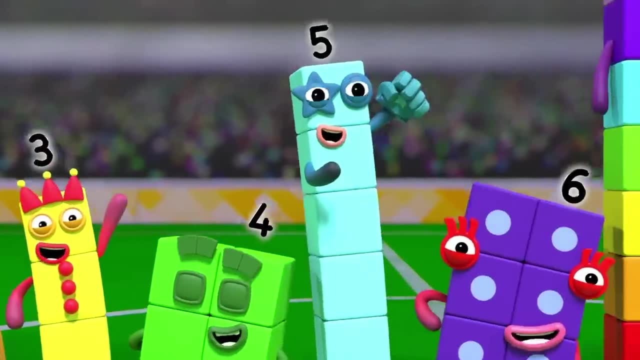 Bubble hats: One, two, three, four, five, six, seven, eight, nine and ten, And one more is eleven. Hooray, We're on our way to victory. We're on a roll, We're ten on the pitch and one in goal. 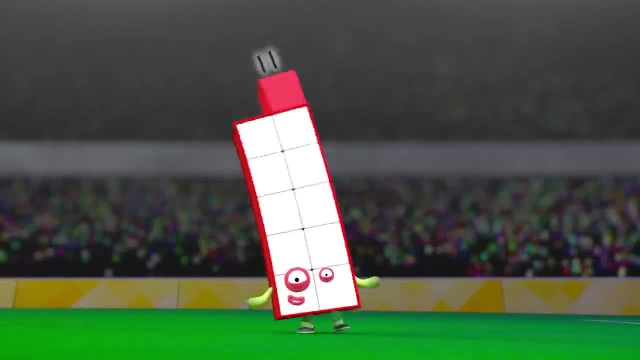 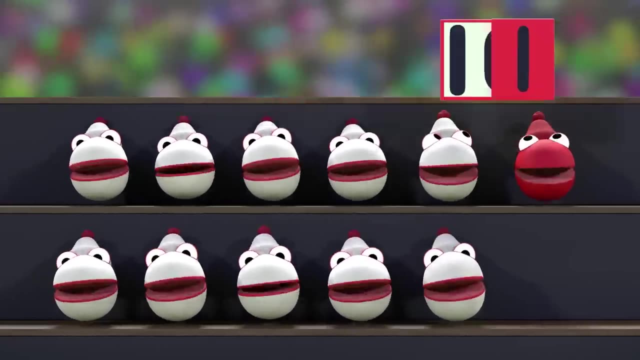 We will never be denied. We'll take it in our pride With ten and one, ten and one eleven on our side. One ten one, one ten and one eleven. One ten one, one, ten and one eleven. 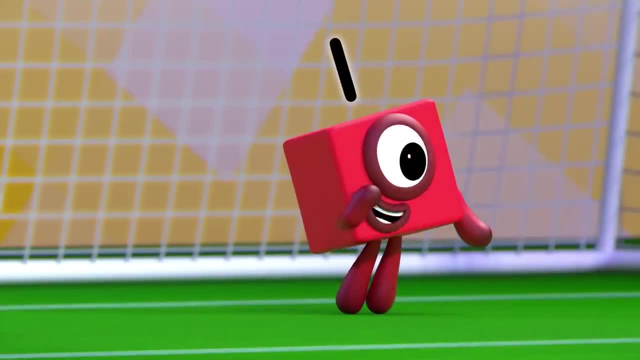 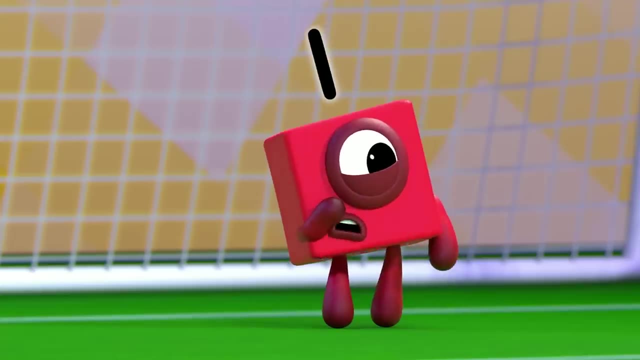 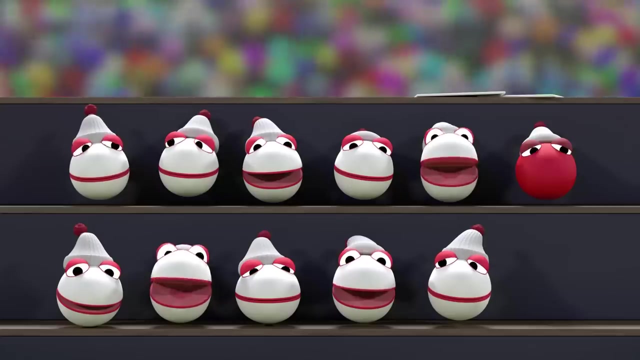 The number blocks are out on the pitch for the big match And their captain, Eleven, looks ready to lead the team to victory. Something's wrong. What can it be? I've forgotten something? The other team. We need eleven more players. 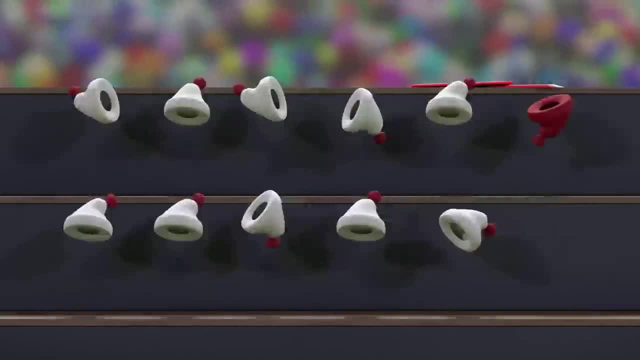 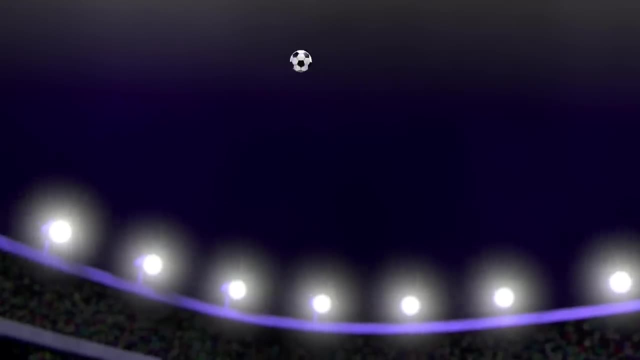 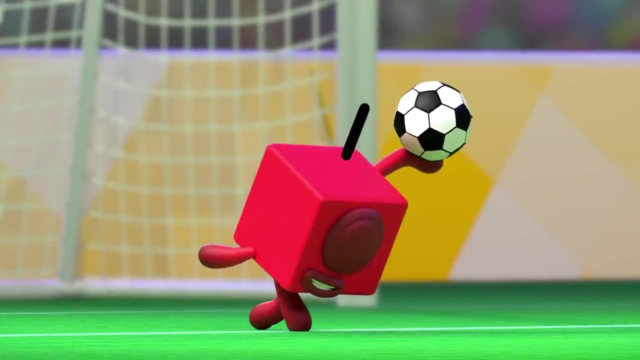 Number loves Game on WHISTLE BLOWS And the number blocks have kicked off. It goes high towards the goal And saved by one. Take a bow, one WHISTLE BLOWS, One throws it down to two. 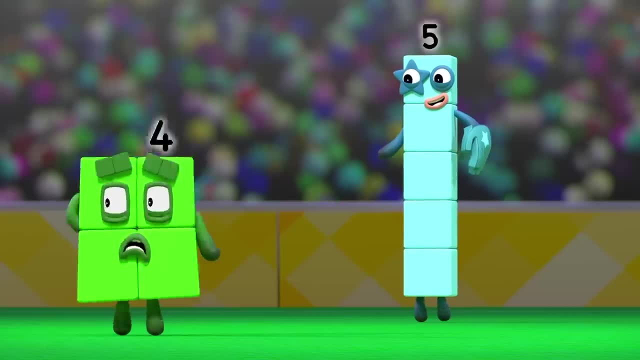 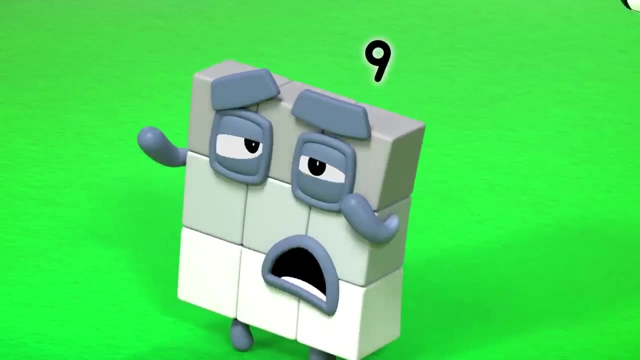 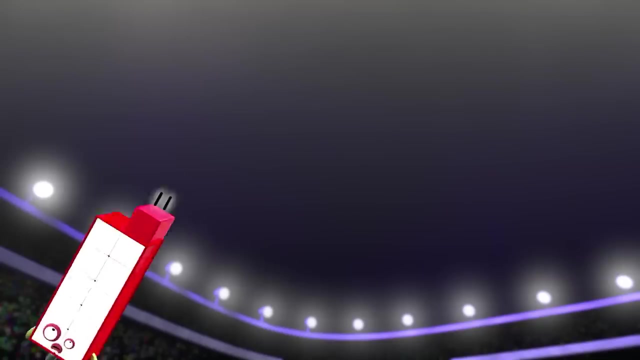 Who passes it? that's right to three, four, five, six, seven, eight, nine and ten. Now pause it to eleven. Ten passes, Eleven seats for the head, The header, and, oh, my, Splits into ten and one to reach the ball. 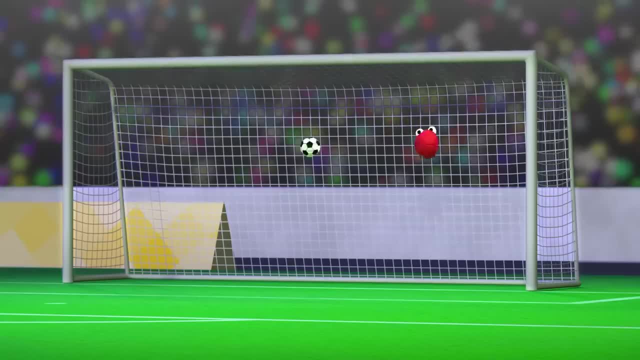 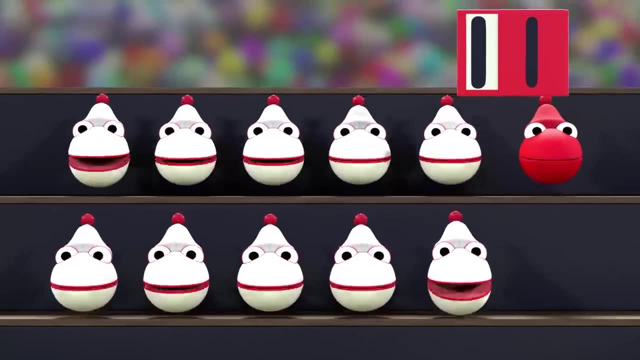 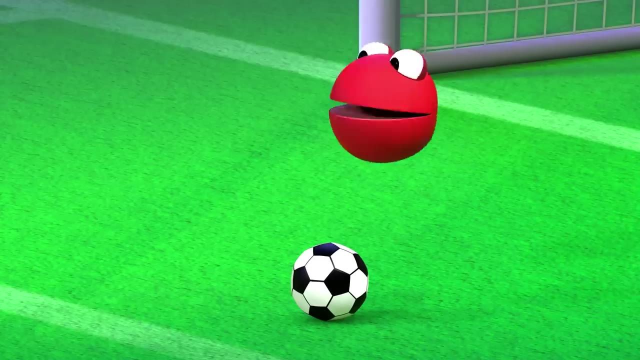 Incredible, And it's a save. What a save. Cut it off. two and one goes louder than the rest. Ten and one. ten and one, eleven is the best Number. Blob passes to Number Blob. who finds Number Blob And a lovely header there to Number Blob. 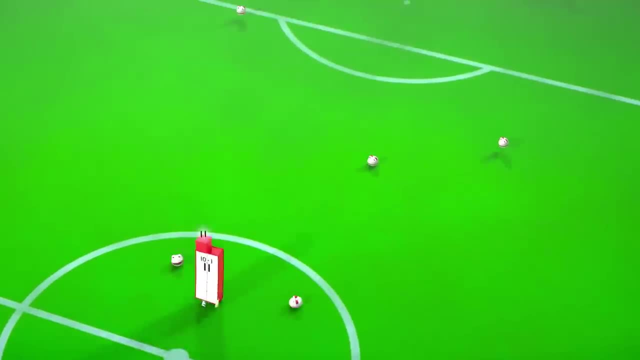 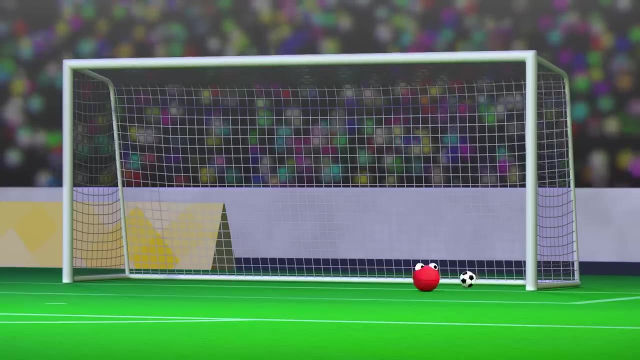 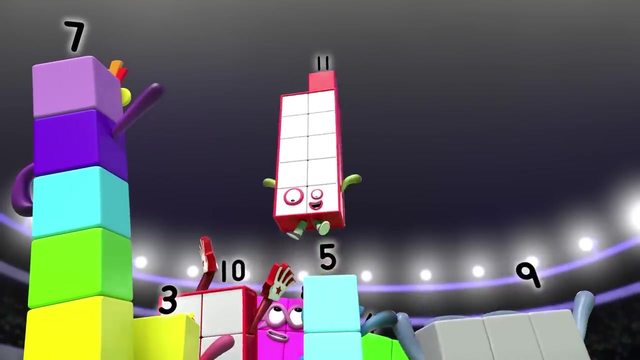 Look, he's alive. He heads it to eleven And it's eleven, Eleven, Eleven. WHISTLE BLOWS, WHISTLE BLOWS, Yeah, Goal. WHISTLE BLOWS, CHEERING. We're on our way to victory. 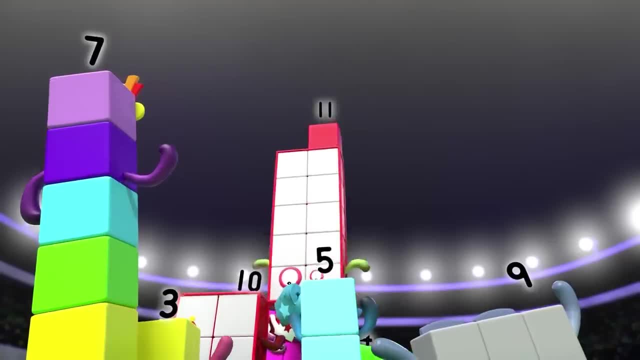 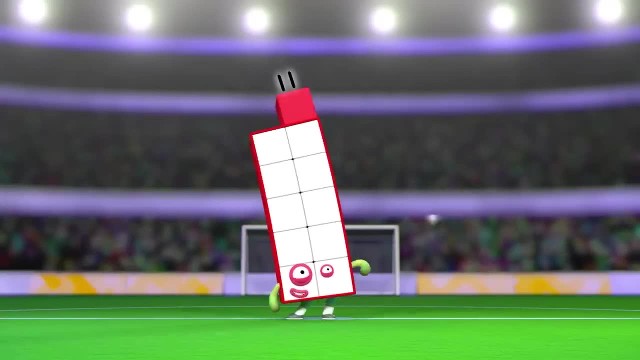 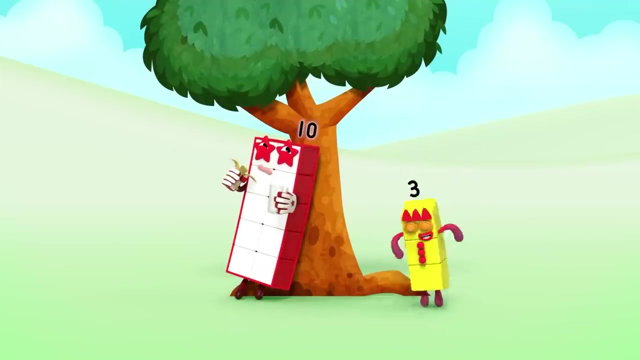 We're on a roll With ten on the pitch and one in goal. We will never be denied. We'll take it in our stride With ten and one, ten and one eleven on our side, Ten and one, Ten and one, eleven on our side, Bum-bum-bam. 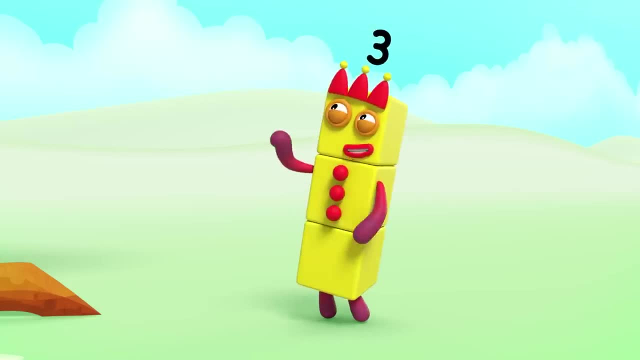 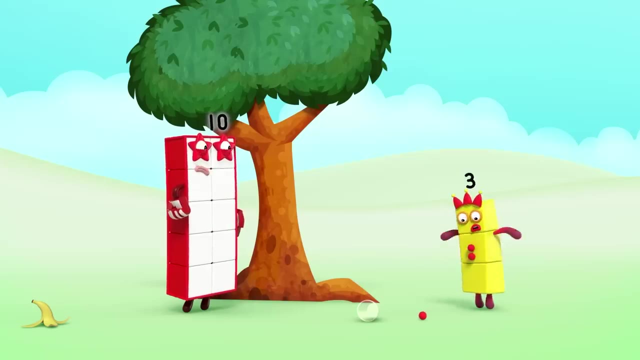 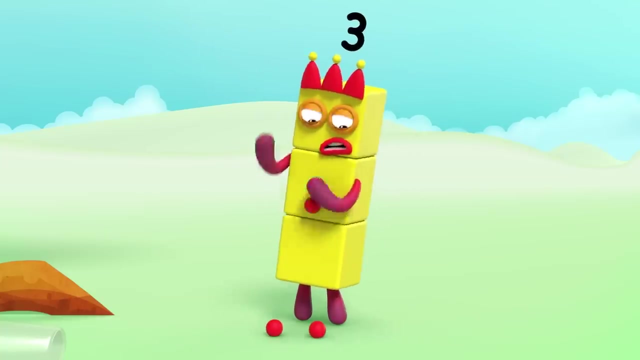 Three, Oh, sorry, Ten. I'm just so excited to show you my new trick. Look at this. Oh, Is that it? No wait, I'm not having much luck with my today. Oh no, My new trick. 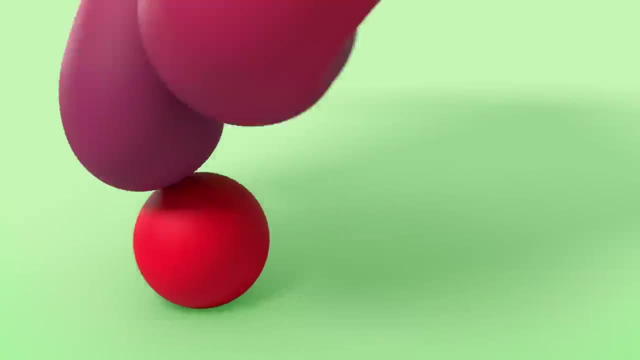 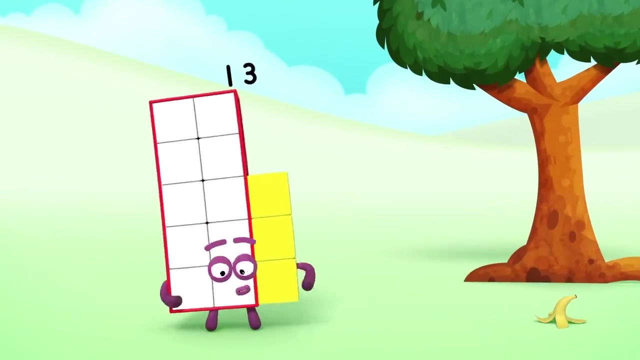 Ready, Ready, Goal, WHISTLE BLOWS, Yeah, WHISTLE BLOWS, WHISTLE BLOWS. Oh unlucky, Oh Hi, Who am I? I'm one, two, three, four, five, six, seven, eight, nine, ten, eleven, twelve, thirteen. 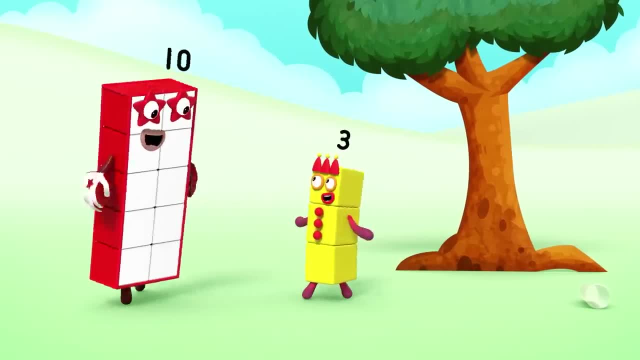 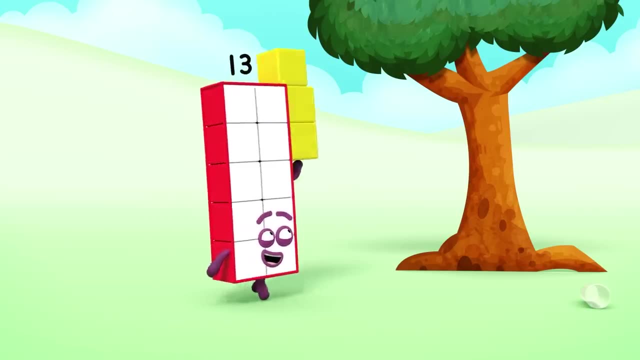 WHISTLE BLOWS, Whoa, WHISTLE BLOWS, Wow, WHISTLE BLOWS. Oh, my three fell off. Never mind, WHISTLE BLOWS, I am thirteen. WHISTLE BLOWS, Oh, whoa. 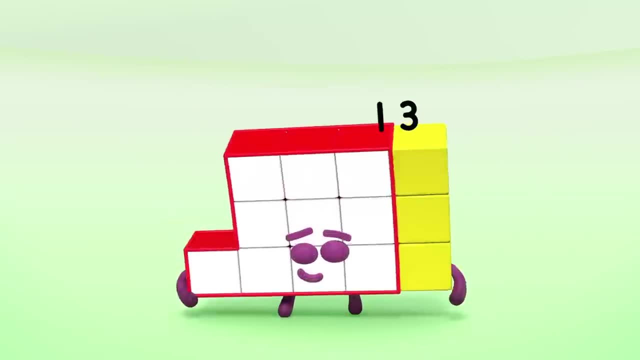 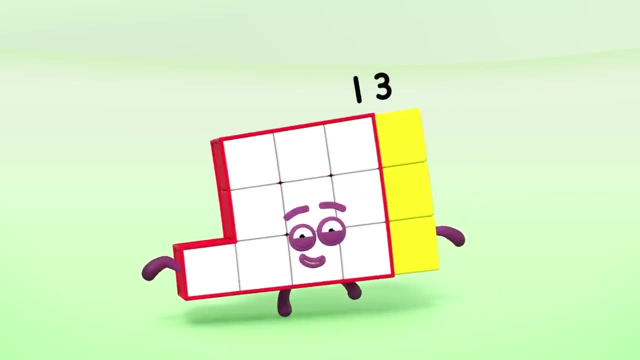 WHISTLE BLOWS, WHISTLE BLOWS, WHISTLE BLOWS. Oh, unlucky WHISTLE BLOWS. Try again. I am thirteen. WHISTLE BLOWS, Hooray, WHISTLE BLOWS. 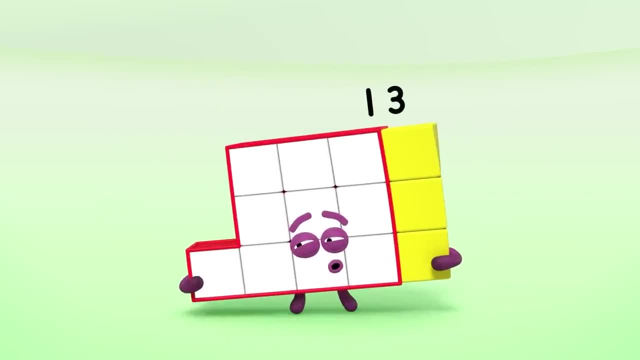 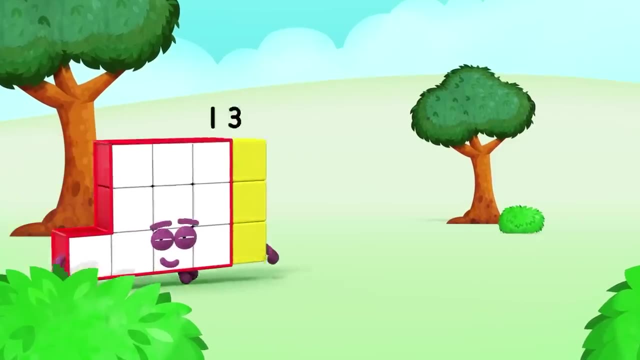 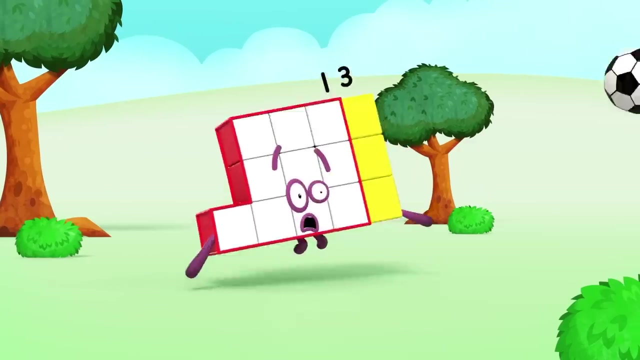 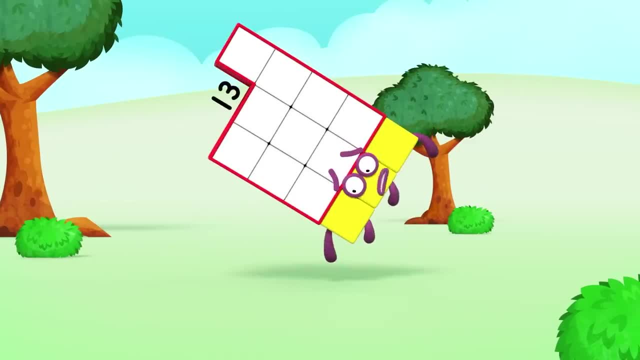 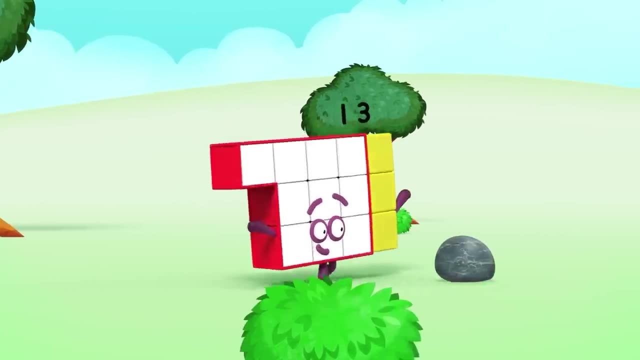 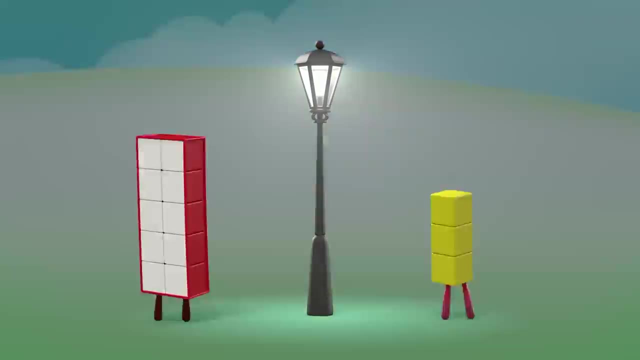 Sorry, It's all jolly japes. when I get into scrapes I'm always coming unstuck. Oh, I'm the clumsiest number you've ever seen. Unlucky number thirteen. WHISTLE BLOWS, It's happened again. a three and a ten. 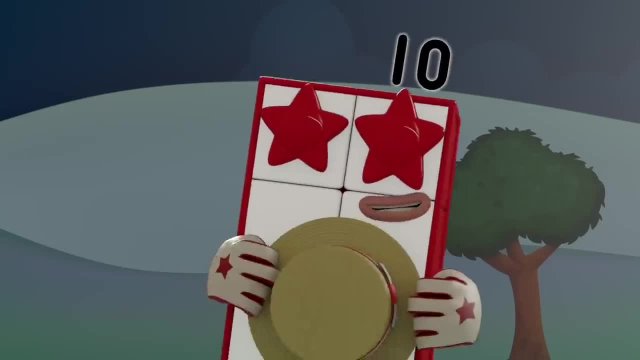 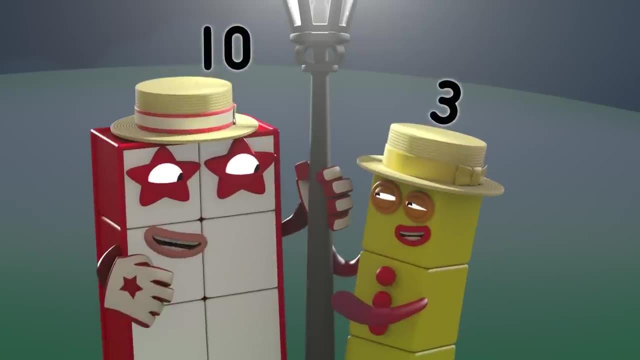 WHISTLE BLOWS, Tell him that it's happened again. I don't have the heart to be fussy or picky. Thought he'd fallen apart. He's a bit unsticky. WHISTLE BLOWS, It's happened again and no-one knows when. 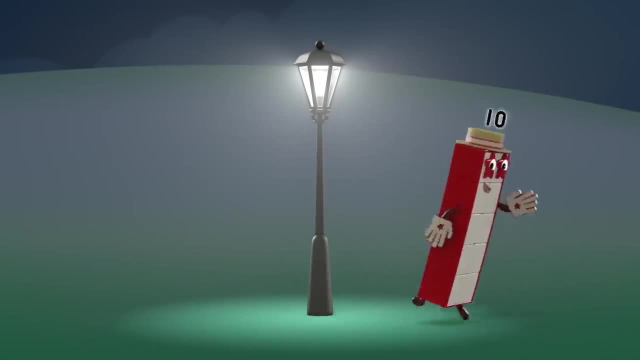 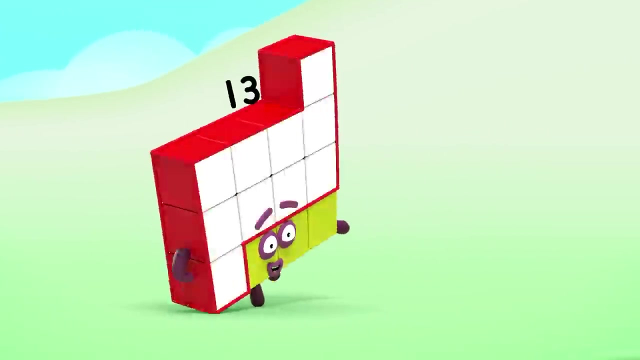 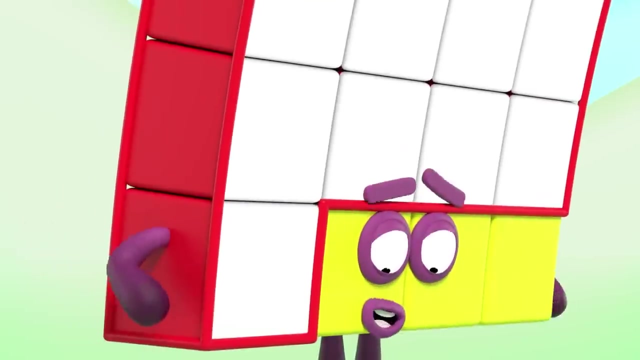 So far. we should tell him that it's happened again. WHISTLE BLOWS. WHISTLE BLOWS. Me again, three and ten expecting to fall down a hole- WHISTLE BLOWS. I jump through a hoop- WHISTLE BLOWS. 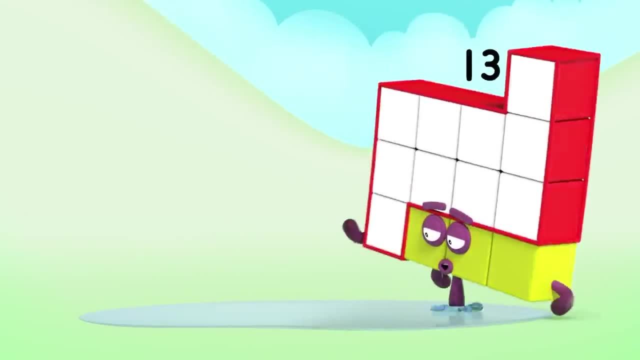 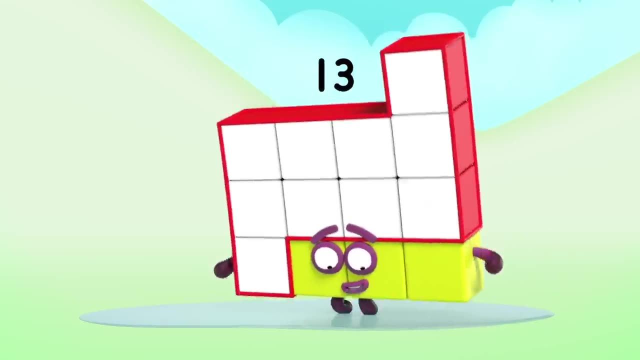 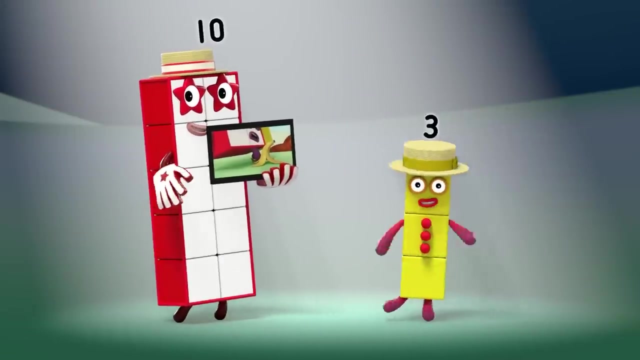 in a puddle that seems to sum up my row, And wherever I end up, I'm meant to slain Unlucky number thirteen. Oh whoa, It's always the same when he says his name. Somebody should tell him that's the name of the game. 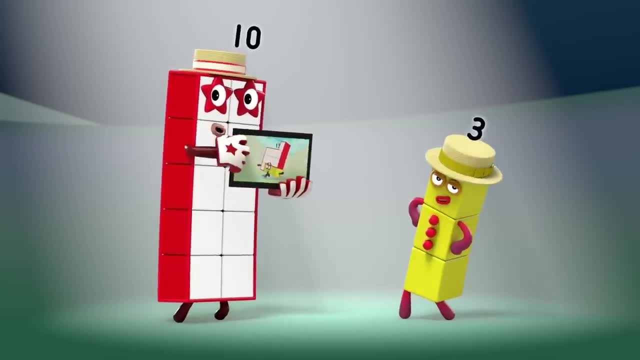 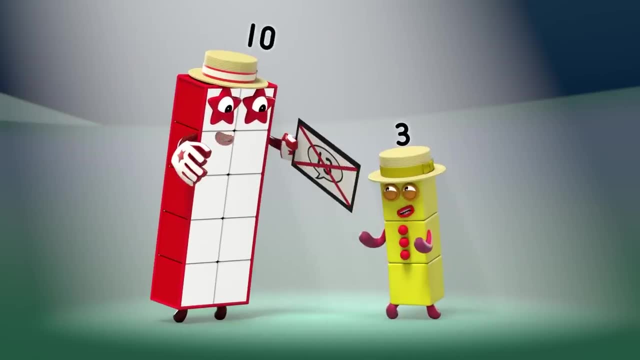 It's happened before a total disaster, but he's going to need more than a sticking cluster. It's always the same. we know what to blame. Somebody should tell him not to mention his name: WHISTLE BLOWS. WHISTLE BLOWS. 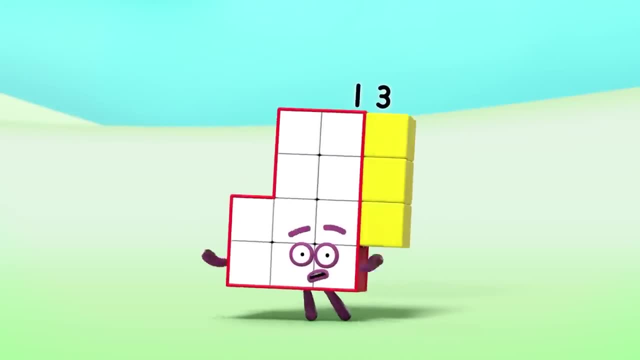 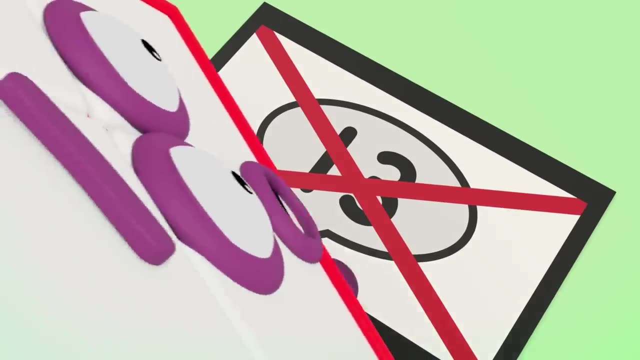 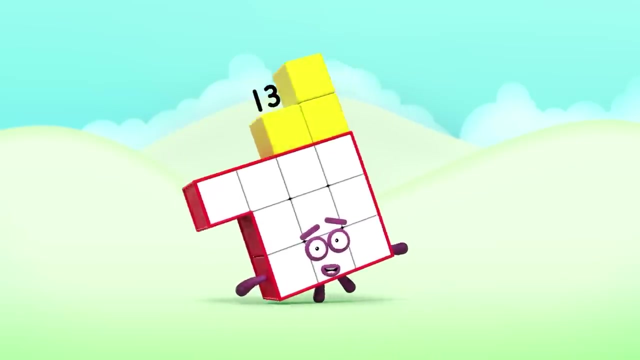 It's getting routine. I say I'm thirteen, Keep it together. this is absurd. You know what I mean. I say it's thirteen, End of my tether. don't say that word. It's always the same. it's getting routine. 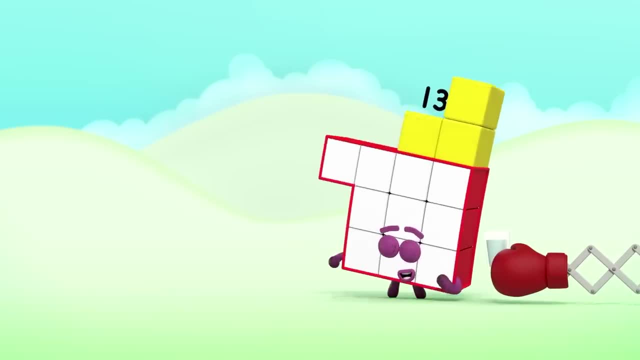 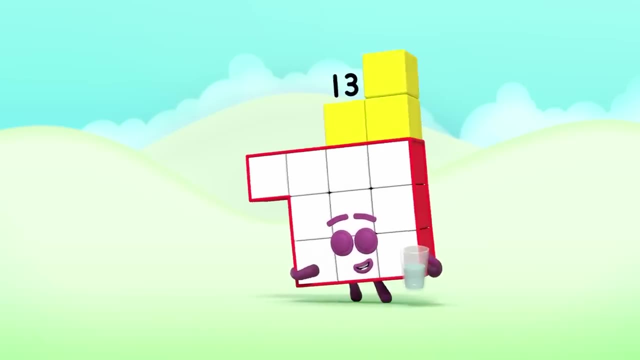 They ask me my name, I say I'm fir, WHISTLE BLOWS Thirsty. I say I'm thirsty, WHISTLE BLOWS. They ask me my number. you know what I mean And I always say it's a. 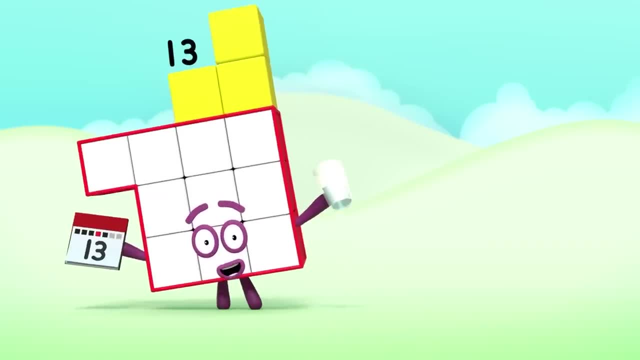 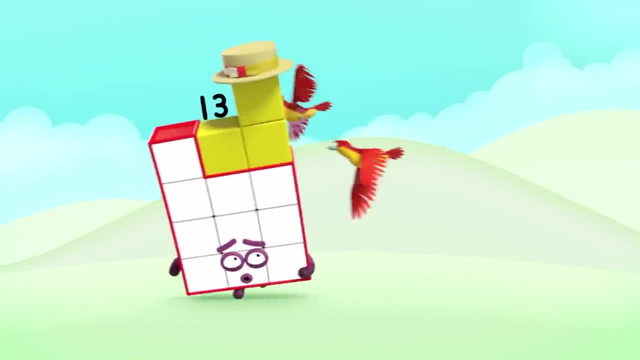 Thursday. I always say it's Thursday, Andy's jacking, it's their time. WHISTLE BLOWS. This is me. ten and three turning this into a game. I'm changing my luck. I won't come unstuck. 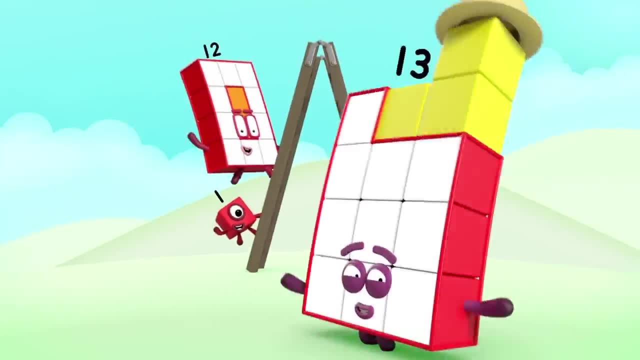 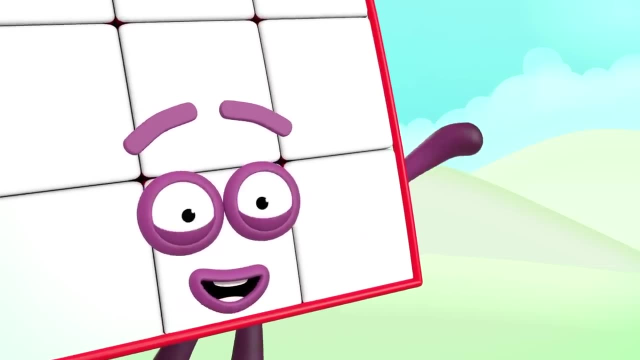 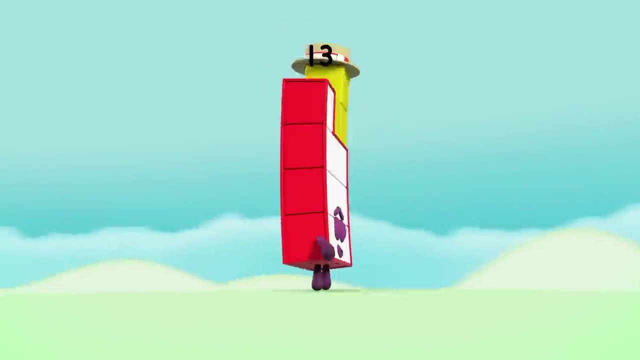 as long as they don't say my name, WHISTLE BLOWS Ten and twelve, or ten and three, whatever you call me, I'm still me. I'm the happiest number you've ever seen. So lucky to be unlucky. 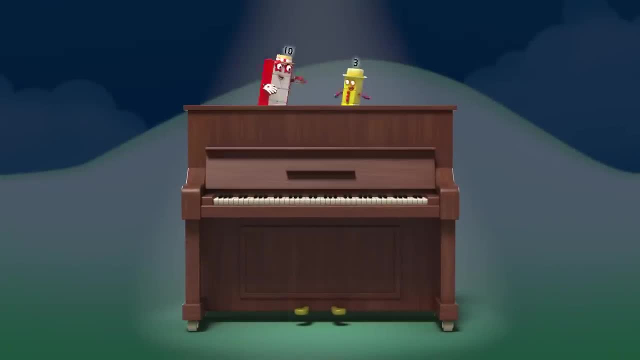 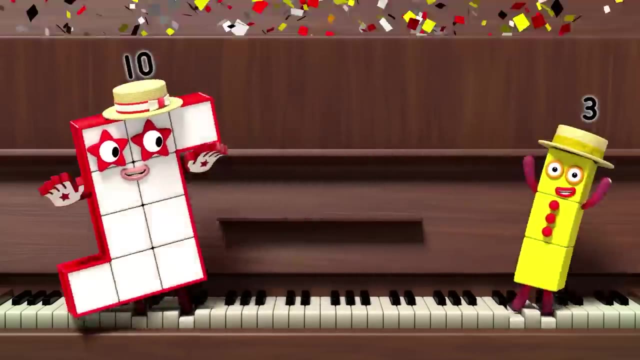 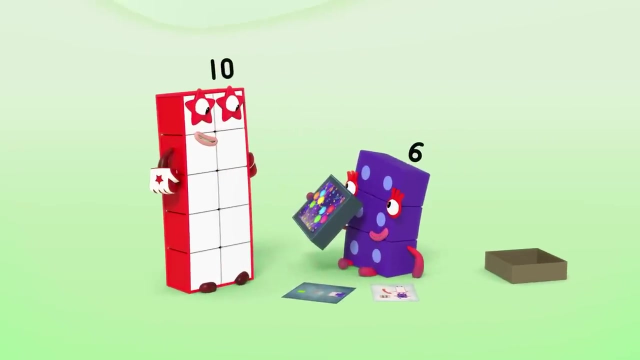 Number thirteen: WHISTLE BLOWS. Thirteen, Thirteen, Thirteen, Thirteen, Thirteen, Thirteen. Unlucky me, I'm going to play my new game. It's called Party in a Box. Ooh. 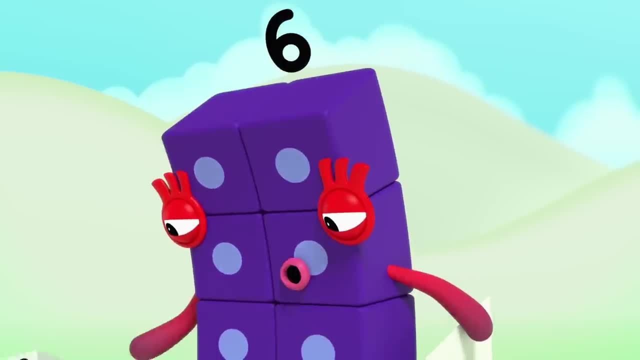 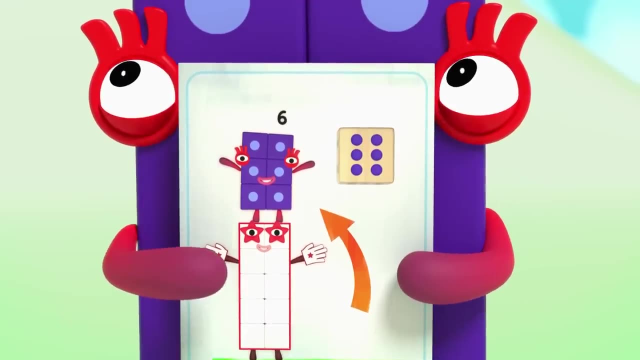 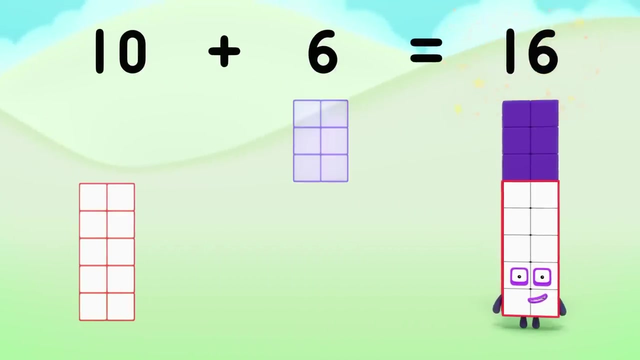 First roll the dice. Let's roll: WHISTLE BLOWS Six. If you roll a six, jump on your friend's shoulders. Hmm, WHISTLE BLOWS. Ten plus six equals Sixteen. WHISTLE BLOWS. 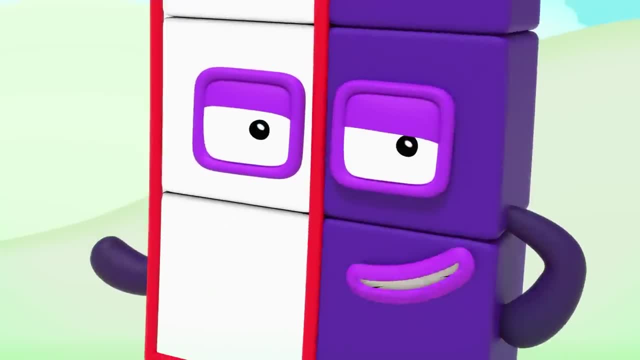 Oh, look, And then. well, that's nice, isn't it? Right, then let's get on with it. see what shapes I can make. Yeah, WHISTLE BLOWS, Hmm, WHISTLE BLOWS, Ooh. 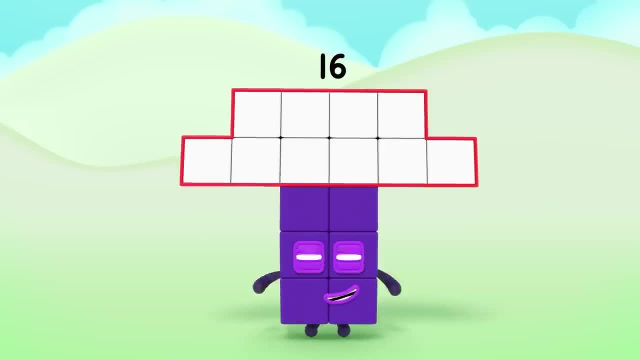 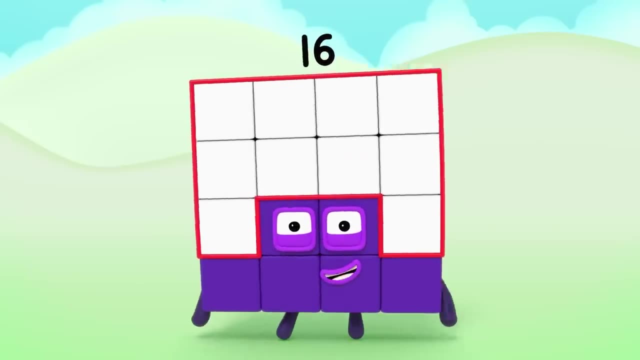 WHISTLE BLOWS, Erm, WHISTLE BLOWS, Aha, WHISTLE BLOWS. Oh Oh No, No way, I can't believe it. I'm so excited. Guess what? I am sixteen. 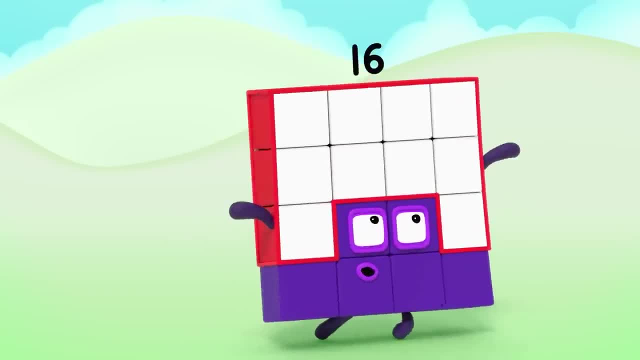 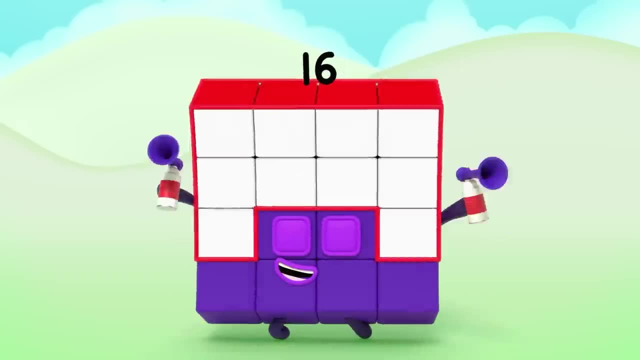 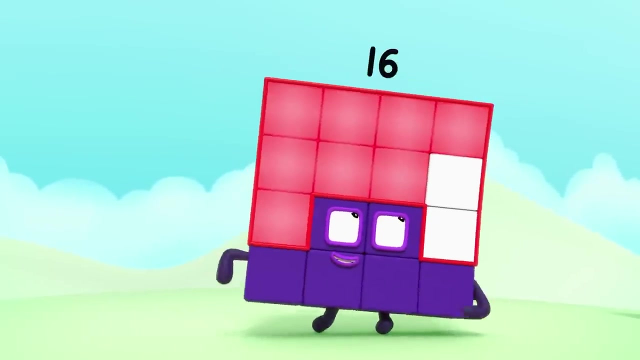 And I am a square, Woo-hoo. Right then, what do squares do? I bet it's really amazing. Wait, no, let me guess. I know. Square party WHISTLE BLOWS One, two, three, four, five, six, seven, eight, nine, ten, eleven, twelve, thirty, forty, fifteen, sixteen. 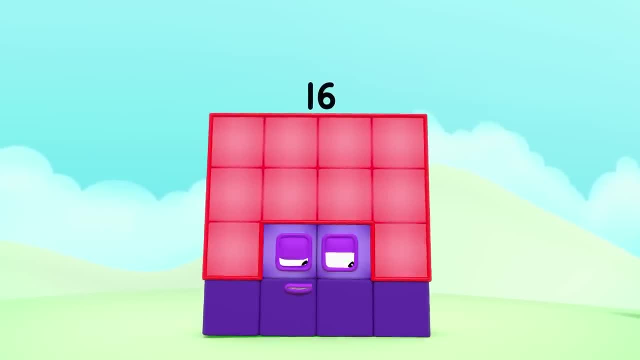 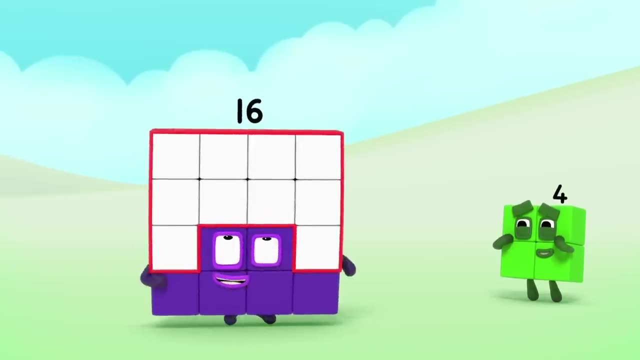 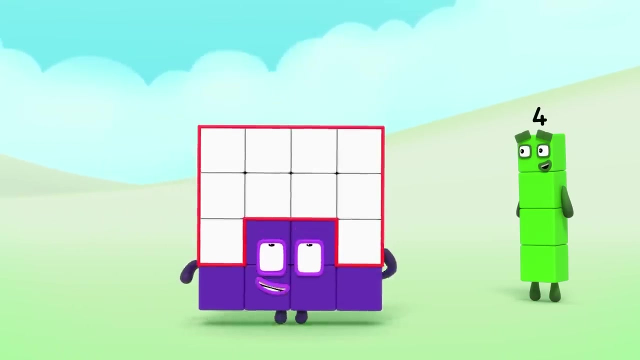 I am sixteen square as a box and guess what? I've got sixteen blocks Square, Really big square. Sixteen WHISTLE BLOWS, Ten and six WHISTLE BLOWS. I like this game. Sixteen. 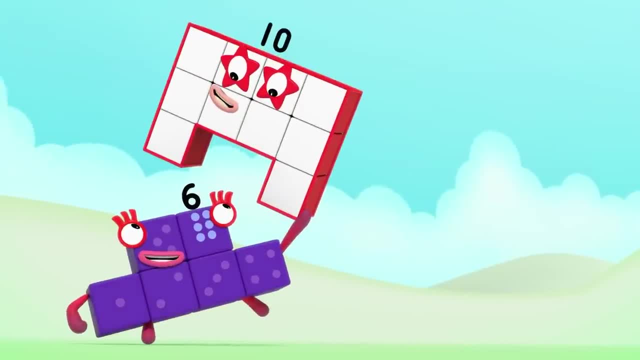 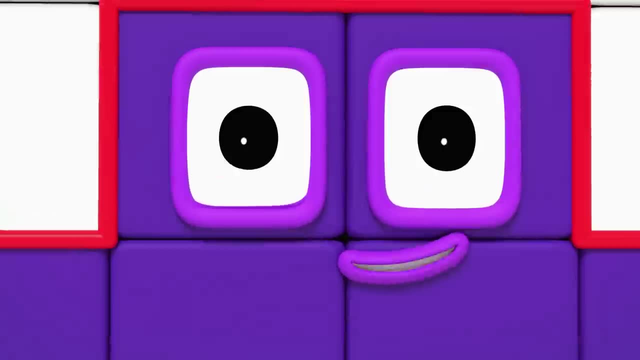 Ten and six. WHISTLE BLOWS, Party Sixteen, I am sixteen, I'm ten and six And I've got loads of party tricks. Lie down, Stand up, Lie down, stand up, Lie down, stand up. 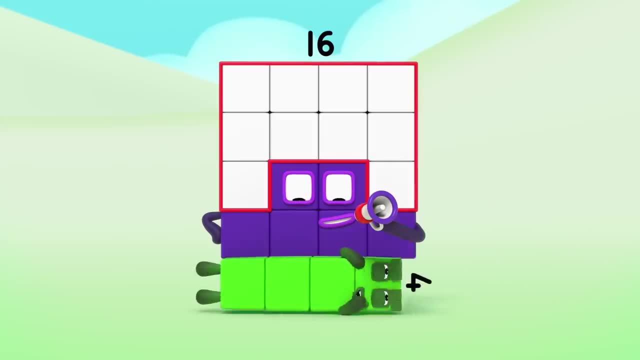 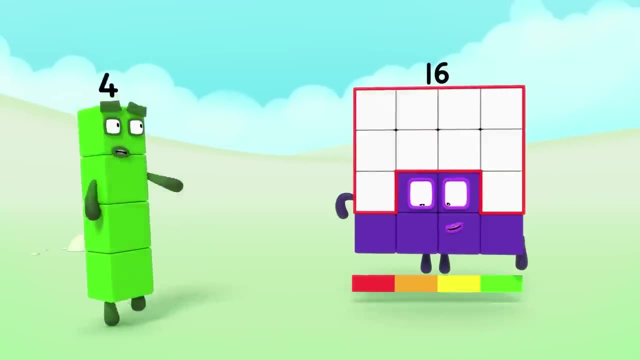 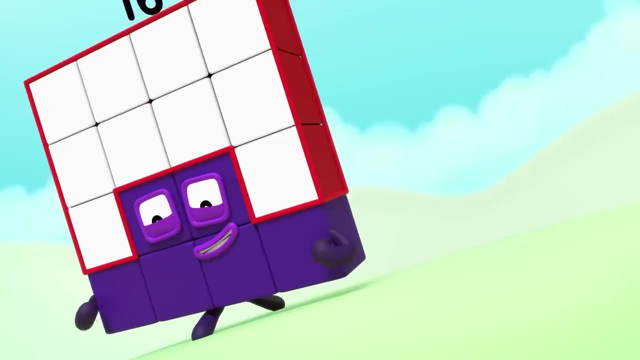 Keep going. Four by four, four by four, four by four. I am a square, Are you sure? Of course I am. I'm four by four. Sixteen. WHISTLE BLOWS, WHISTLE BLOWS, WHISTLE BLOWS. 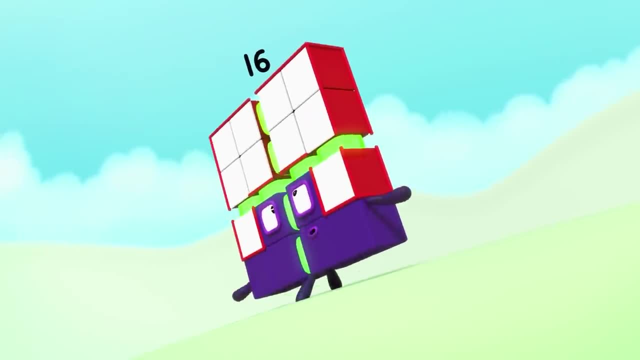 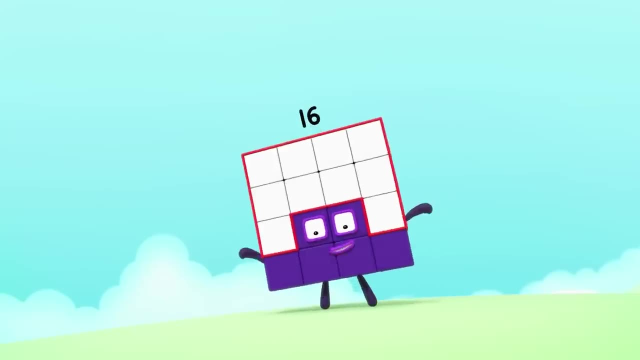 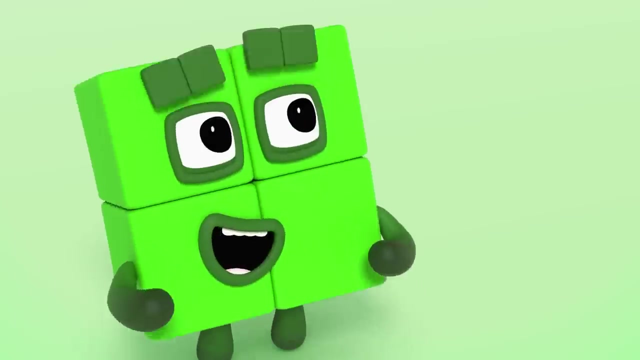 I have four columns and four rows, Four out of the four. I'm four of those. A square made of squares, I can do the splits. Four fours. WHISTLE BLOWS Four fours. WHISTLE BLOWS Four fours. 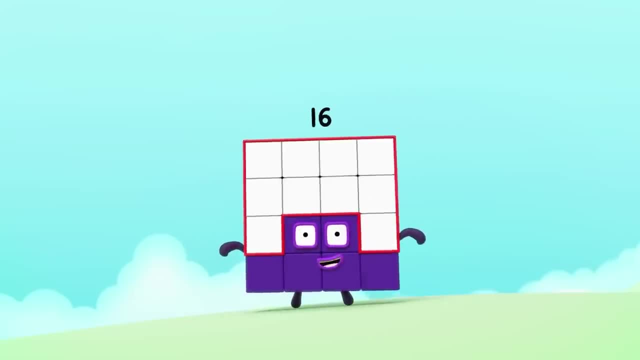 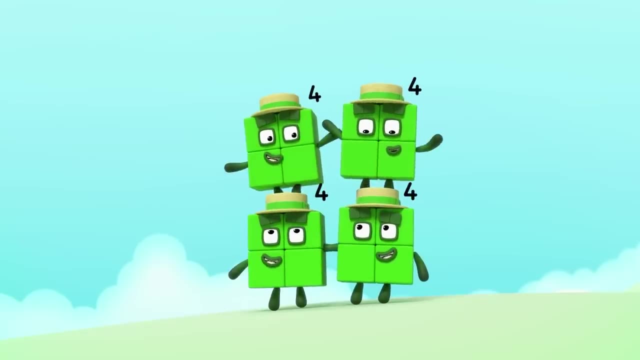 WHISTLE BLOWS, Sixteen Still here. One, two, three, four, four fours. One, two, three, four, four fours. One, two, three, four, four fours. You know what four fours are? 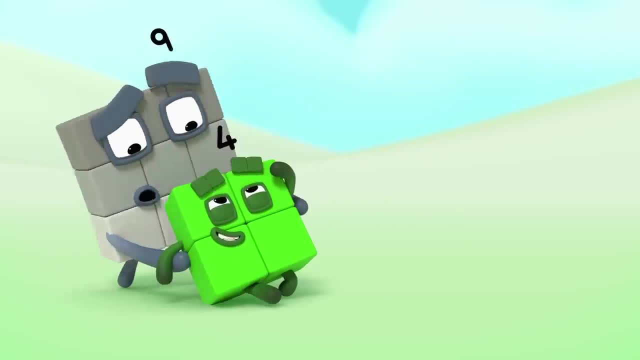 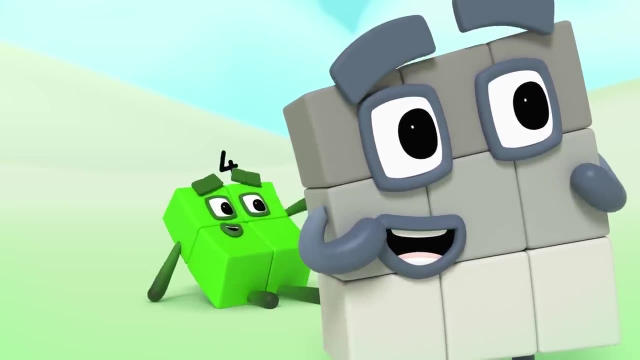 Sixteen, WHISTLE BLOWS. Oh, um, it's all right. four: It's only a really big square. Wow, WHISTLE BLOWS. I am sixteen. I'm four by four. I'm larger than a dinosaur. 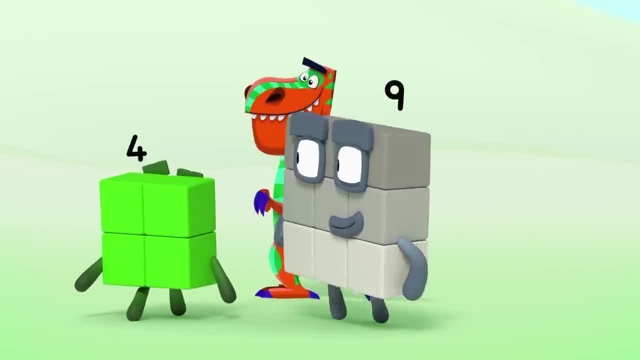 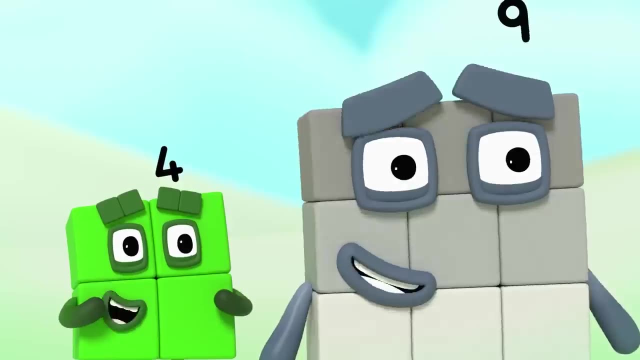 WHISTLE BLOWS Whoa, Whoa Later. Zaraxi, I am sixteen, I mean no trouble, But have you seen me? Ah, the devil No Alone. WHISTLE BLOWS Sixteen. 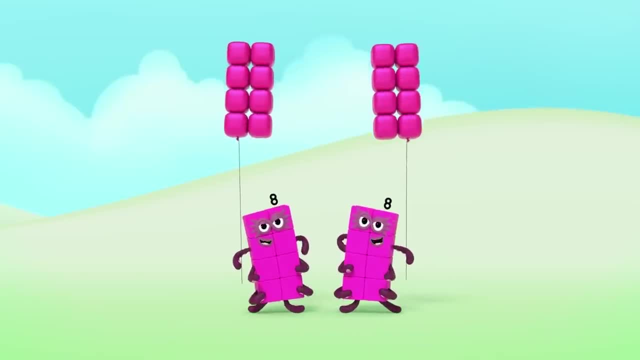 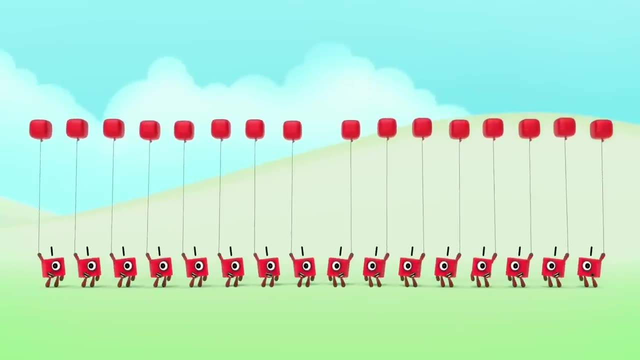 I'm going to split in half now Two. eights. We're going to split in half now Four, fours. We're going to split in half now Eight, twos. We're going to split in half now Sixteen ones. 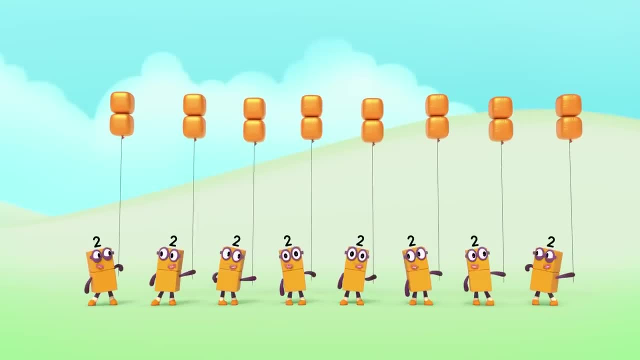 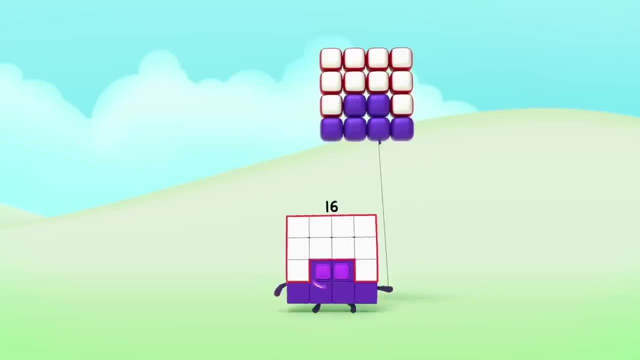 Hooray. We're going to double up now Eight. twos, We're going to double up now Four, fours. We're going to double up now Two. eights, We're going to double up now Sixteen. I'm going to. 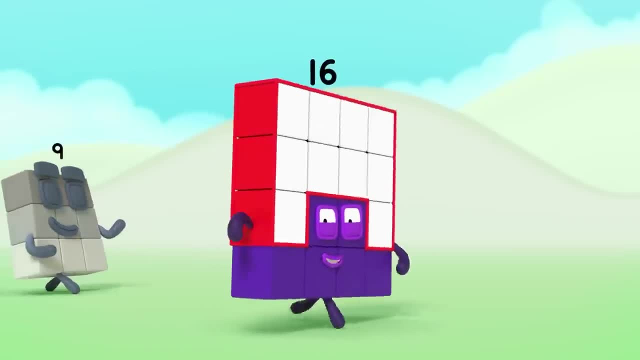 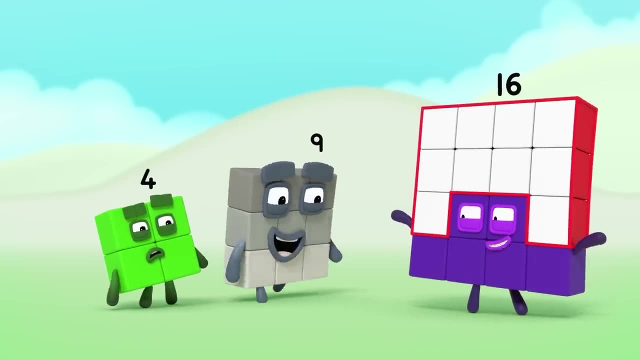 Ow, it's me silly, WHISTLE BLOWS, Do, do, de, do, Do, de, do, Do, do, de do. Oh Well, come on then. Hmm, Square dance, Square dance, WHISTLE BLOWS. 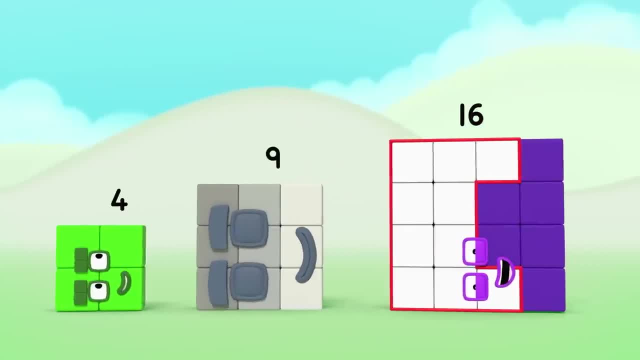 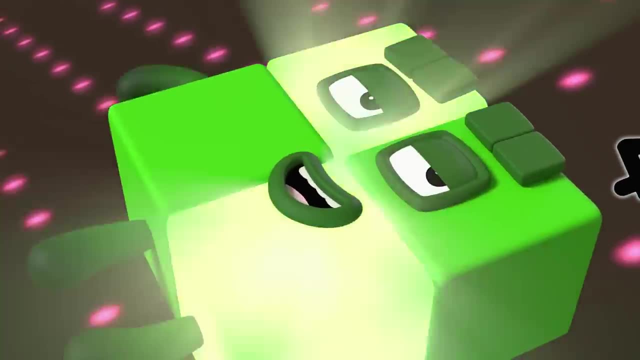 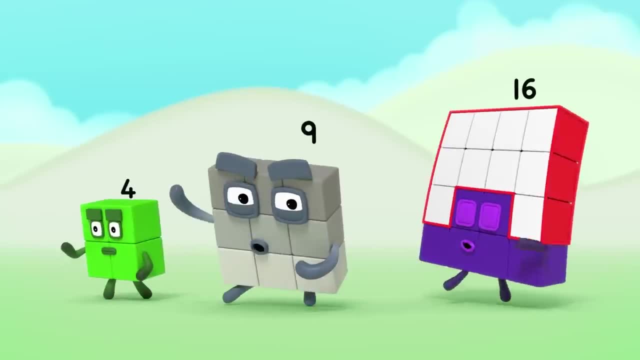 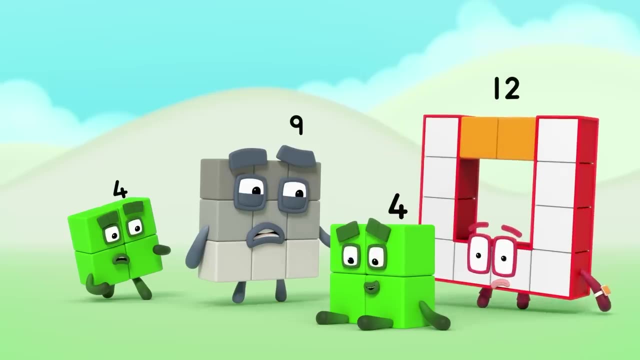 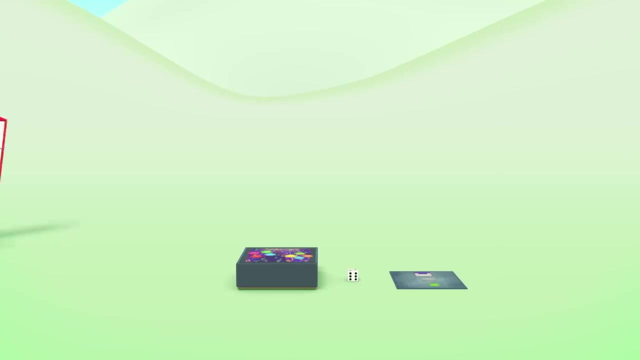 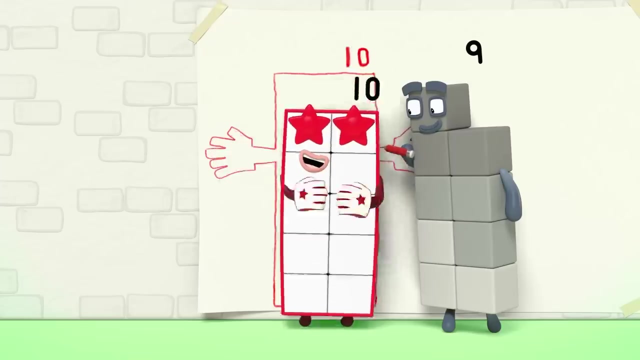 I am the square Freestyle Gennady. Huh, Huh, Huh, Ah. Square party, Square party, Square. Ooh Ta-da, I love it. Your turn, Super Rectangle, Ha-ha. 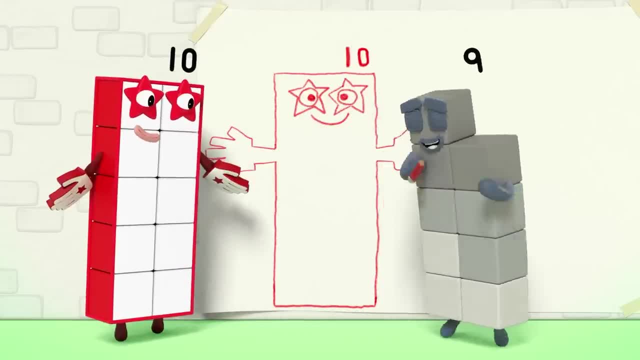 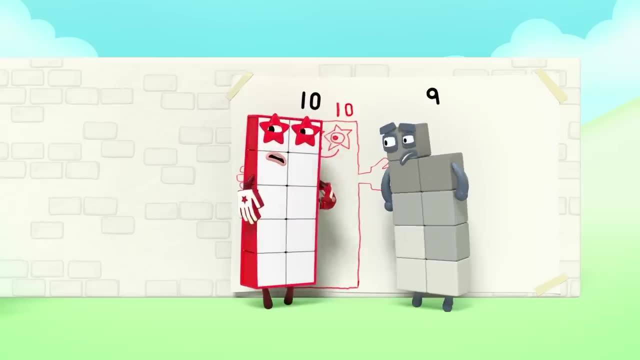 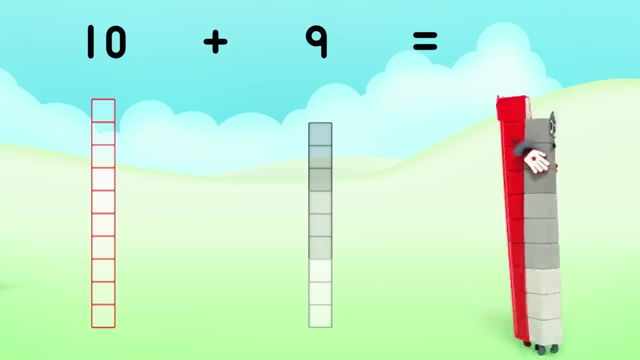 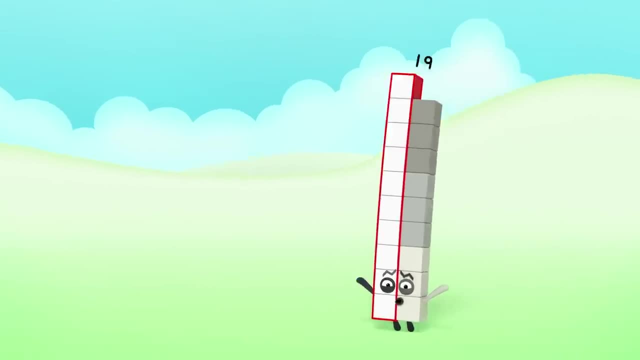 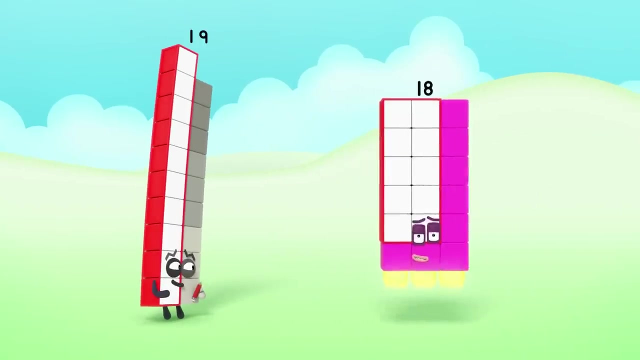 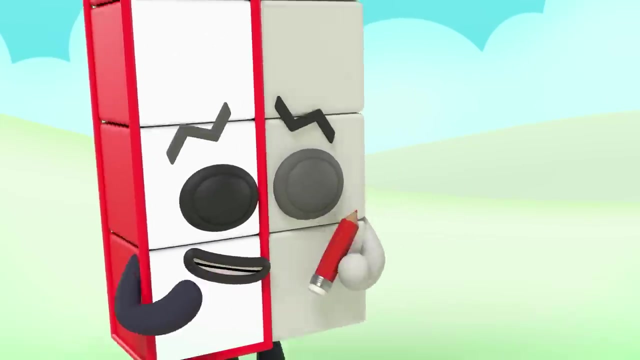 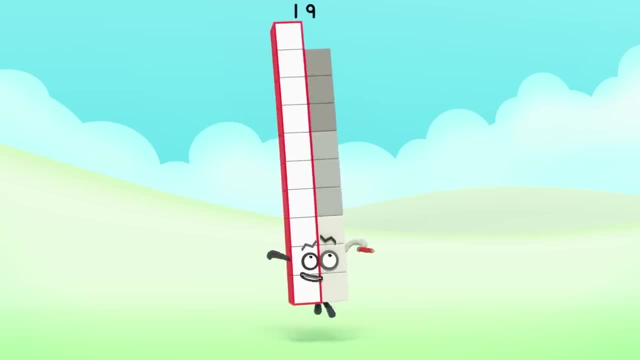 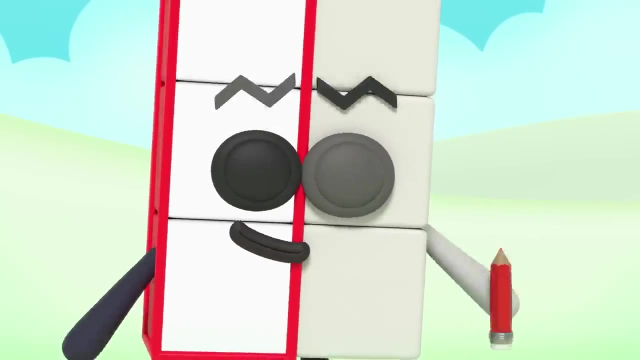 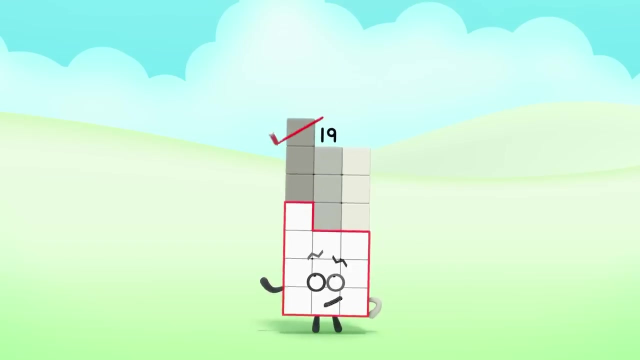 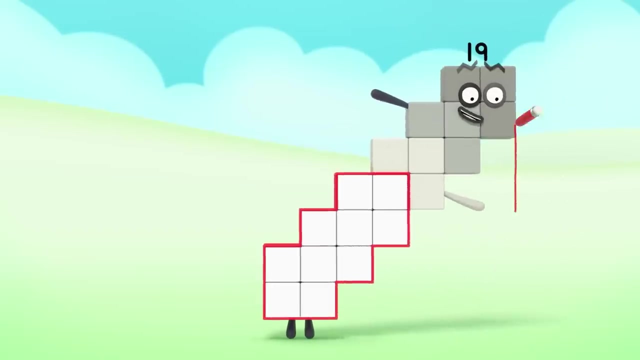 Right, let's do this. Two by Oh, Oh, silly me. One block missing, Try again. Three by One, block too many, Never mind. Four by One. off again, You can do this. Oops, Not a rectangle. 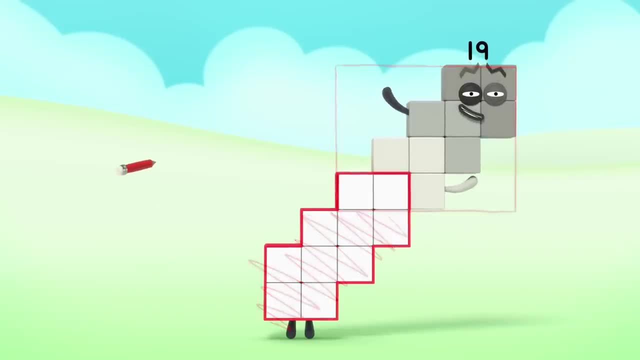 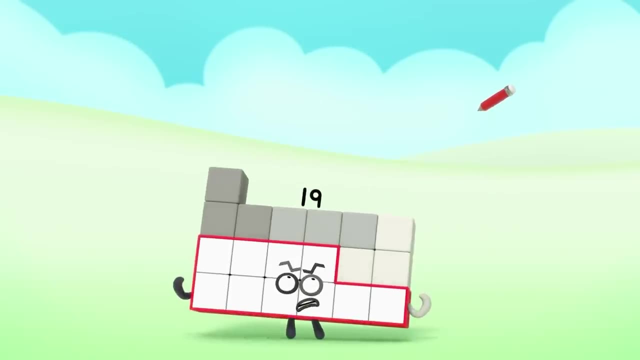 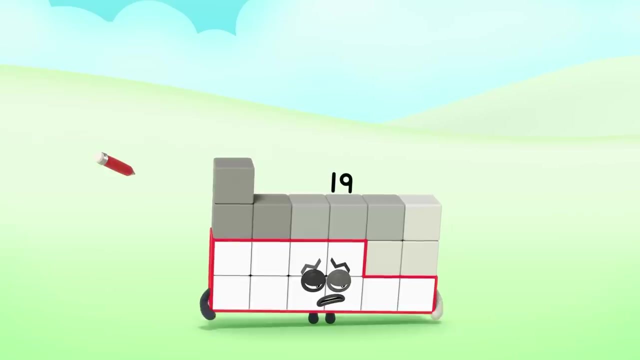 Come on 19. Concentrate: Five by No One off, Six by One off. Oh, I can't do it. I'll never be a super rectangle, I'm just a silly old Teapot, I mean. 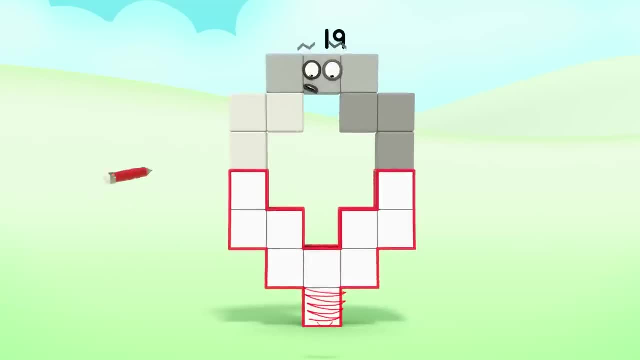 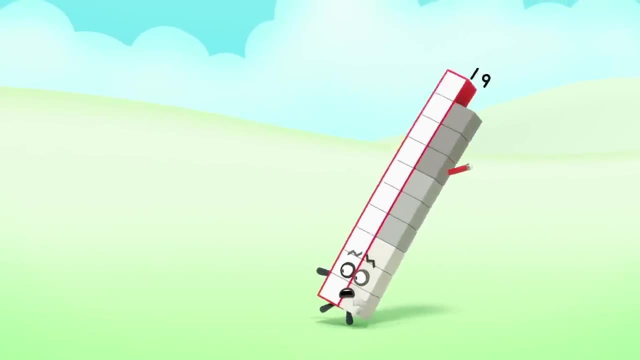 Elephant, I mean Like, I mean Monster, Super Rectangles. I wish I could be like 18.. Make everyday shapes with neat, straight lines, But there's always something not quite right, So I make crazy shapes. That's where 19 shines. 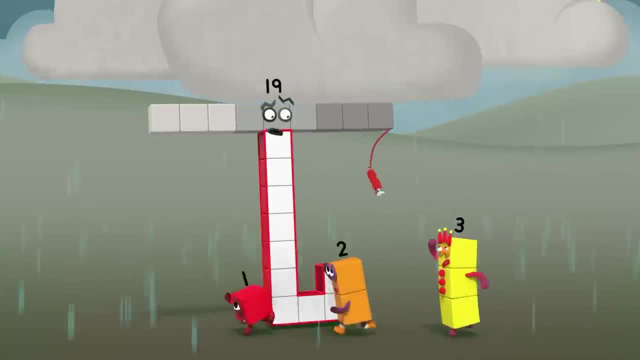 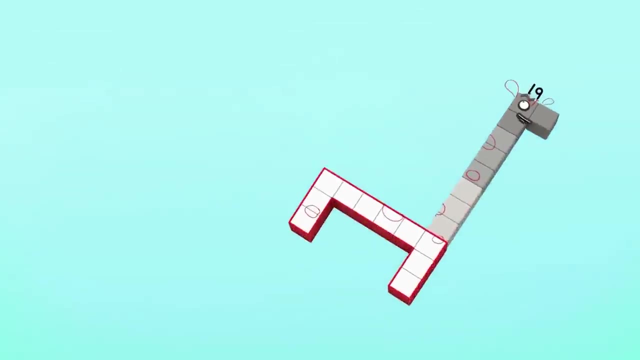 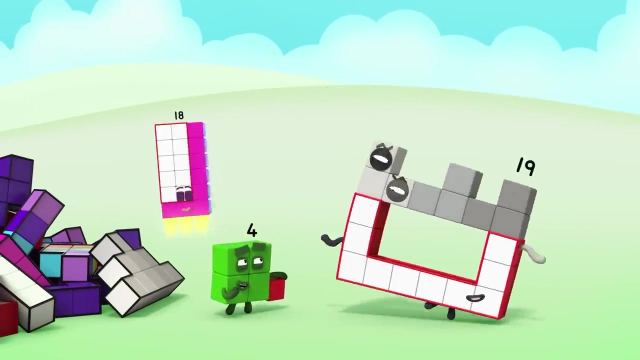 I can be a cactus in the desert, An umbrella when it rains, Oh. I can stretch right out to make a tall giraffe, Oh thanks. And if you need some building blocks, I can make a crane. Then make lots of funny faces to make you laugh. 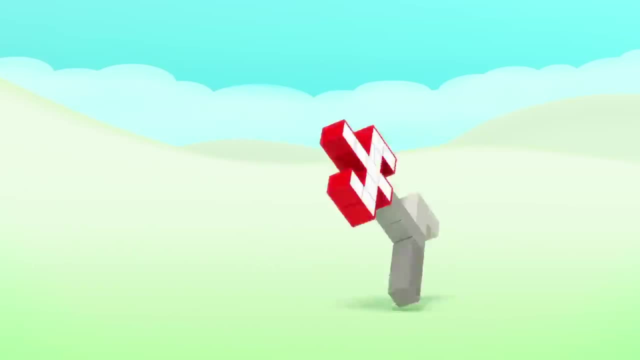 Because I make crazy shapes. Crazy shapes are what I do: Thingamabobs and what's-its, and whatchamacallits too. I can make most anything. So put me to the test: Crazy shapes. Crazy shapes are the thing that I do best. 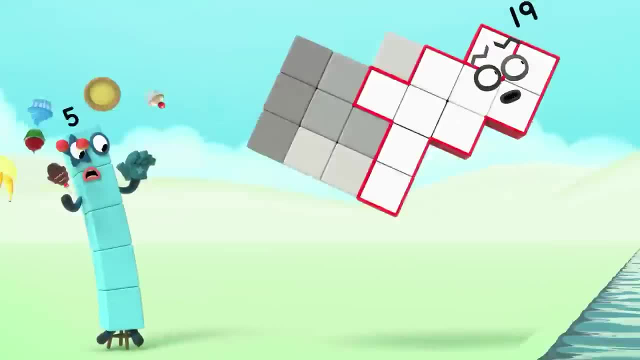 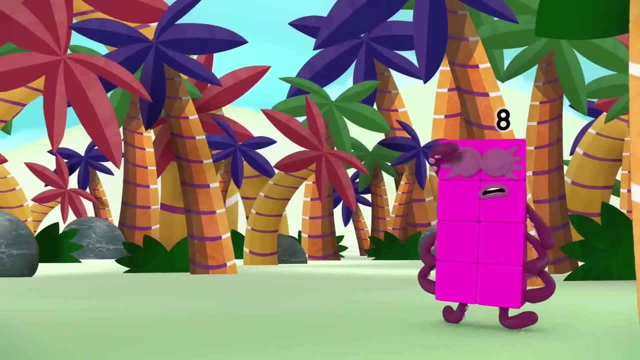 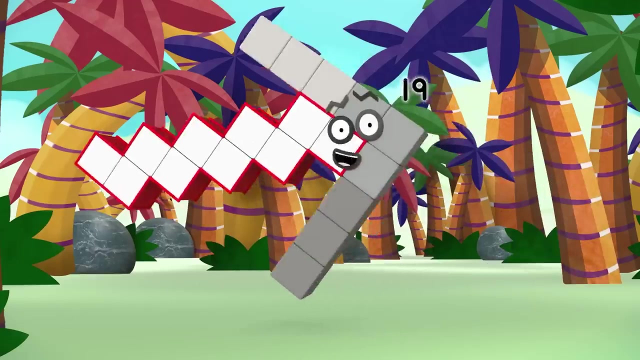 I can make a table you can eat at, Or a funny kind of fish When you're digging. I can make a garden spade. When you're lost, I'll give directions With an arrow if you wish. When it comes to making wacky shapes, I've got it made. 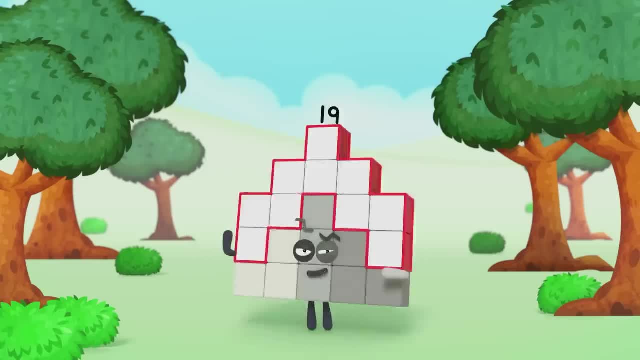 Because I make crazy shapes. Crazy shapes are what I do: Thingamabobs and what's-its, and whatchamacallits too. I can make most anything. So put me to the test: Crazy shapes. Crazy shapes are the thing that I do best. 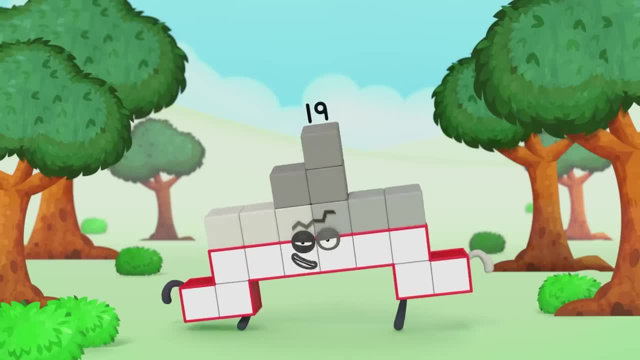 Oops, I'm a one-off. I'm unique, As I'm sure that you'll agree. I'm a one-off. I'm at my peak. No one's better at being me than me. Come on, Come on, Come on. 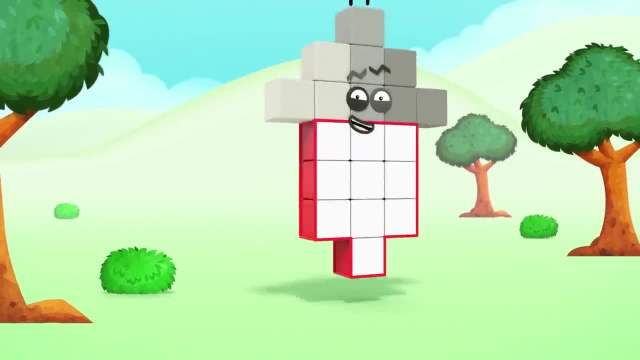 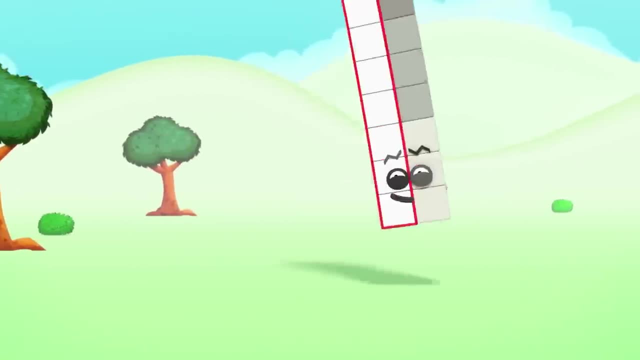 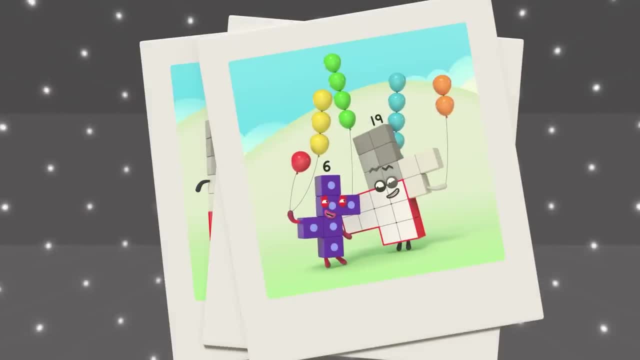 Throw some shapes with me, Cause I make crazy shapes. Crazy shapes are what I do: Thingamabobs and what's-its, and whatchamacallits too. I can make most anything. So put me to the test, Crazy shapes. 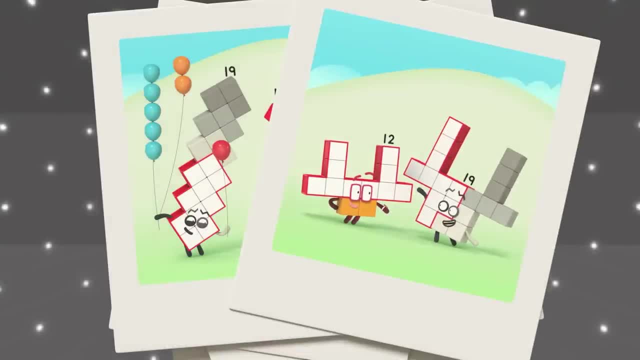 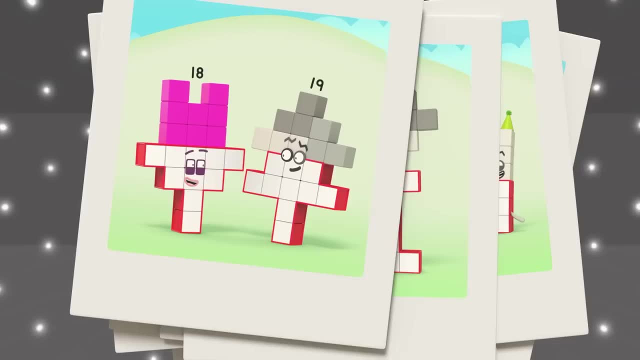 Crazy shapes are the thing that I do best. Crazy shapes, Crazy shapes are the thing that I do best. I am nineteen. I am grated. I'm green, I'm blue, I'm orange, I am green, I am purple. 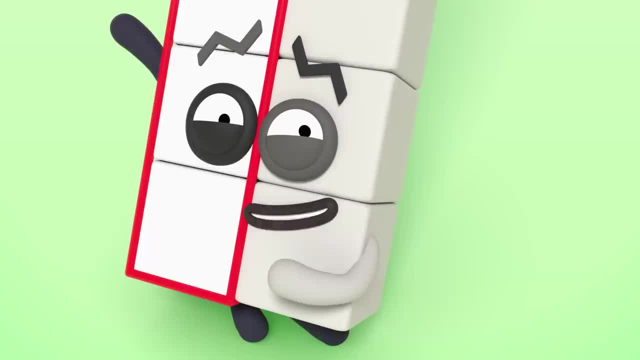 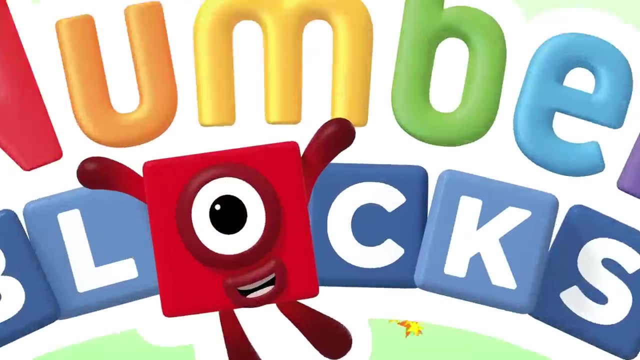 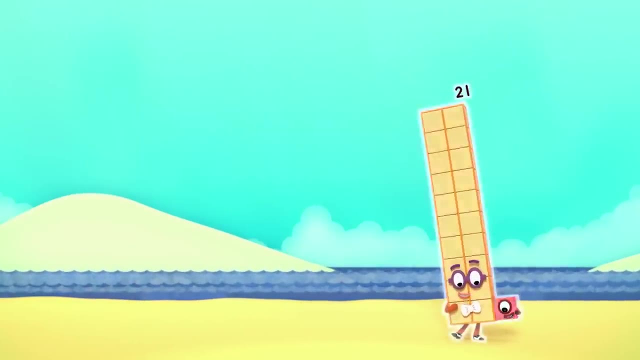 I am blue, I am blue, I am pink, I am red, I am pink, I am white, I am purple And I am a one-off And I love it. 20 plus 1 equals 21.. I'm 21.. 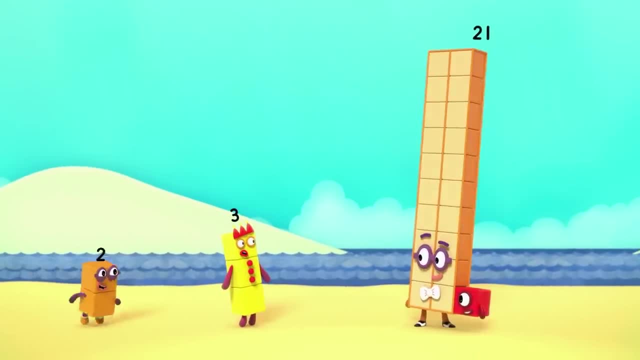 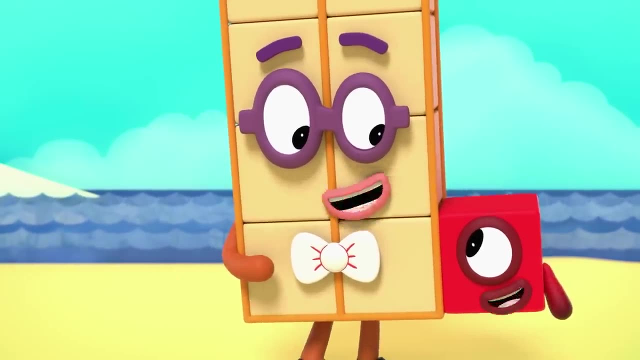 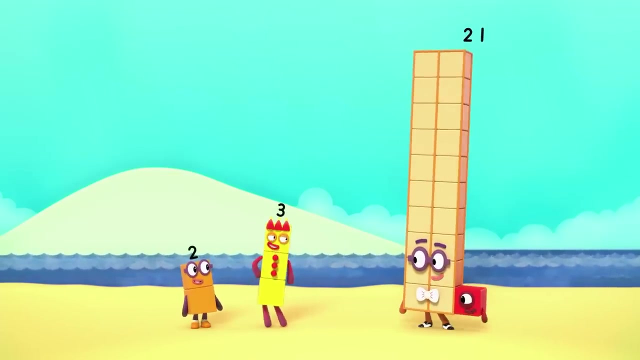 I'm 20. And 1. You're 21. You've got two faces. Sometimes it's easier to think of bigger numbers as two numbers together: 21. 20 and 1.. Oh, I see I wonder who else I can be. 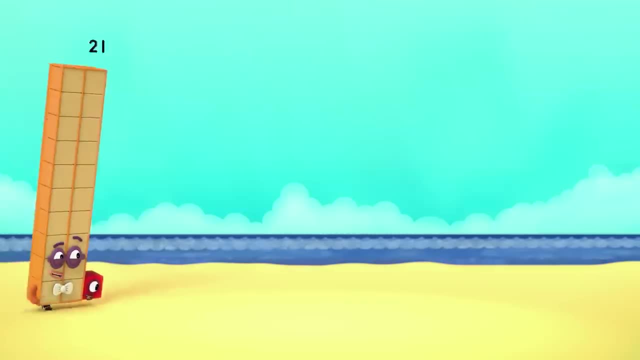 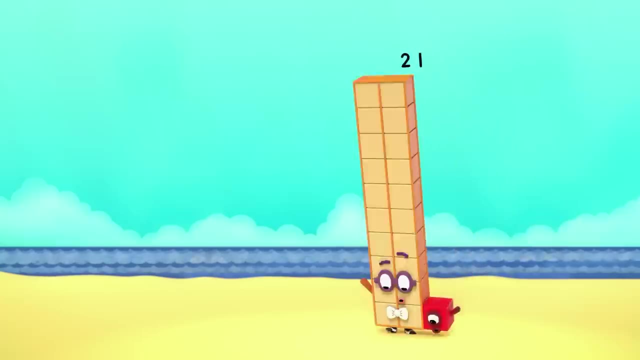 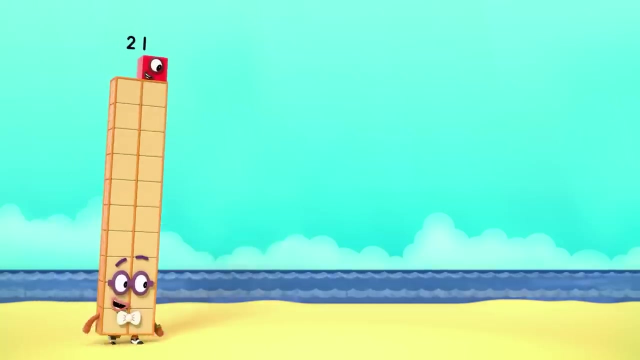 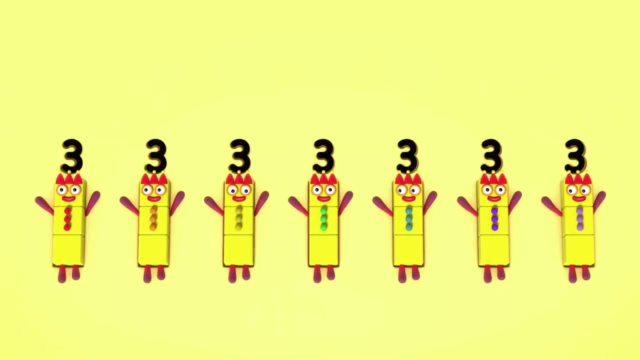 That's me 21.. I'm two tens and 1-1.. Two blocks wide leaves an odd block on top. I'm an odd number And if I do this, I can be Seven threes, Which means I'm also. 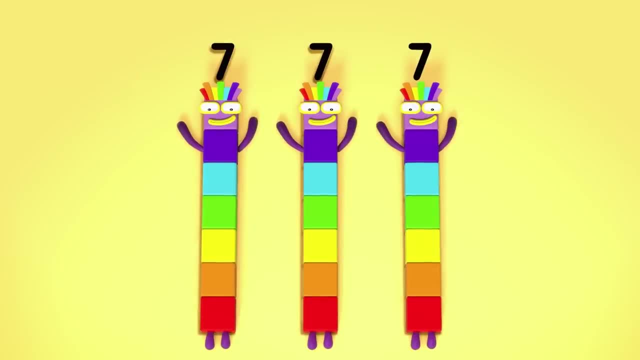 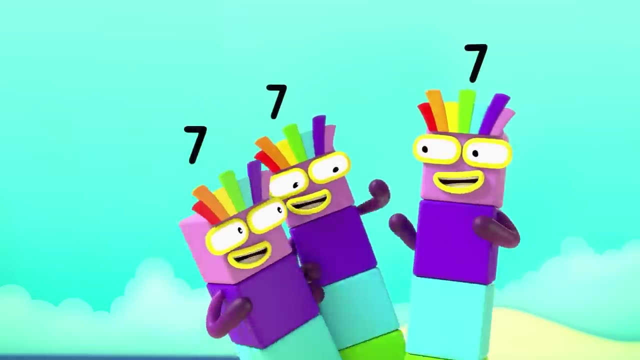 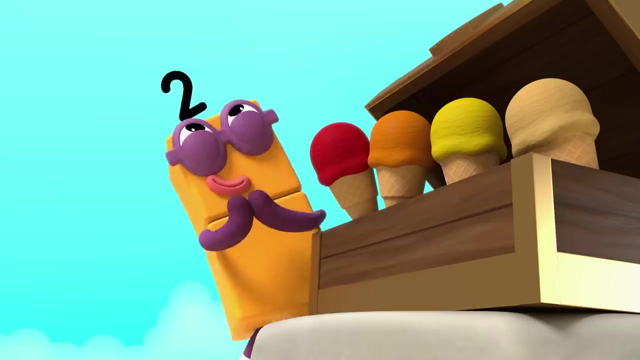 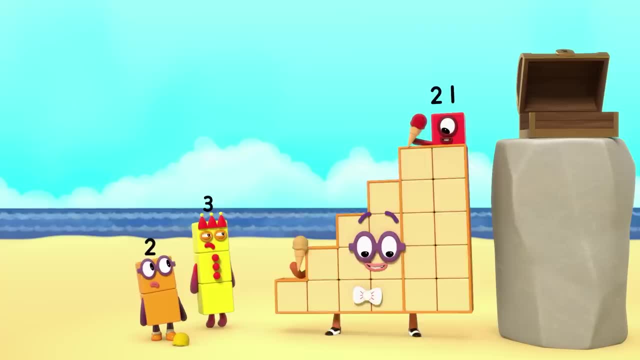 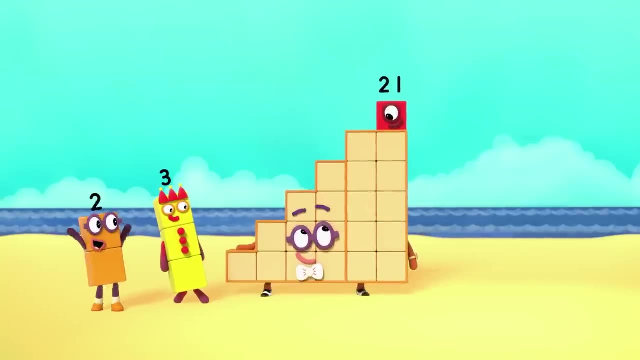 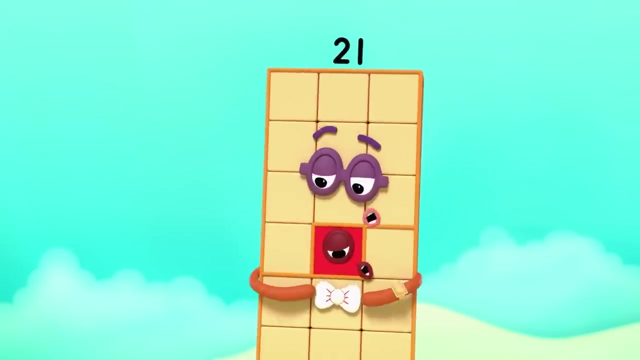 Hmm, Hmm, Hmm, Hmm, Hmm. Hey, wait, I'm a step shape. That means I can be a Step squad, Ready for action. Wow, We found out so much about you 21. And I found out that I love finding things out. 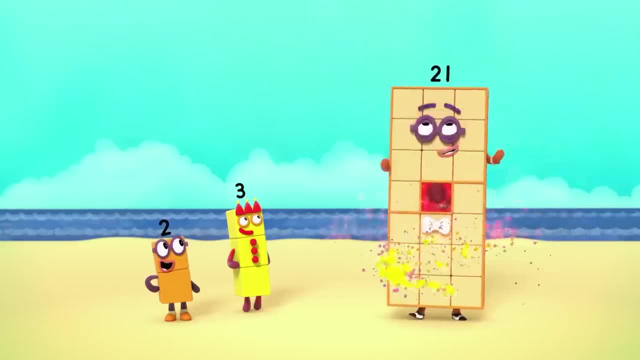 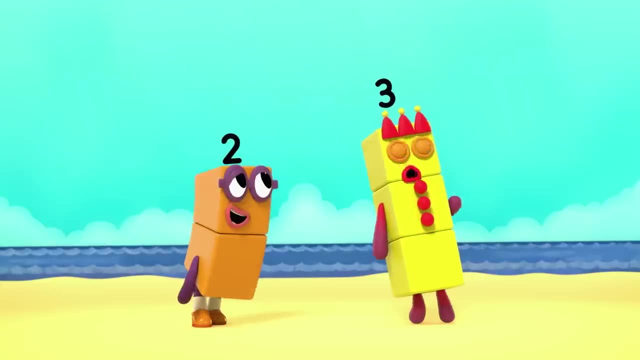 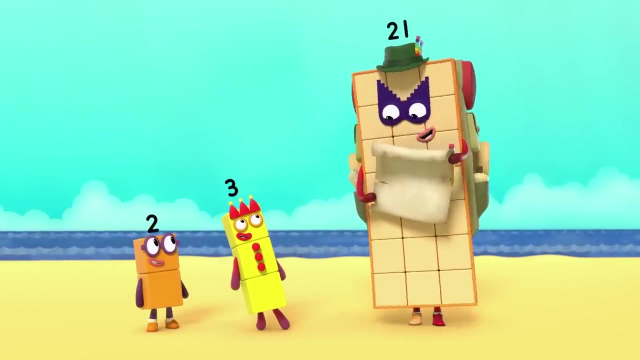 I figured myself out: I am 21. And I'm a number explorer. Wow, The quest, The question is: what comes next? There's always more to explore. We'll need a magic mirror. Oh, there's one, Triple lucky. 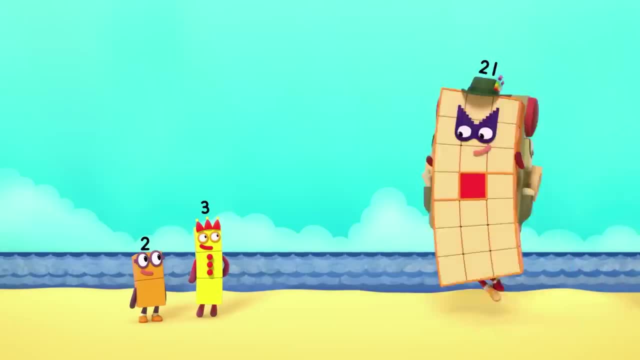 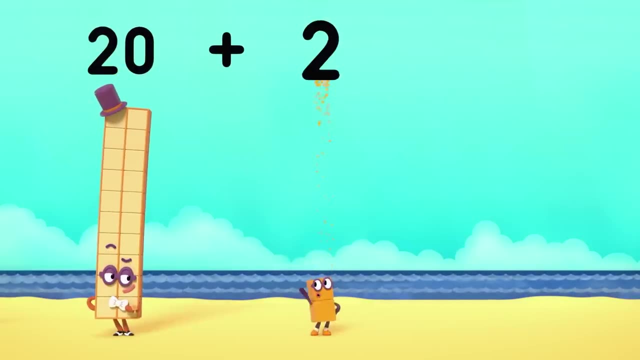 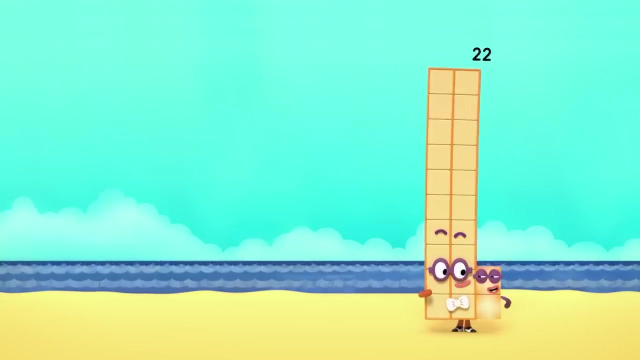 Hello me, Ready to And go. 20 plus 2 equals 22!. I'm 22.. I'm 22.. I'm 20. And 2. Oh Excellent, Let's find out what you can do. 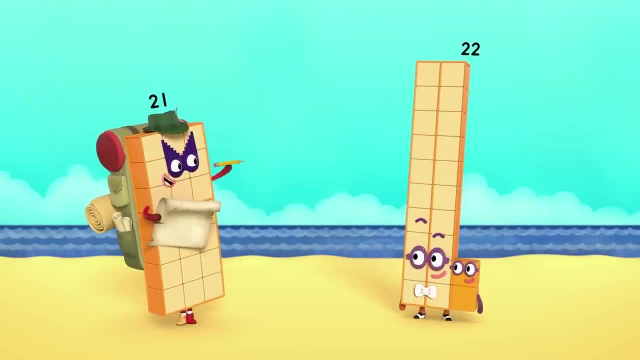 You're 22 blocks, which is 2 tens and 2 blocks more. Let's try the 2 on top. Ah, you're an even number, which means you're a double. Try splitting down the middle: I'm double 11.. 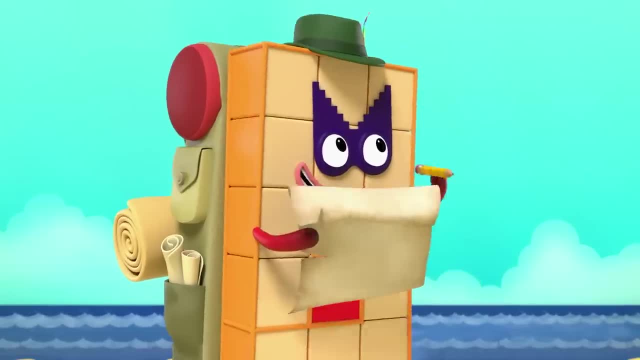 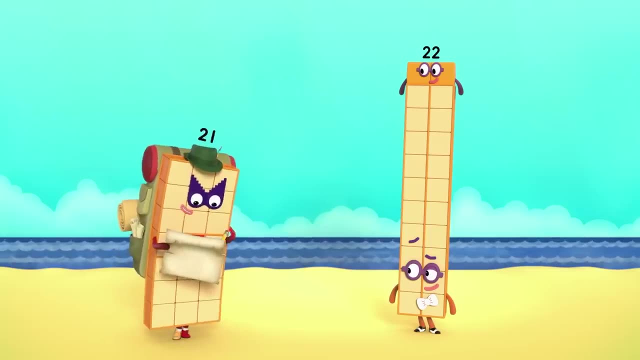 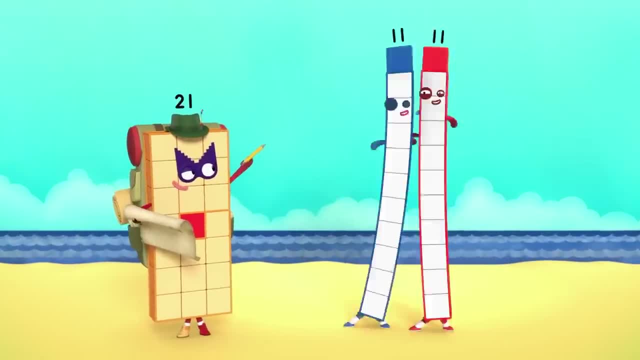 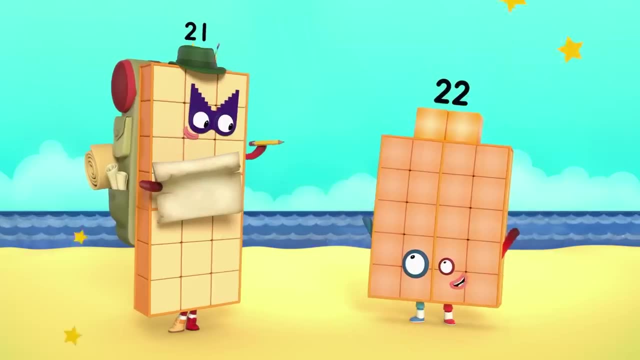 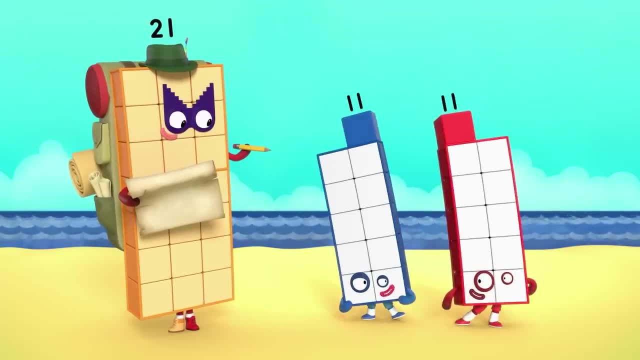 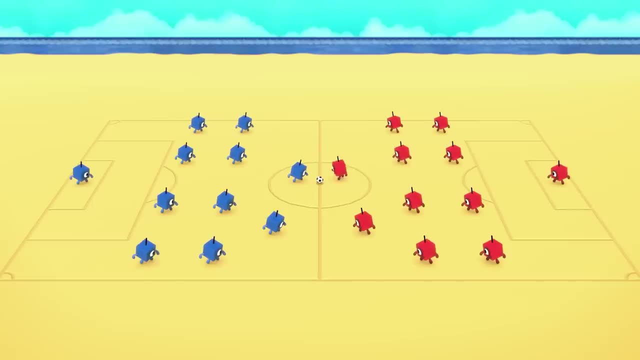 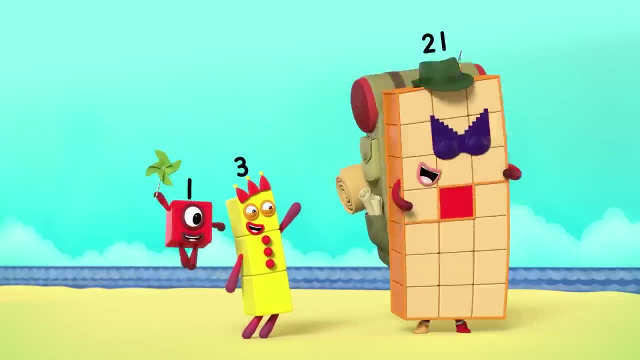 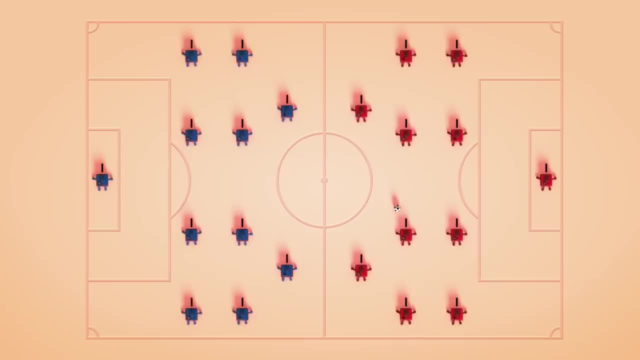 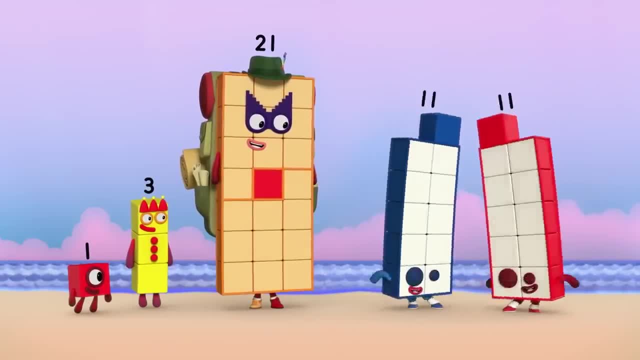 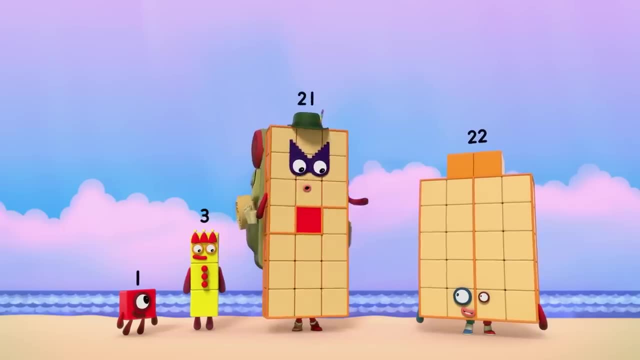 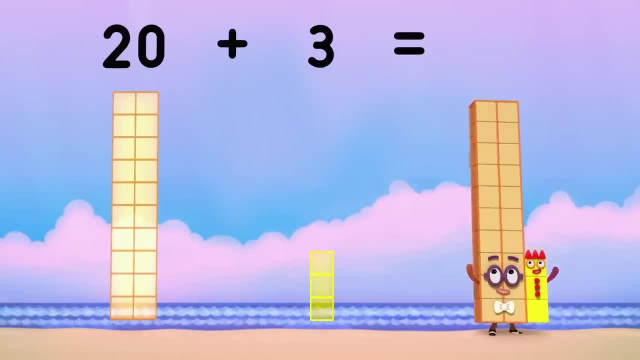 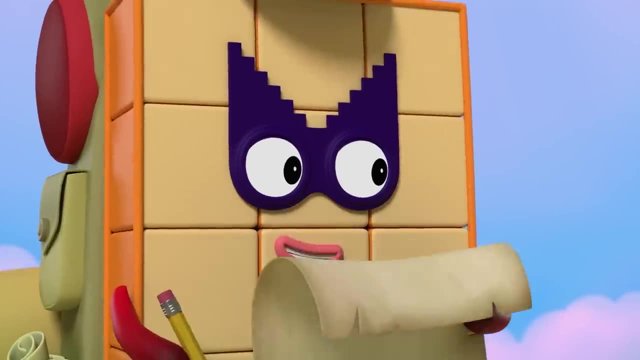 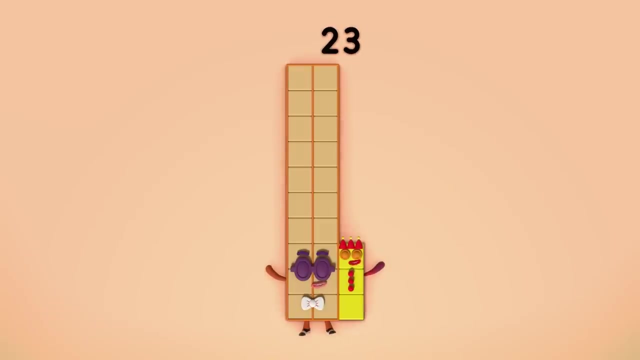 20 plus 3 equals 23! I'm 23.. I'm 20 and 3.. Now let's figure out who you are. I told you I'm 23. And I'm happy being me, But I want to explore more now. 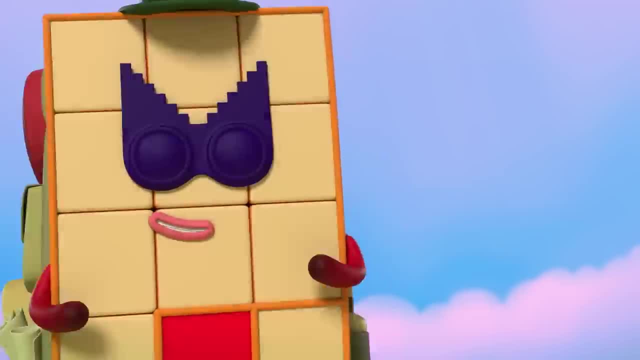 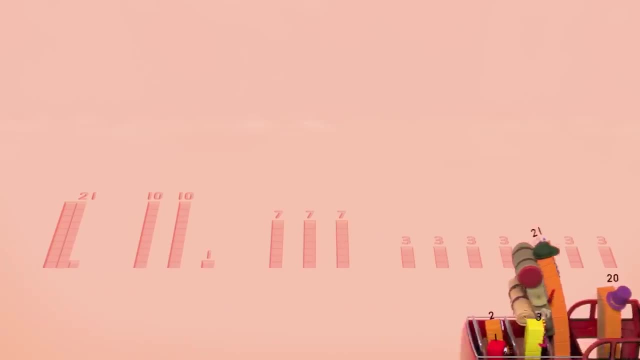 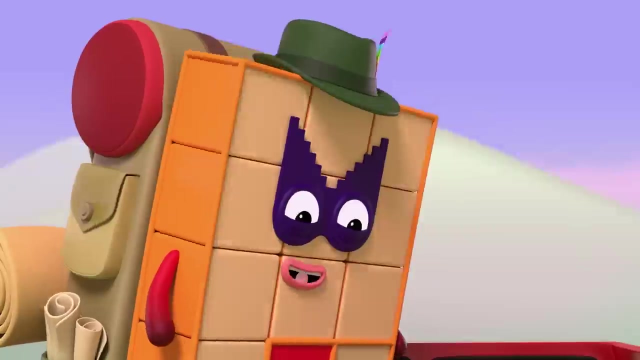 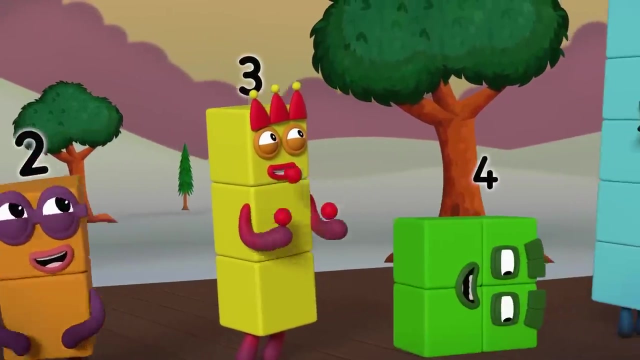 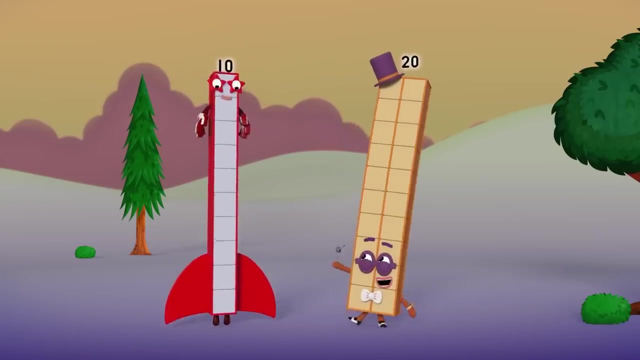 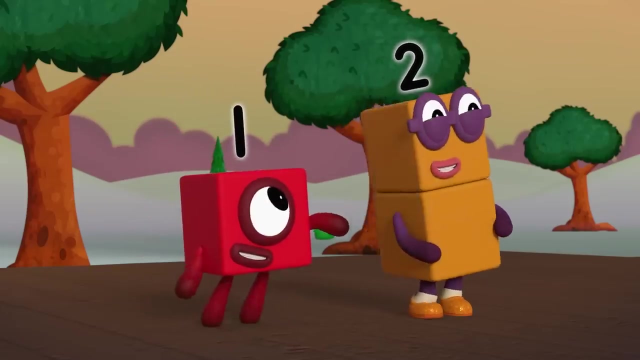 Well, I have got a bus back there, All aboard and off we go. Let's see what's out there. If I were bigger, maybe I'd be able to leap as high as you Ten. If I were bigger, maybe I'd be able to dance as well as you Twenty. 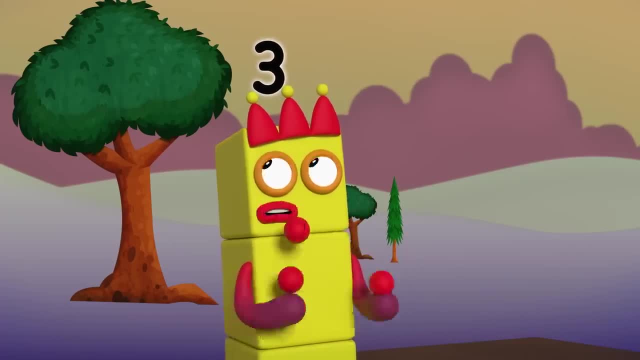 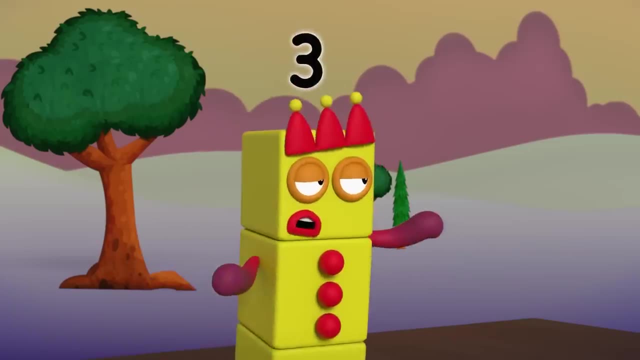 I don't want to be bigger. There's nobody in the world who's a better juggler than me. You know Three. there's someone you should meet. Huh, Who? Well, I'm 110.. And I'm 20.. I'm 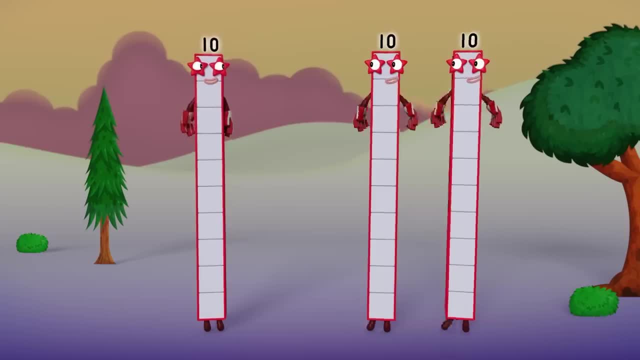 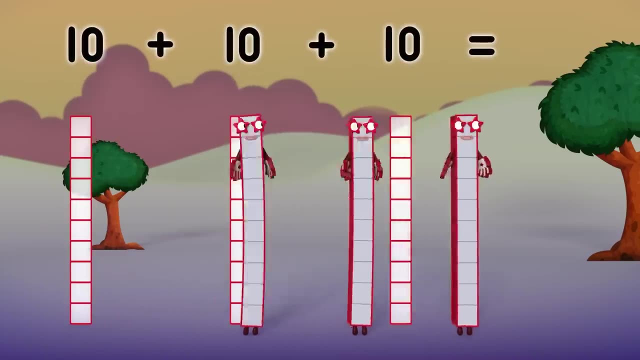 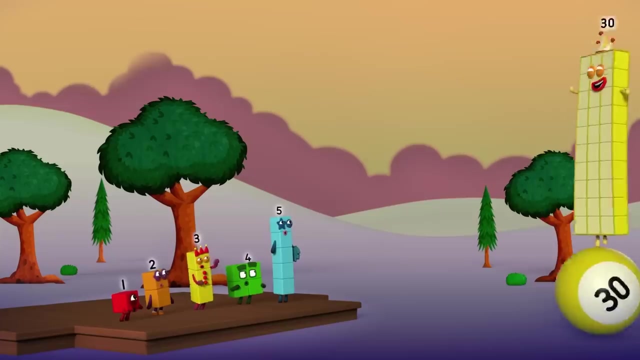 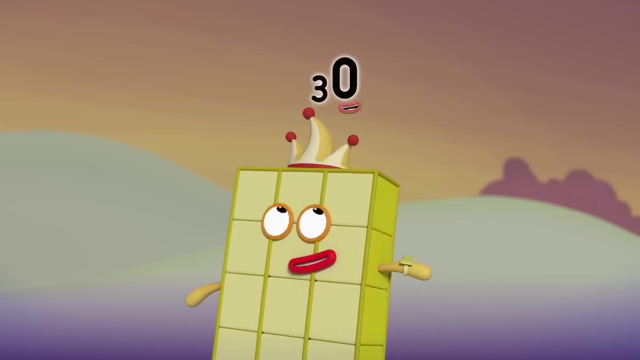 Two tens. Put us together, and what have you got? Three tens. Ten plus ten plus ten equals 30!. I am 30, the big entertainer. This three stands for three tens And nothing more. Oh, If you'd like to see more, then come to the circus. 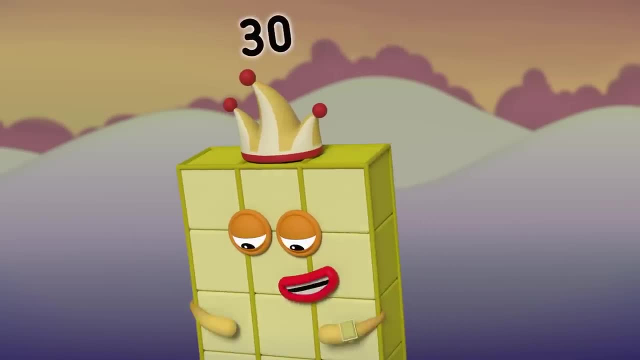 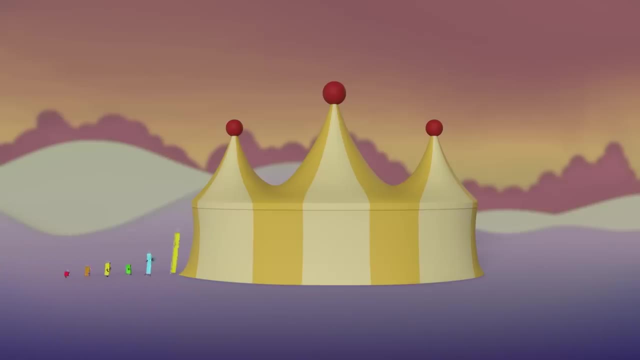 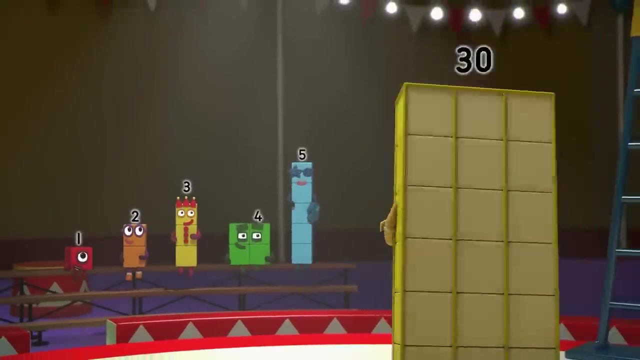 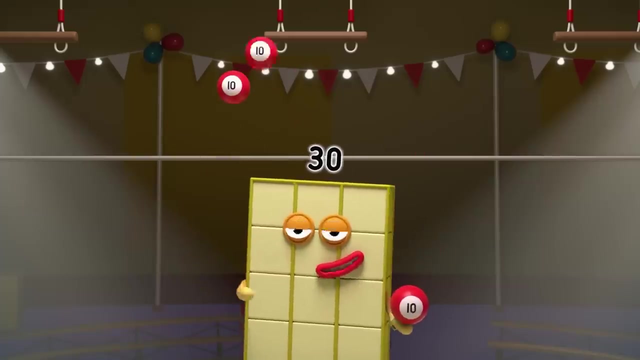 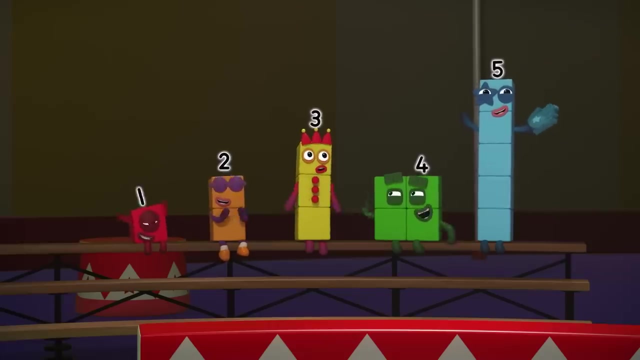 What circus. I like to keep it under my hat. Yay, Ho-ho, Welcome to the big, big, big top. Ho-ho, Three tens are ten twenty thirty, Thirty balls. Hold me, Wait, there's more. 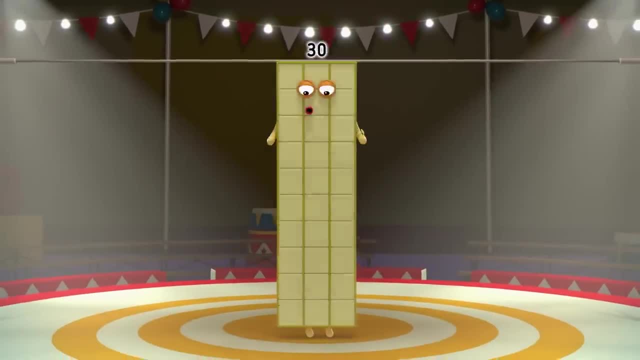 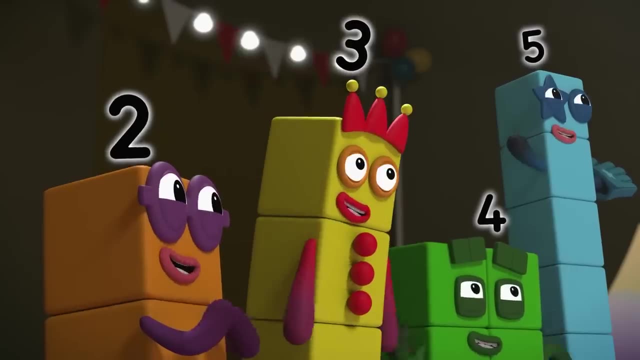 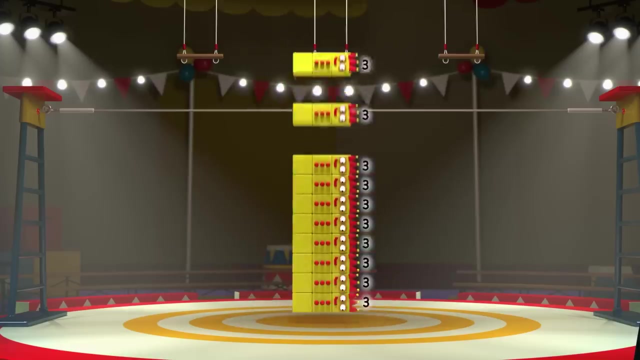 I'm three tens, which means I'm also Three tens Wow juice, Wow Ho-ho-ho, Ho-ho And three Ho-ho If you like that. you're going to love this next act. 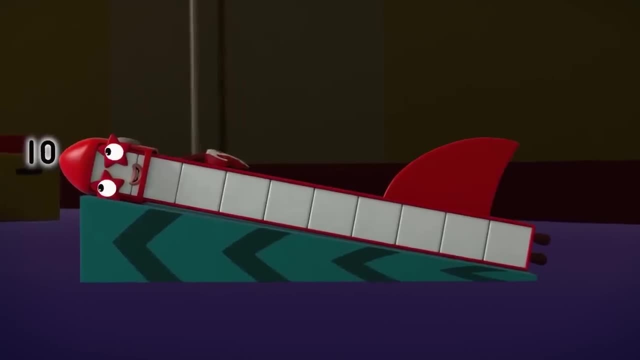 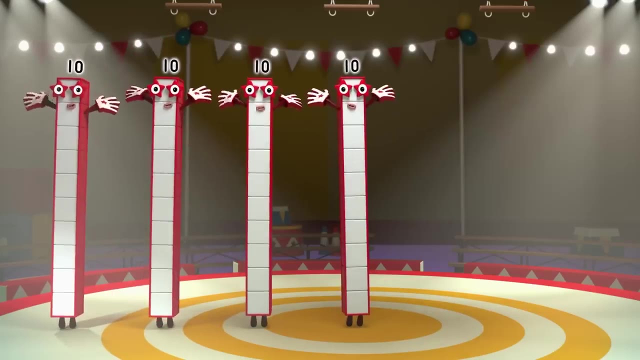 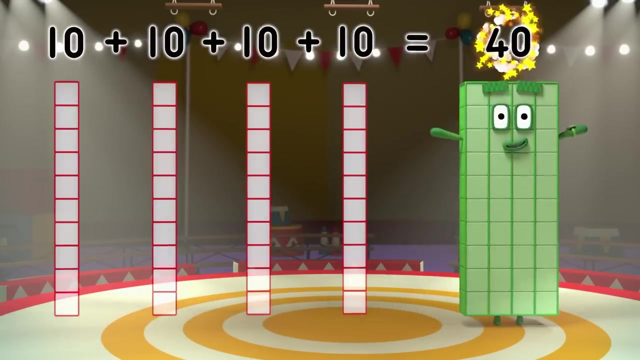 for which we need another ten. Woo-hoo, Four tens. Put us together and what have you got? Ten plus ten plus ten plus ten equals Forty. I am forty and I'm a big square. Oh, you're not a square. 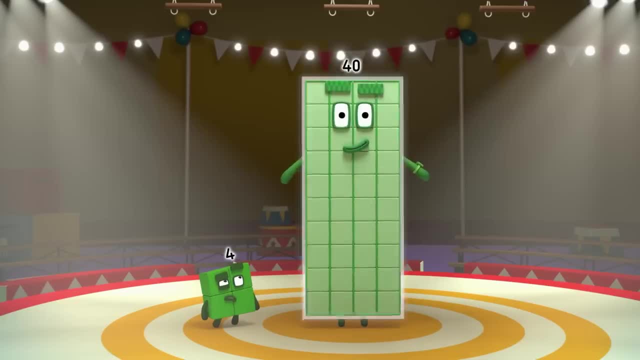 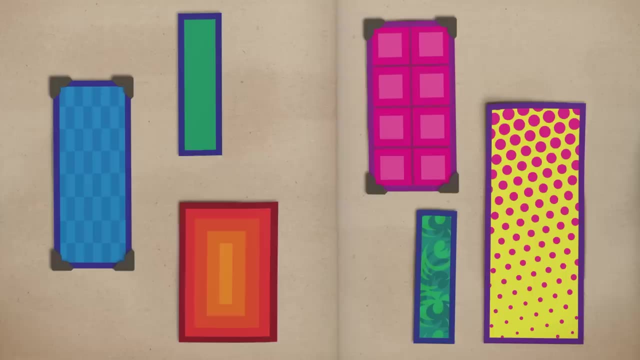 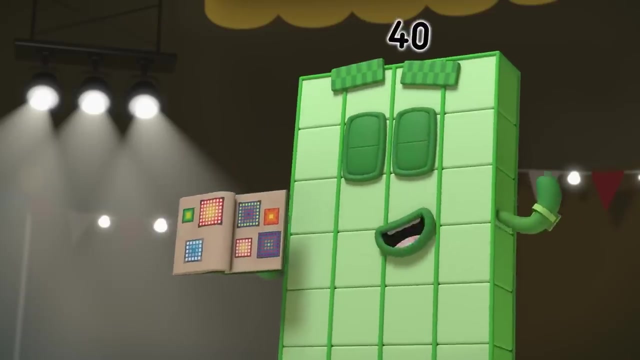 Oh no, I am not. I'm a rectangle. I love rectangles. Would you like to see my collection? I've got loads of different ones: Tall ones, wide ones, I've even got square ones. Huh, Squares are a special kind of rectangle, you see. 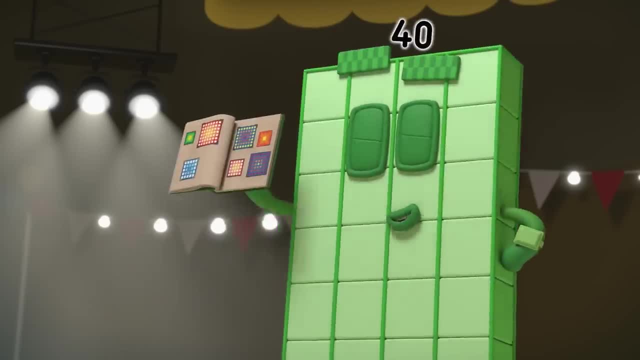 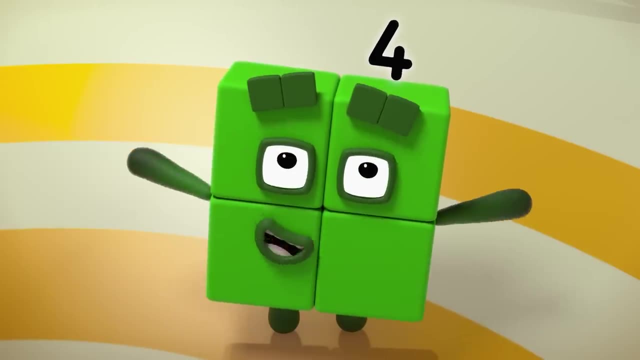 where all four sides are the same length, And a rectangle that's not a square is called an oblong. Ooh, I'm excited, A special rectangle. But if it's squares you want, it's squares you're going to get. 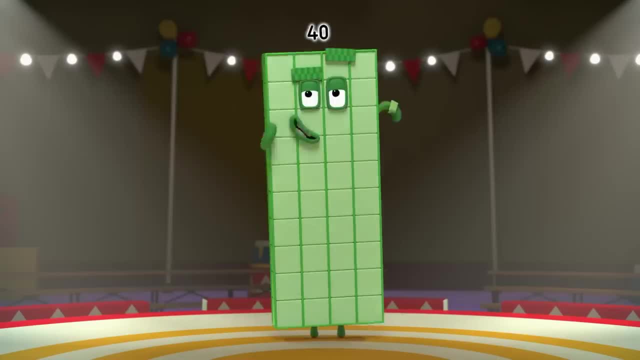 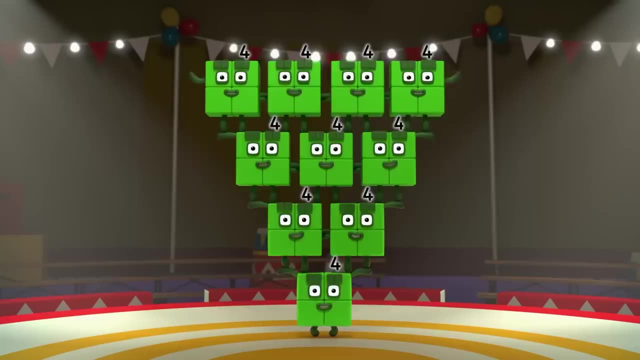 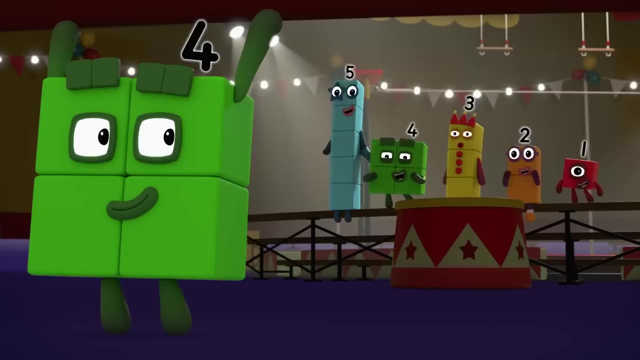 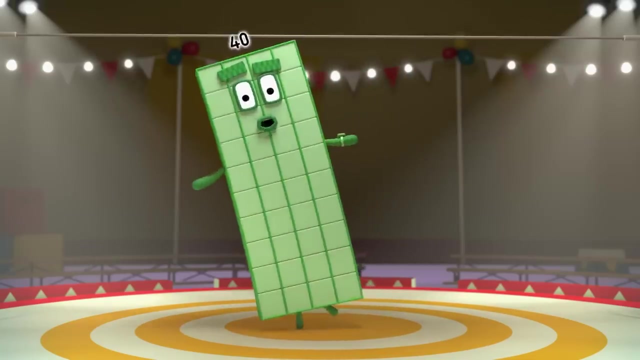 I'm forty. I'm four tens, Which means I'm also Ten-fours. Yay, With ten strong squares you can really Raise the roof. Whoa, That's all from me for now. Take care, square. So long oblong. 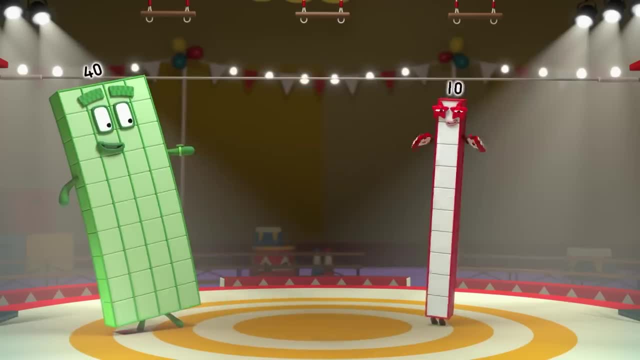 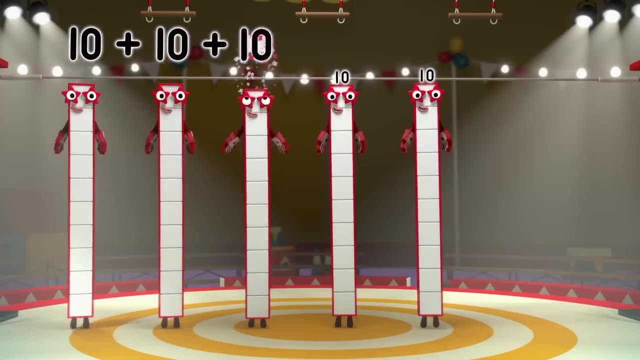 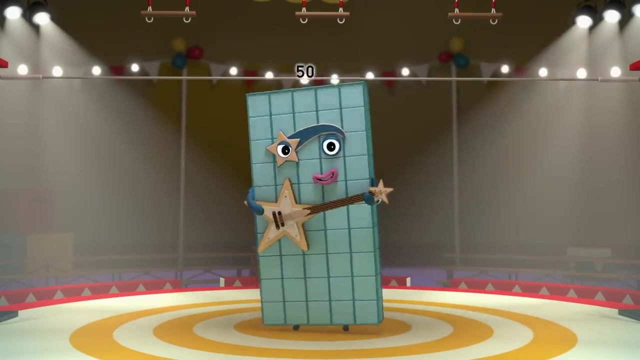 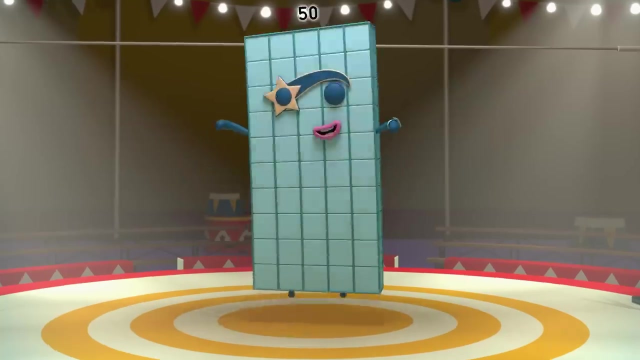 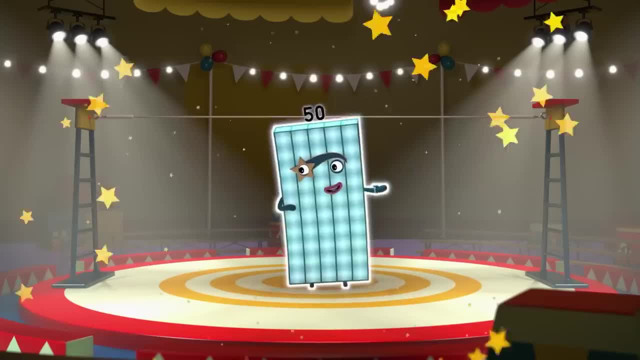 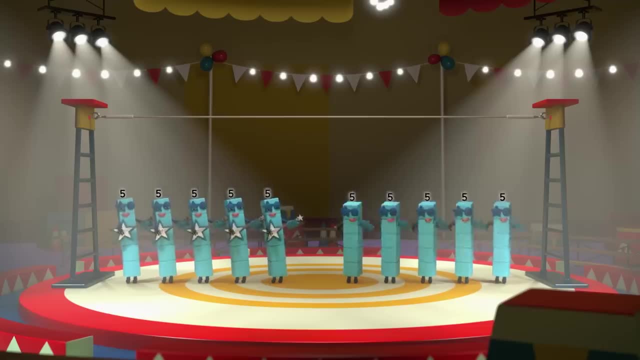 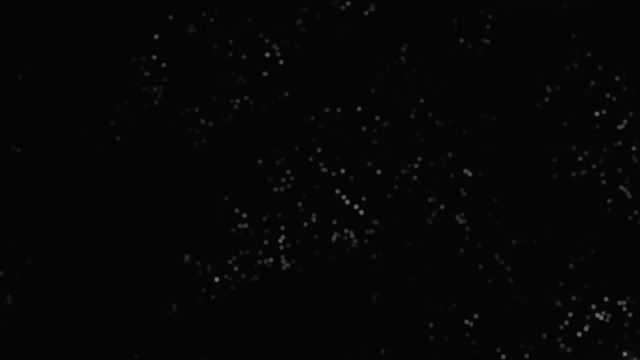 Yay, I'm fifty. I'm five tens, Which means I'm Ten, fives, High five. Ooh, Woohoo, Yay, Ha, ha, ha, ha, Yeah, Woohoo, Yeah. Now that's what I call a showstopper. 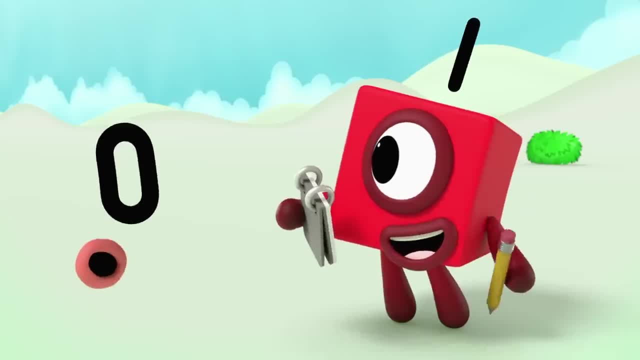 Showstopper, Showstopper, Showstopper. Shout out to the big one. Oh, hello one. What are you up to? Hello, zero, Today's the big one. I'm going to count higher than I've ever counted before. 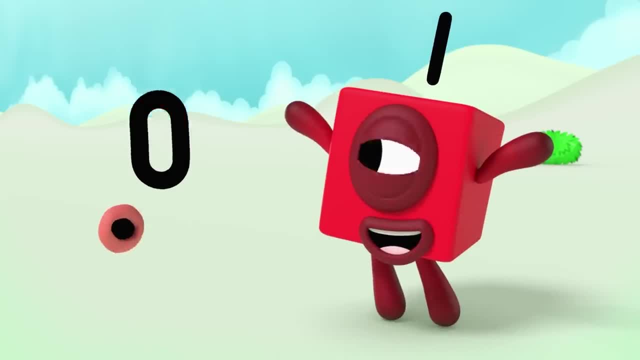 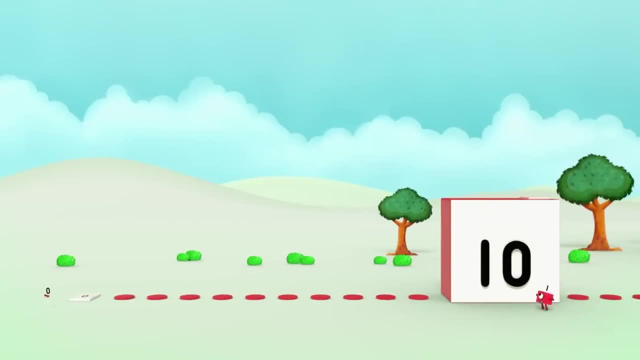 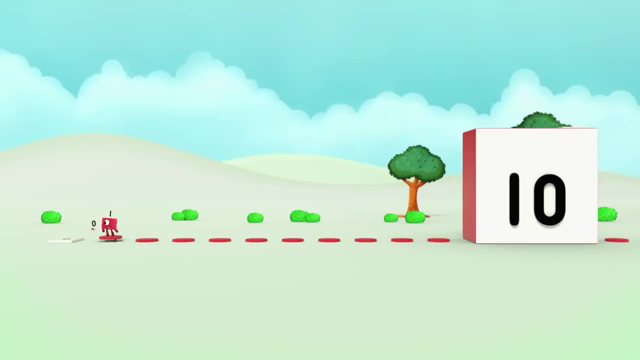 Ooh, I've got ten fantastic flippers like this one, Ten tall towers like that one And ten lots of ten springy springs. Woohoo, That looks fun. Can I have a go? I was counting them all. I think I have a ball game to play. 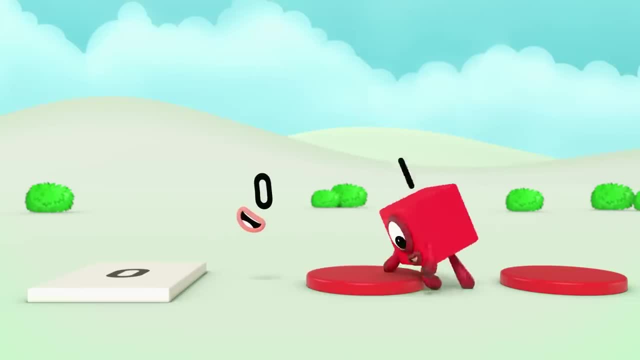 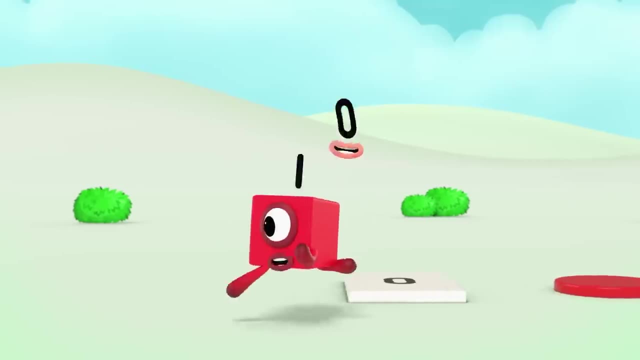 I like it. Ooh Easy. There's a flipper here with your number on. Then let's go for it. Great, but we need to go fast so we reach the last tower in time to catch this Ha Zero. 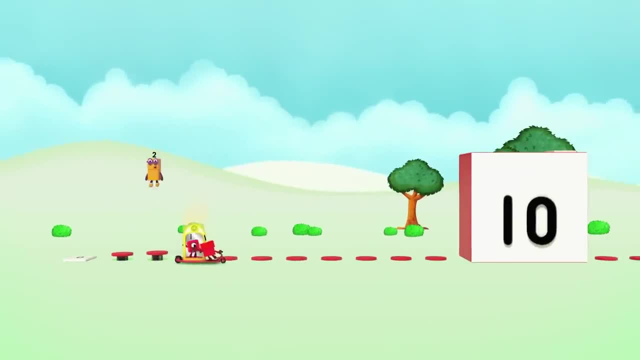 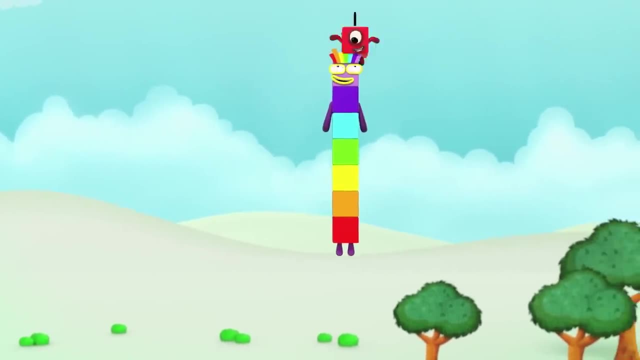 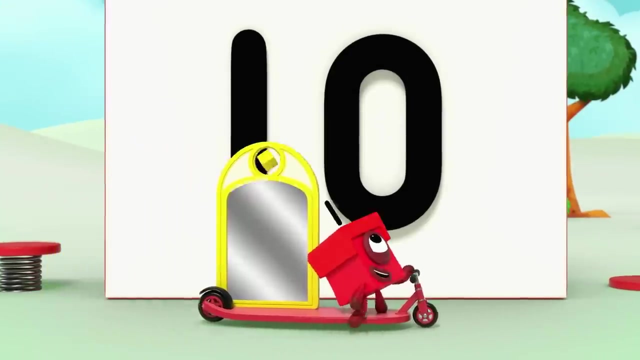 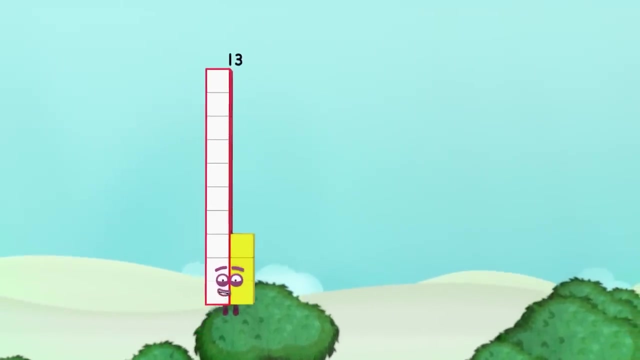 One, two, three, four, five, six, seven, Eight, nine, ten Coming in for landing. Keep going, Every second counts And clear for launch. Eleven, twelve, Thirteen, Fourteen, Fifteen, Sixteen. 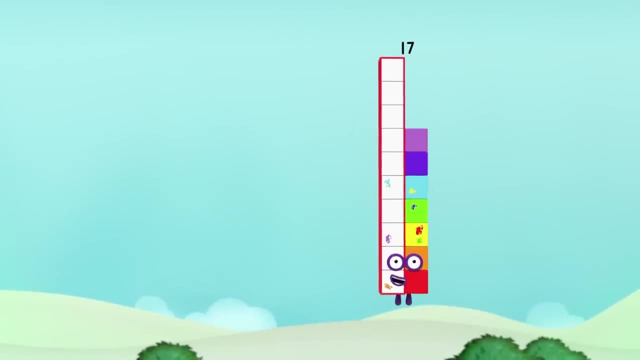 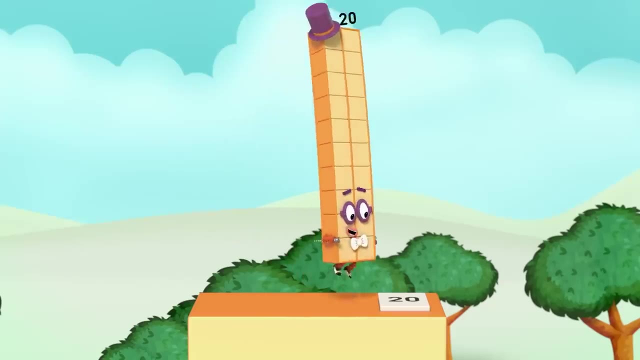 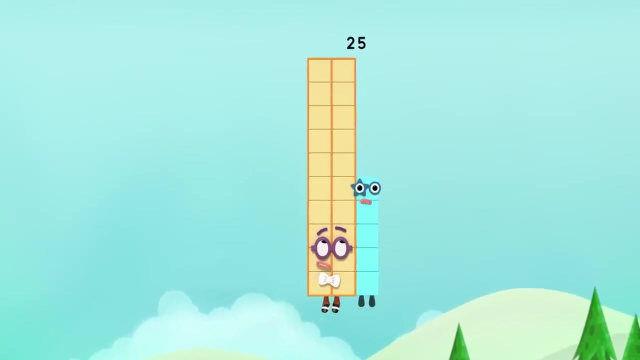 Seventeen, Eighteen, Nineteen, Twenty. We're going to make so many new friends today. Three, two, one Go Go. Twenty, Twenty-one, twenty-two, twenty-three, twenty-four, twenty-five, twenty-six. 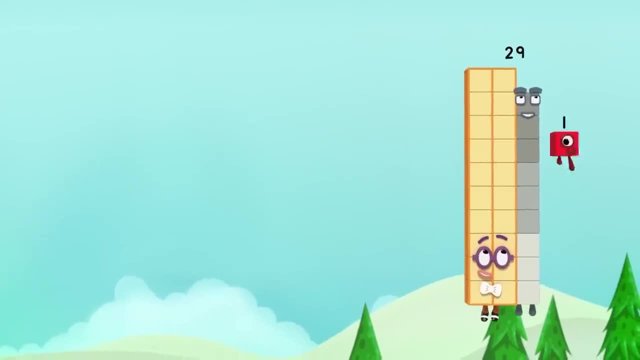 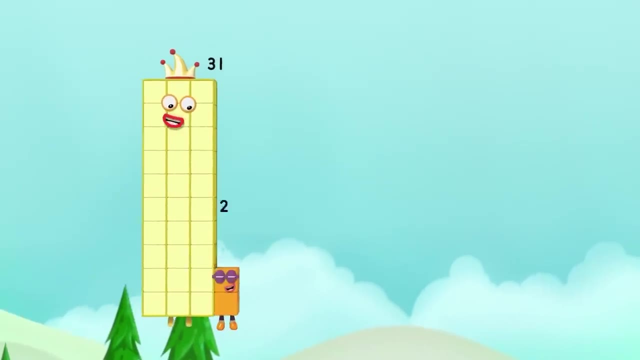 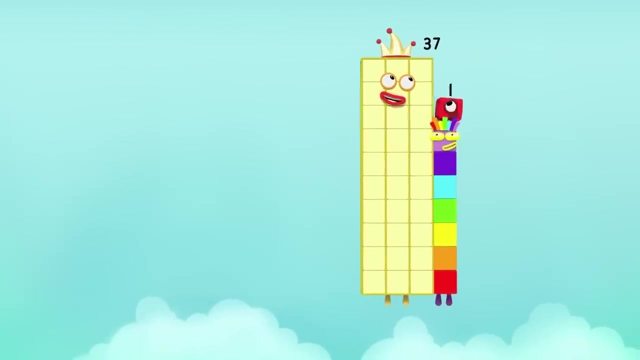 twenty-seven, twenty-eight, twenty-nine, thirty. Excellent acrobatics. everybody On with the, show. Thirty-one, thirty-two, thirty-three, thirty-four, thirty-five, thirty-six, thirty-seven, thirty-eight, thirty-nine, forty. 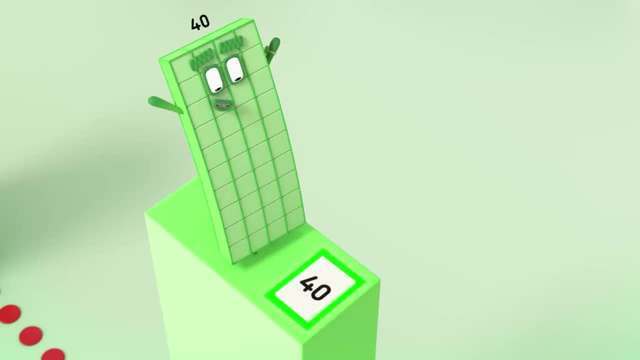 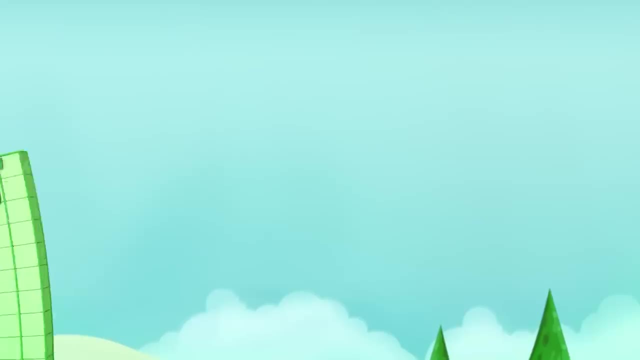 Ooh, I like the flipper. It's rectangular. Stay focused, We can do this. Sorry, Ahem. Oh. Forty-one, forty-two, forty-three, forty-four, forty-five, forty-six, forty-seven, forty-eight, forty-nine, fifty. 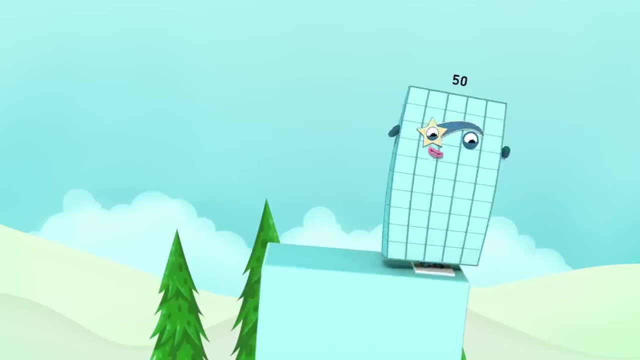 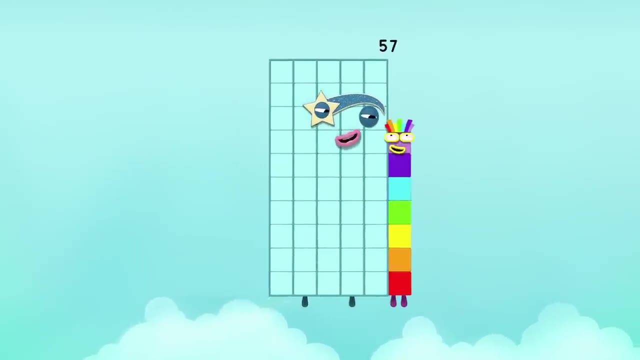 We're halfway there, Whoa. Fifty-one, fifty-two, fifty-three, forty-five, forty-six, forty-seven, forty-eight, forty-nine, fifty, Fifty-two, Fifty-three, Fifty-four, Fifty-five, Fifty-six, Fifty-seven. 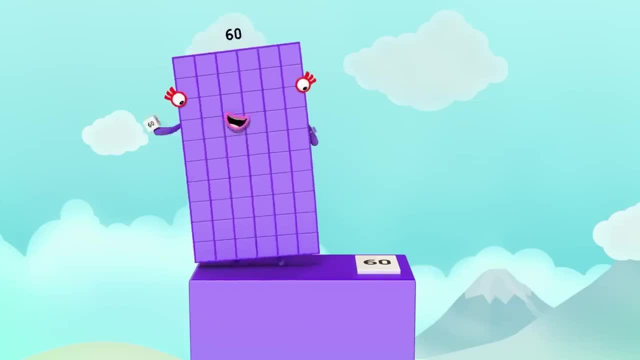 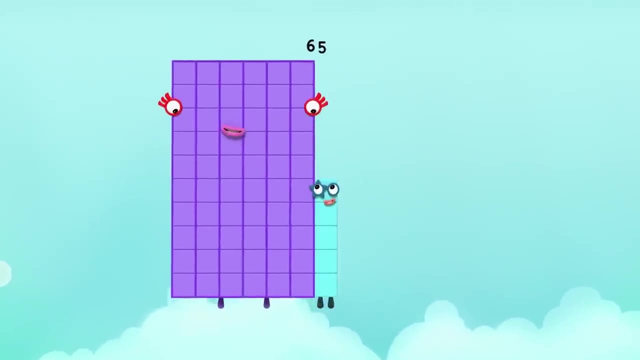 Fifty-eight, Fifty-nine, Sixty. Racing through the sky, this high roller is gonna fly. Sixty-one, Sixty-two, Sixty-three, Sixty-four, Sixty-five, Sixty-six, Sixty-seven, Sixty-eight, 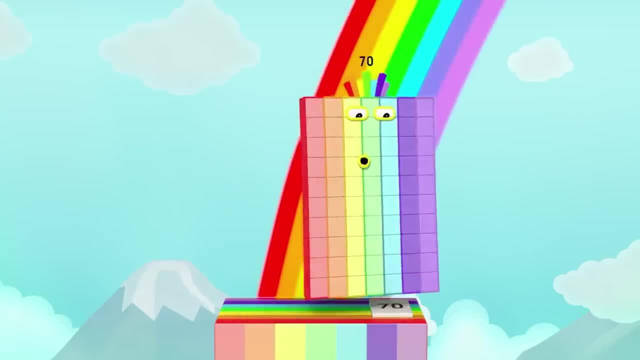 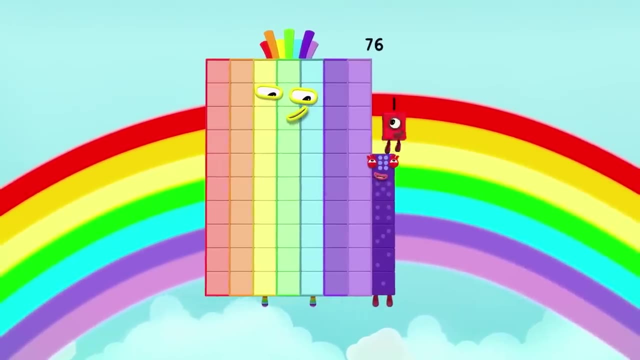 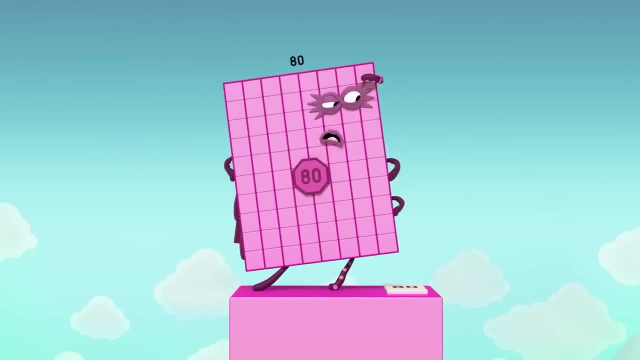 Sixty-nine, Seventy- We're going over the rainbow- Seventy-one, Seventy-two, Seventy-three, 74,, 75,, 76,, 77,, 78,, 79,, 80!. I don't like the look of those clouds. 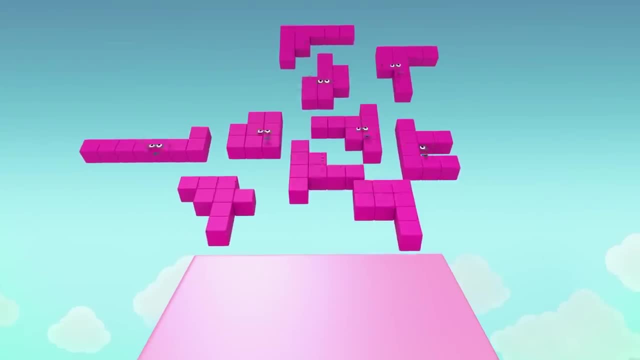 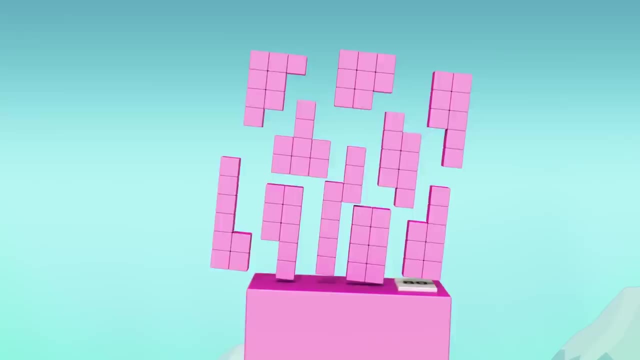 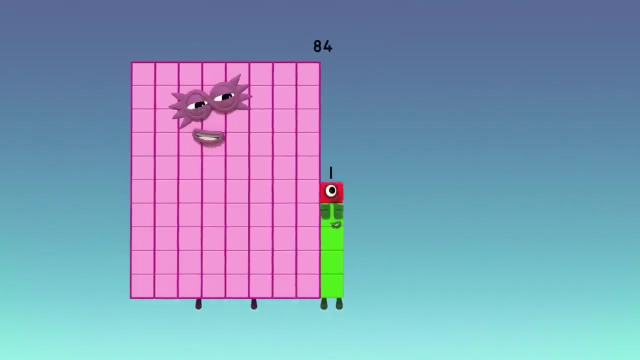 There's no time to stop Octoblocks, assemble Dinoctoblock. roar, Roar Up up and away: 81,, 82,, 83,, 84!, 85,, 86,, 87,, 88,, 89,, 90!. 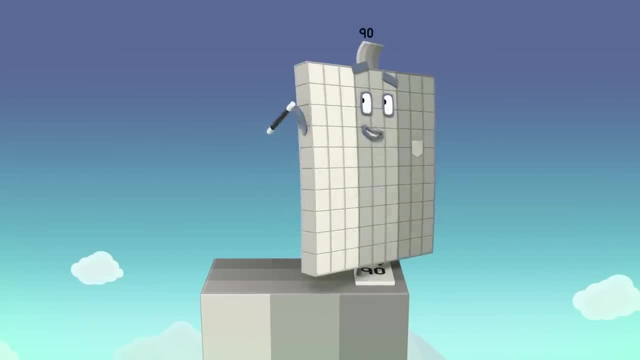 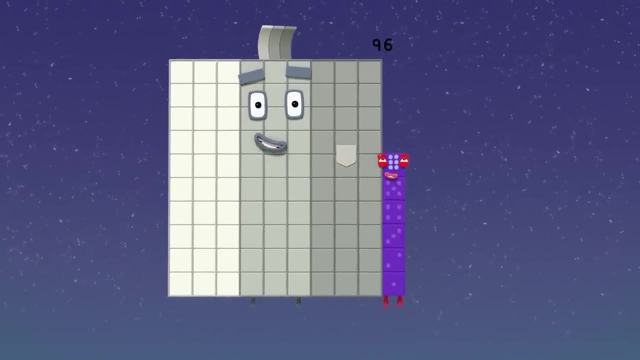 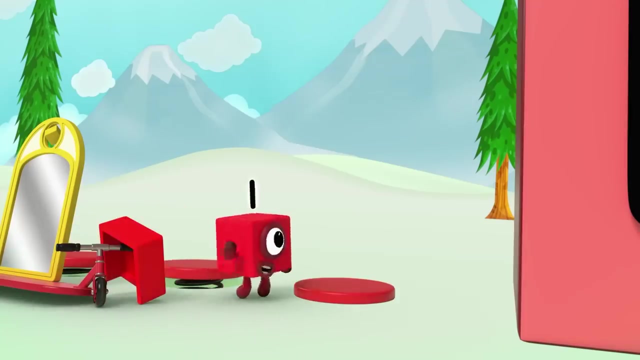 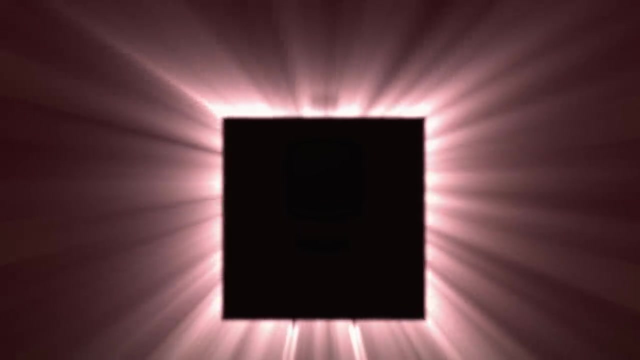 Nearly there, with no time to spare. This should do the trick. 91,, 92,, 93,, 94,, 95,, 96,, 97,, 98!, 99? And one more is 100!. I am 100!. 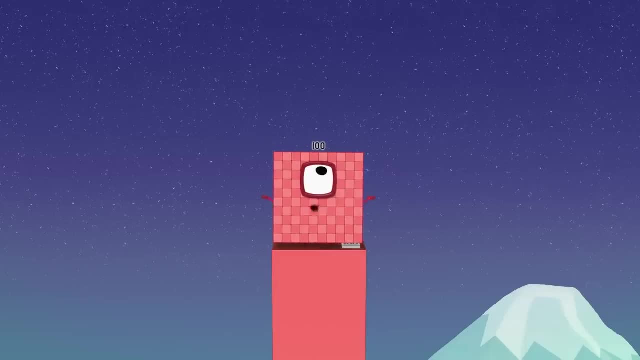 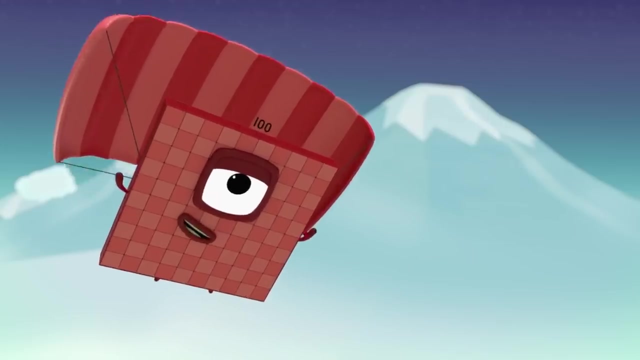 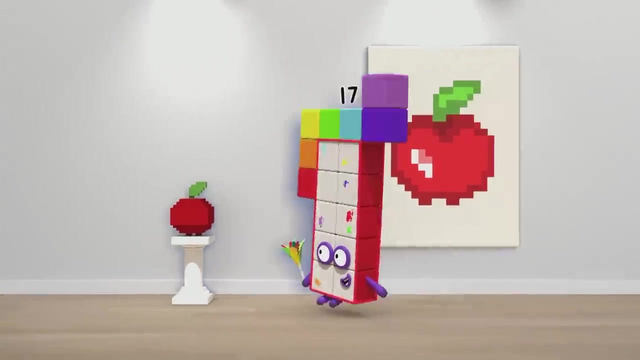 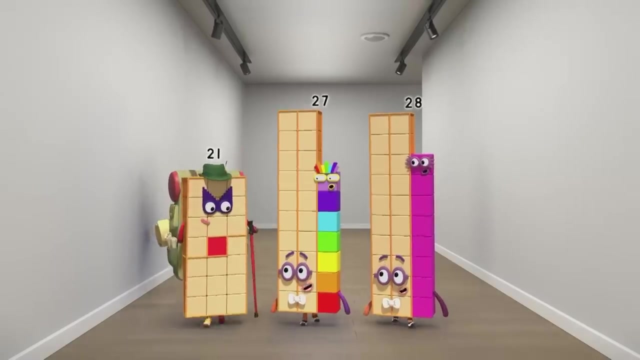 Ten, lots of ten on top of the world. Now how do I get down again? Ah, a parachute. 100 is 100!. 100 words gaan, Hm, wheyhee, Come on. Today feels like a good day for figuring out some numbers. 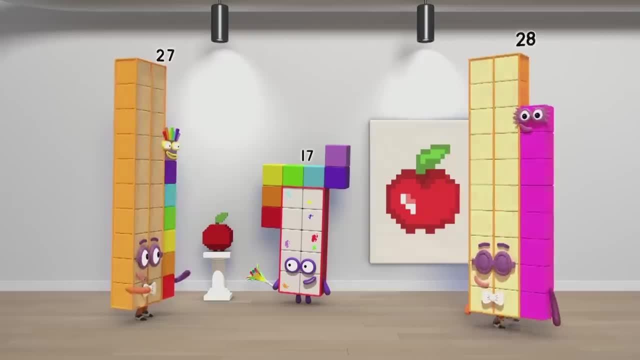 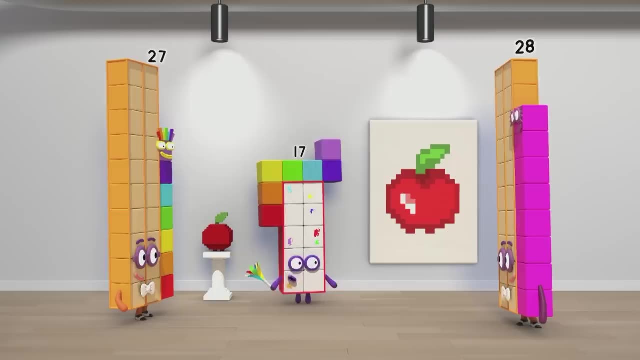 And art is an excellent way of expressing yourself. Ohhh, I like this sculpture. Personally, I prefer this painting. Art is all about finding different ways of looking at things. Take my new exhibit, for example: The Pattern Wall. The Pattern Wall. 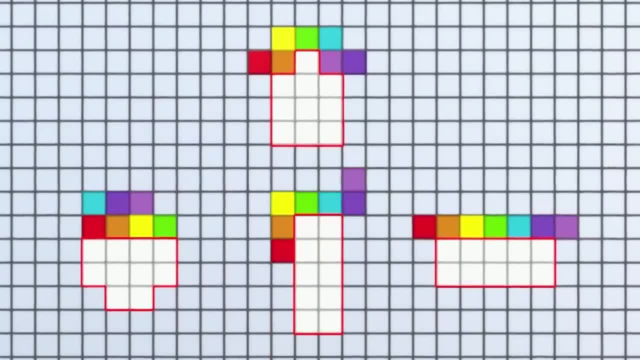 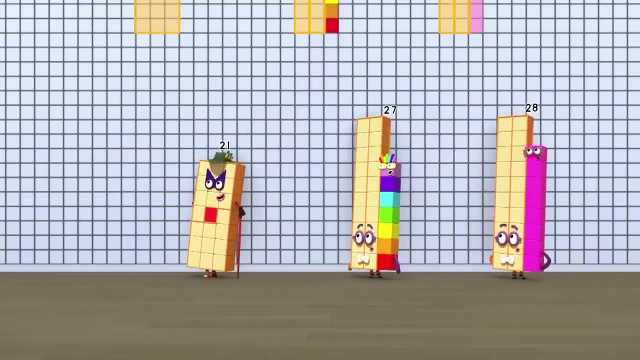 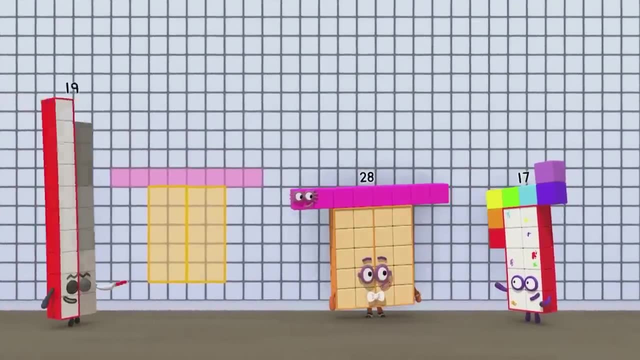 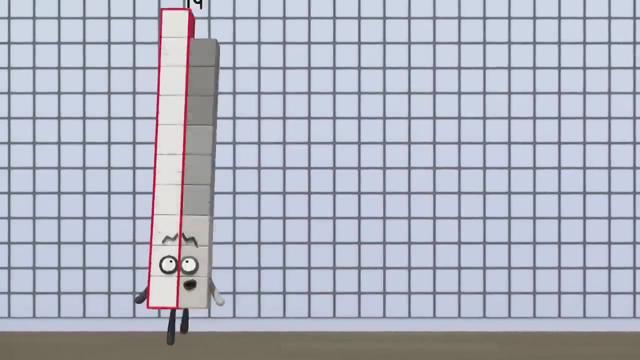 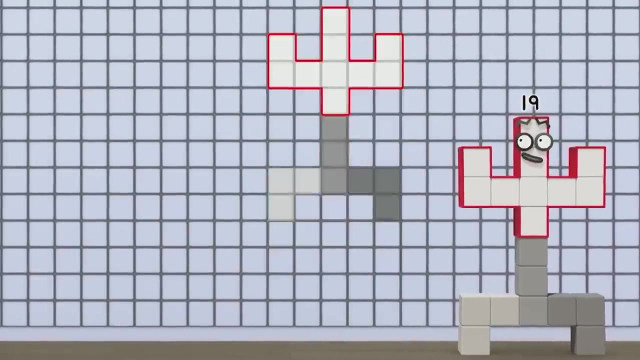 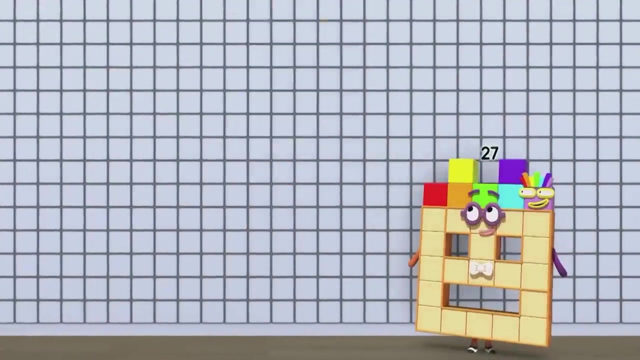 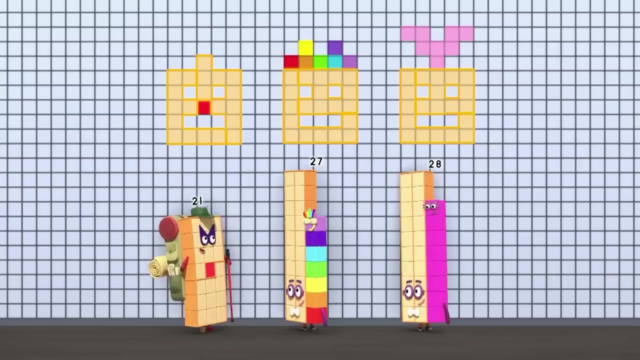 Whatever shape you make with your blocks, the pattern wall will copy. Not bad, may I Help yourself, A surprised cow? But now let's loosen up those blocks and make some crazy shapes. Now let's find a clean bit of wall and see what we can do. 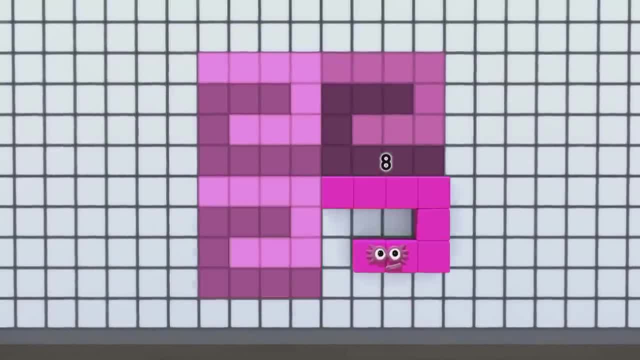 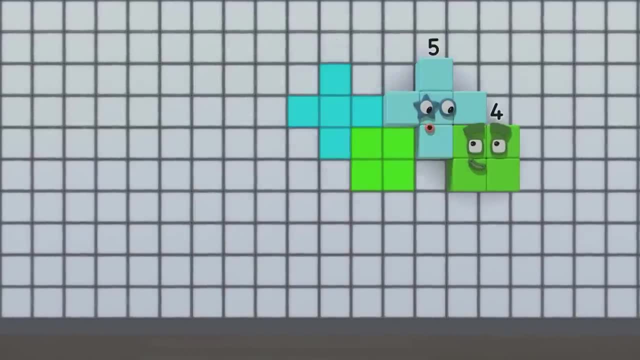 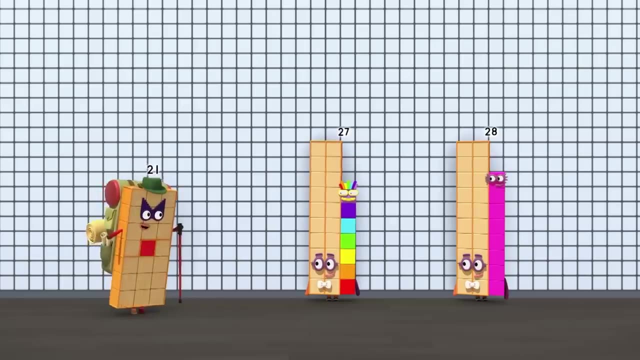 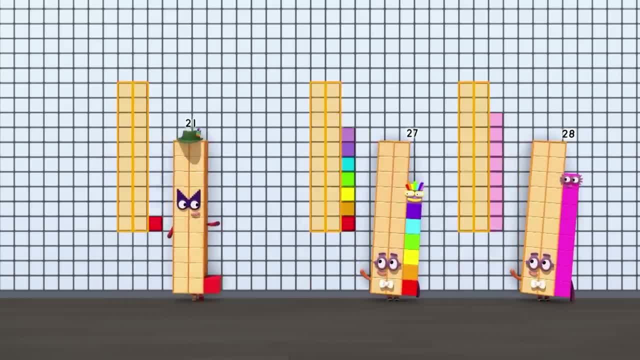 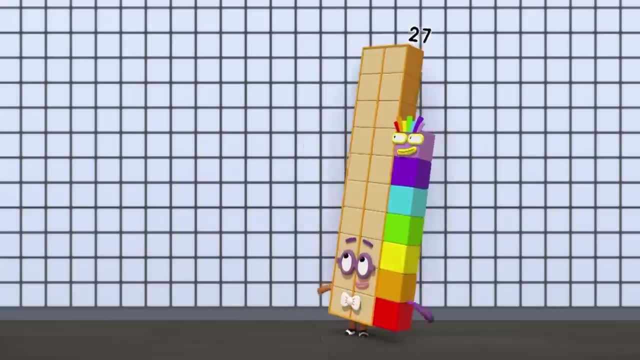 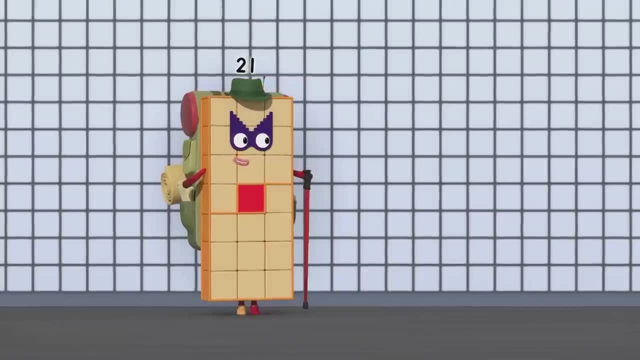 Ten, Ten, One. That's a good first step. It helps you see where you fit in the pattern of counting numbers. Oh yes, I'm between twenty-six and twenty-eight And I'm underneath eight, And I'm beneath nine And eighteen. Now see what shapes your blocks can make. 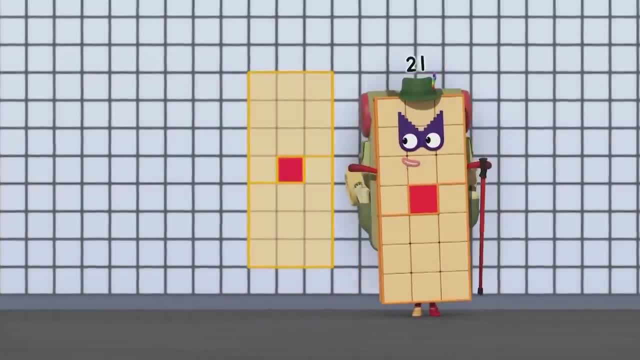 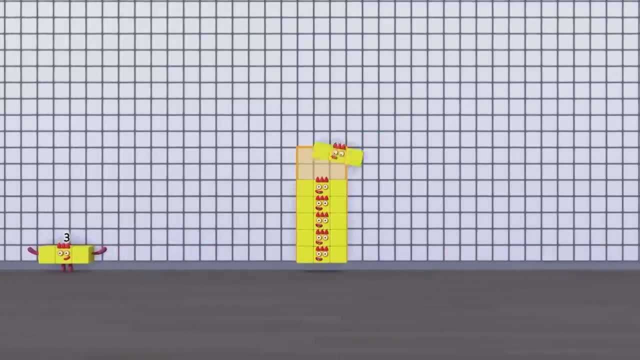 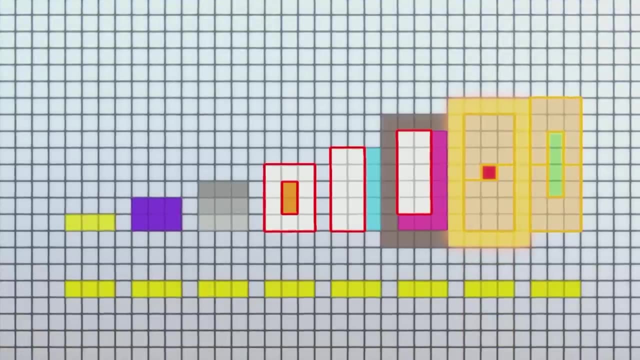 Rectangles are the simplest. Look, my twenty-one blocks can make seven. lots of three, See, see, see, see me, me, me. So I fit the pattern of the family of threes Between eighteen and twenty-four. Ooh, I can fit that pattern too. 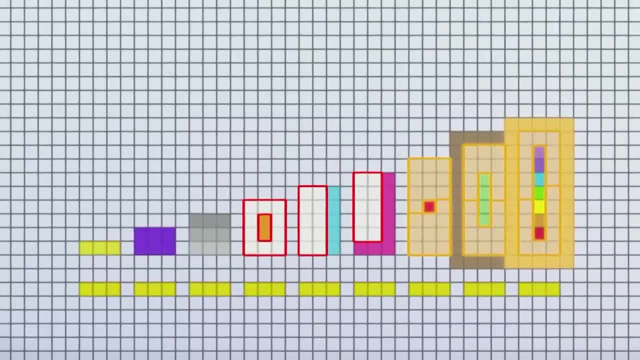 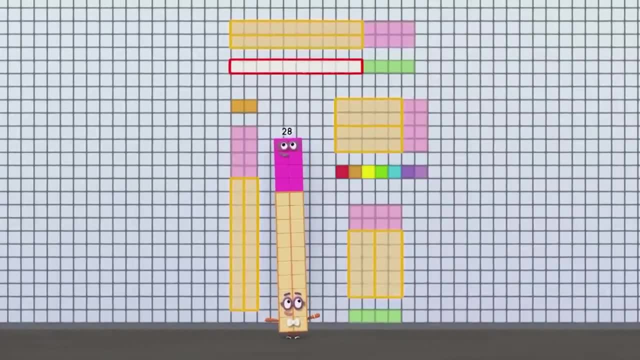 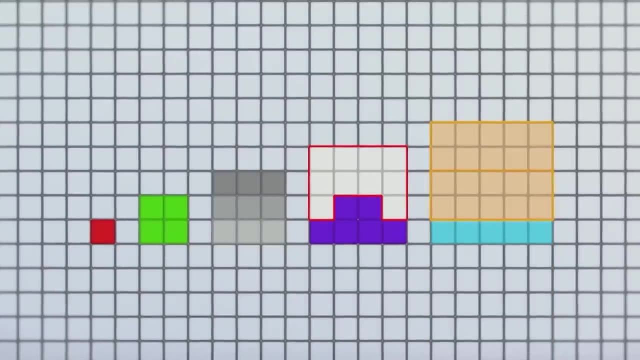 I'm three, more than twenty-four. Well, I'm part of the family of twos, fours, sevens and fourteens too. Ooh, lots of rectangles. Now me, I'm part of the family of squares. Maybe we're squares twenty-seven. 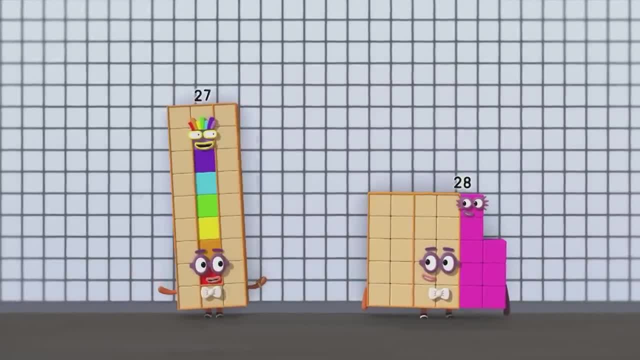 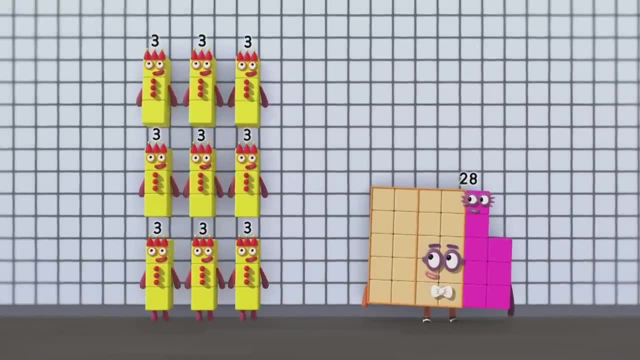 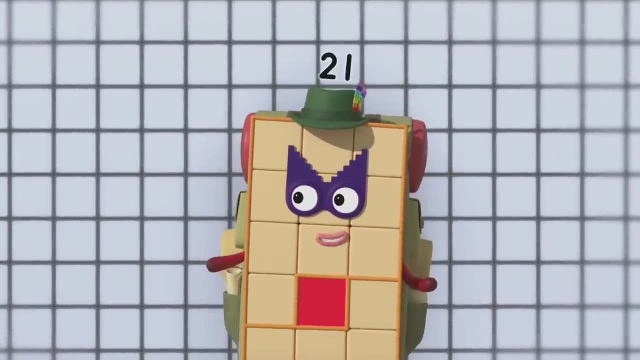 Nope, Guess not, Although I can make three square nines, And each nine is Three threes. Where are the three, three, threes? Woohoo? Oh, there are lots of patterns to explore, Like my favourite Step shape: One, two, three, four, five, six. 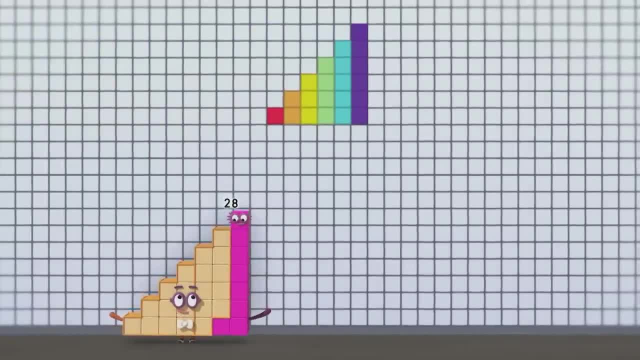 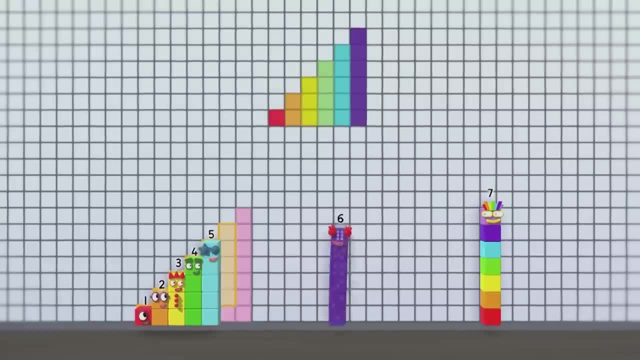 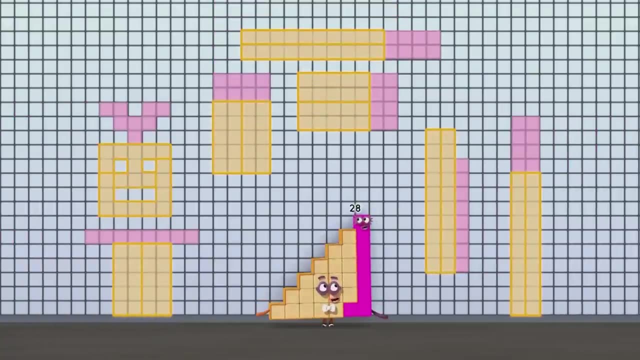 Ooh, let me try. Yes, I'm seven blocks bigger than you twenty-one, So I can make a step shape too. One, two, three, four, five, six And, lucky rainbow, seven. So many patterns to play with. I figured myself out. 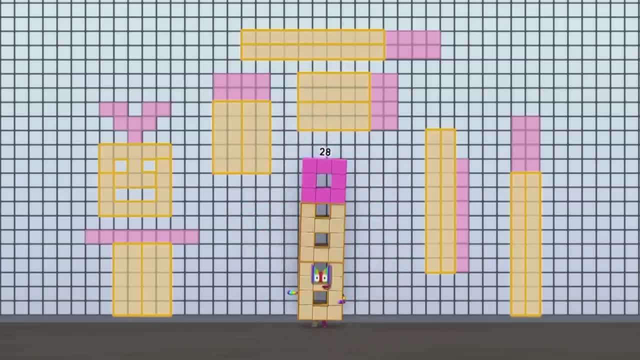 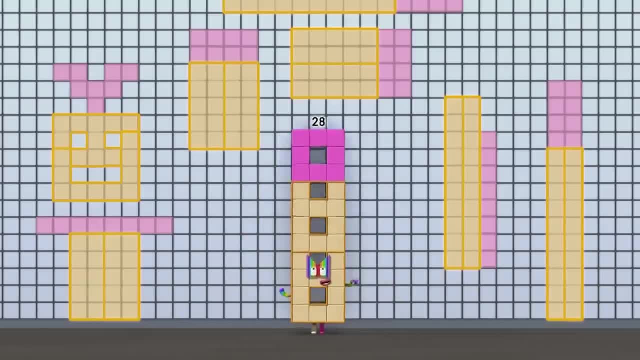 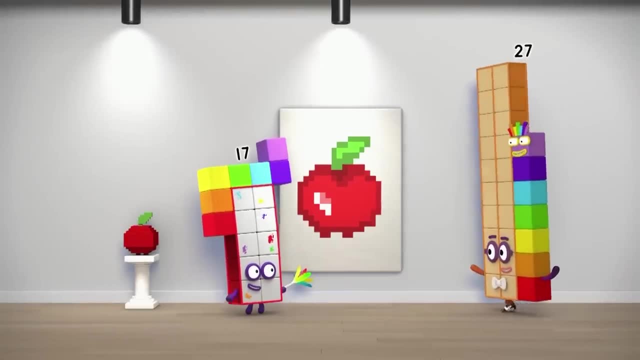 I'm twenty-eight and I'm a pattern: pioneer Square with a hole, chunky cross tower with windows. Get in, Hello twenty-seven looking for something. Yes, I'm just not sure what. There's something I'm missing. Art is all about explaining. 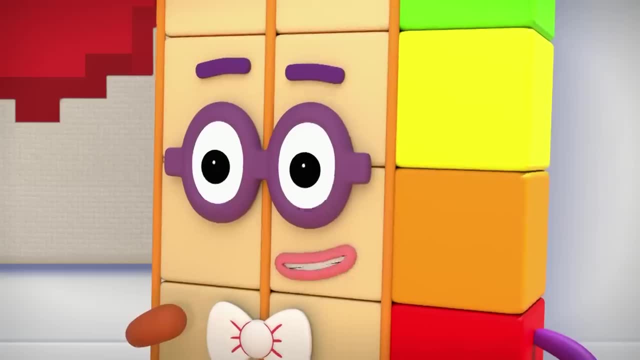 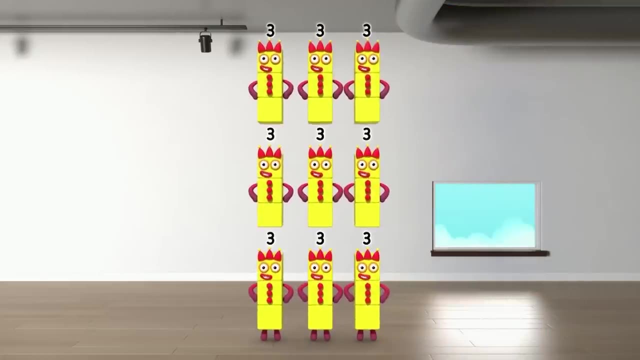 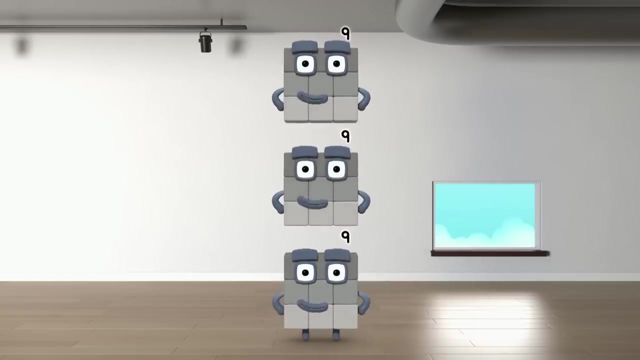 Exploring new directions. New directions, That's it. Three, lots of three. threes can make Three square nines, And if you put us together in a new direction, We make a cube. I figured myself out: I'm twenty-seven and I'm a cube. 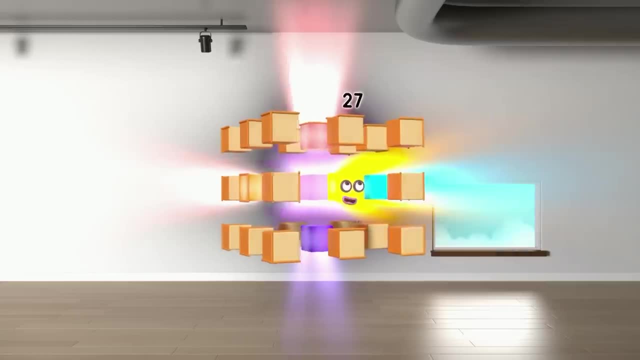 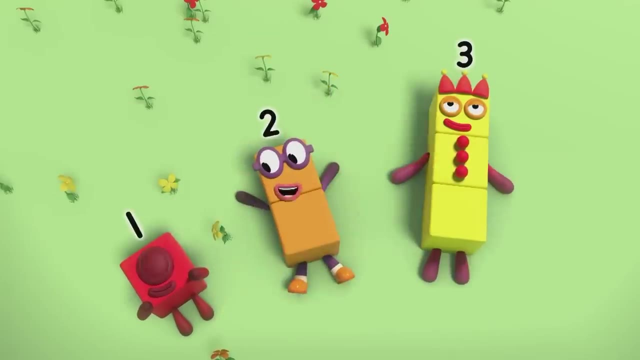 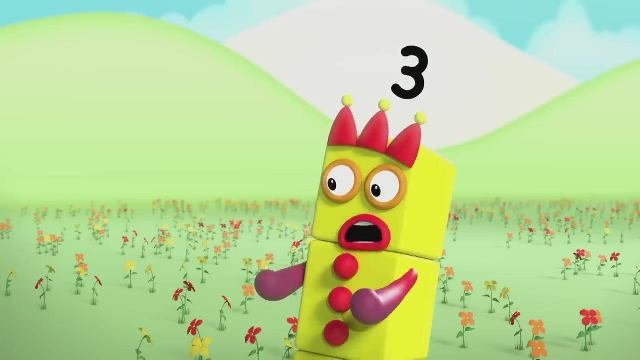 Three by three by three. Wee Making patterns is so much fun, Whichever way you look at it. Remember the last time we were here, Wan? Yes, you asked what if and the what if-er appeared. Wait, wait, wait. 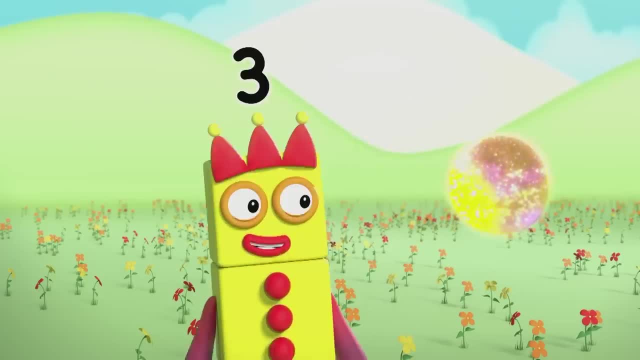 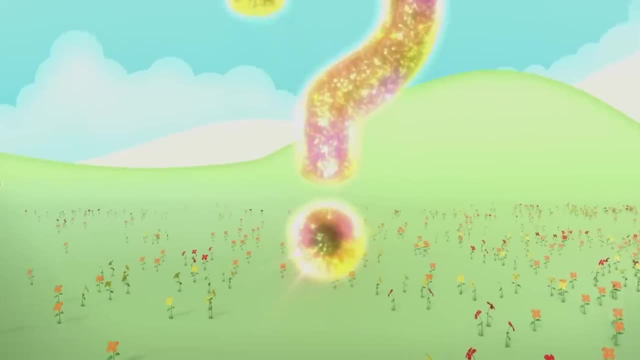 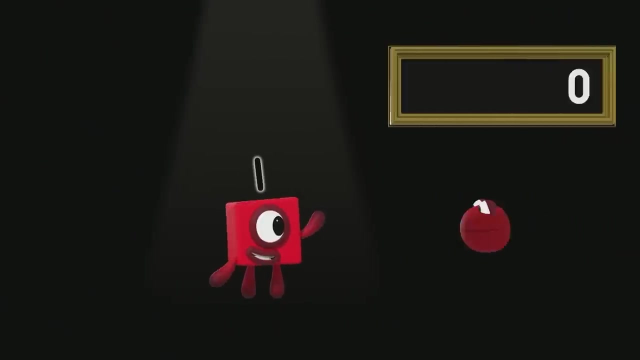 What's a what if-er? Now, that's an interesting question. What is a what if-er? The best way to find out is to ask me a question. What sort of question? A question like this: What if you kept on counting forever? 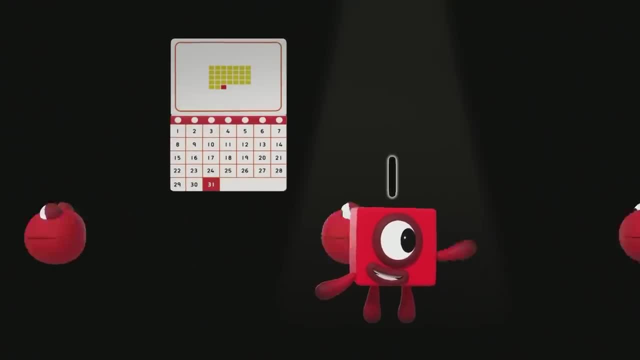 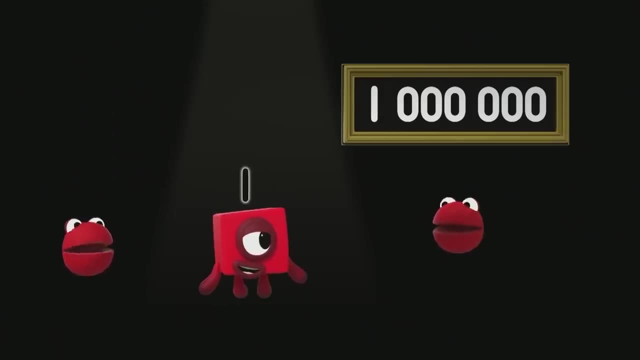 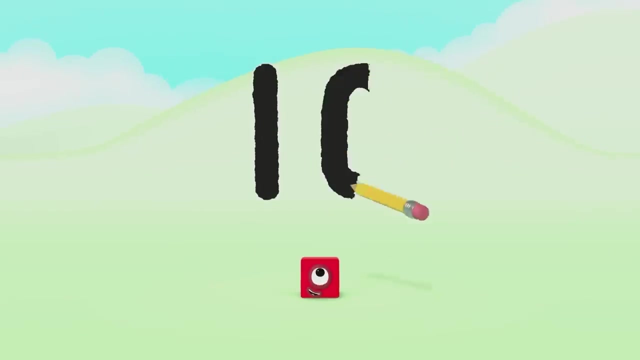 It would earn the admiration of your friends. You might make it to a million in a fortnight. But how high could you get if forever never ends? What if you kept writing zeros after one? It's the same as if you multiply by ten. Pretty soon you'd reach a million again. 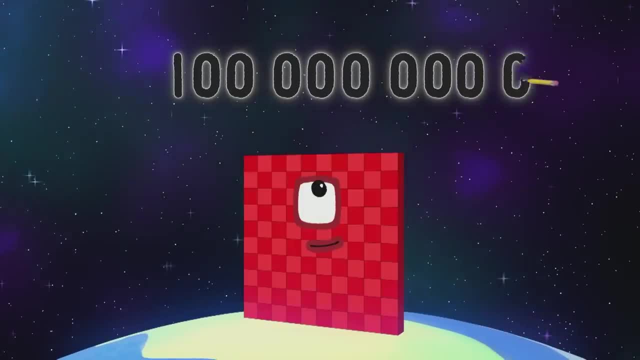 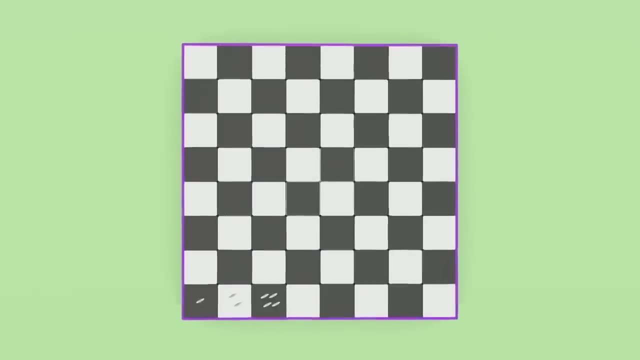 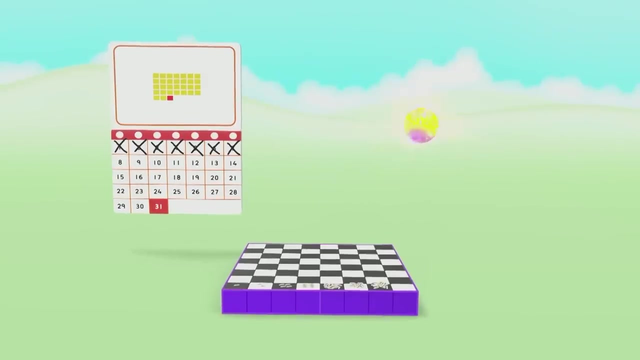 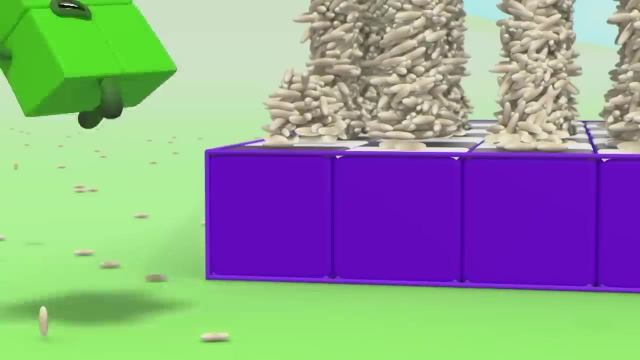 What then? What then? What if you start with a single grain of rice And double it, double it, double it every day. In a week you'd have no more than a handful In a month. you'd be giving it away. Stop the rice. 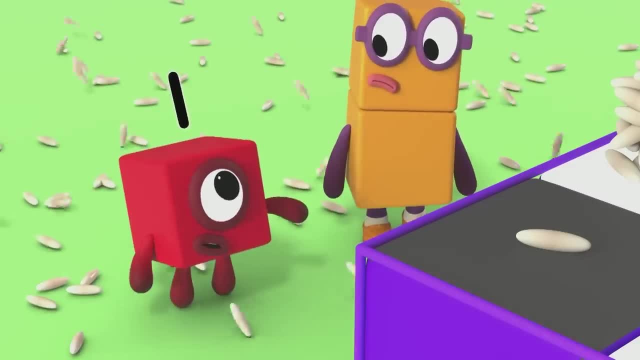 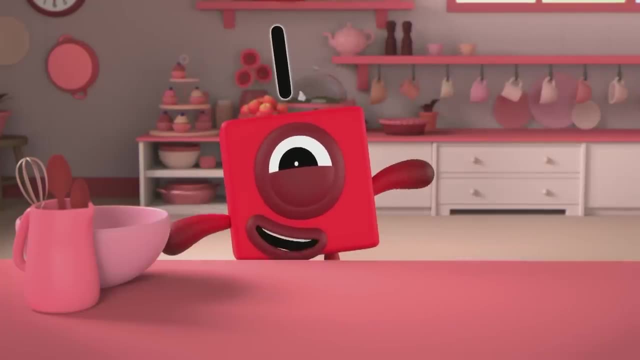 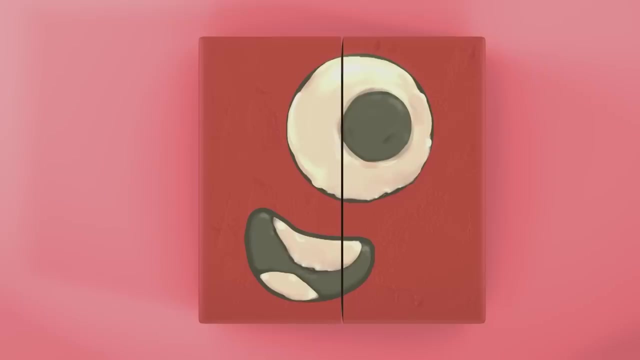 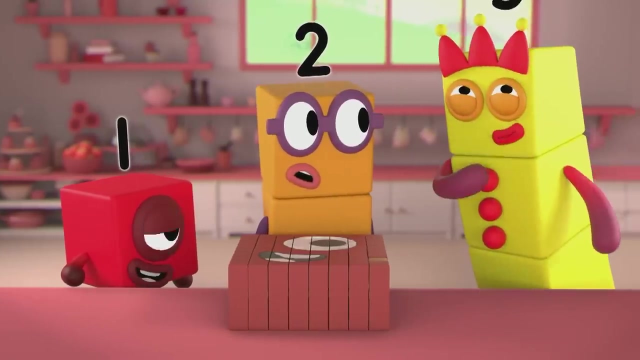 Please stop the rice. What if the rice stopped? Interesting question, Ask me another. What if one could be divided into pieces, Smaller parts, like the slices of a cake? You could cut it into four or eight or sixteen, But is there any end to the fractions you could make? 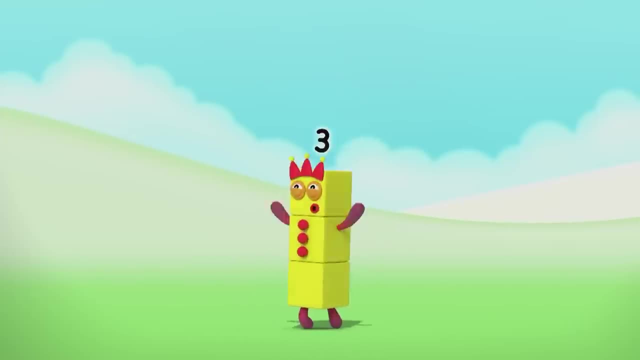 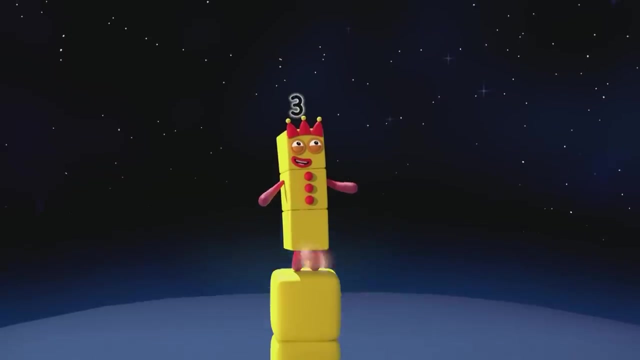 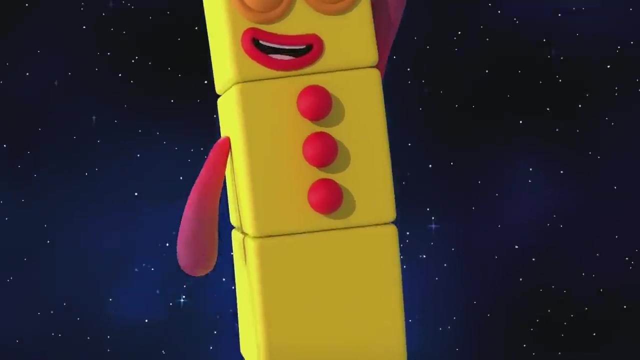 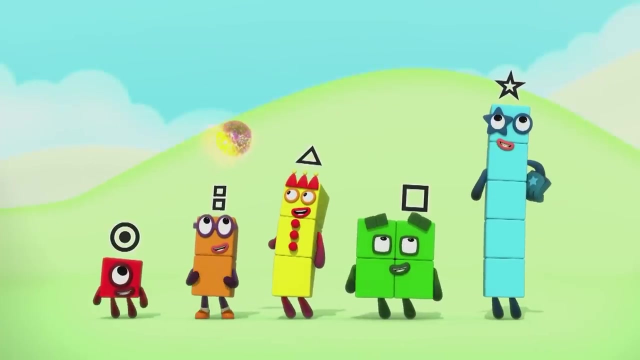 What if we tried to build a tower to the moon? And would it take a hundred years to reach the top, Though you might not want to think about the drop? Huh, Don't stop, Don't stop. What if the number blocks each had a different name? 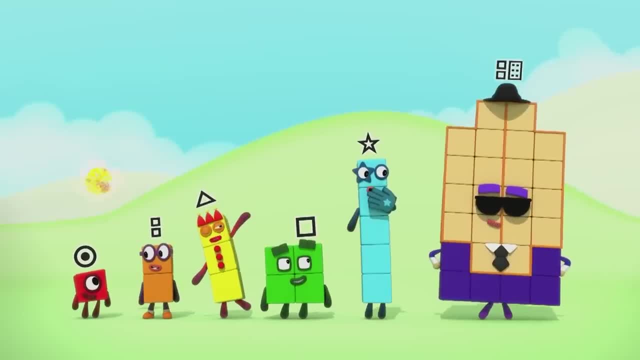 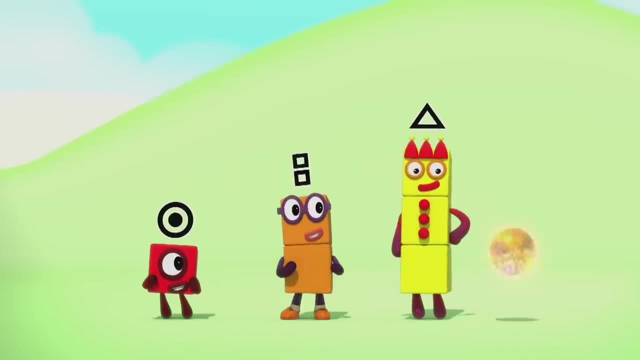 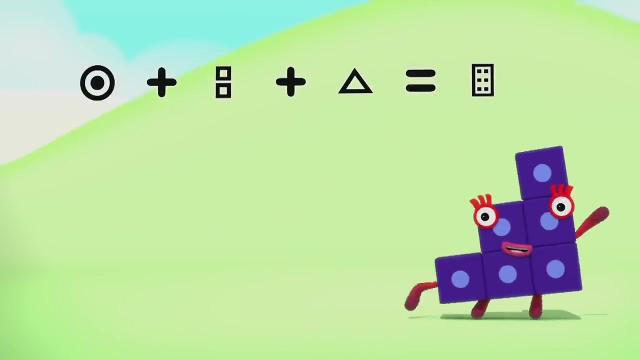 Like new, fling, clop, flinty bun. Well, you'd have to count, would be no different, But you'd have to learn new words for everyone. New plus fling plus plop equals fun. What if three was the highest you could count to? 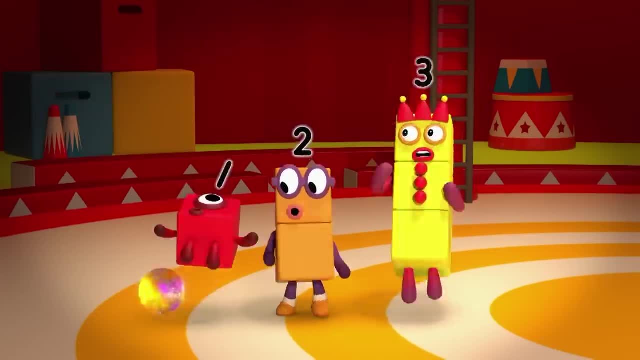 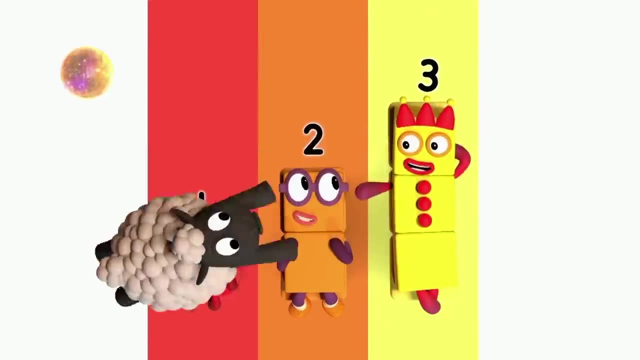 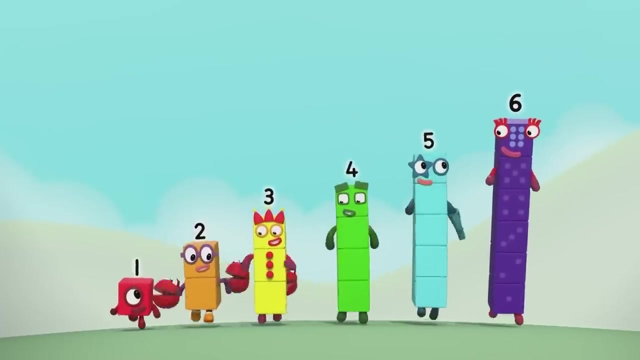 It's a question that could tie you up in knots. Counting sheep to get to sleep could be quite tricky. One, two, three, Plenty, many lots, Five, four. What if the number blocks all disappeared one day? Would one and two and three still equal six? 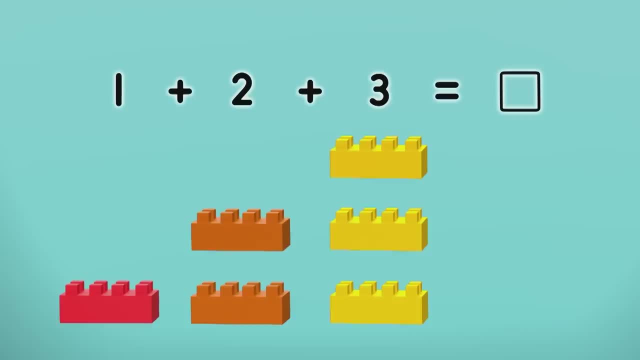 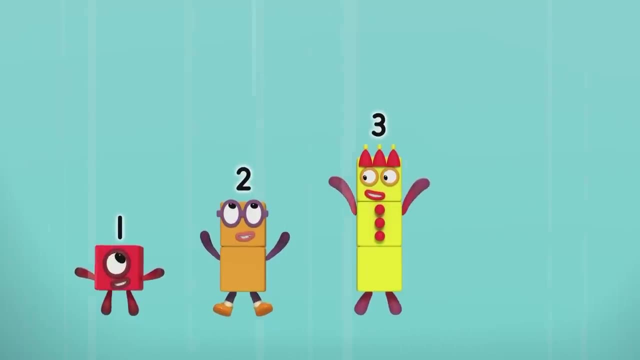 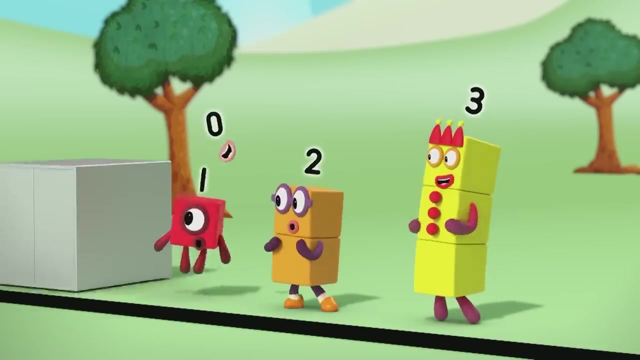 You could count it using pebbles, globs or bricks Or sticks- Good fix. What if there could be a number less than zero? You could draw it on a line to understand, Or imagine there's a lip that keeps on going. Negative one, negative two, negative three.